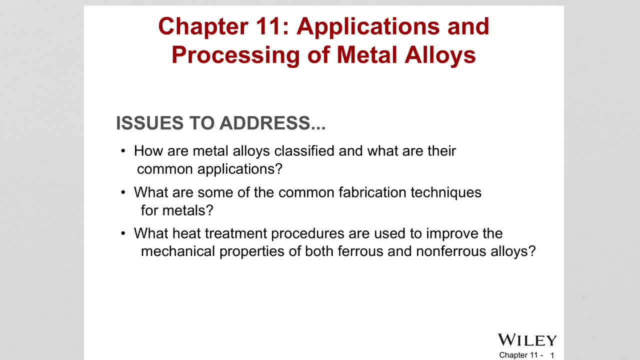 thing is, we look at the properties, and the properties will be changed based on what type of processing technique you are using and it will depend on also the composition of the alloy and it will also depend on if you have applied a heat treatment, because the heat treatment will change the. 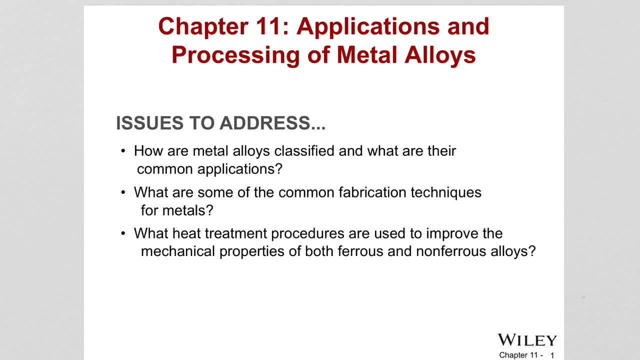 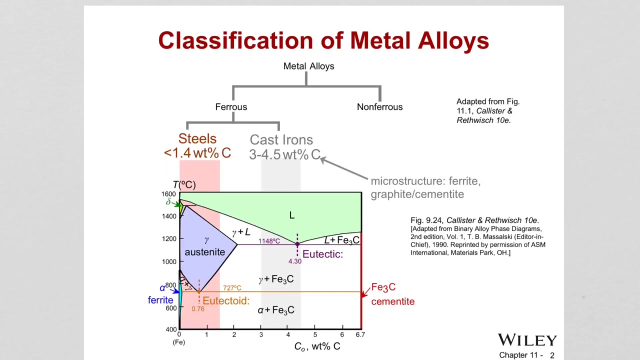 microstructure, therefore the properties. So we all gonna see these: how fabrication techniques affect properties of materials and how heat treatments will change the properties for alloys, metal alloys and how we classify metal alloys. Metal alloys: they are classified into two classes: One is ferrous and other is. 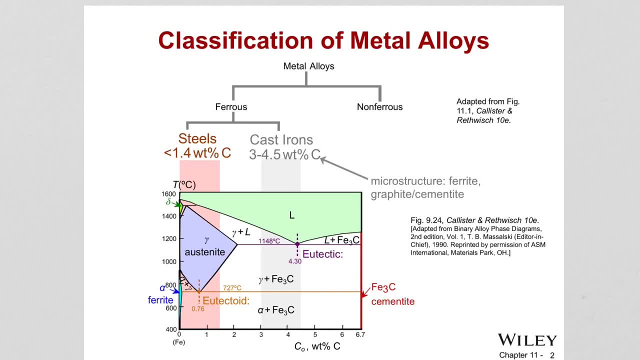 non-ferrous and the ferrous alloys are those which has iron as the main component. These are divided also into two categories. There is steels and cast irons. So ferrous alloys: they are very important engineering materials And why? There are three reasons why ferrous alloys are very important. 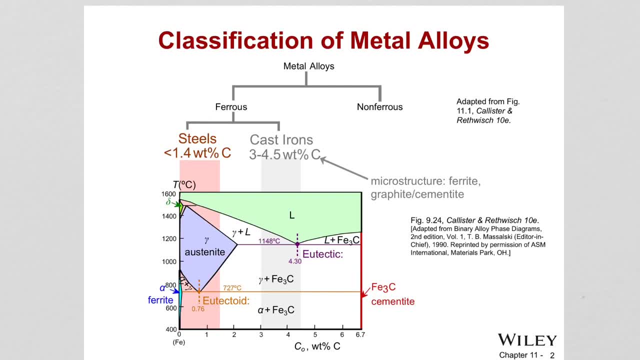 First of all, iron is the abundant within the earth's crust And, secondly, iron and steel alloys can be produced with economical manufacturing techniques. And ferrous alloys are very versatile, Meaning they are very important, Meaning they are very important And properties can easily be changed with different processing techniques, different heat treatments, different compositions. 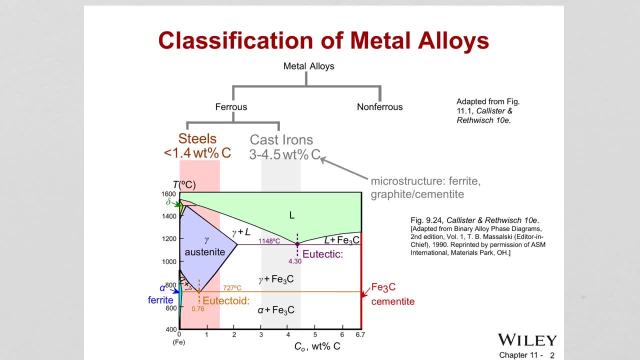 You can come up with a wide range of alloys- ferrous alloys- that will have a wide range of properties which might be suitable for your applications. So the bad thing about ferrous alloys are they are susceptible to corrosion. So the difference between steels and cast irons is in their carbon content. 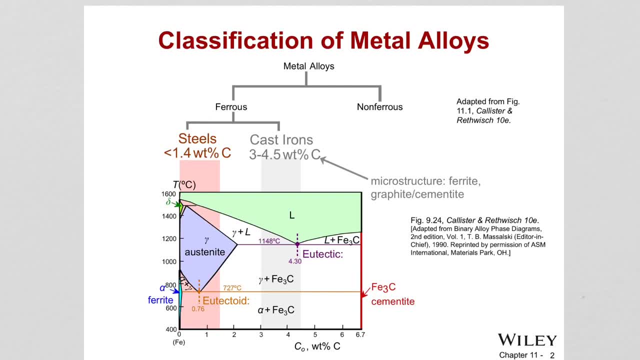 As you see, the pink region in the iron-carbon phase diagram represents the steels. which steels have carbon content lower than 1.4%, Whereas cast irons they have higher carbon content. They have a higher amount of carbons, which shown with the gray region in the phase diagram and it is between 3 to 4.5% carbon. 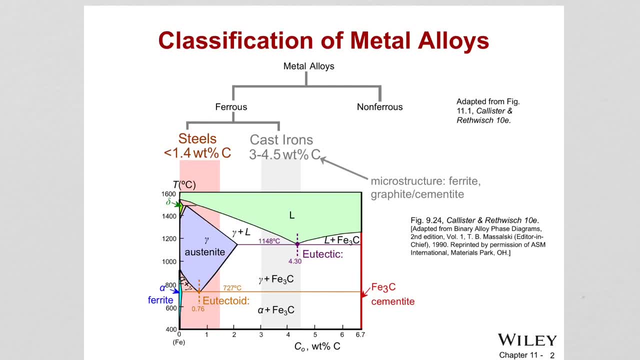 And the microstructure of it is ferrite, graphite and cementite. So ferrite is cementite is actually what we call an unstable phase, meaning with a little bit of trigger, some energy, that will convert into a more stable phase. 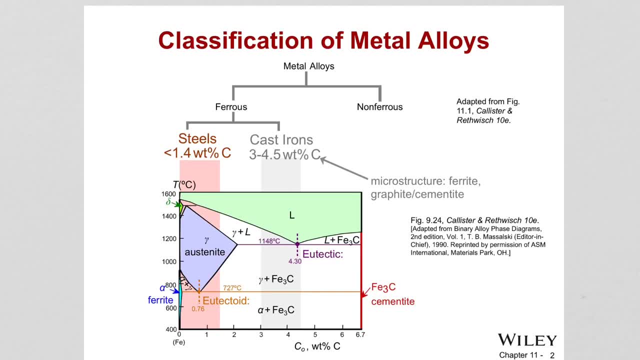 So ferrite is cementite is actually what we call an unstable phase, meaning with a little bit of trigger, some energy that will convert into a more stable phase. So ferrite is cementite is actually what we call an unstable phase, meaning with a little bit of trigger, some energy that will convert into a more stable phase. 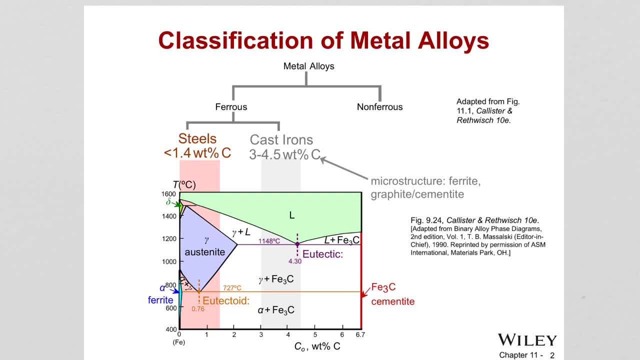 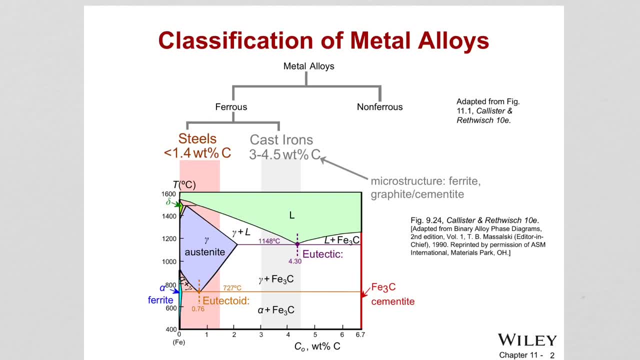 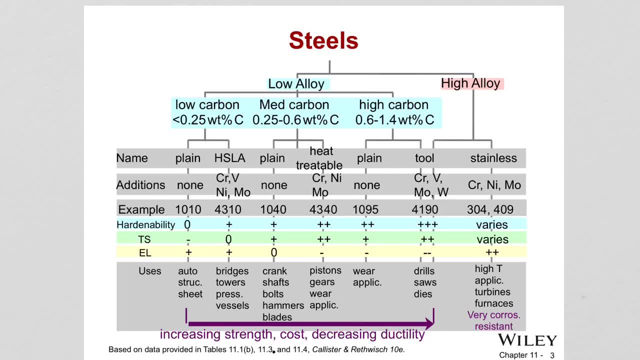 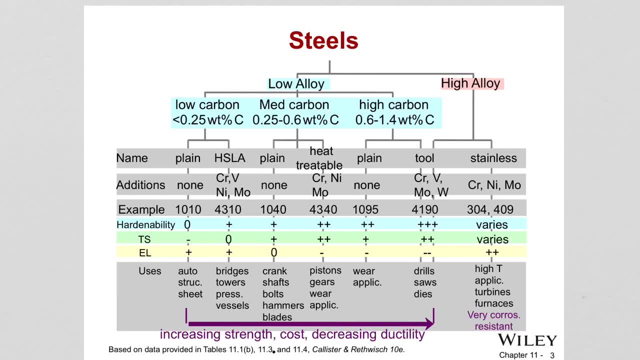 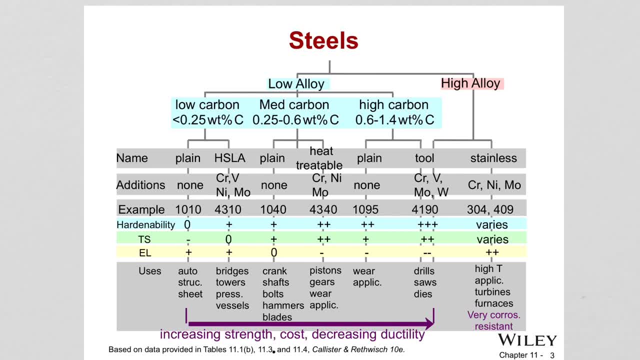 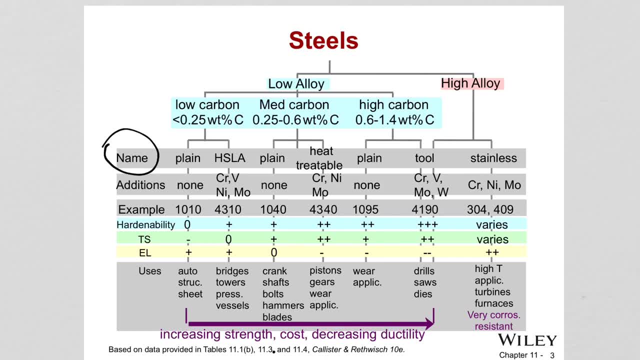 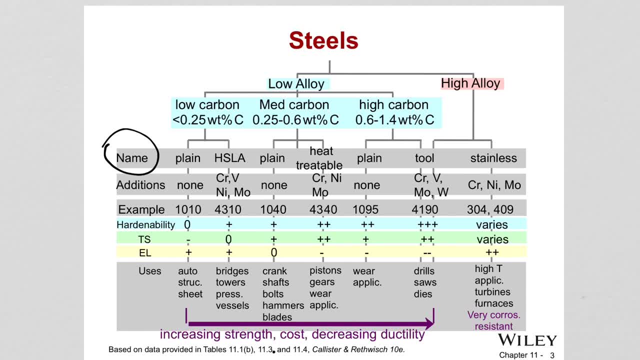 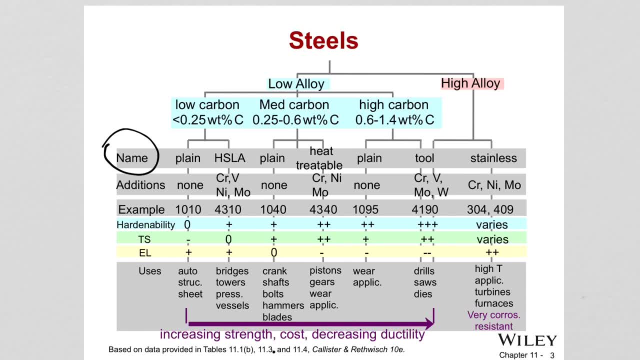 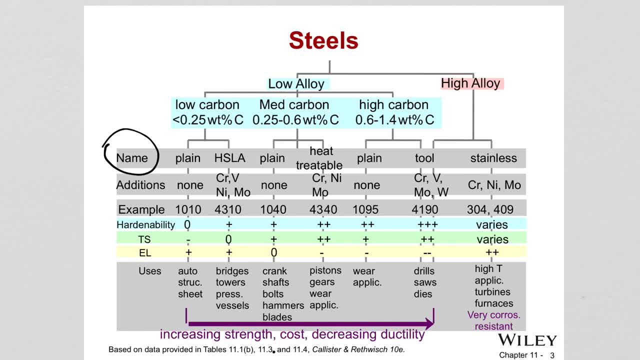 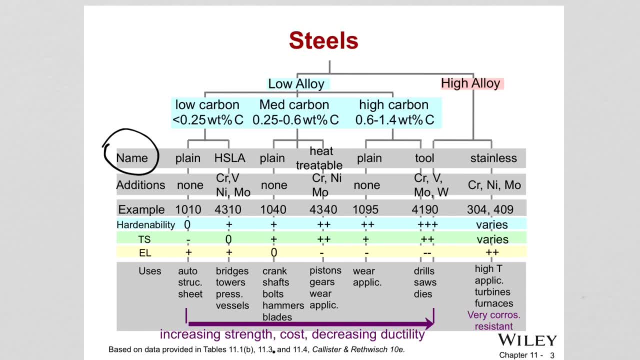 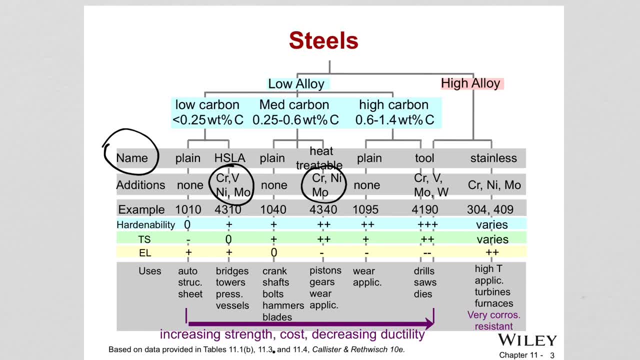 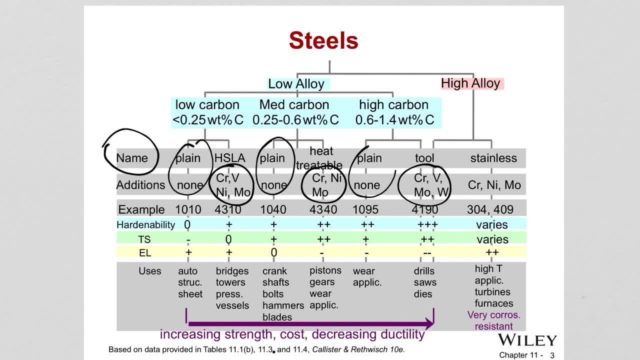 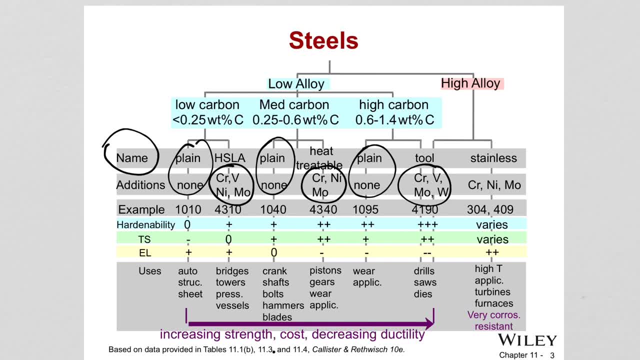 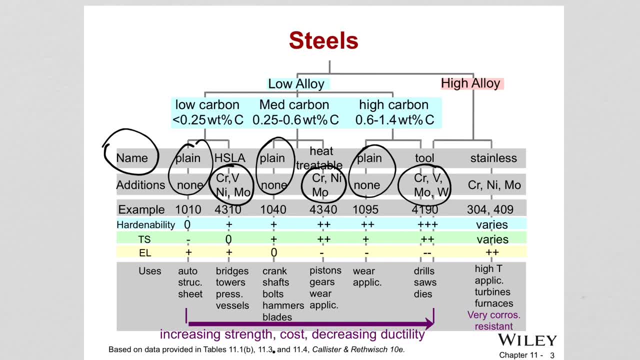 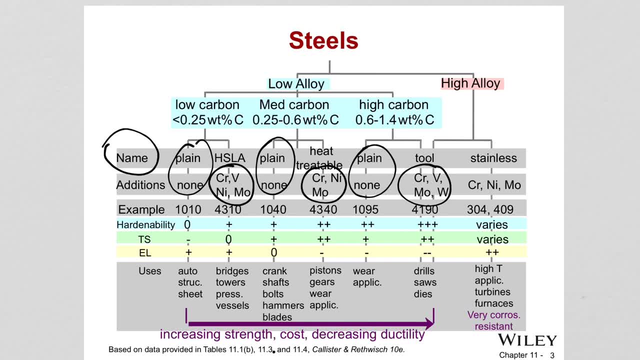 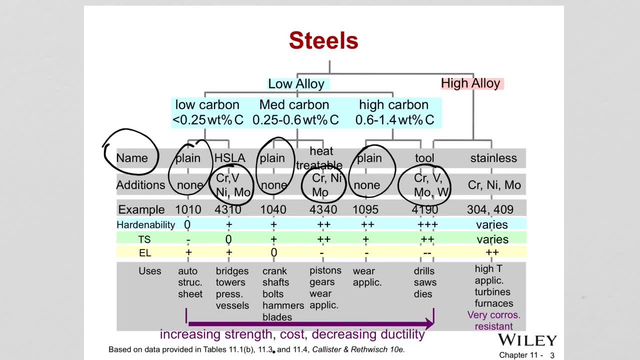 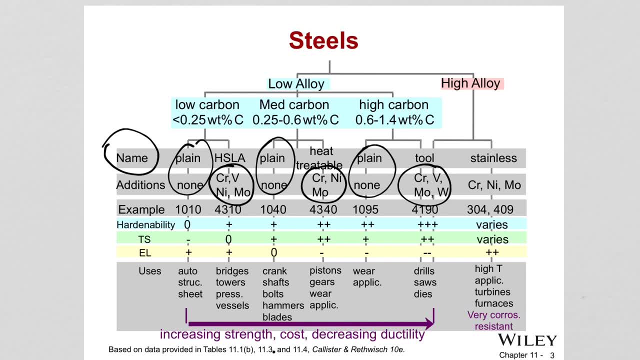 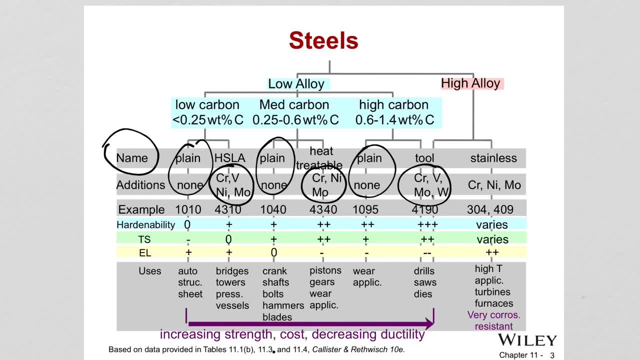 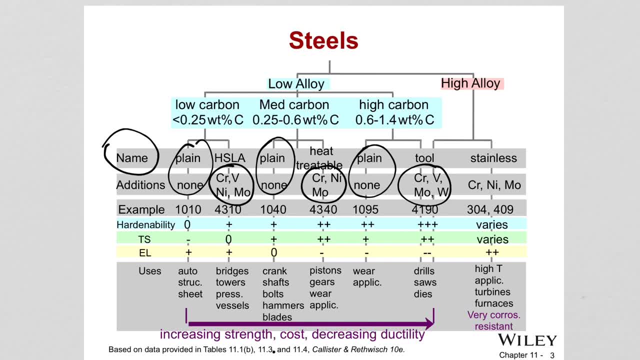 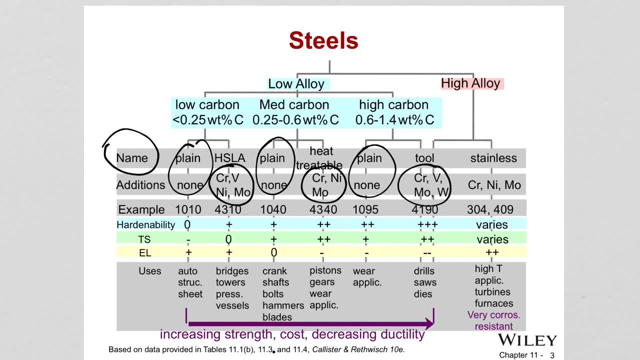 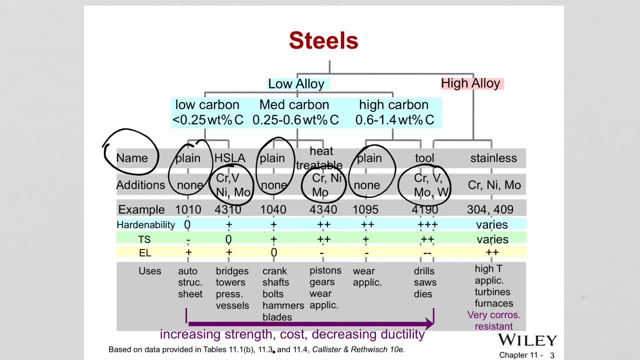 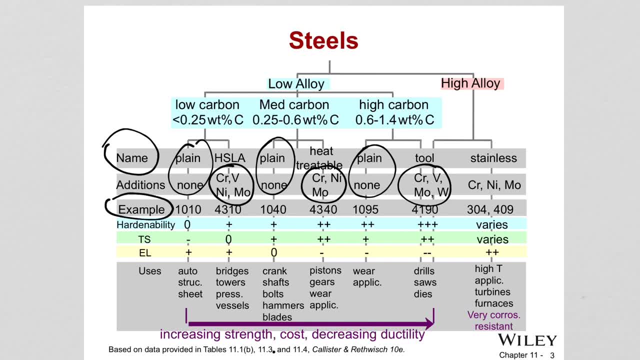 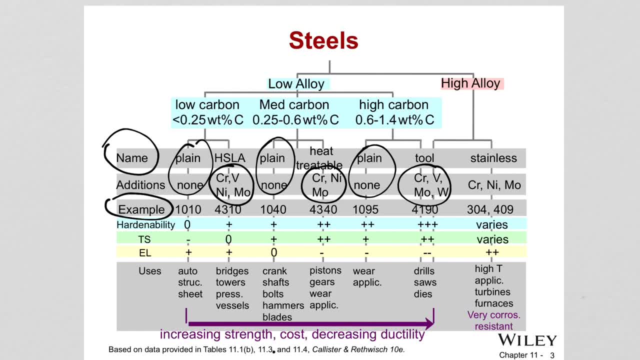 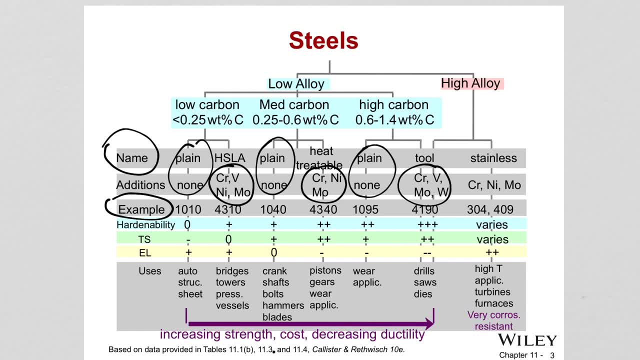 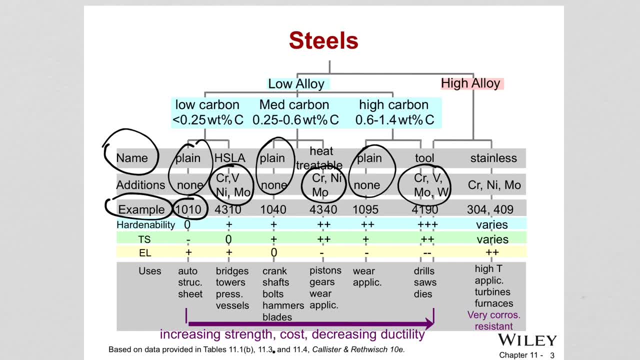 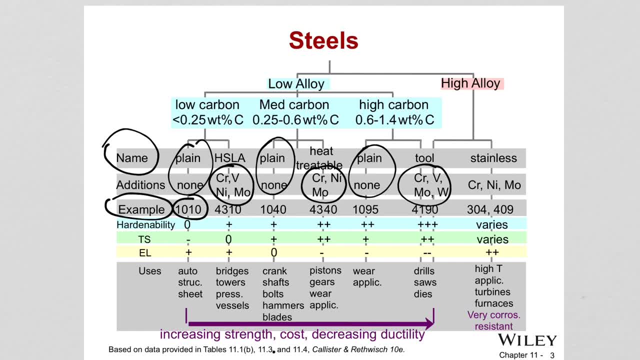 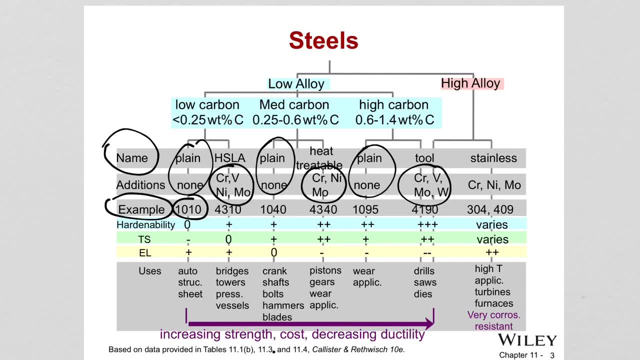 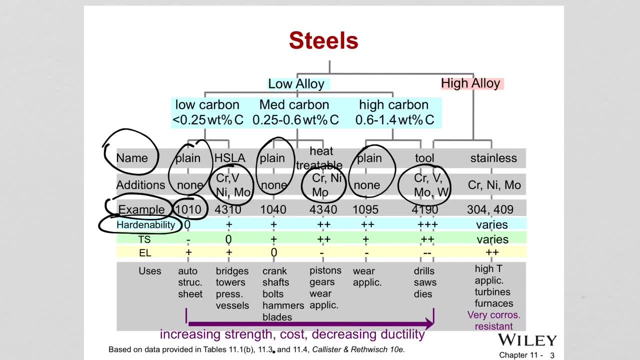 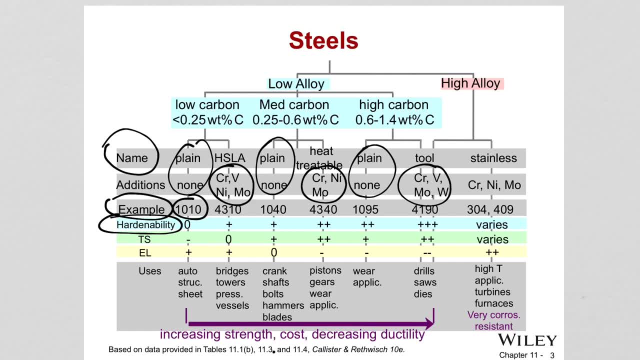 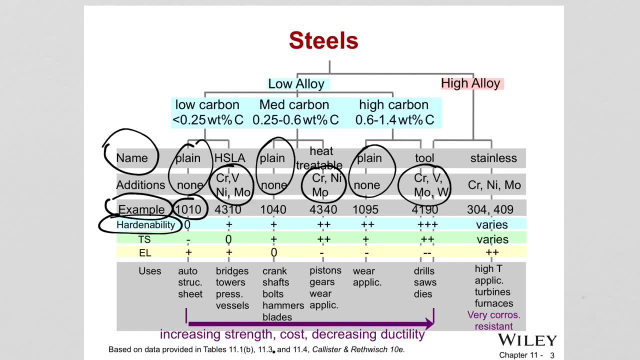 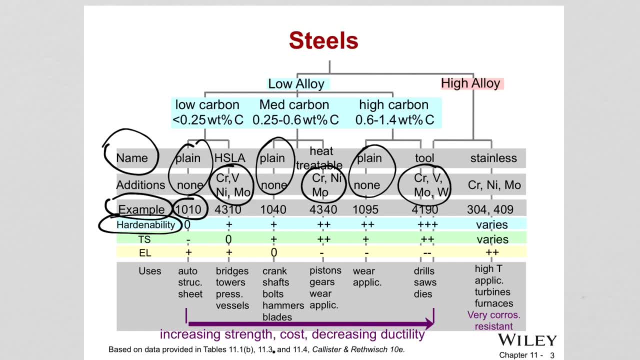 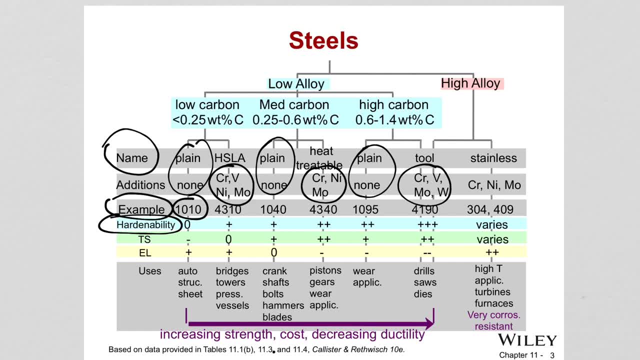 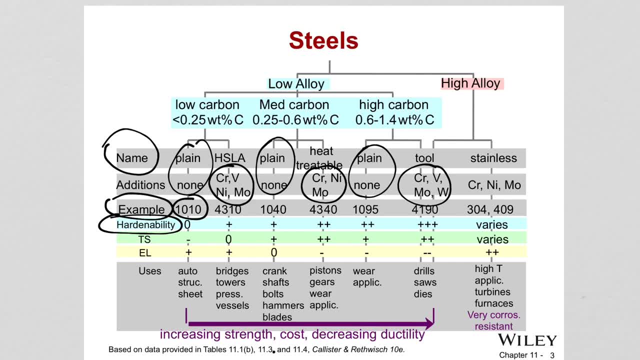 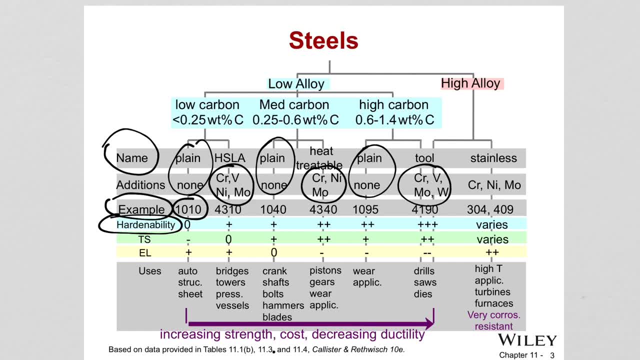 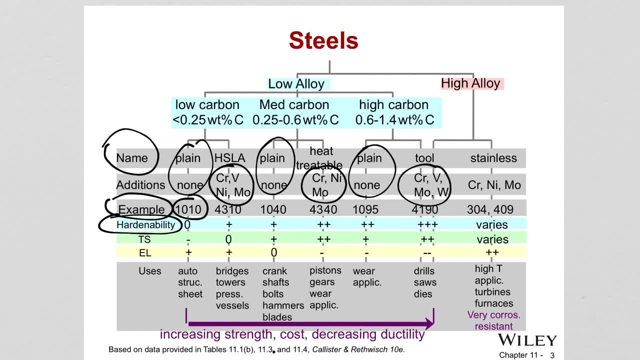 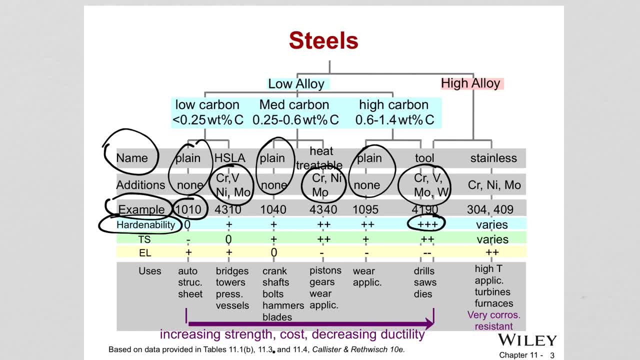 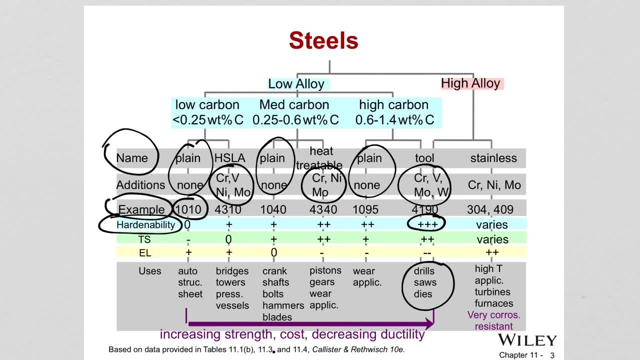 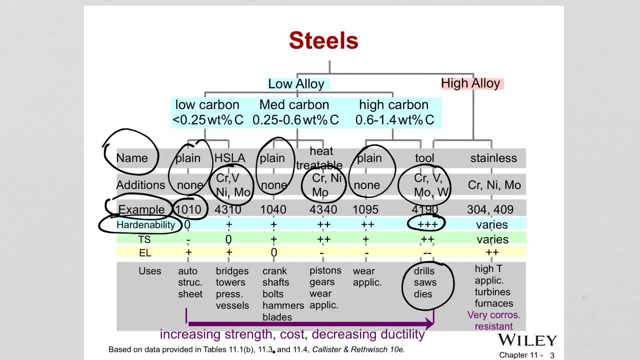 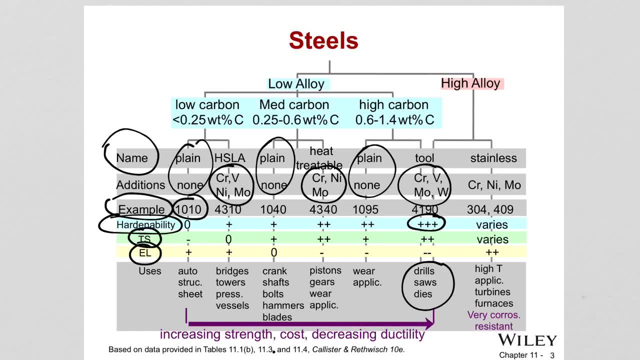 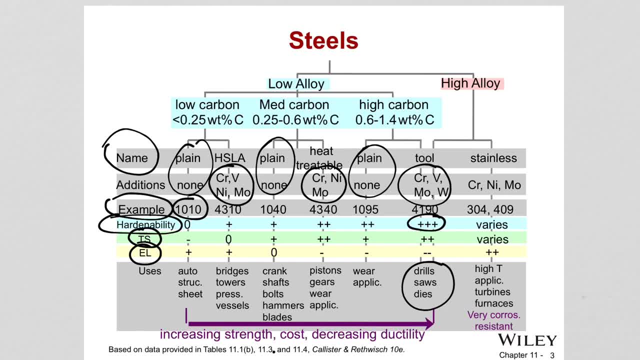 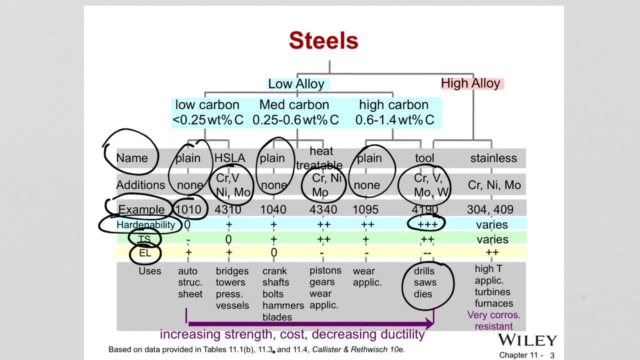 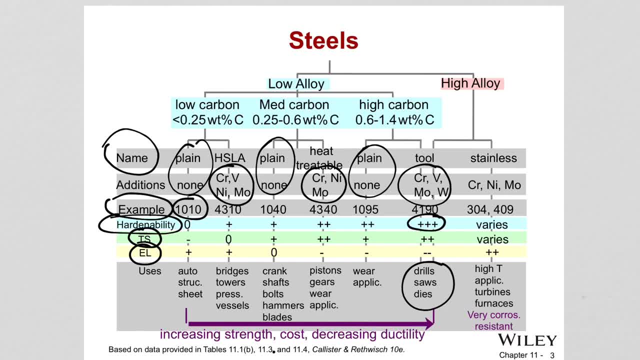 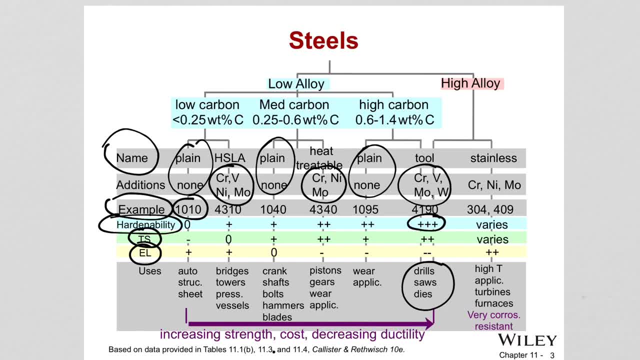 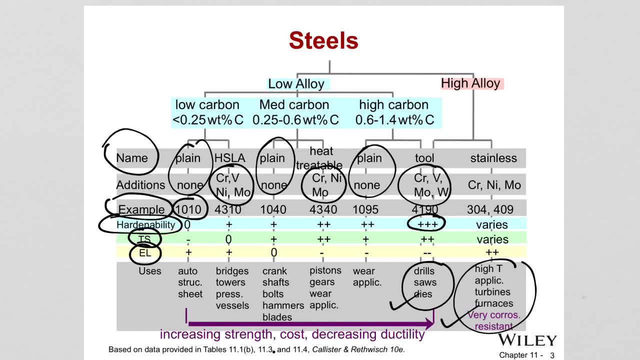 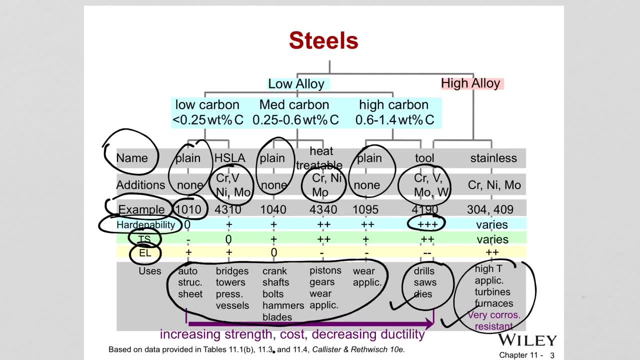 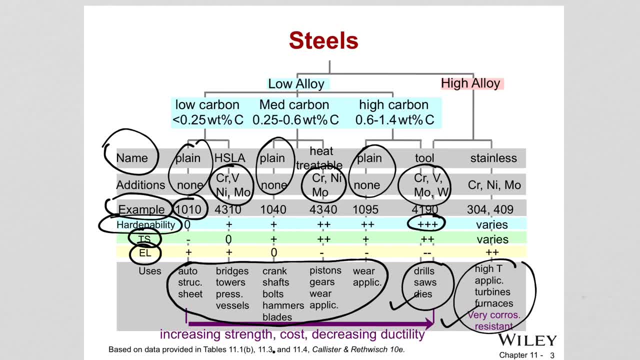 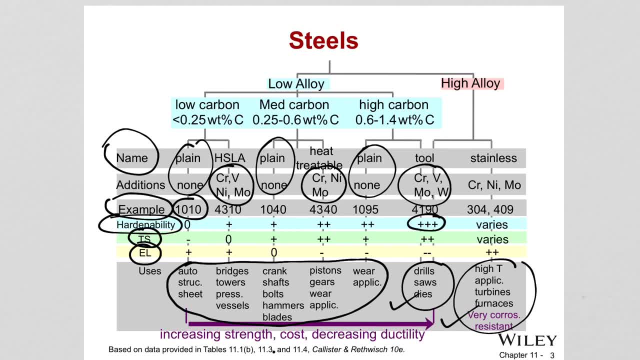 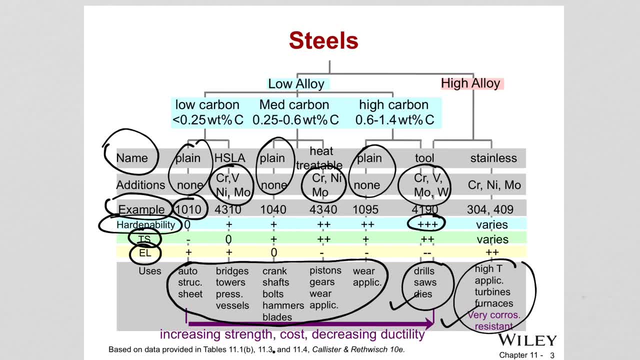 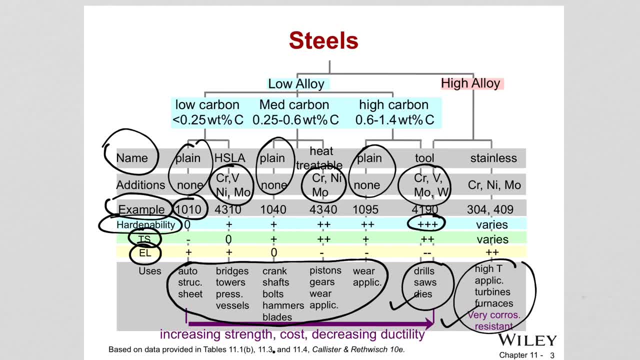 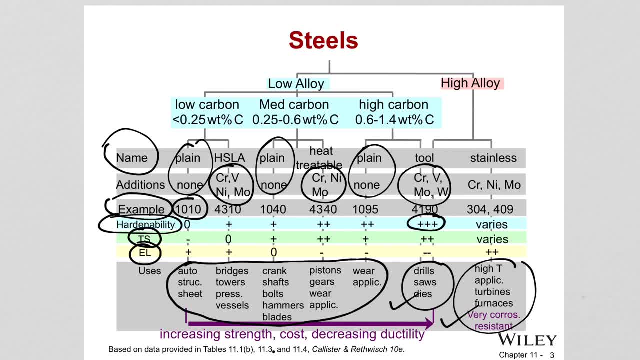 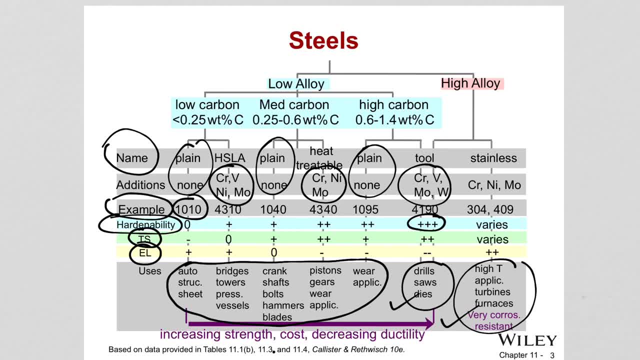 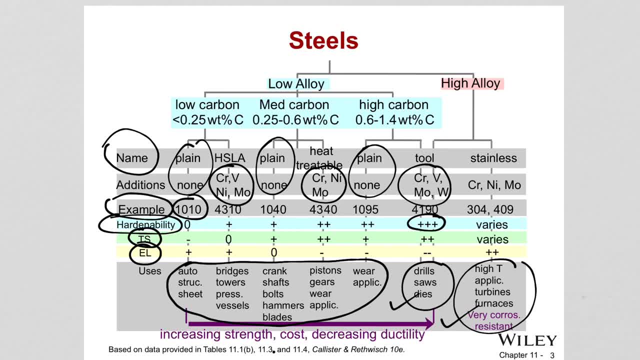 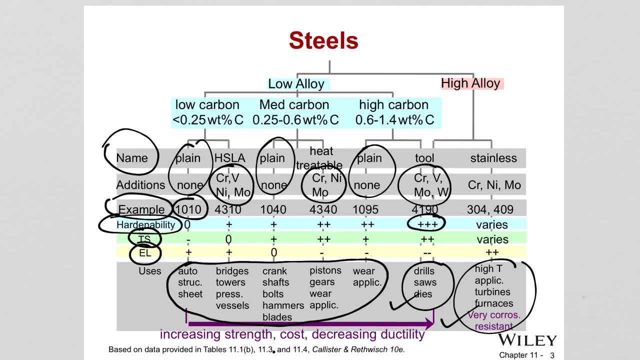 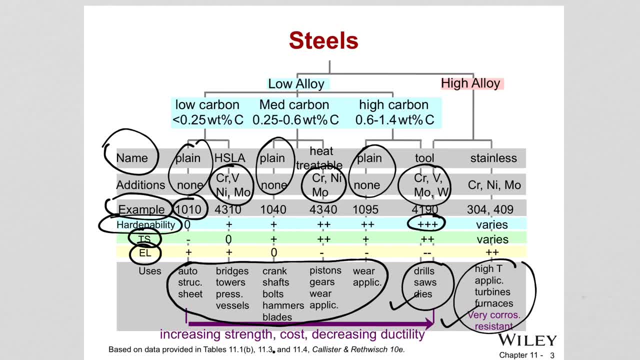 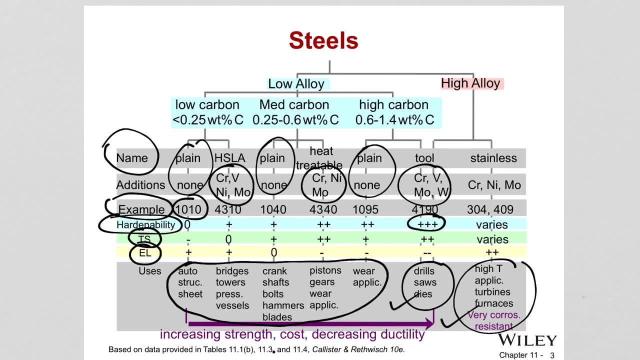 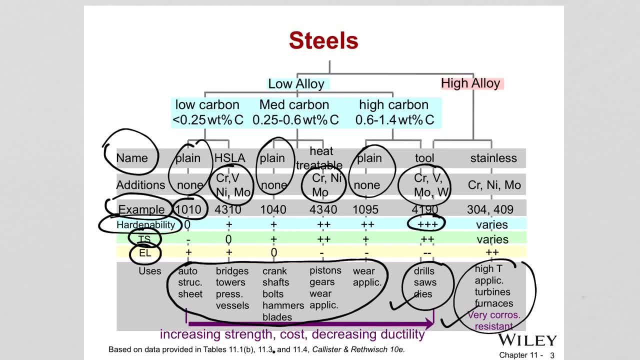 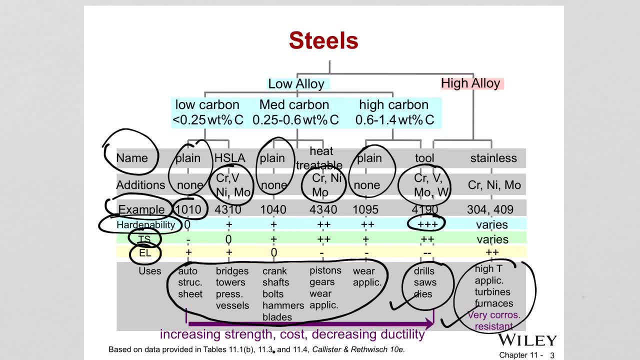 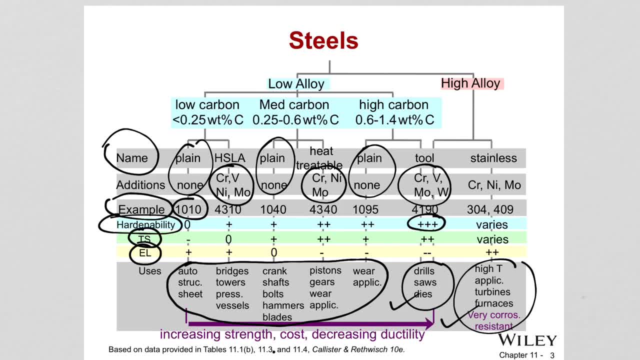 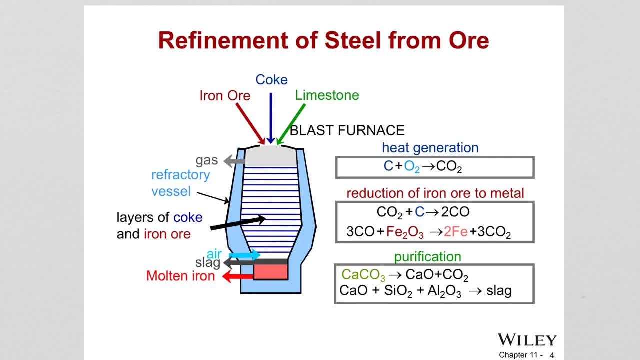 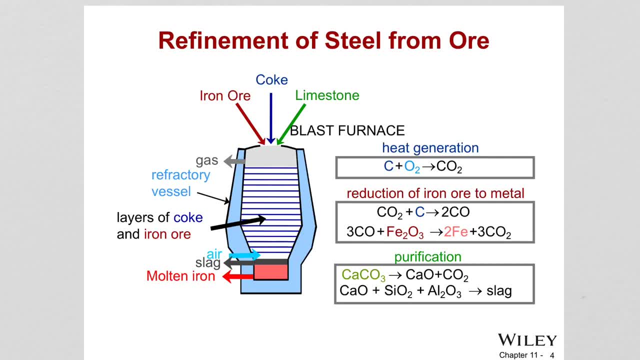 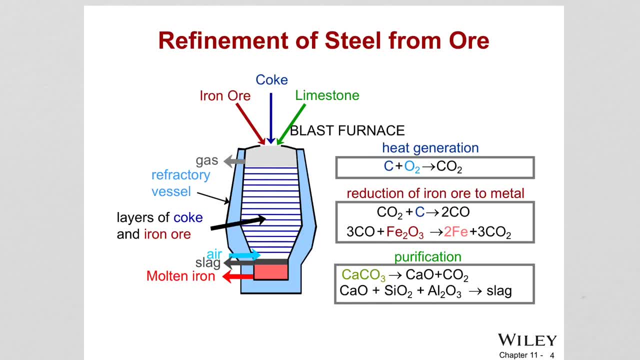 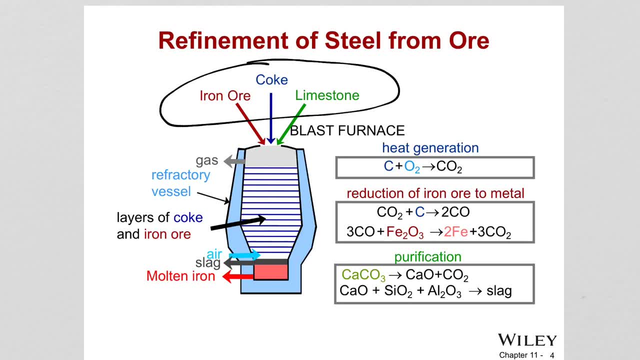 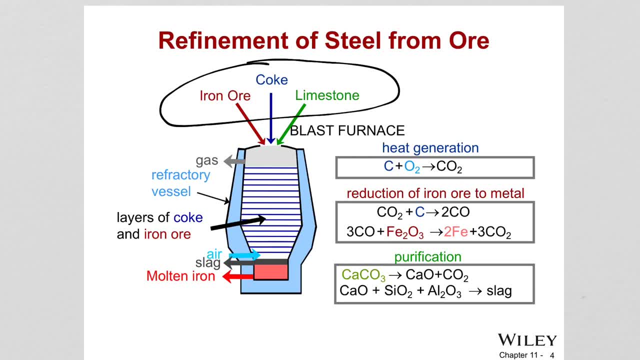 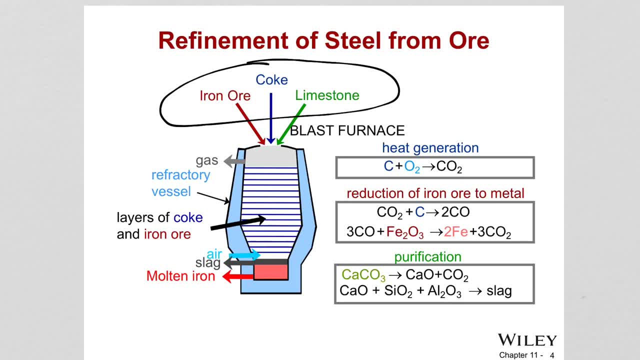 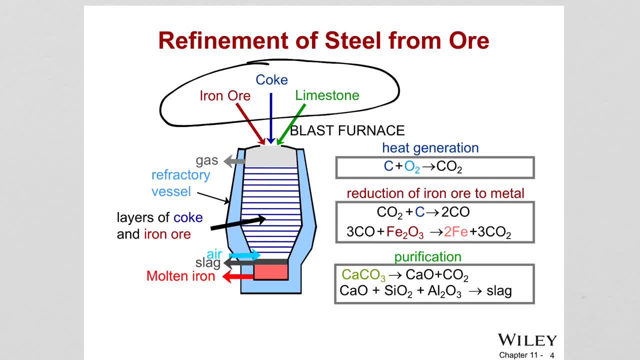 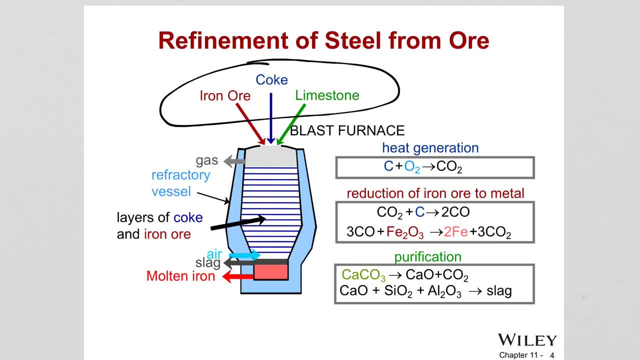 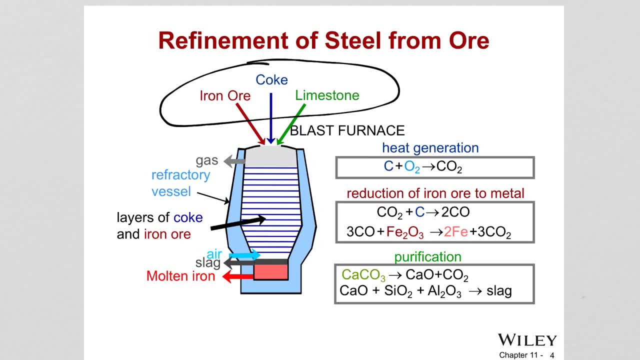 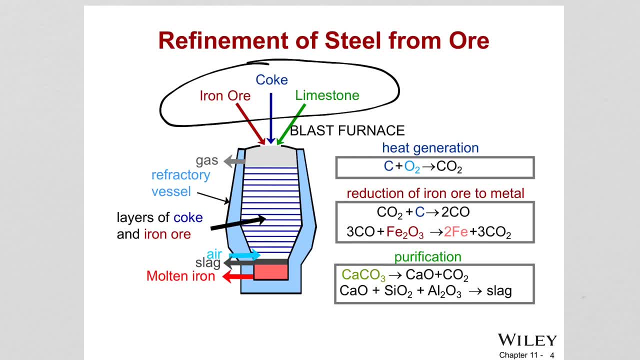 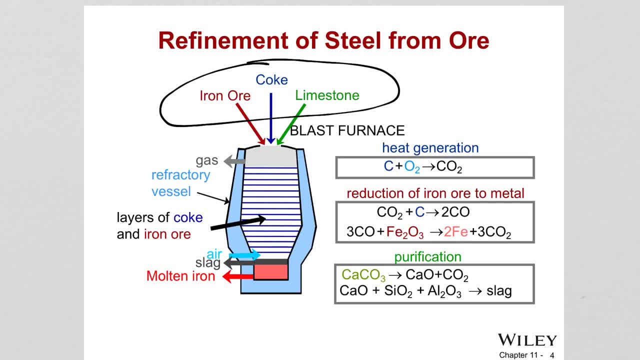 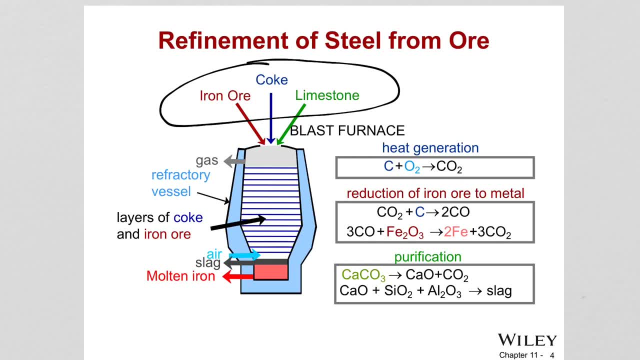 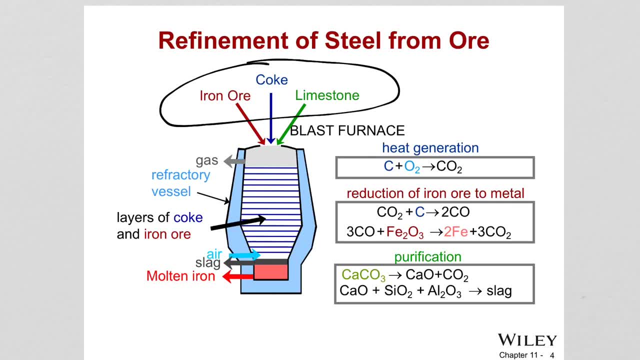 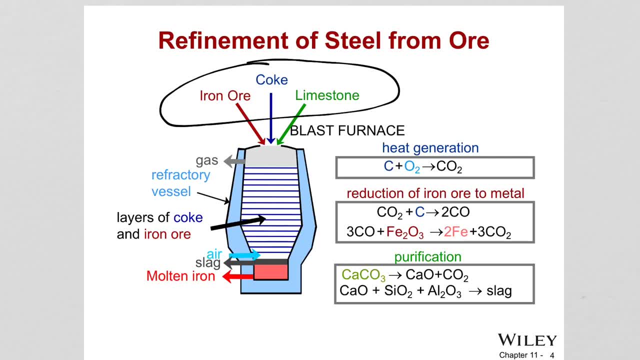 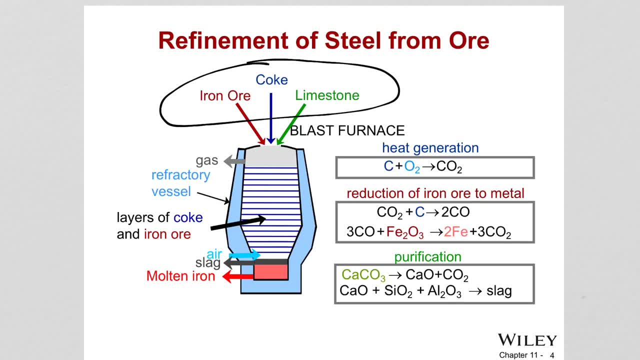 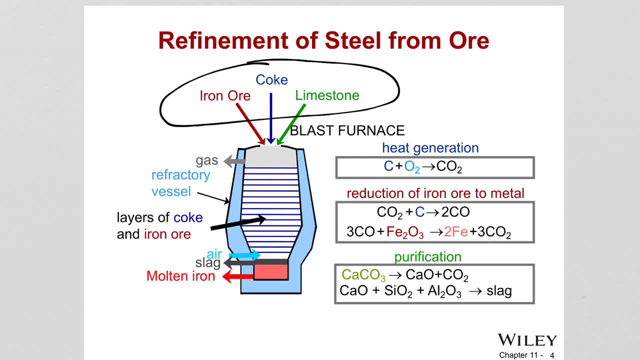 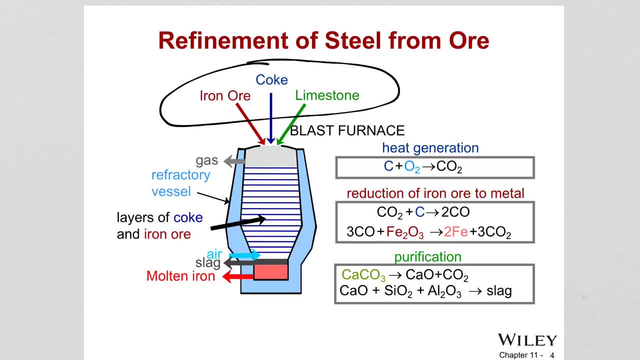 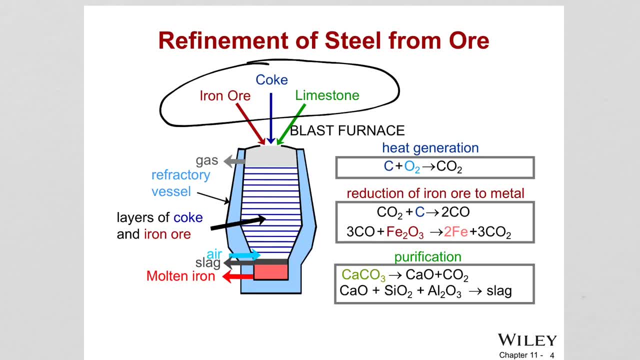 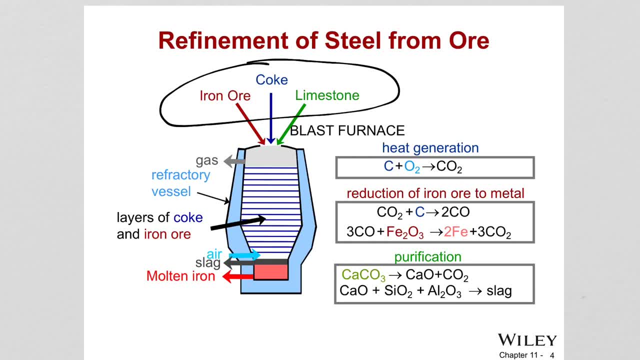 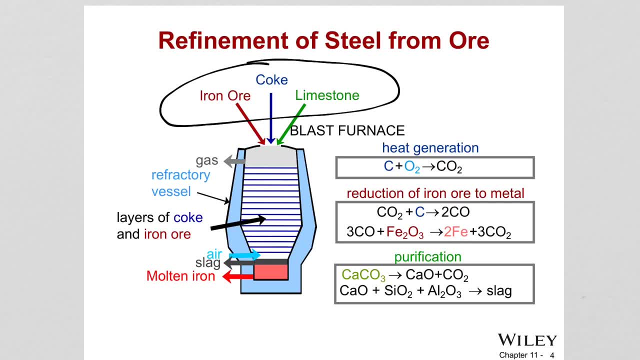 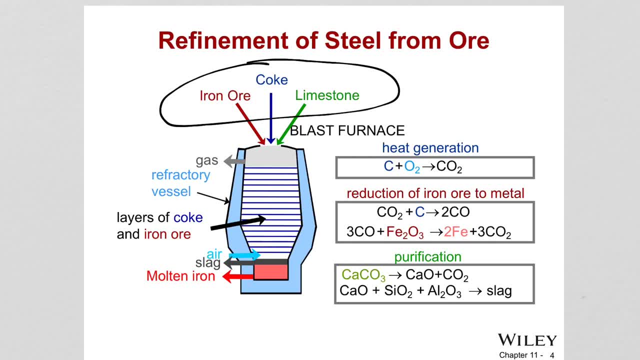 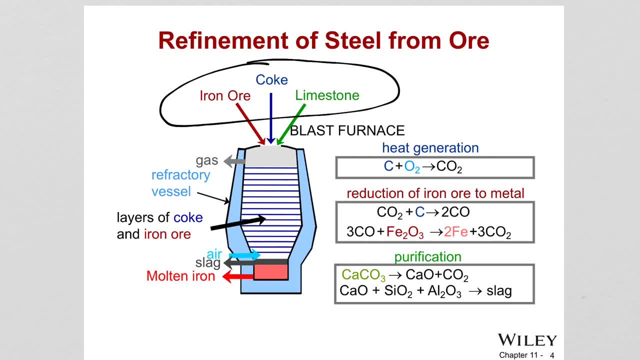 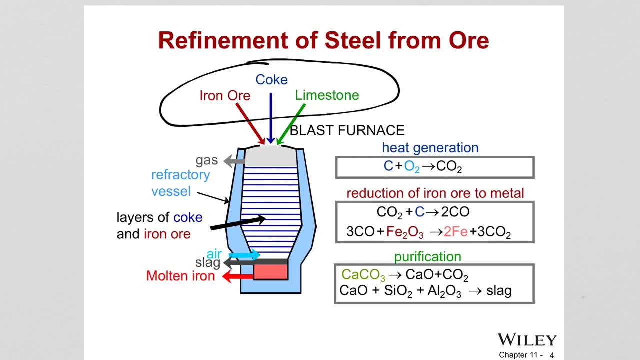 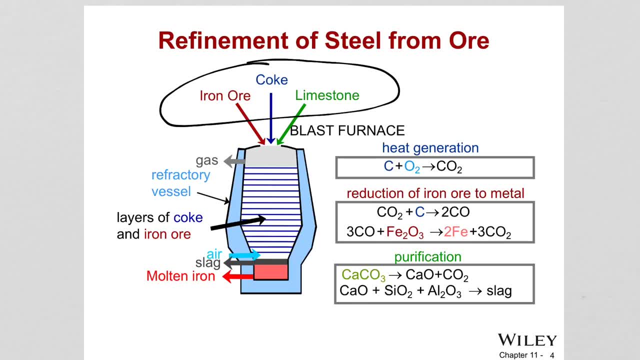 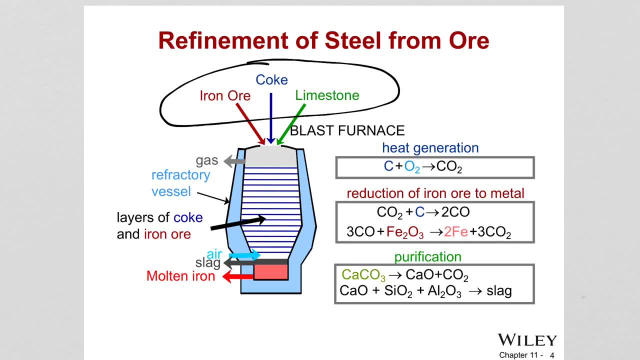 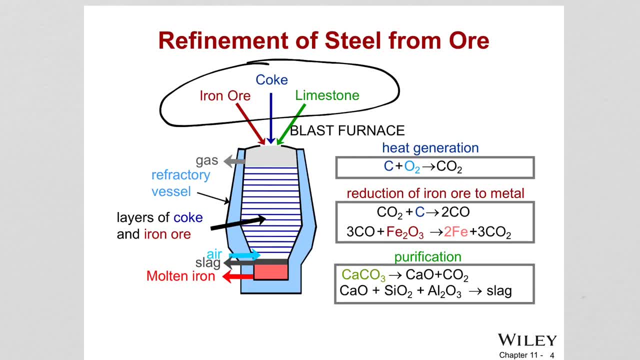 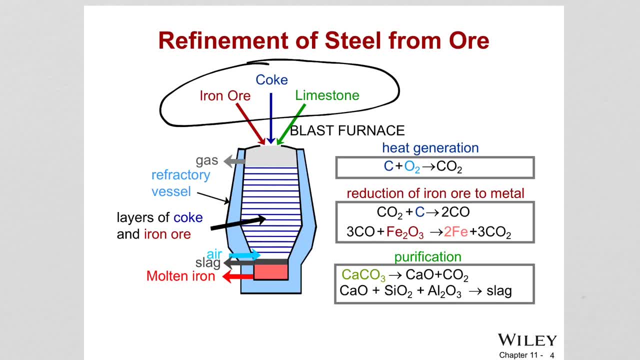 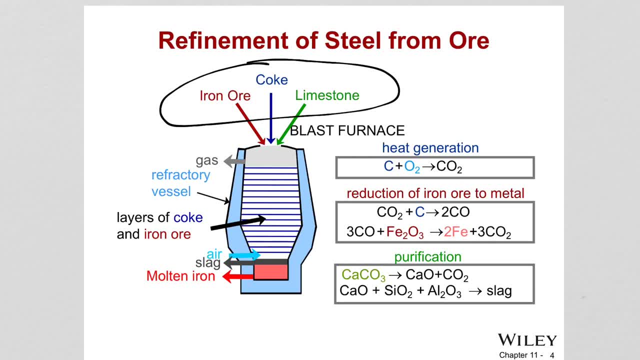 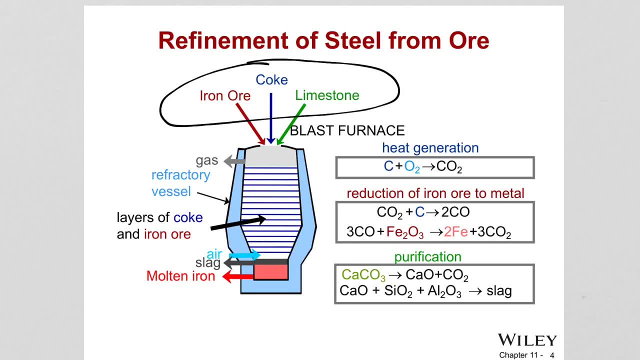 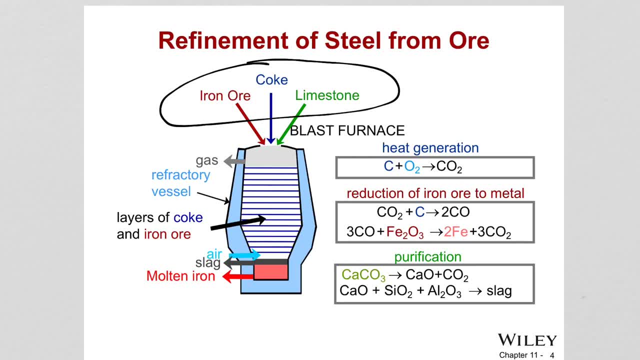 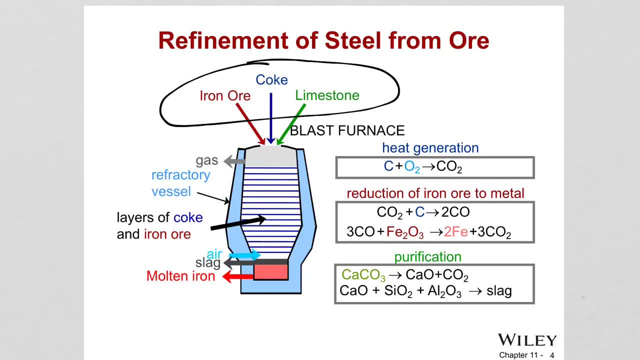 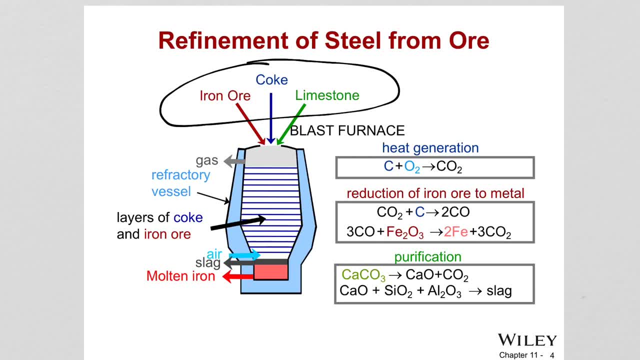 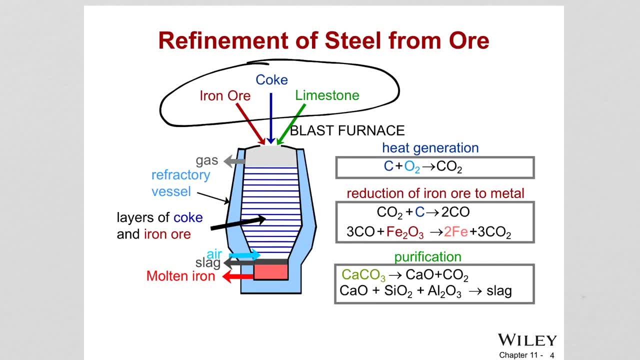 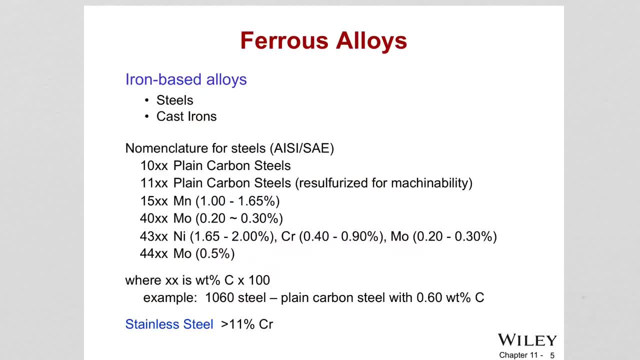 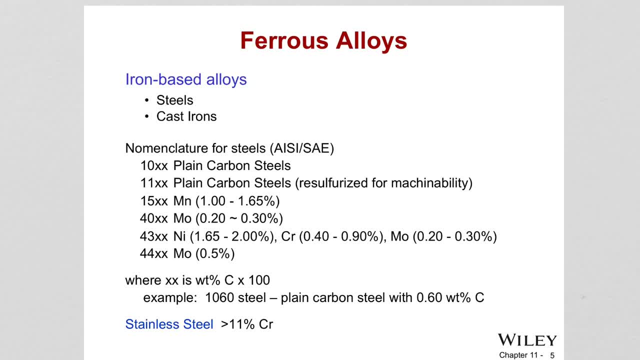 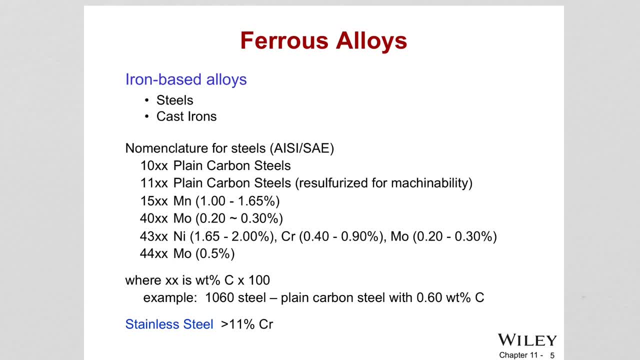 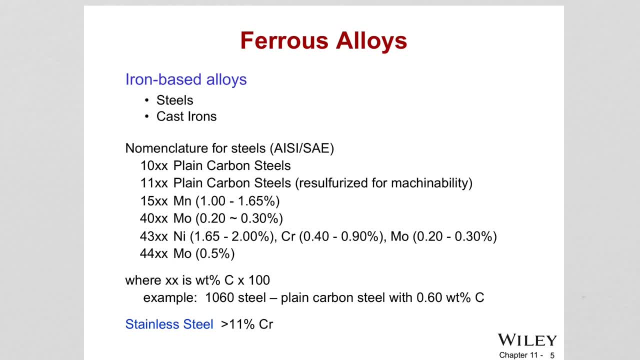 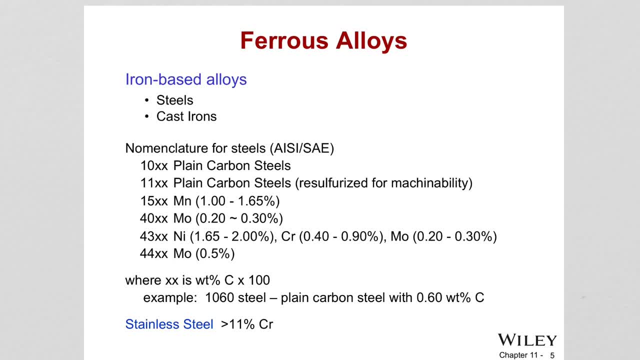 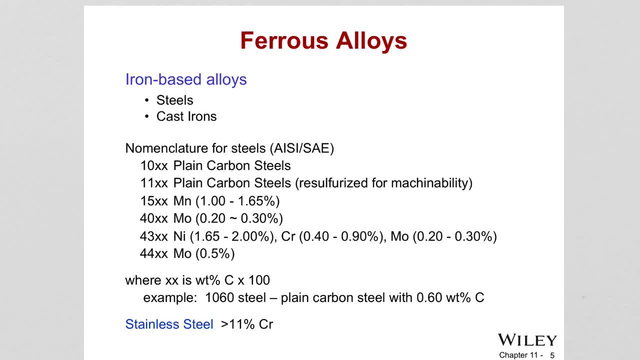 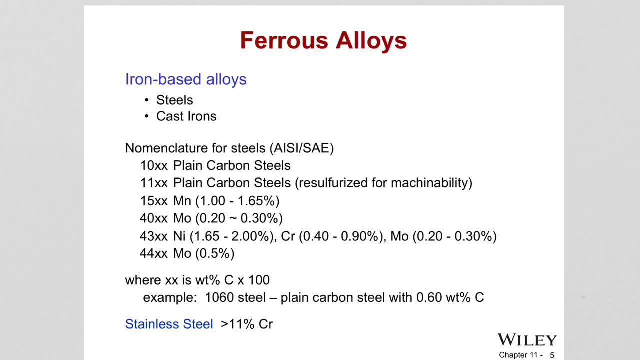 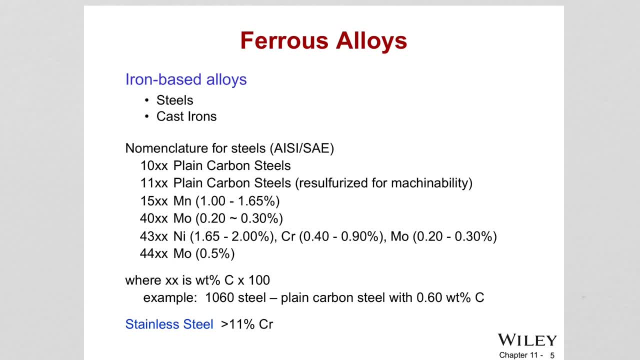 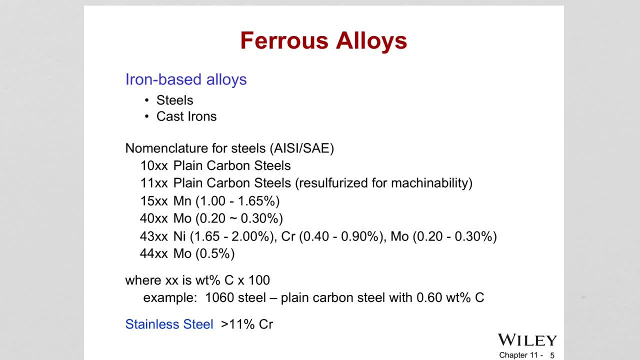 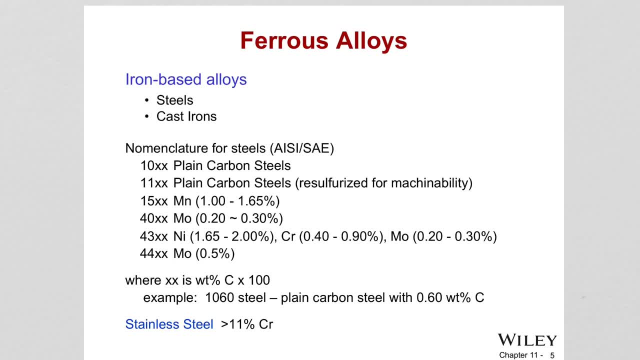 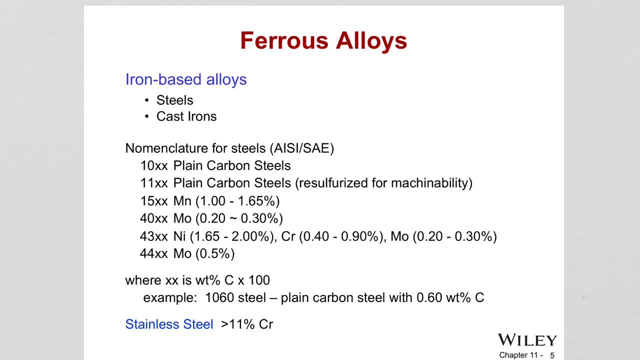 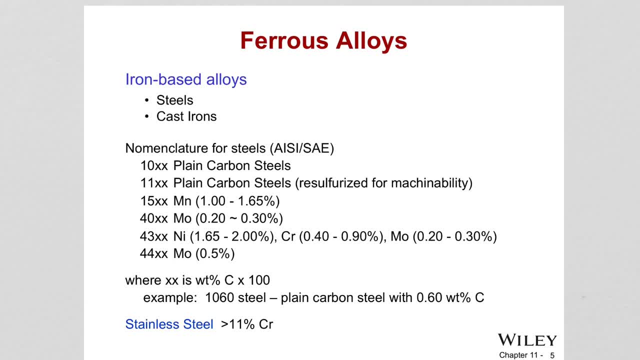 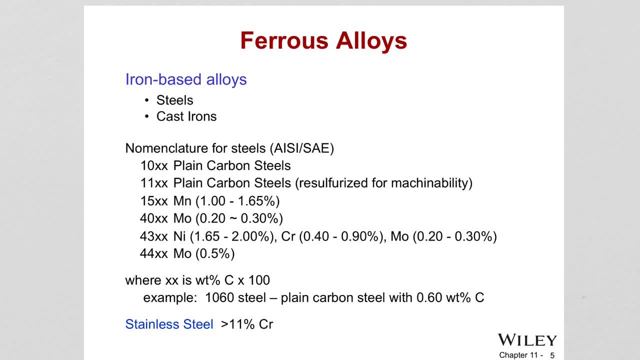 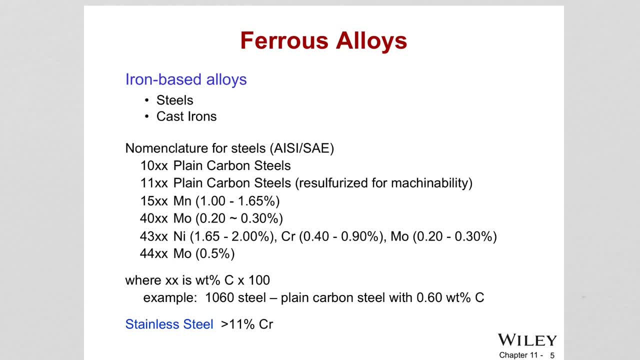 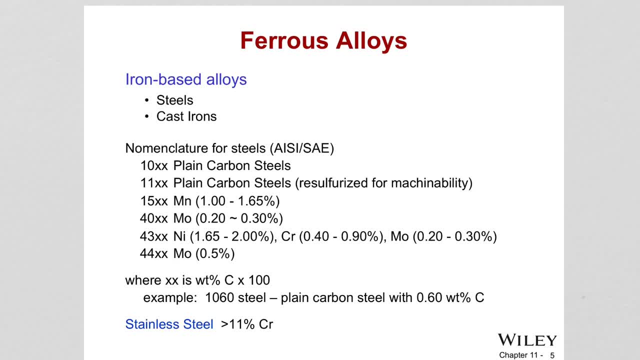 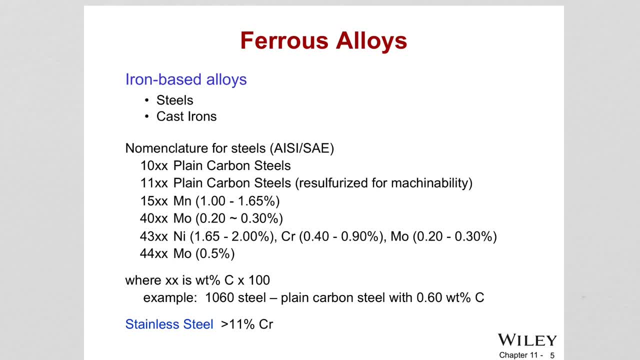 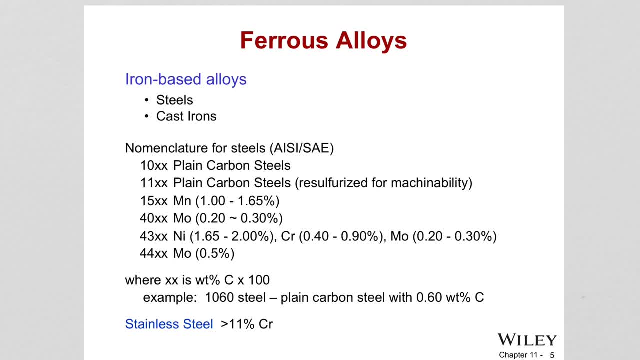 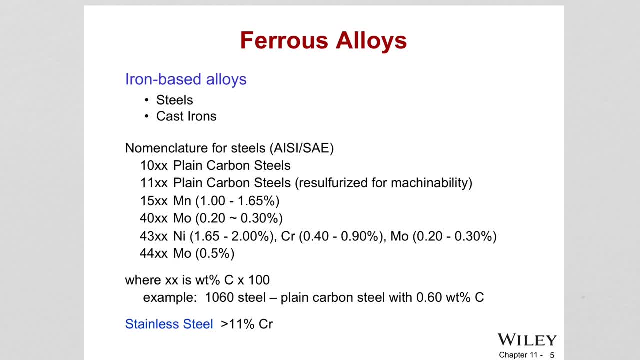 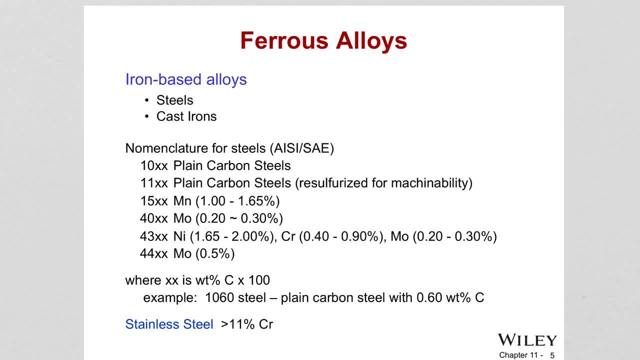 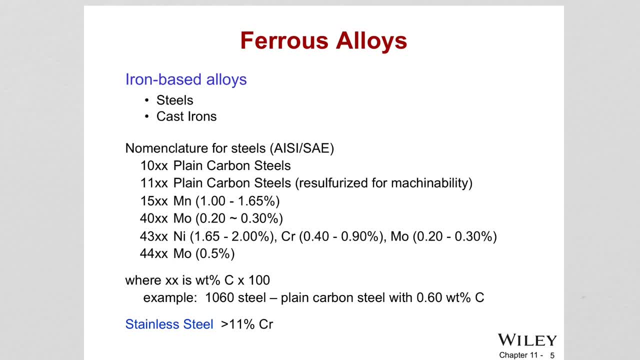 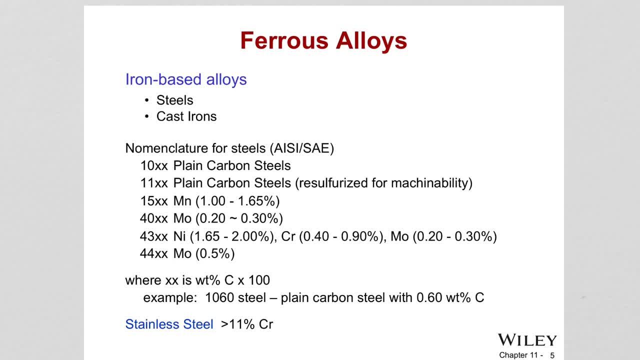 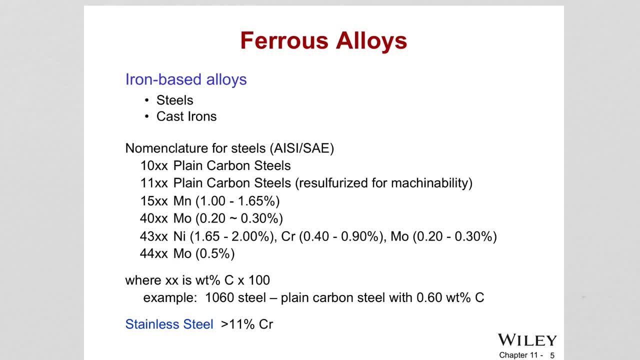 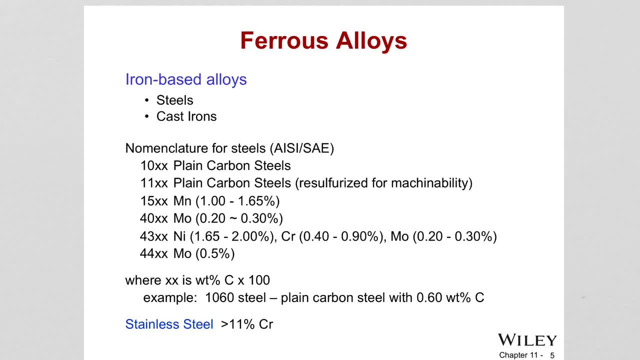 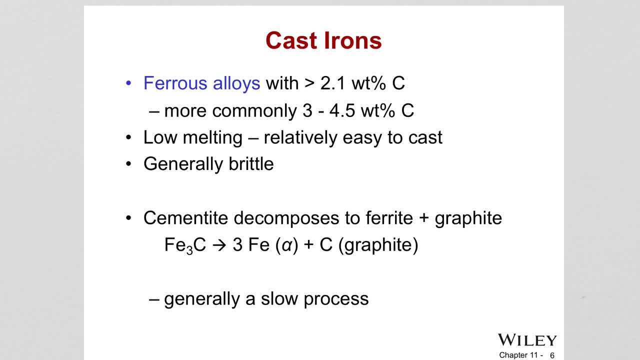 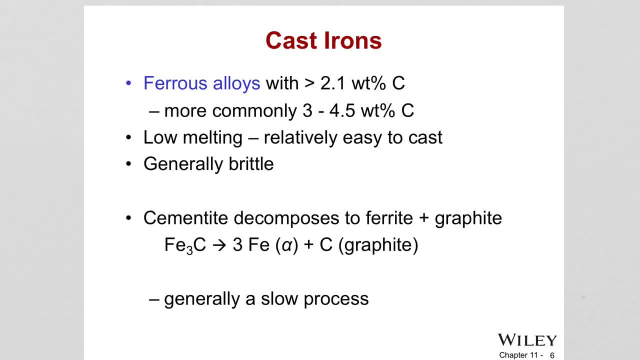 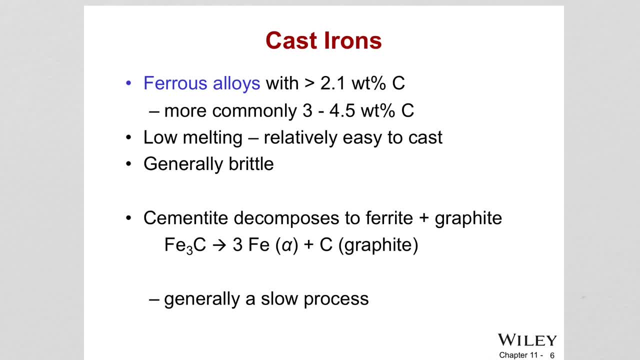 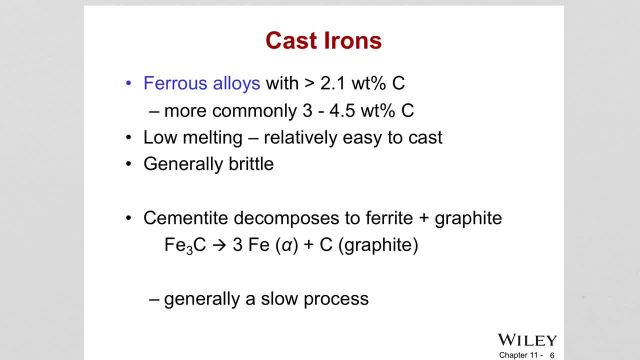 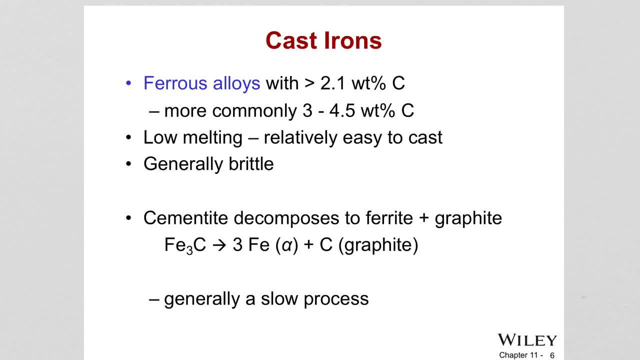 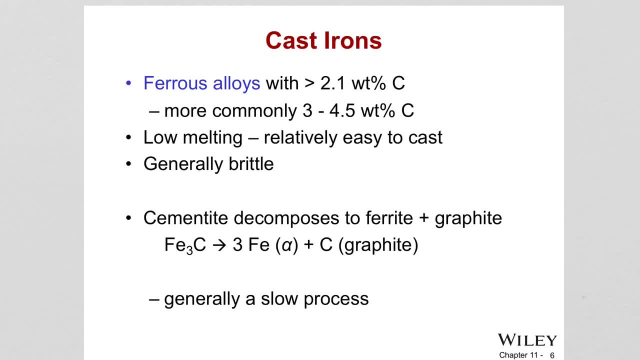 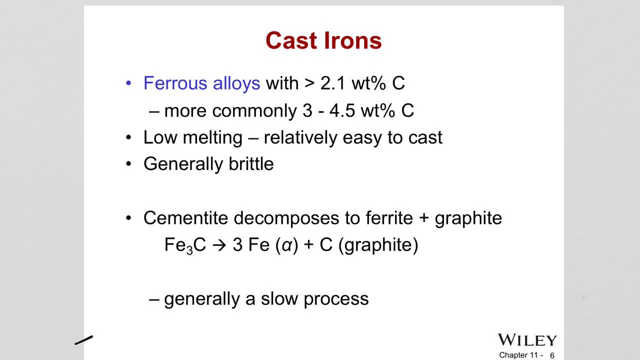 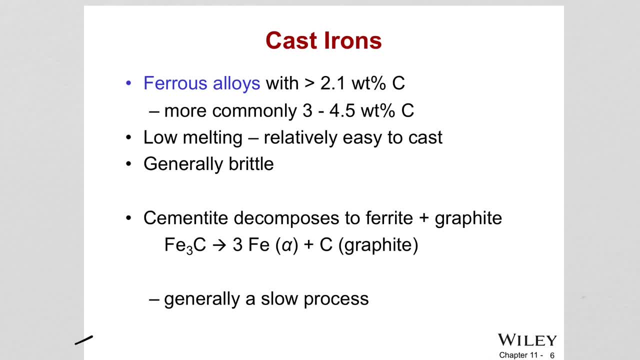 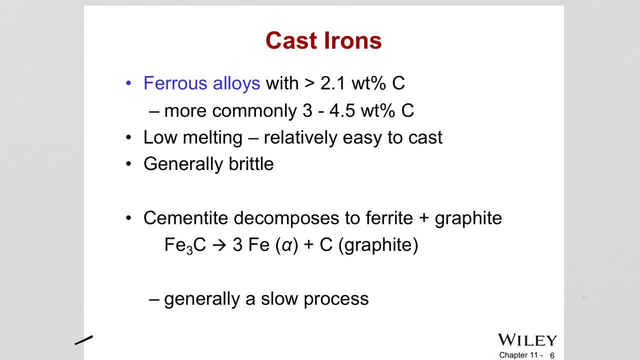 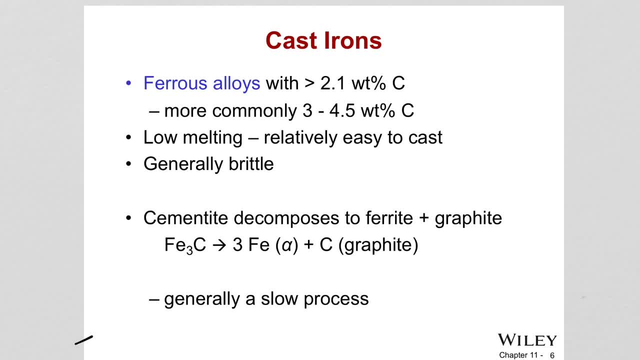 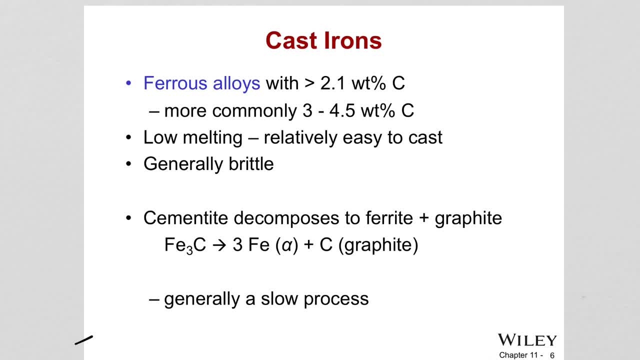 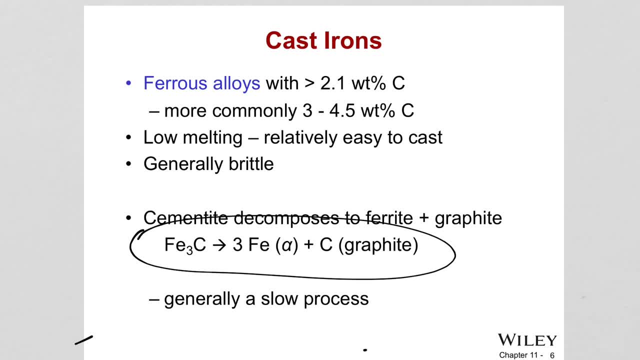 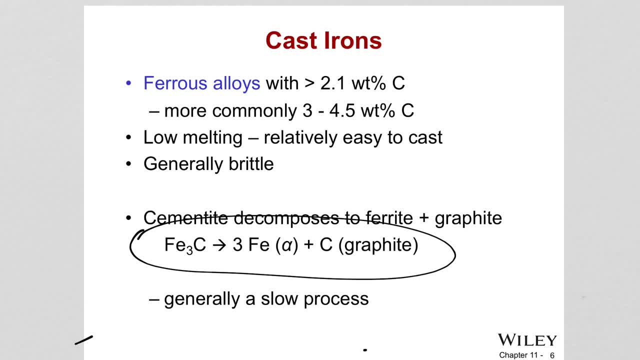 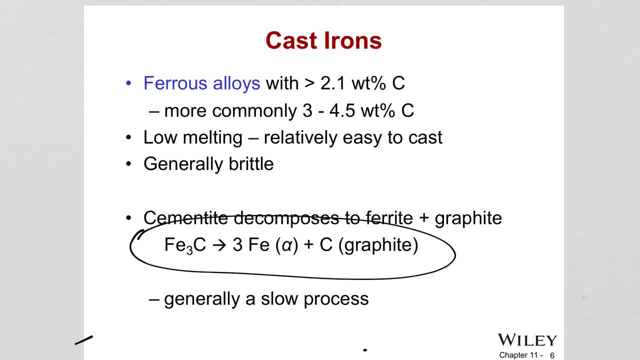 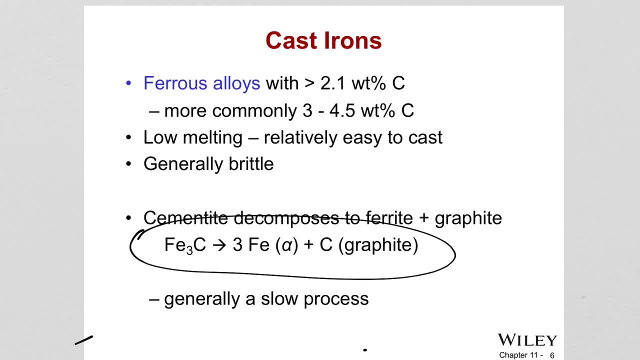 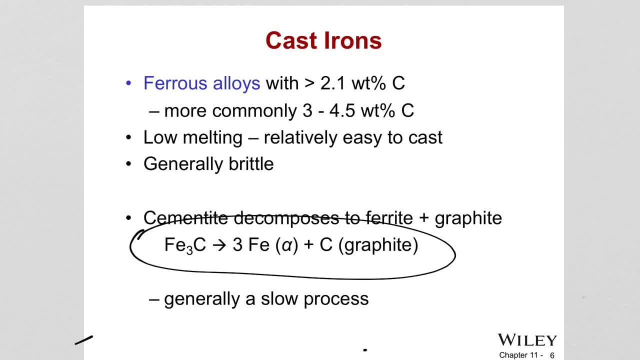 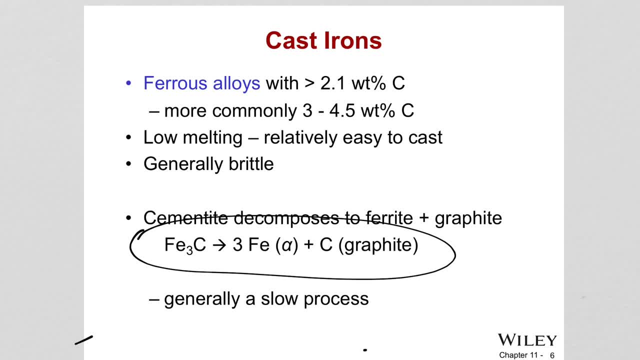 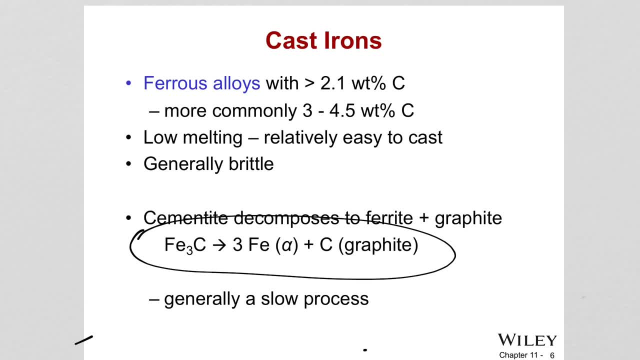 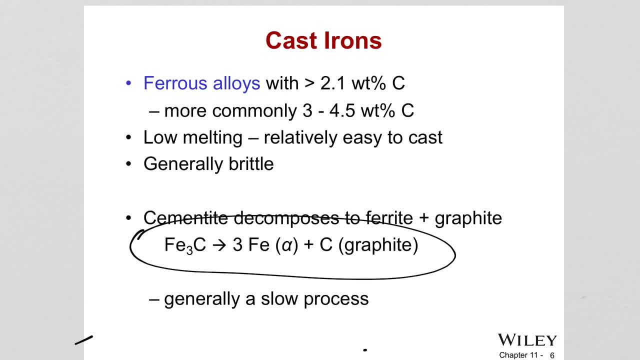 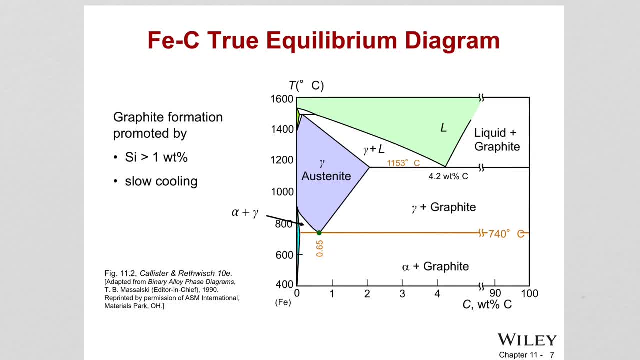 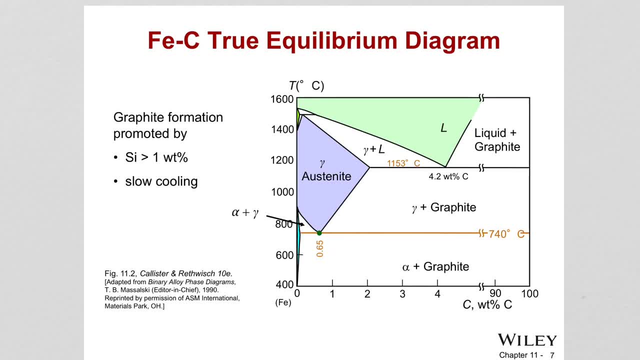 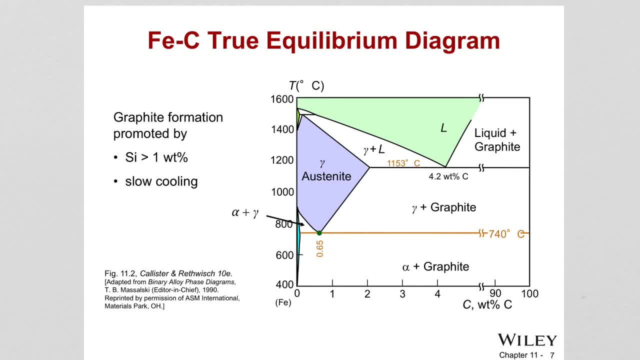 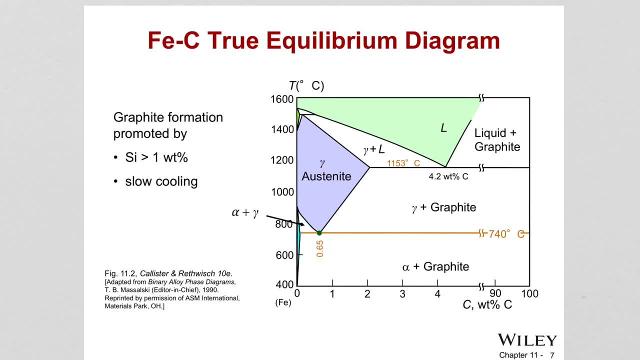 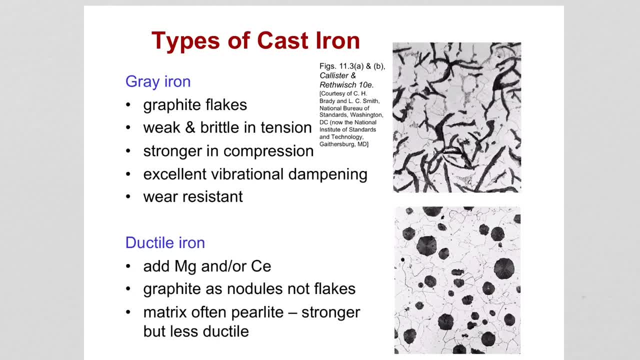 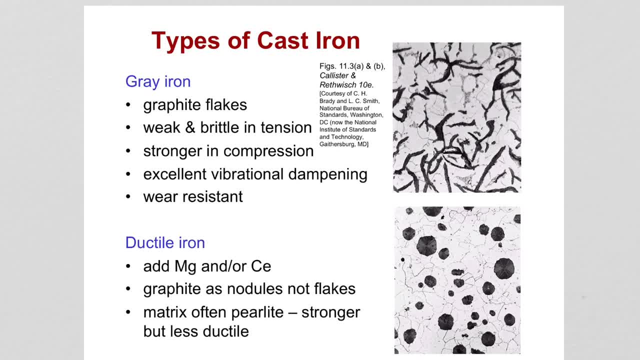 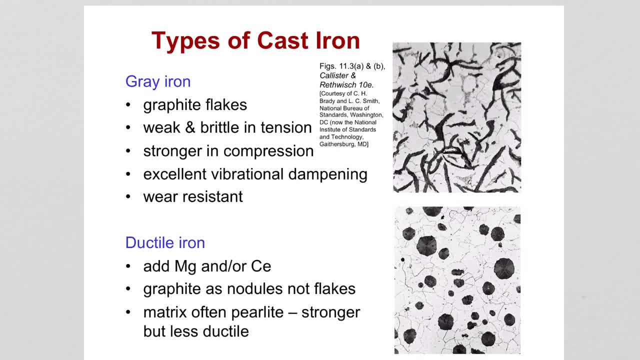 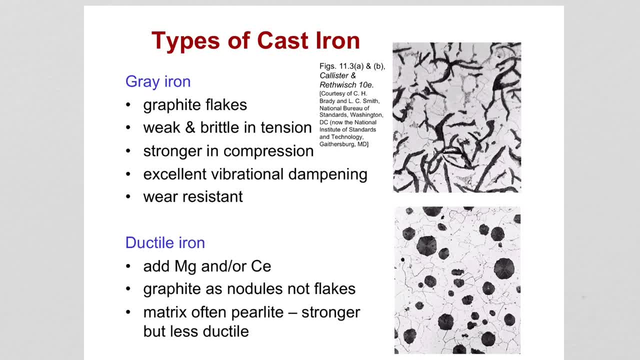 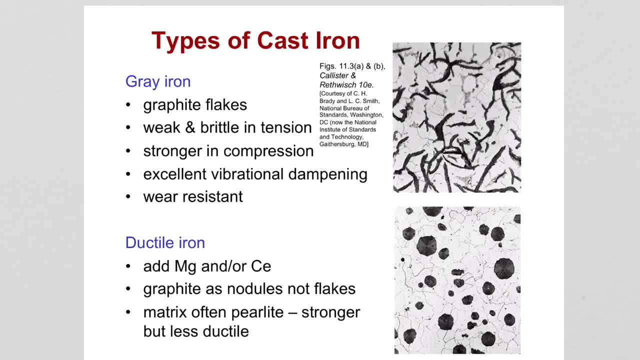 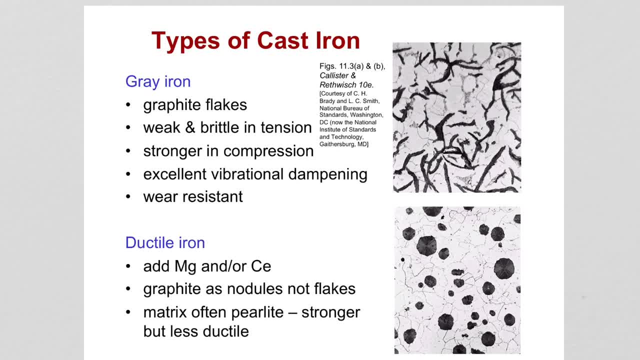 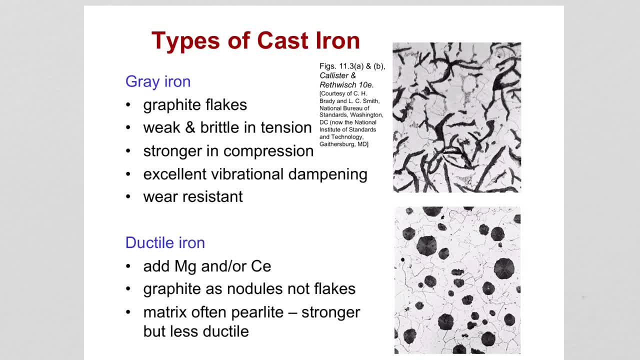 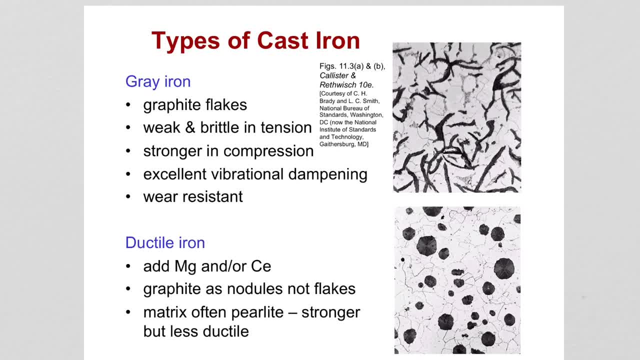 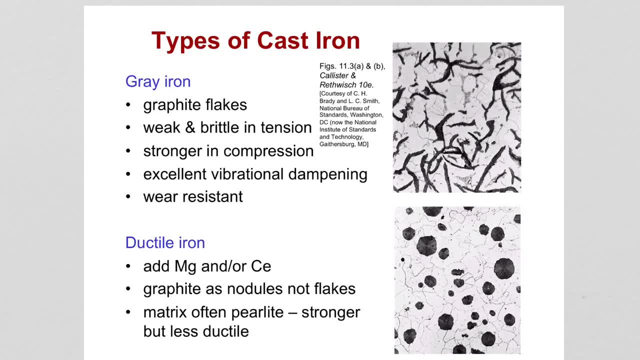 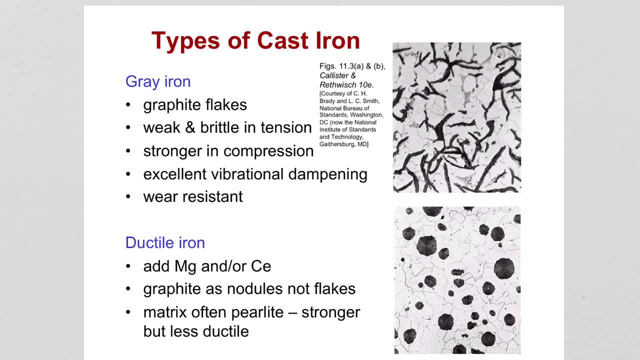 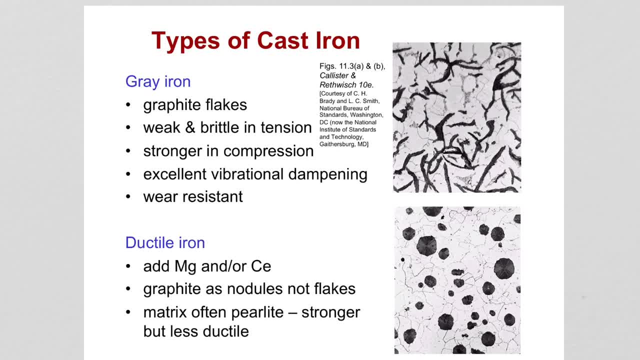 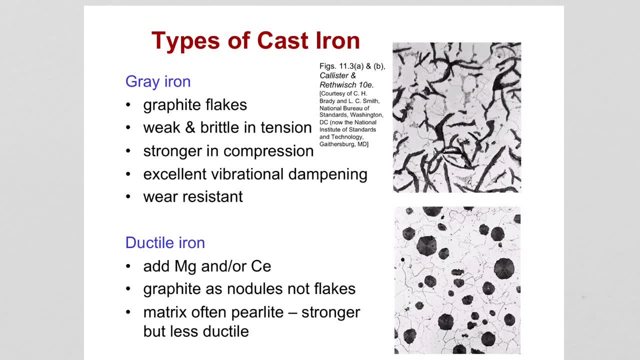 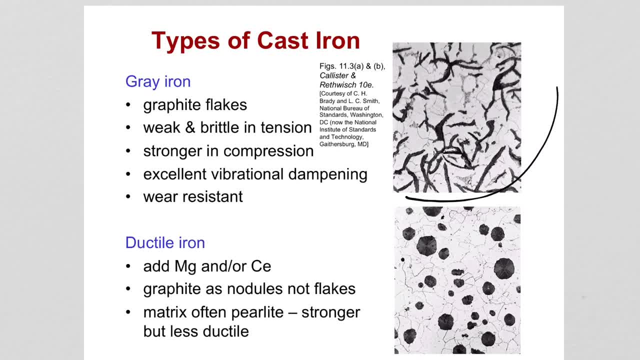 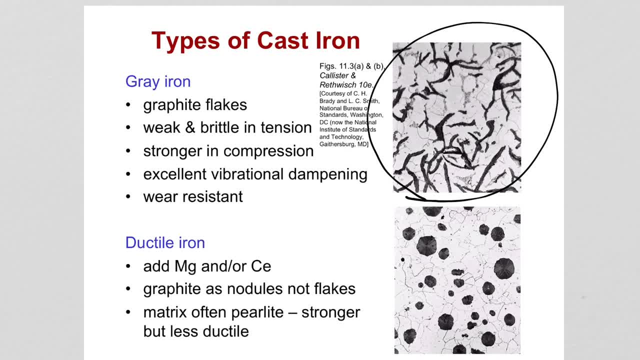 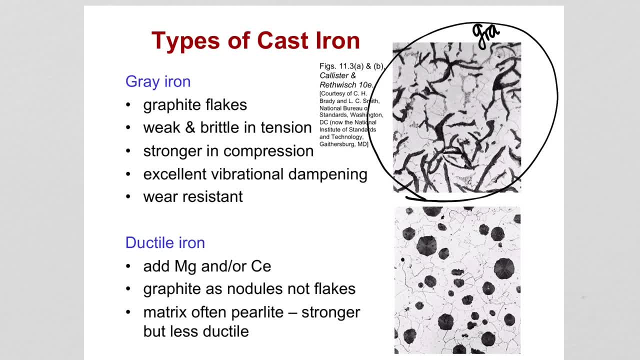 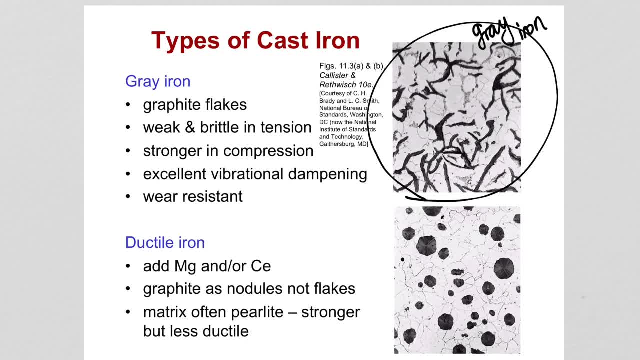 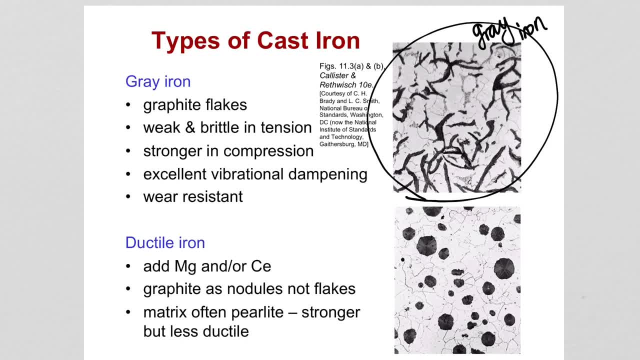 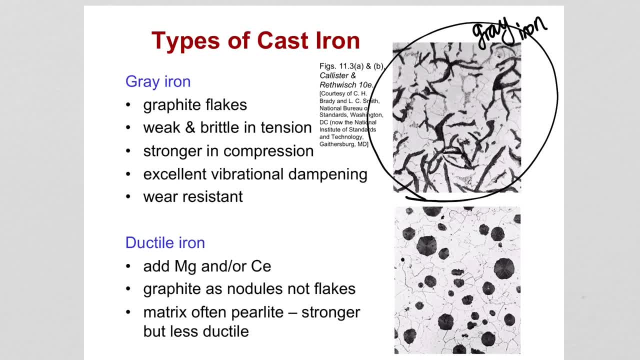 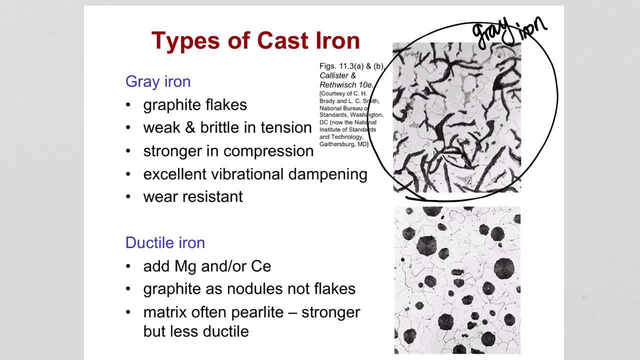 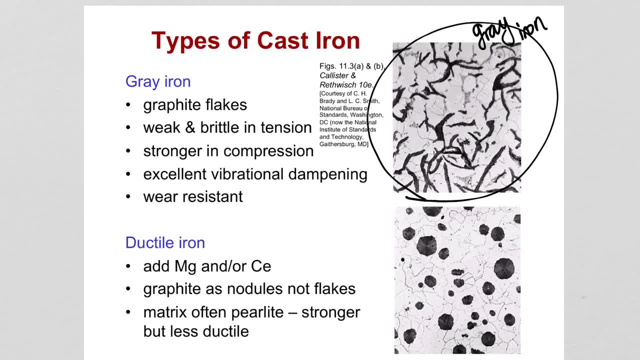 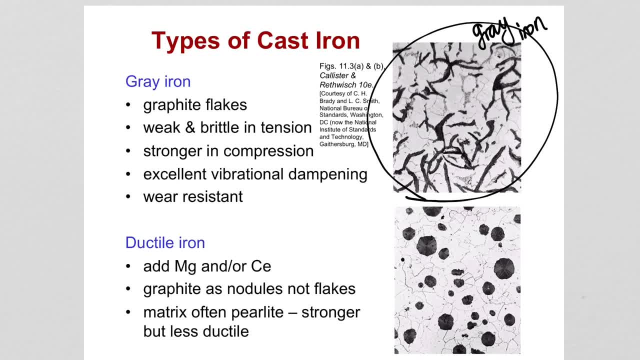 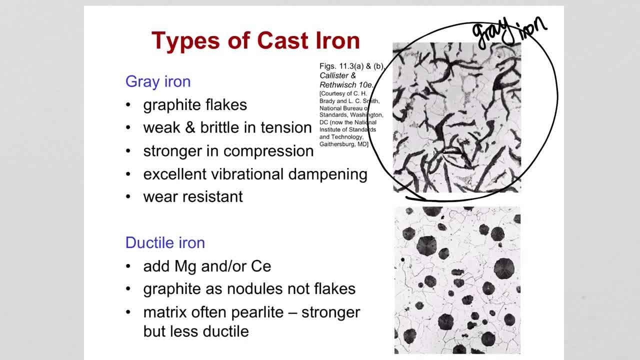 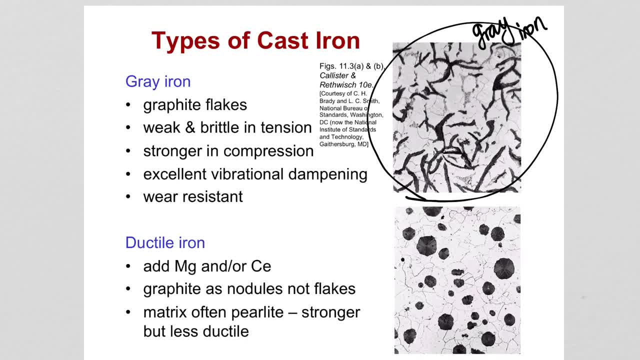 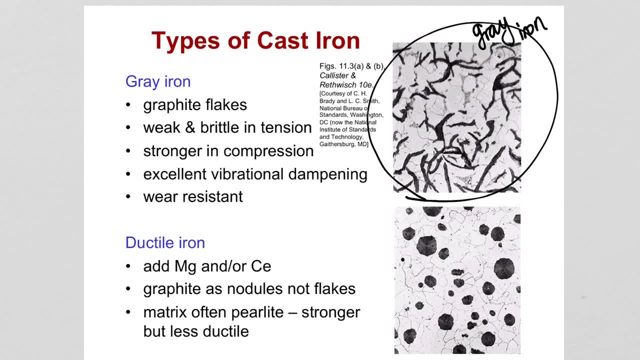 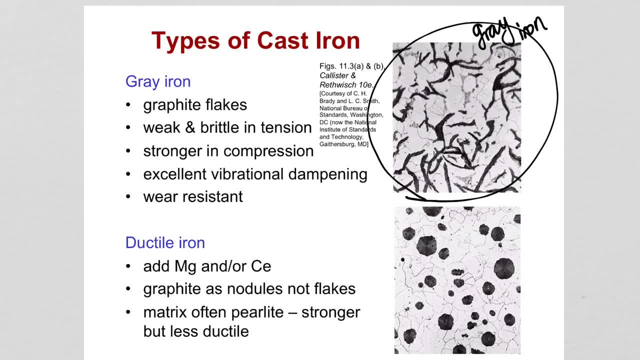 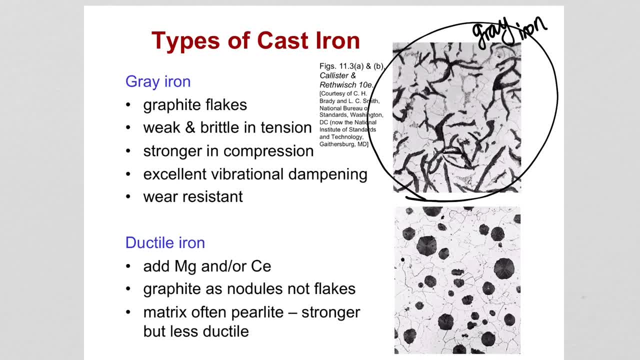 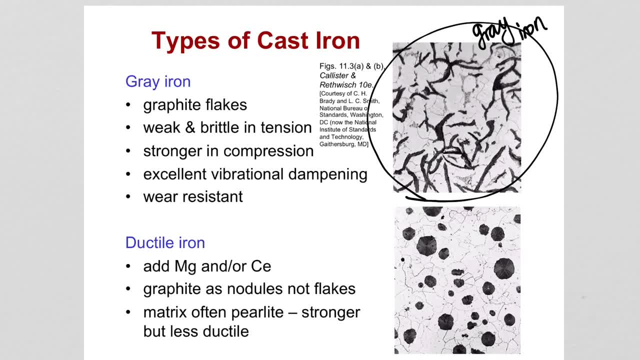 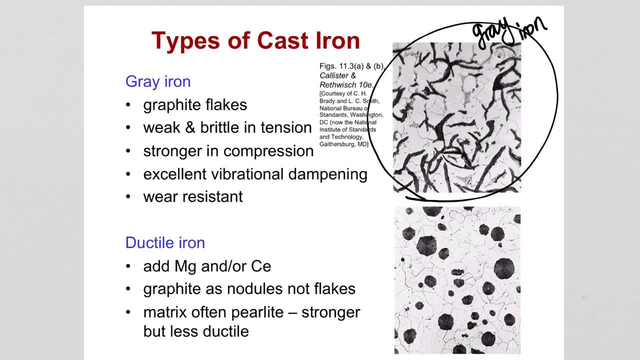 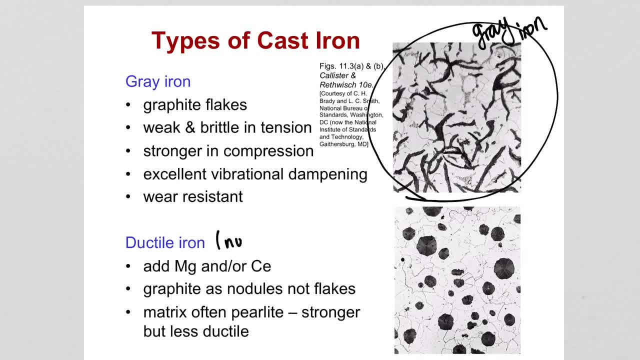 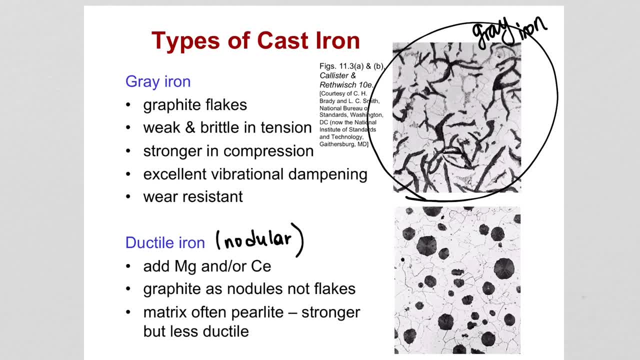 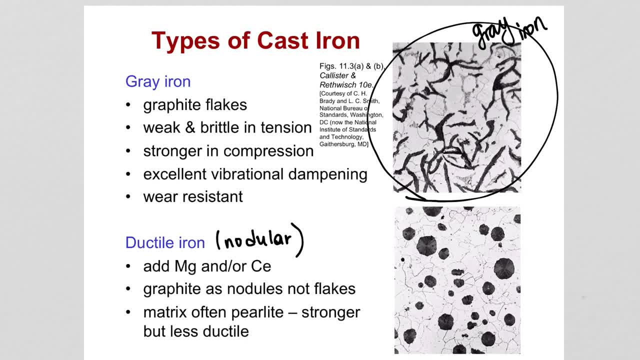 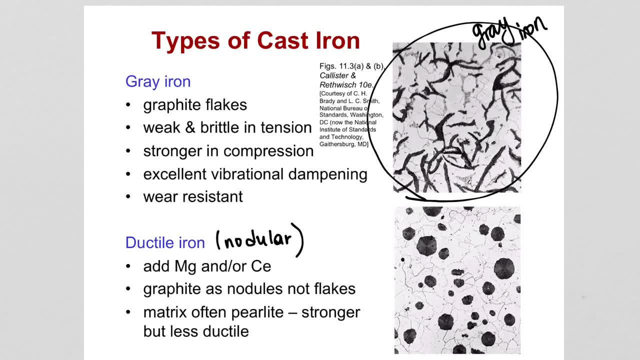 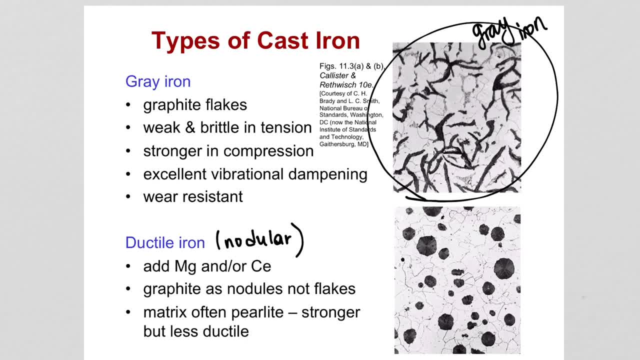 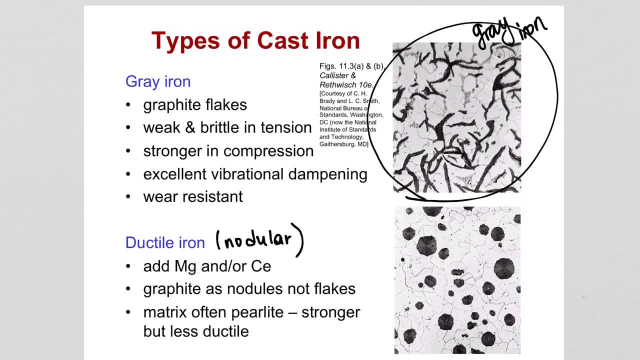 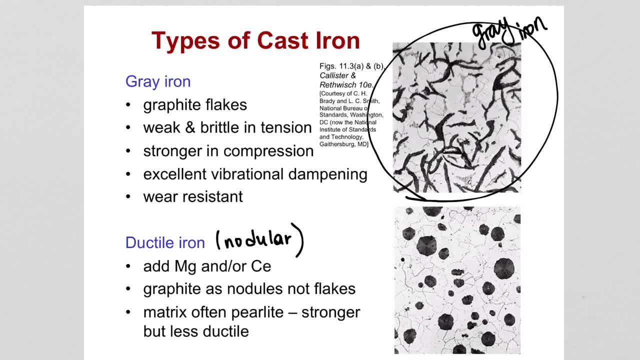 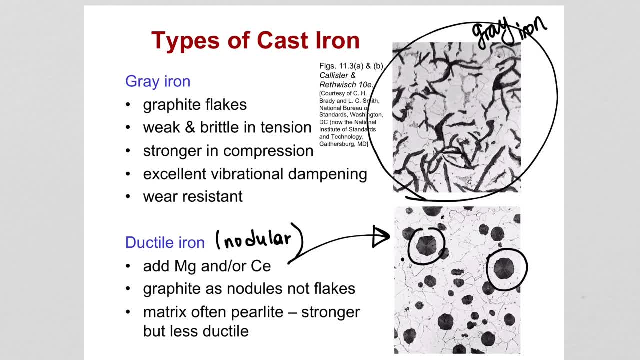 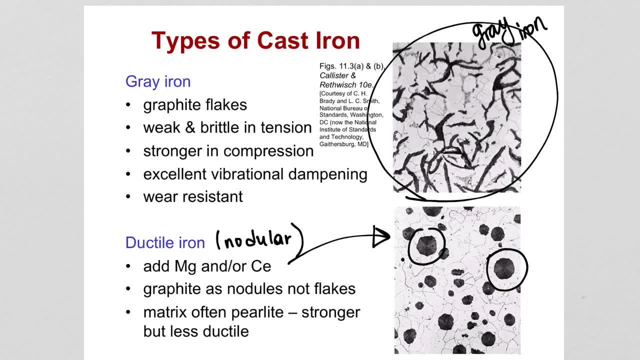 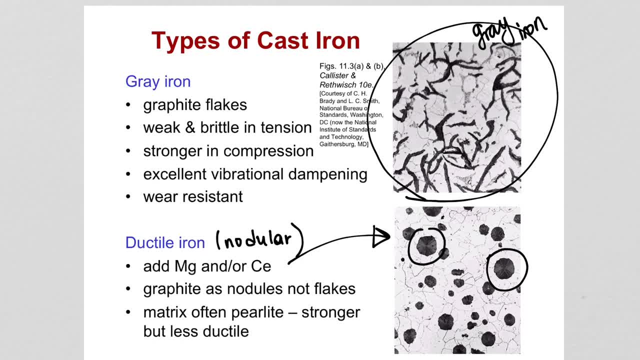 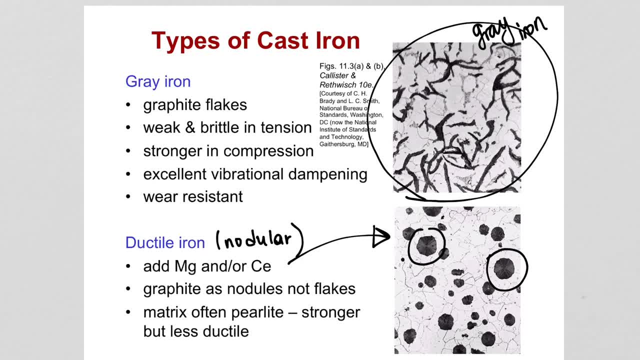 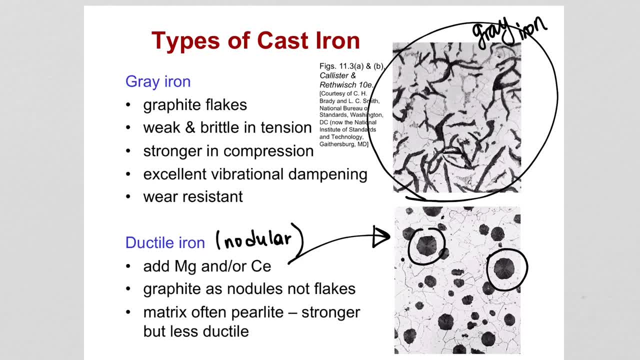 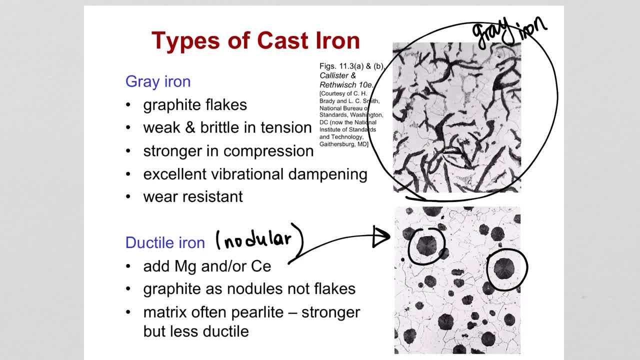 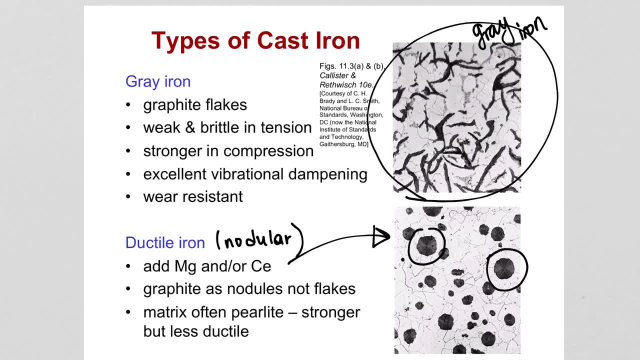 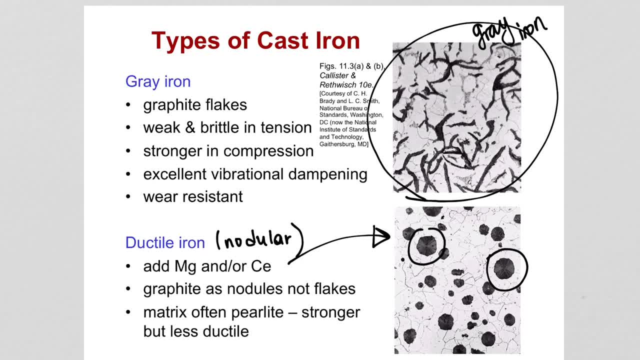 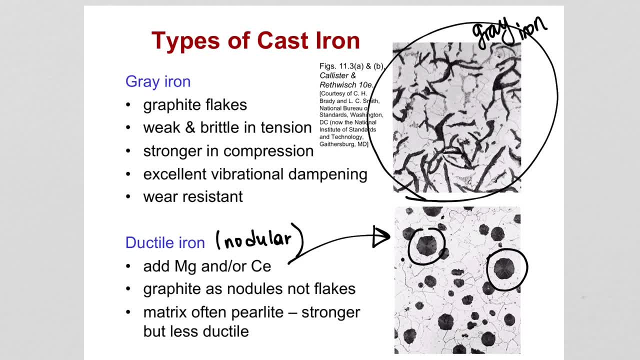 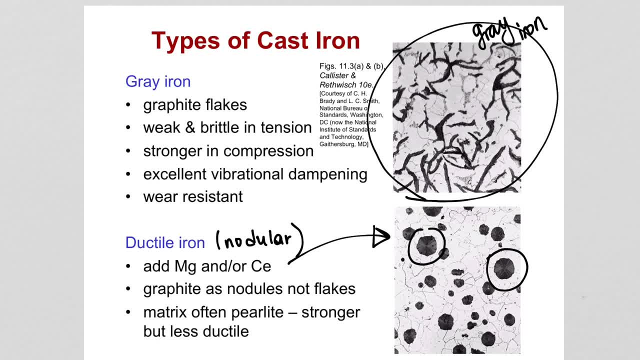 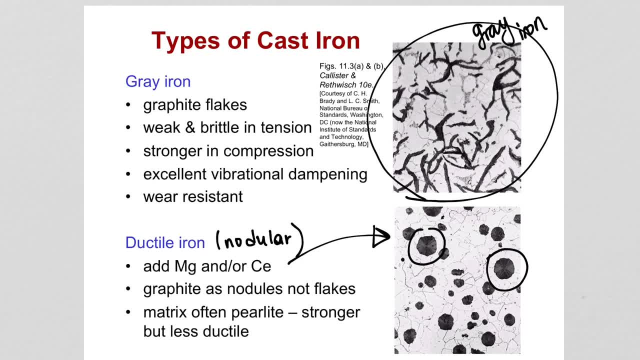 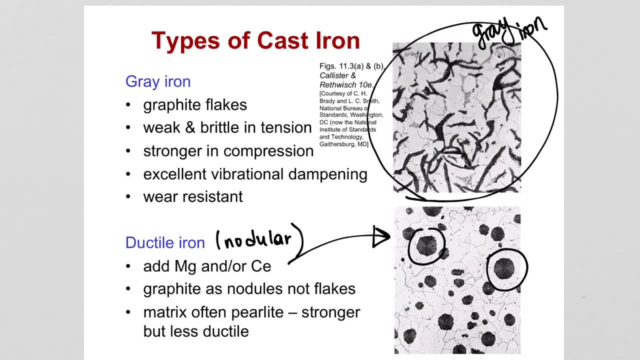 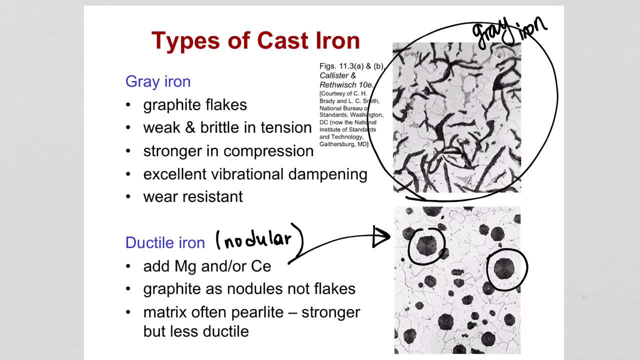 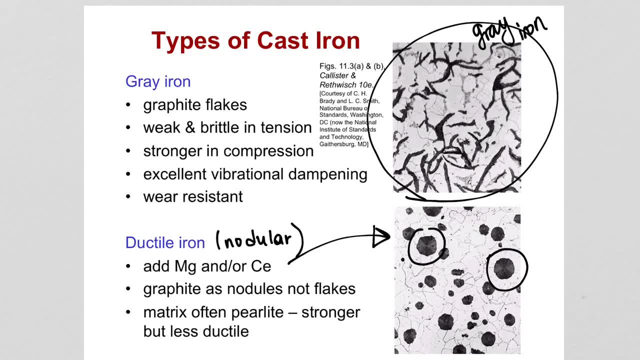 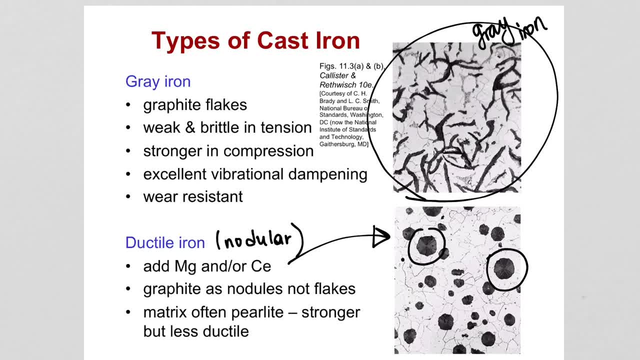 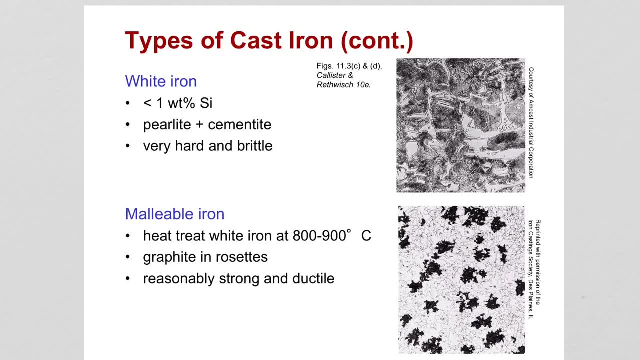 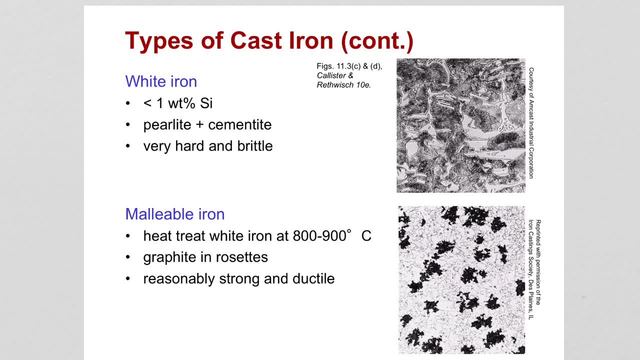 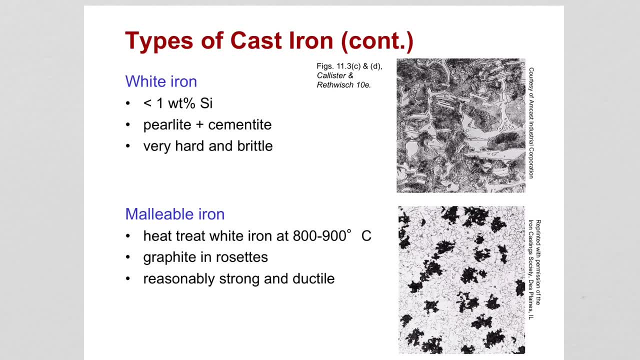 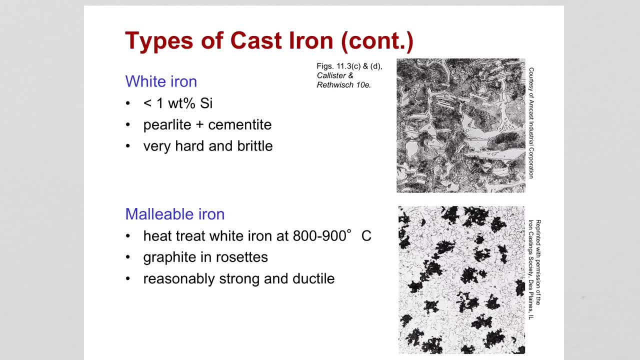 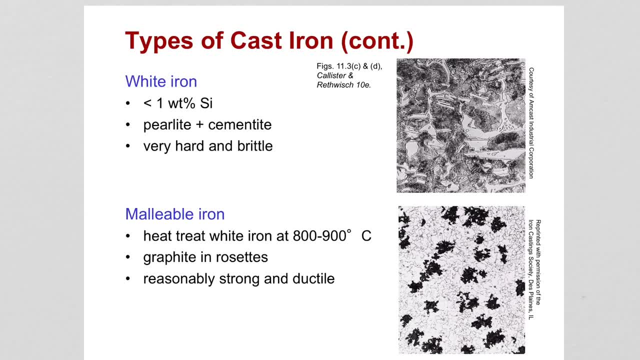 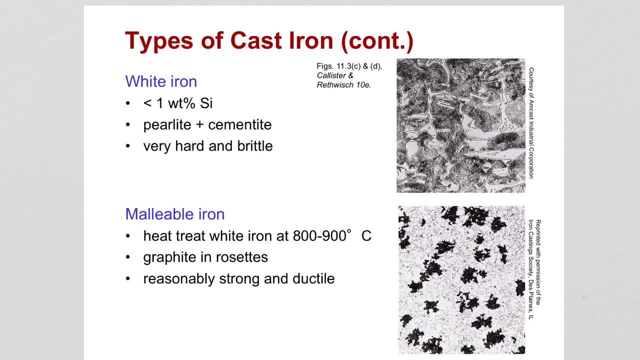 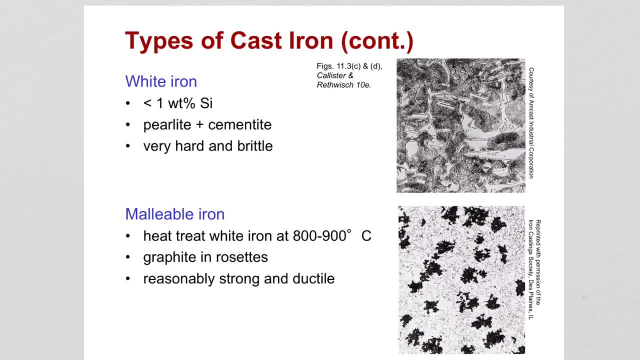 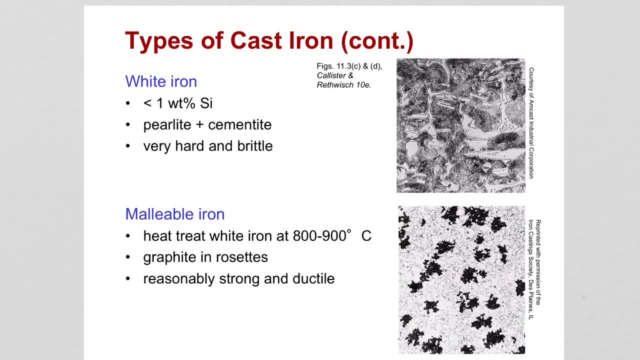 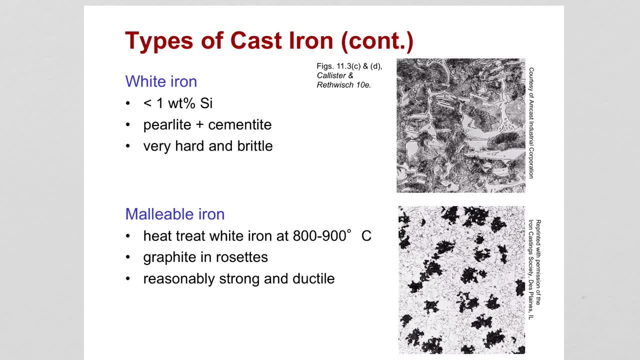 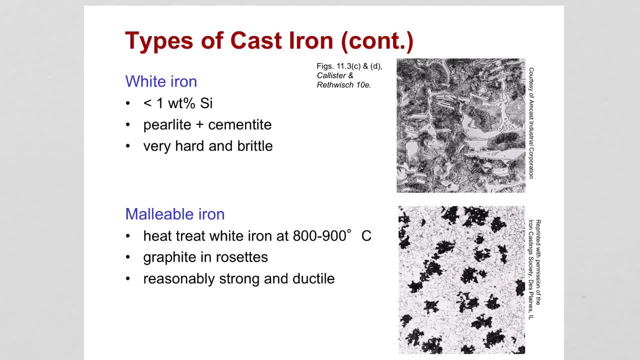 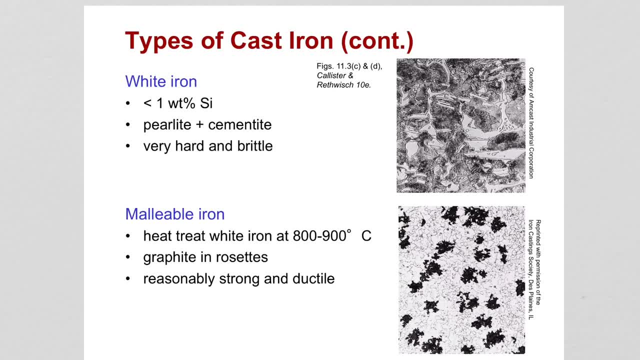 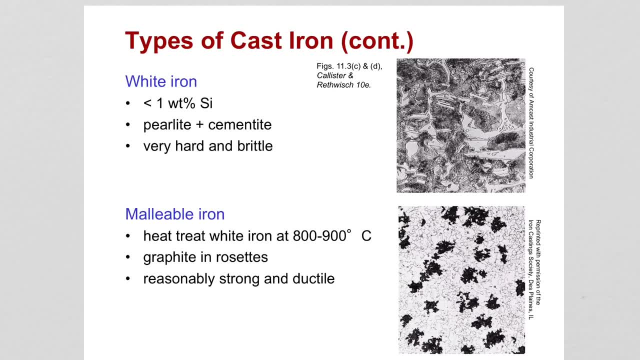 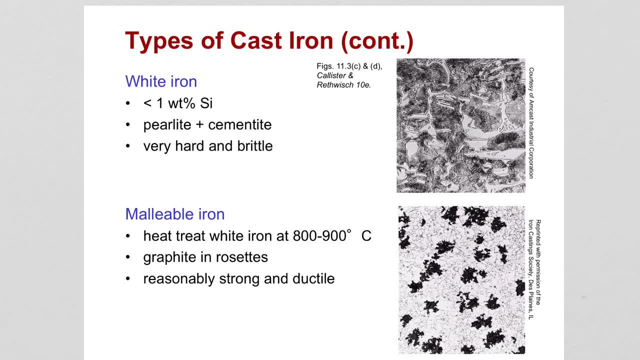 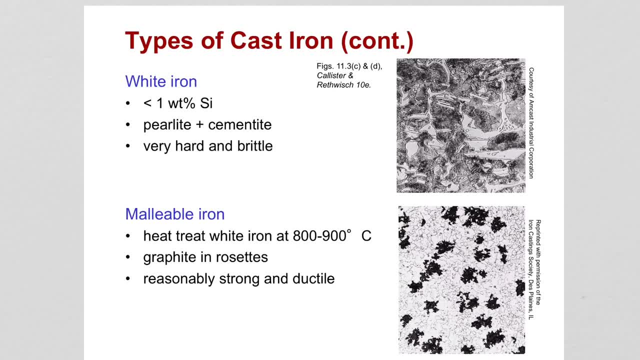 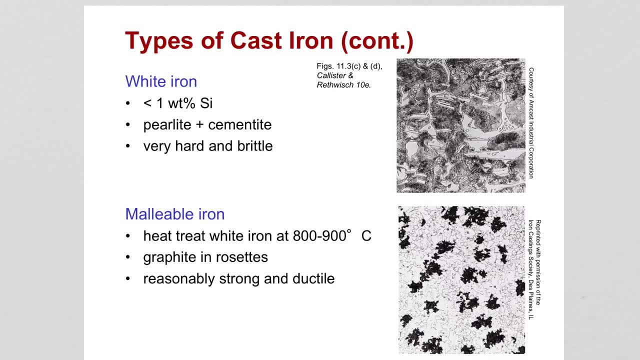 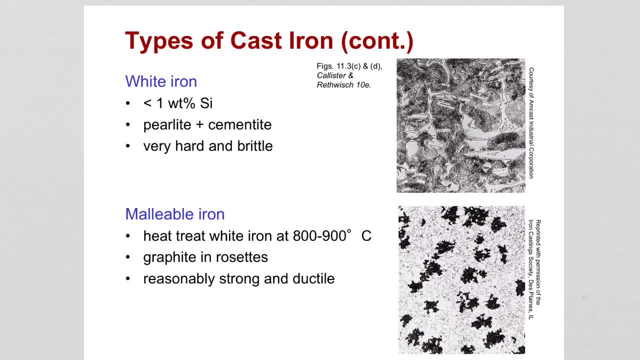 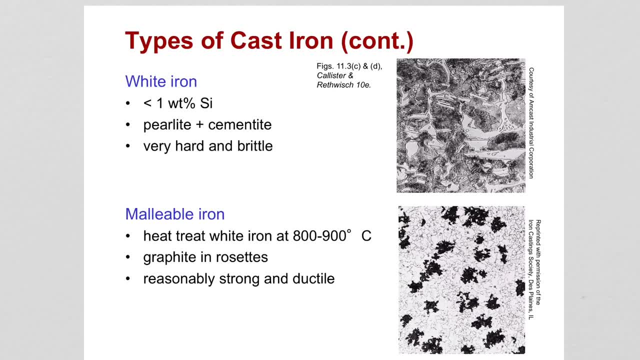 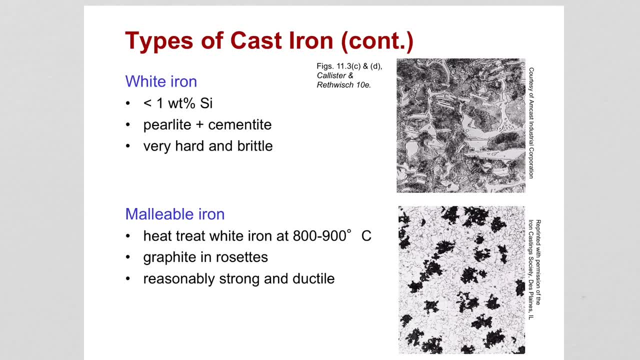 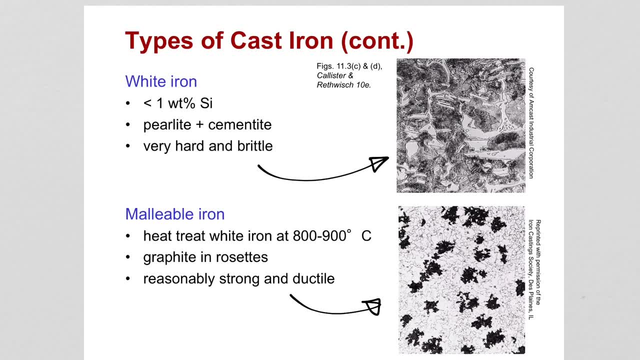 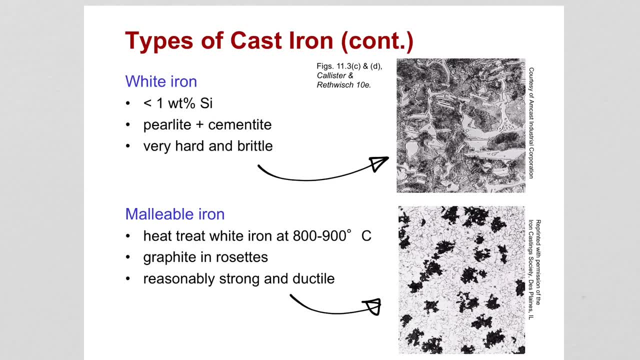 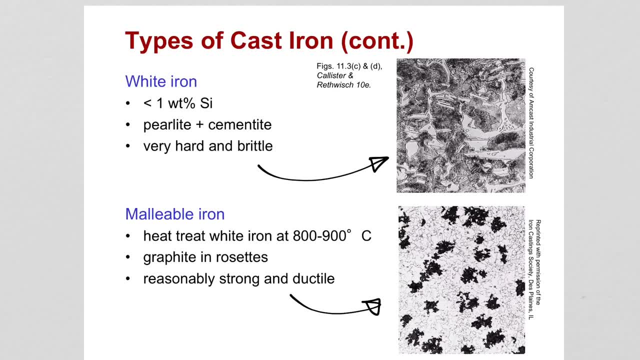 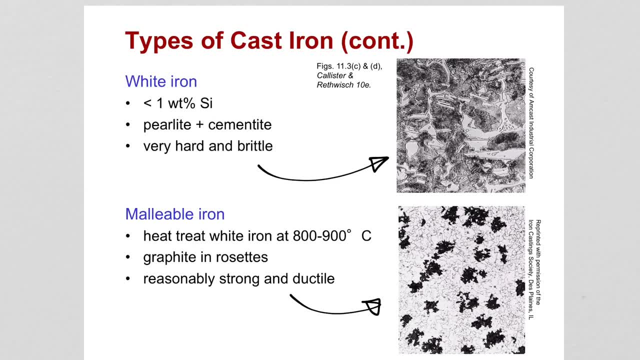 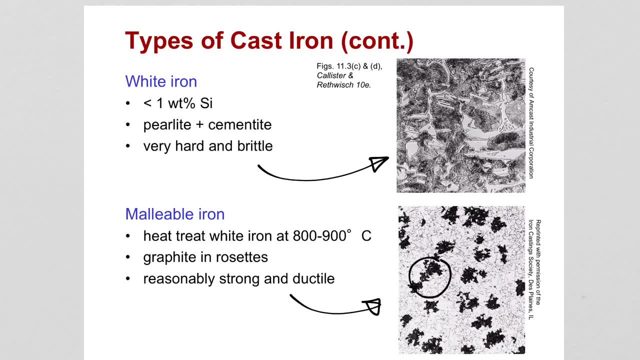 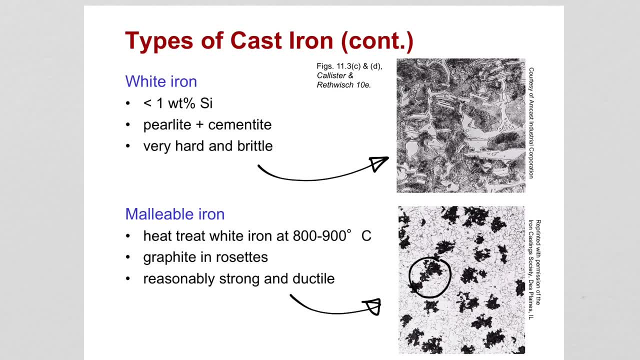 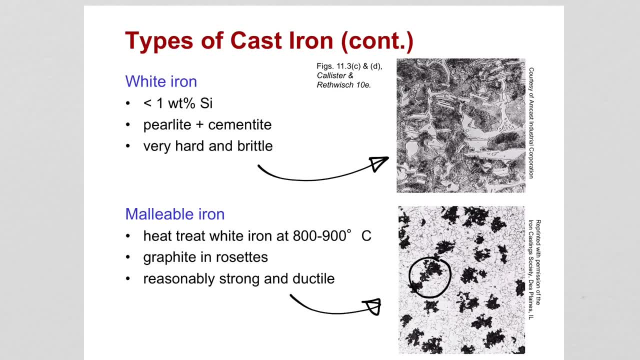 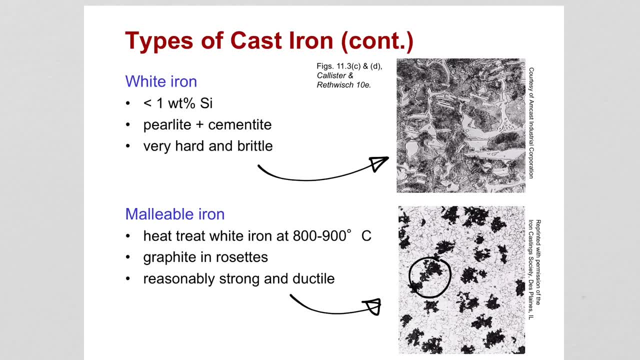 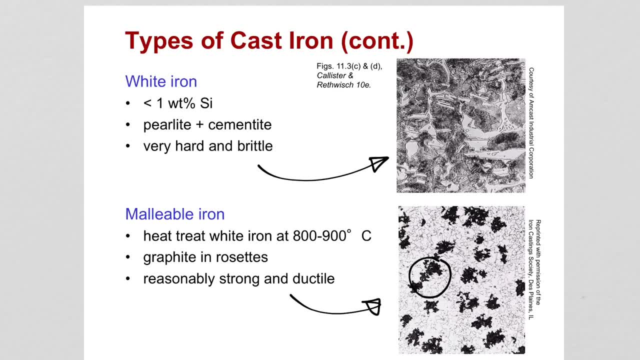 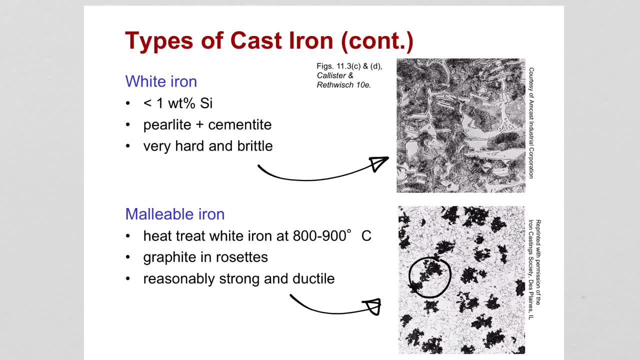 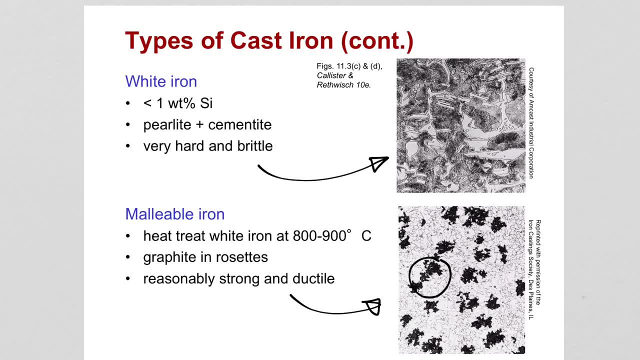 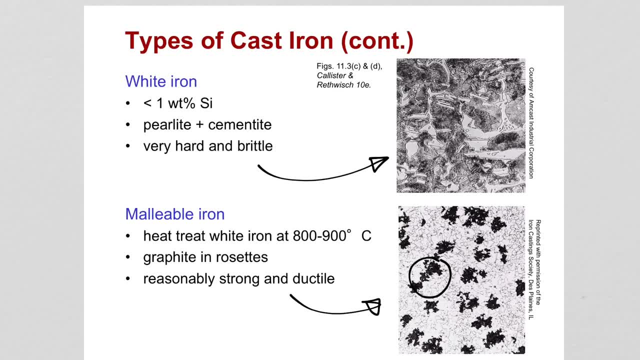 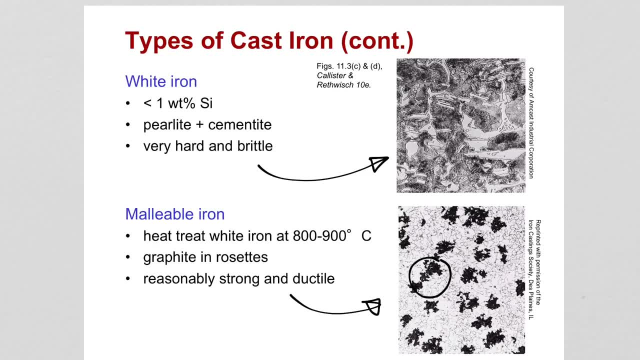 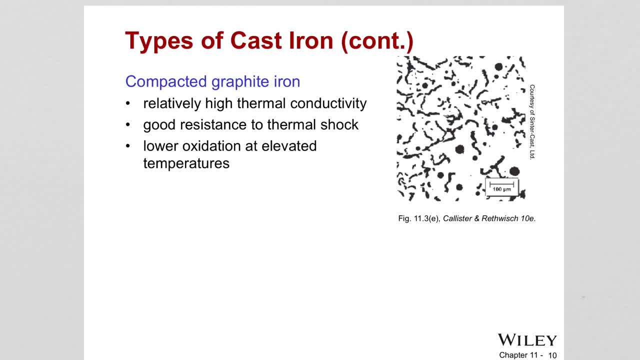 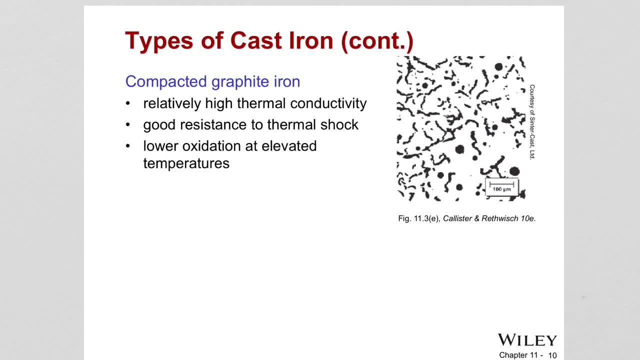 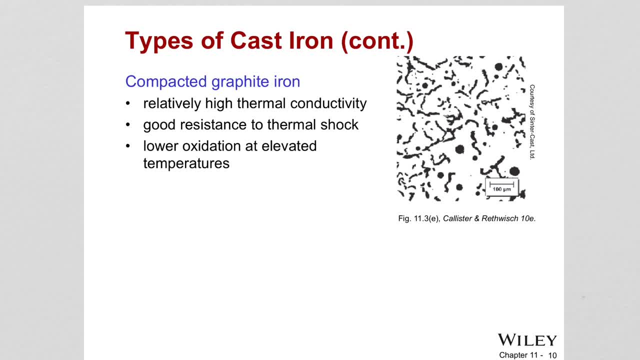 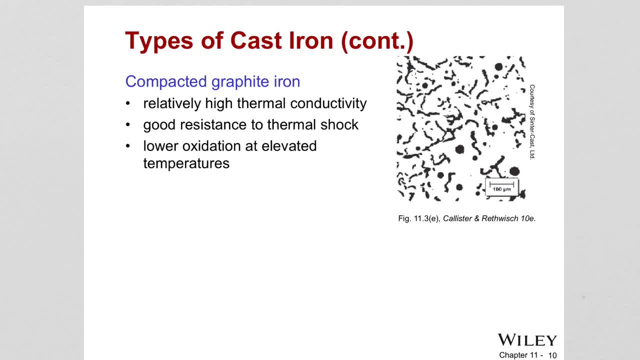 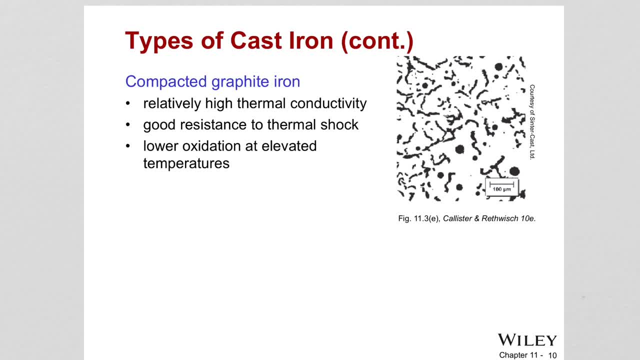 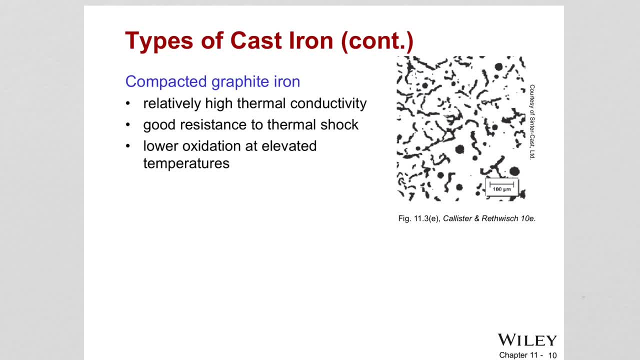 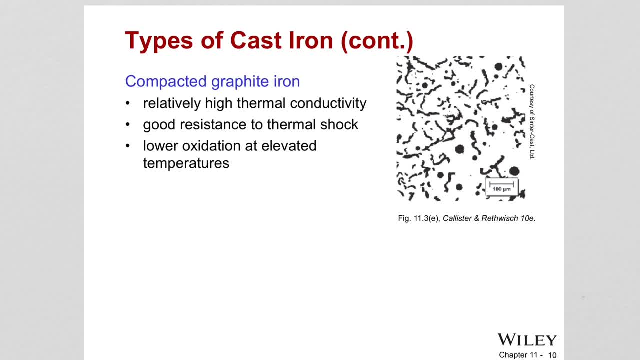 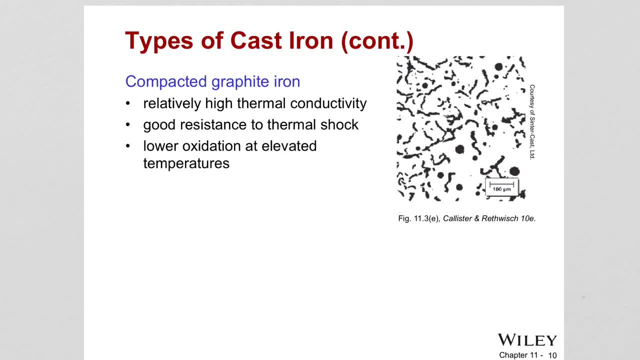 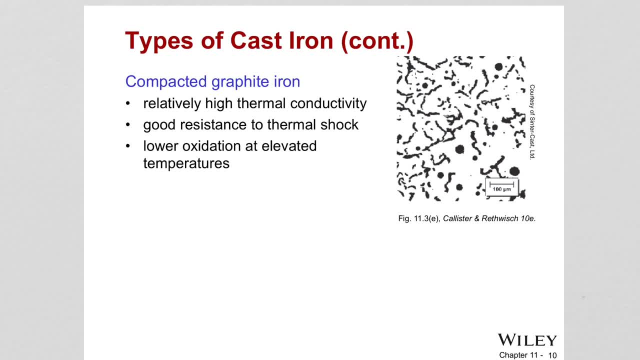 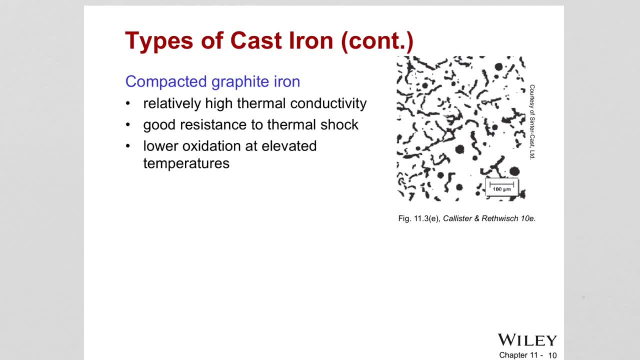 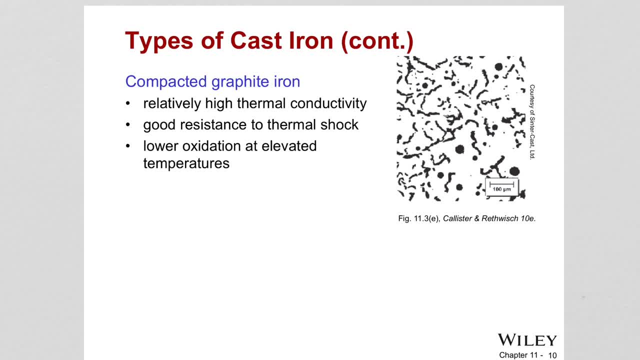 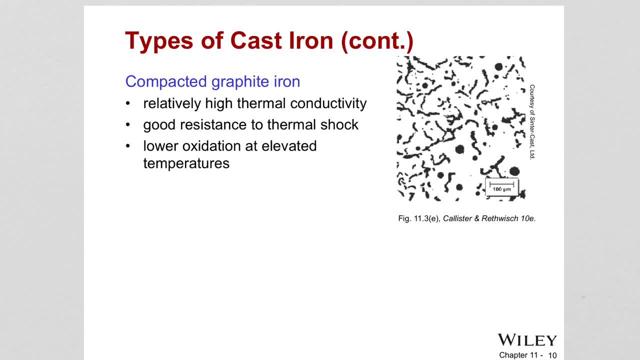 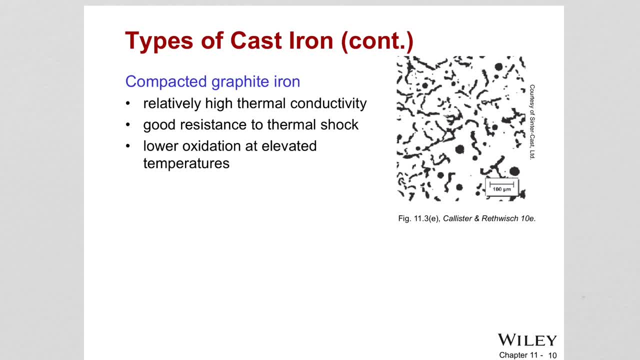 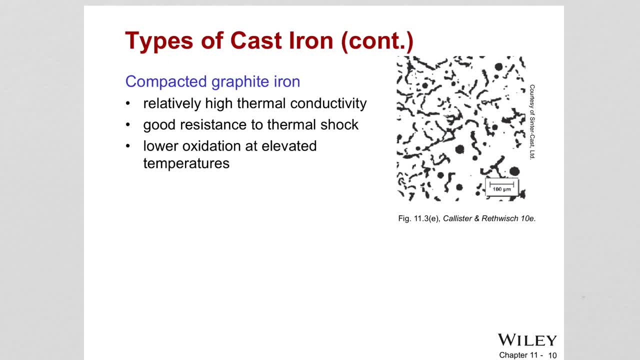 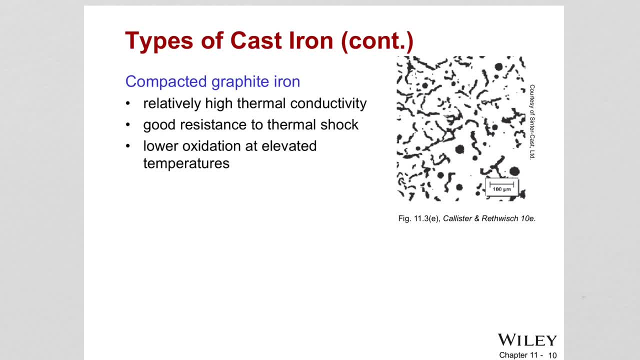 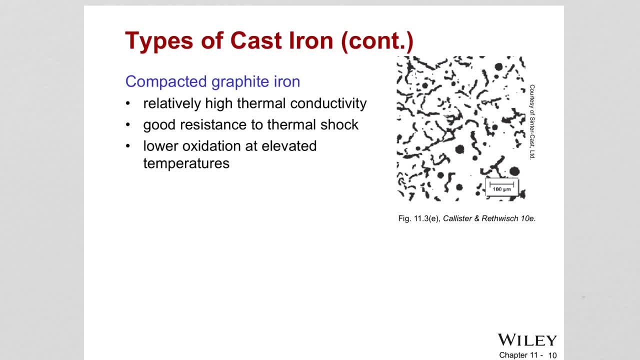 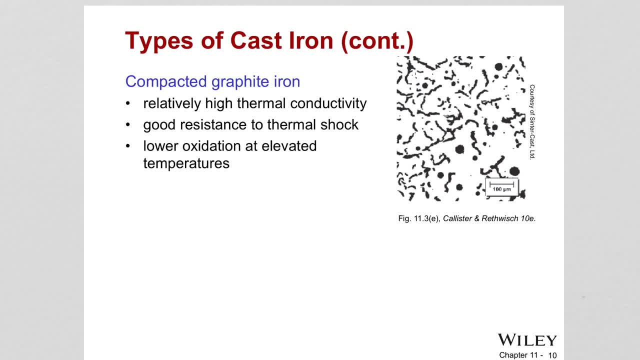 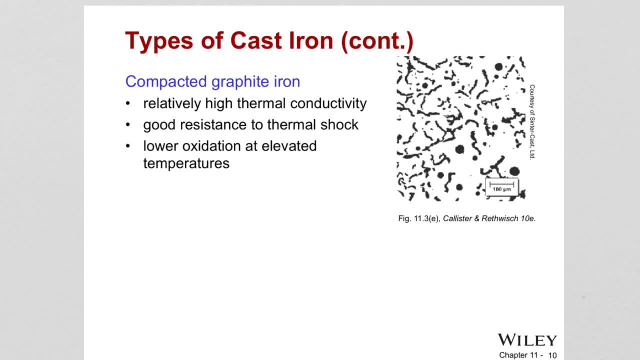 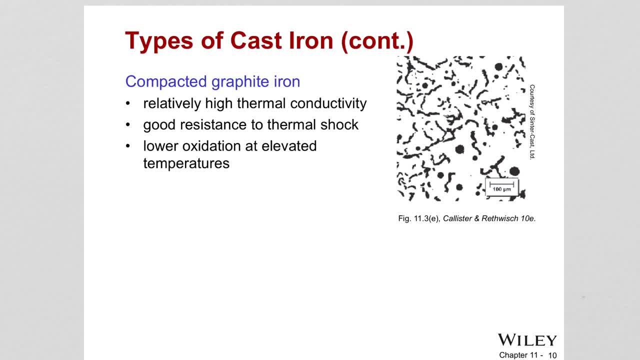 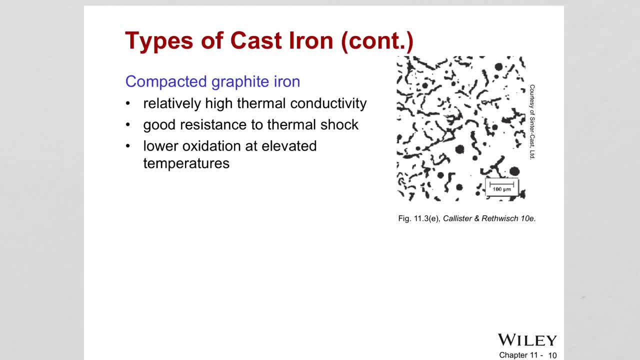 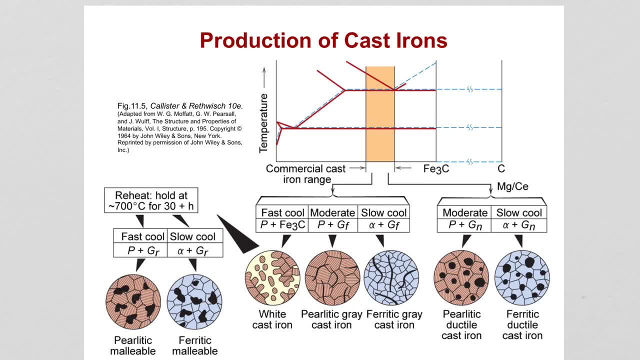 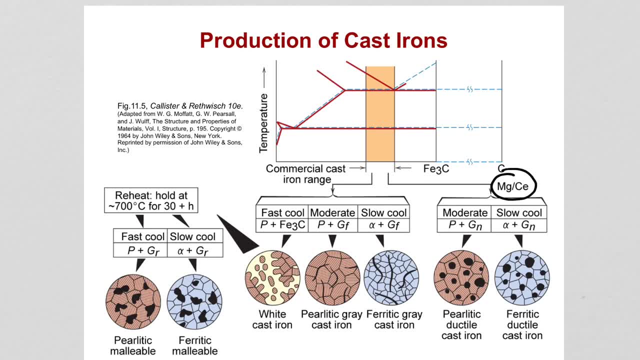 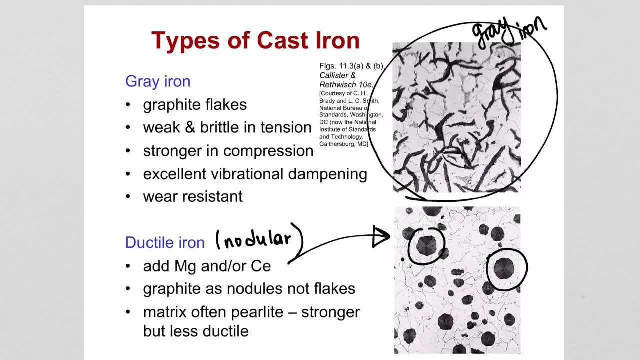 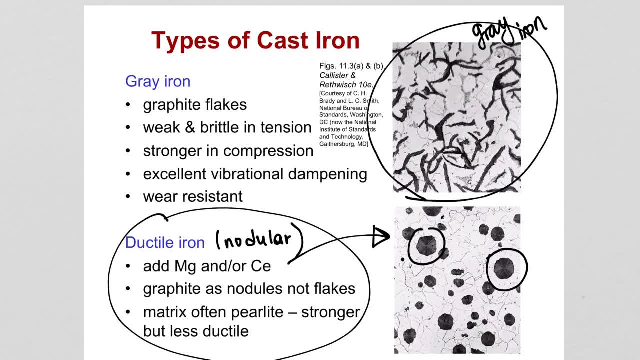 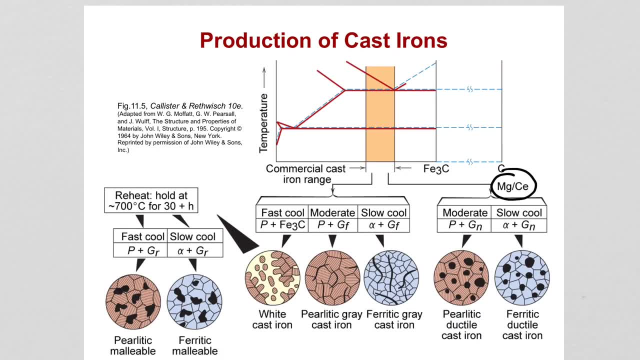 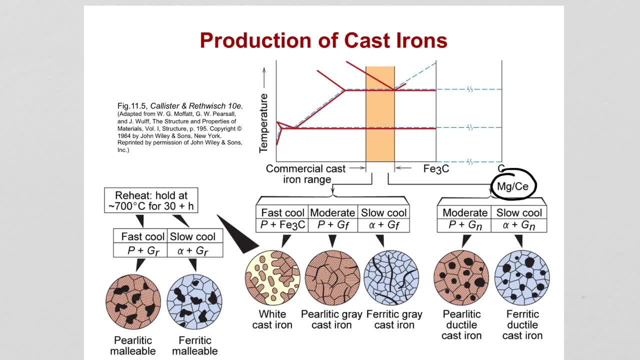 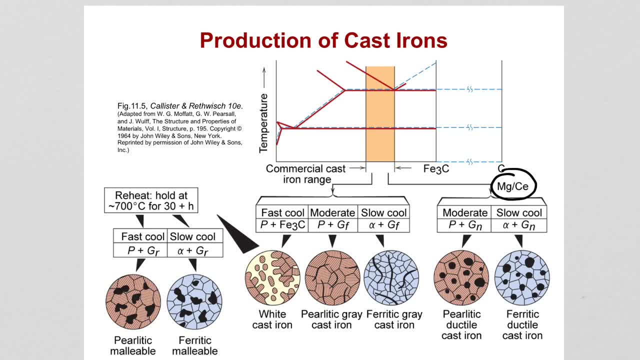 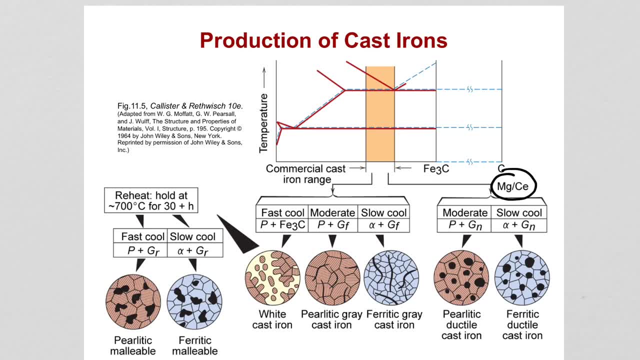 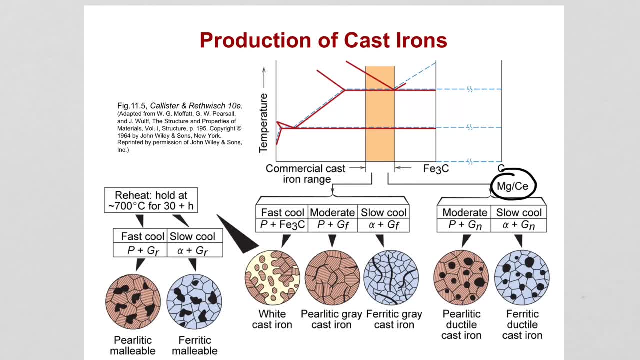 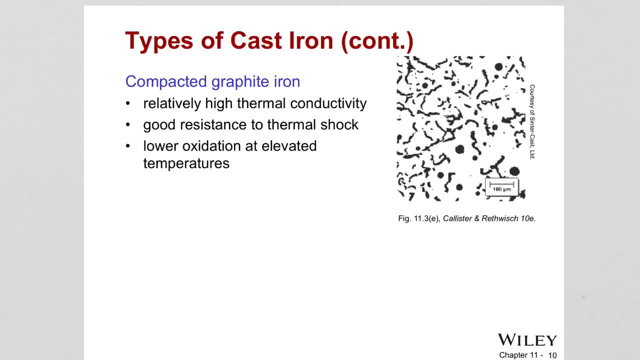 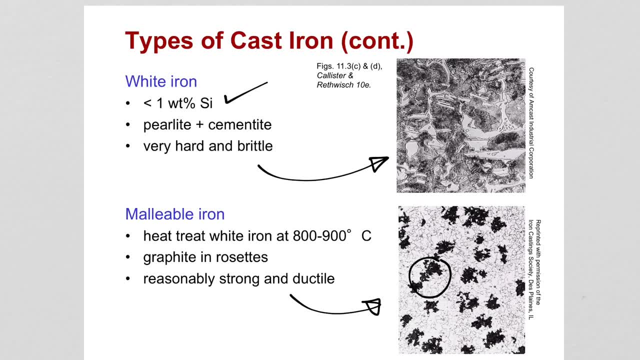 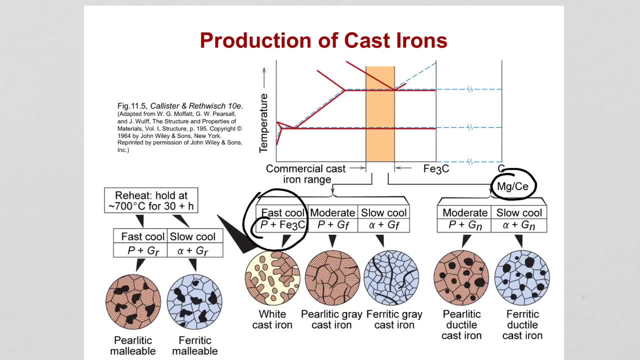 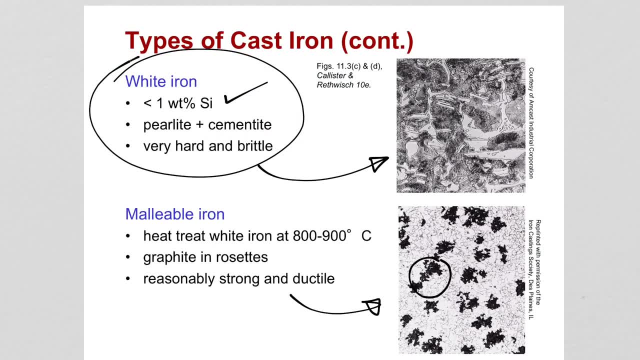 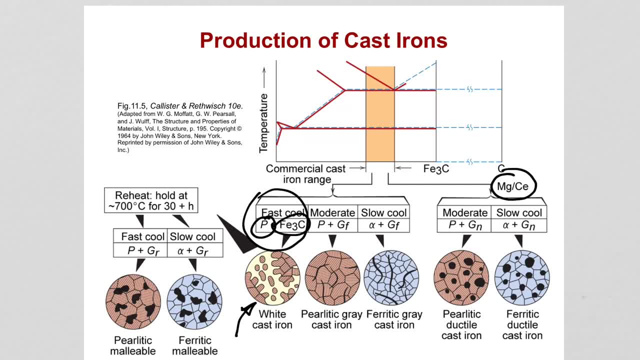 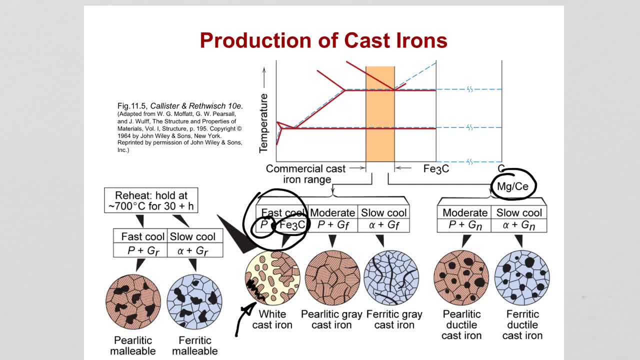 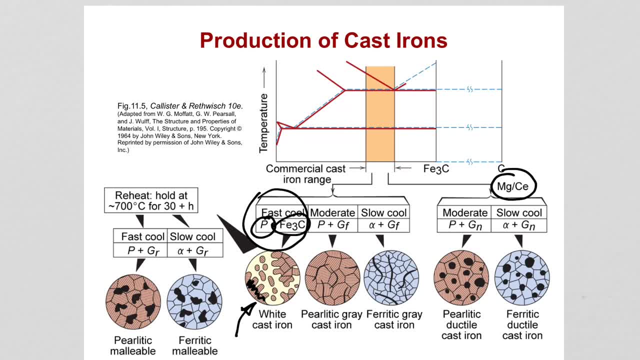 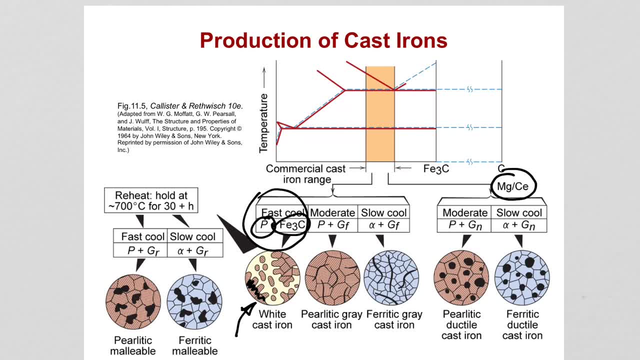 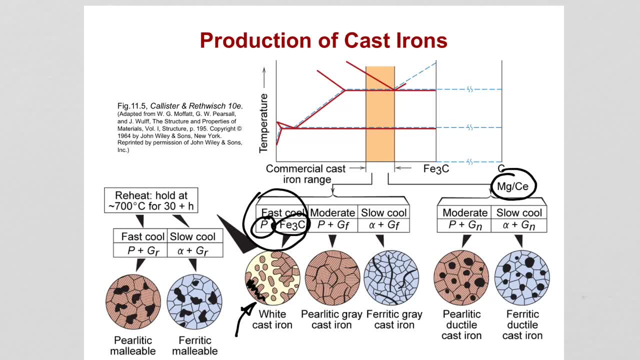 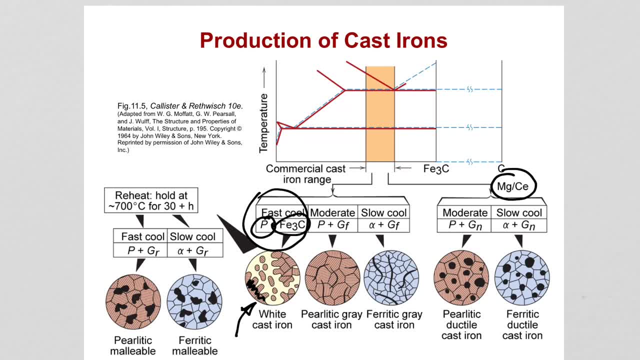 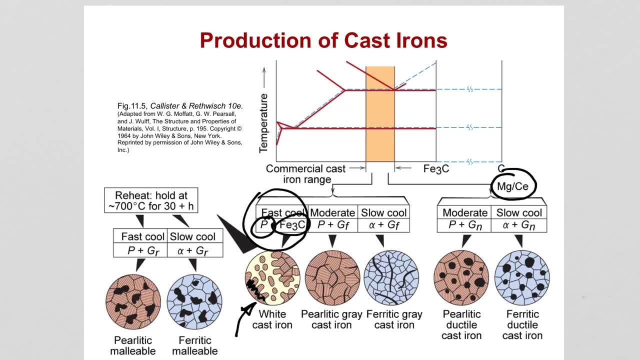 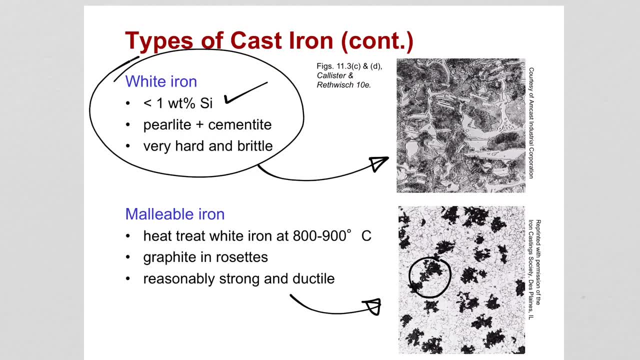 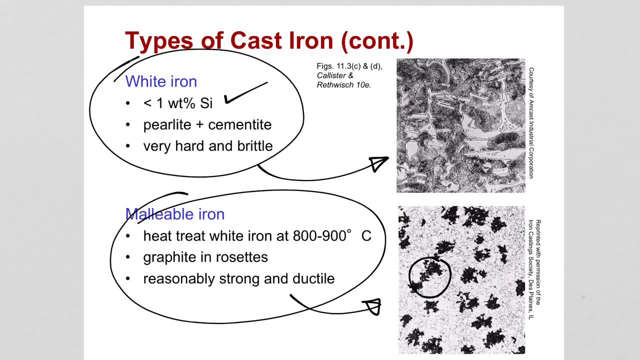 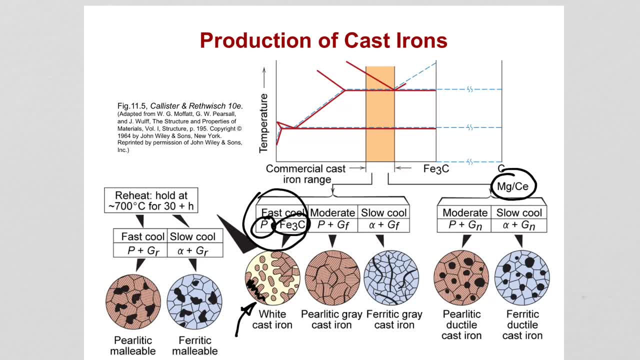 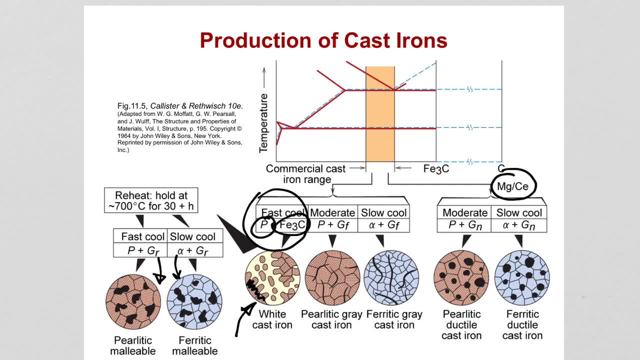 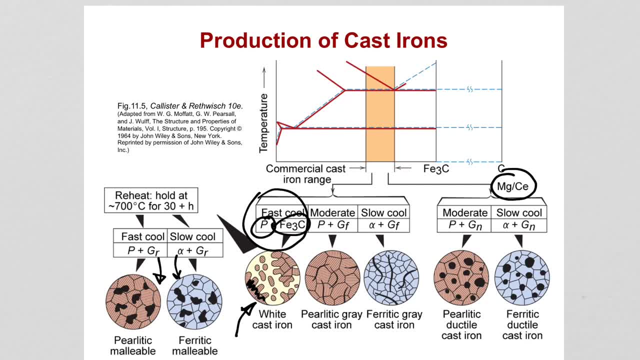 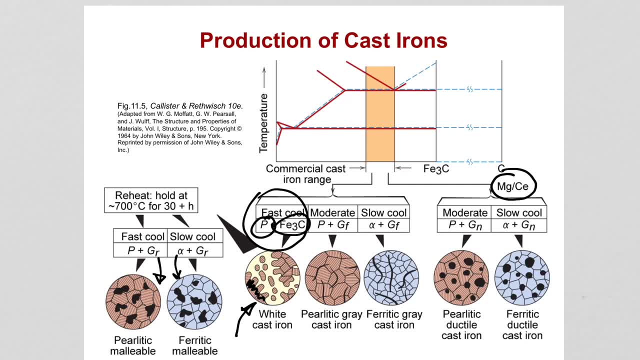 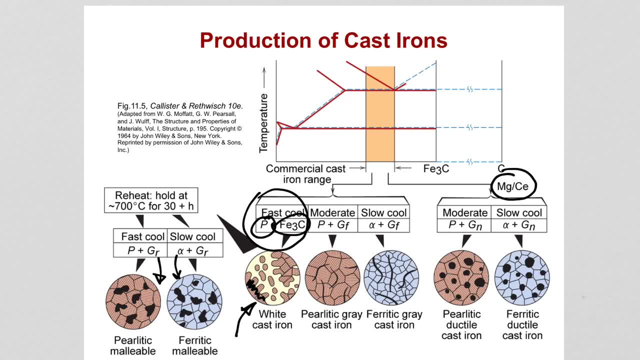 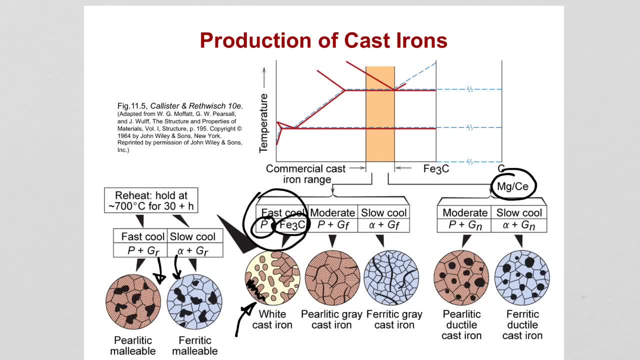 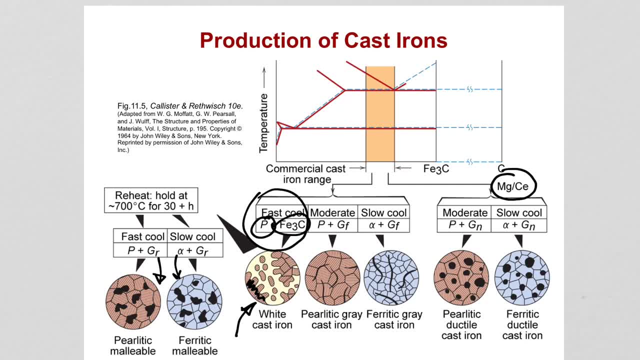 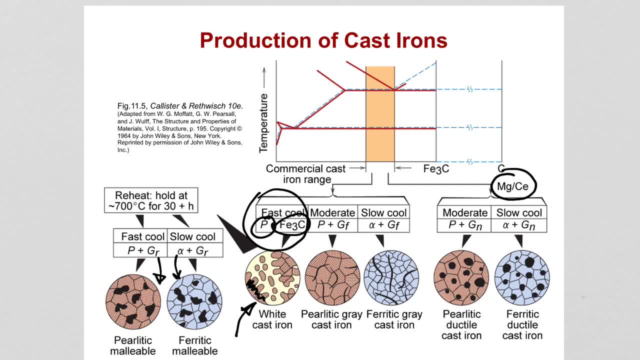 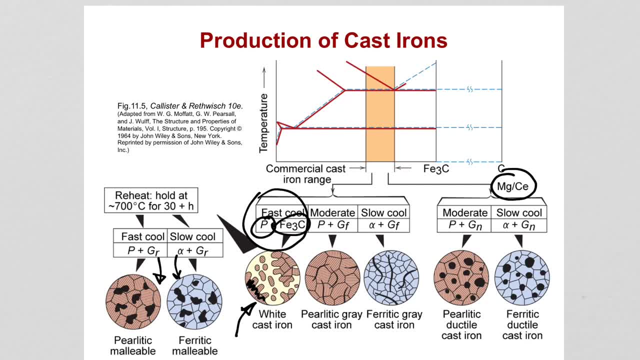 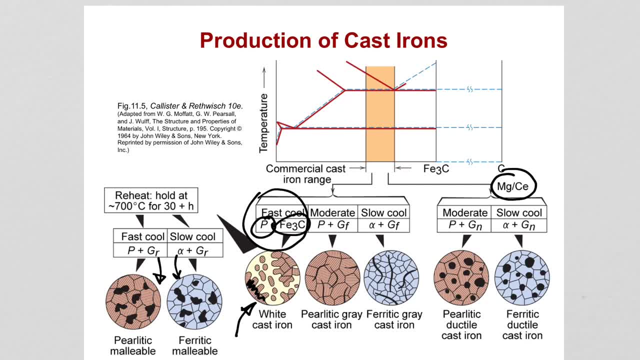 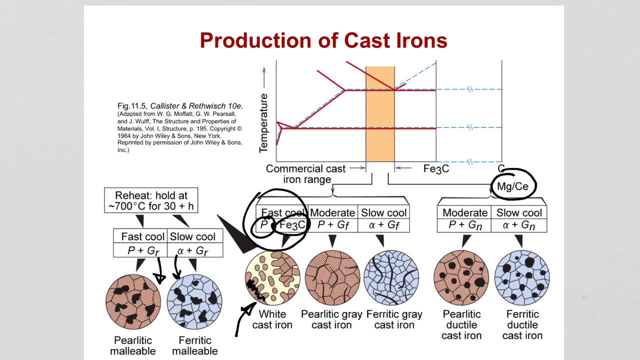 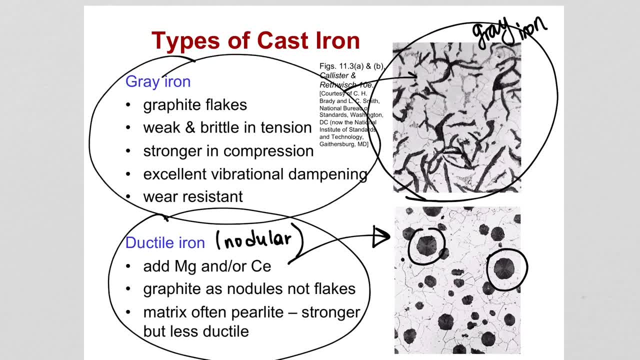 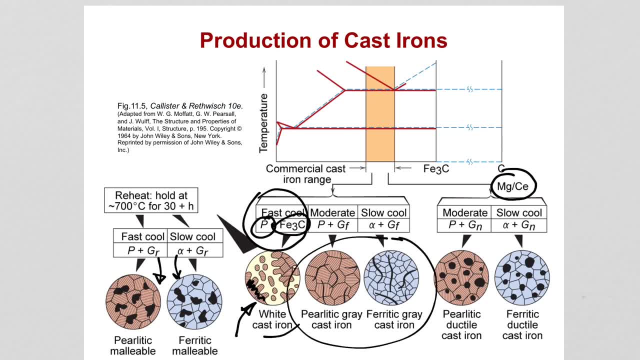 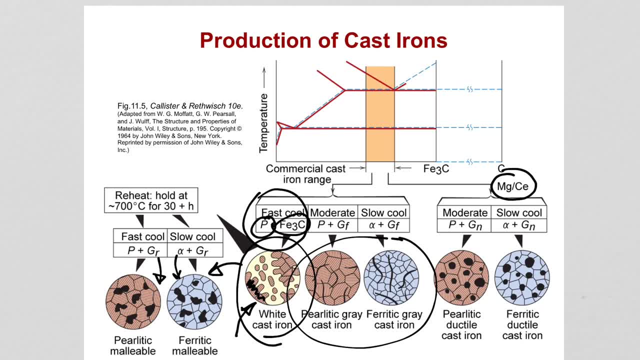 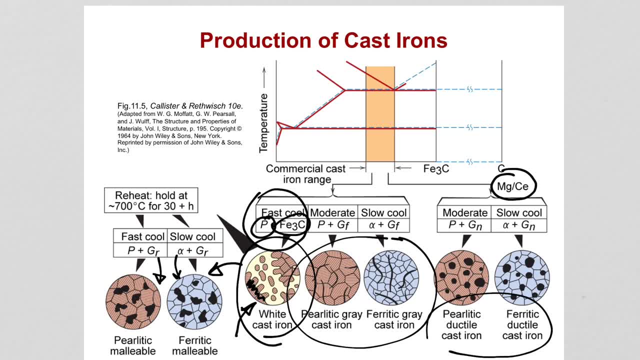 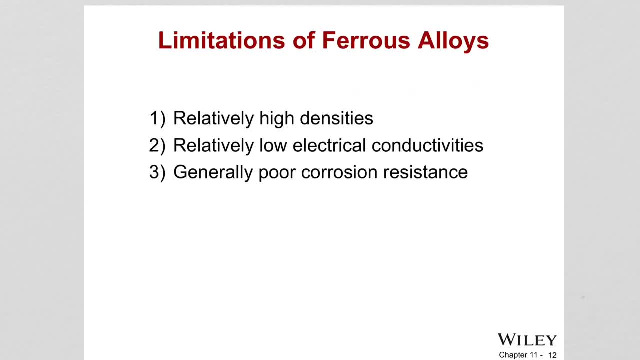 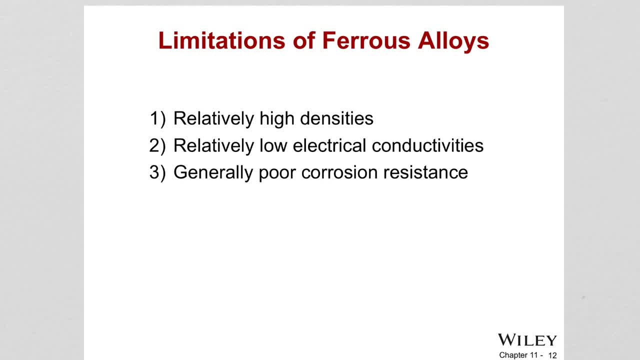 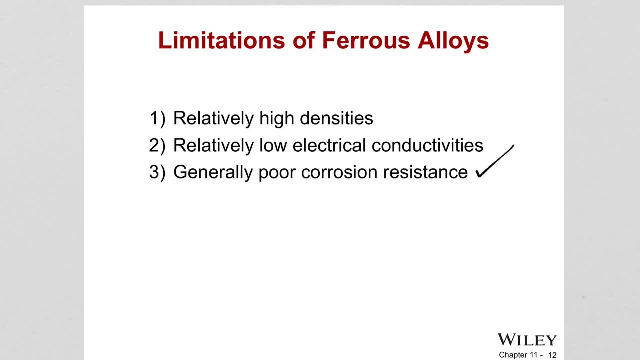 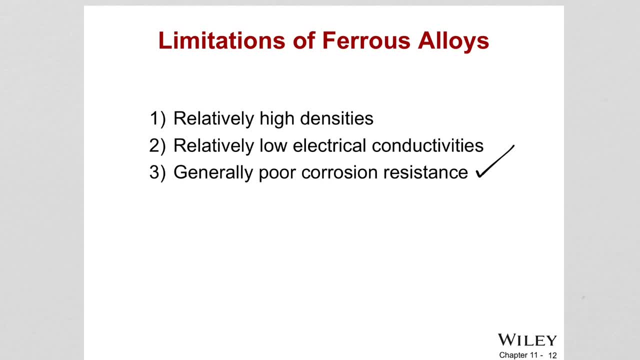 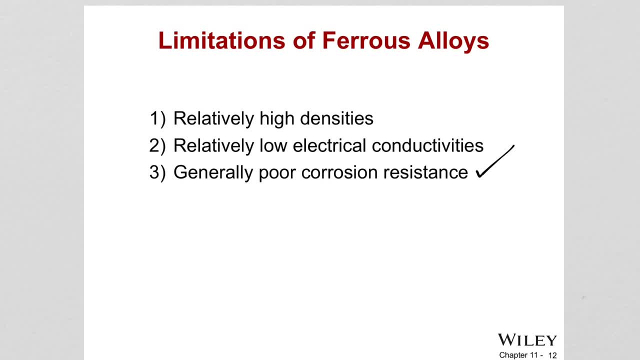 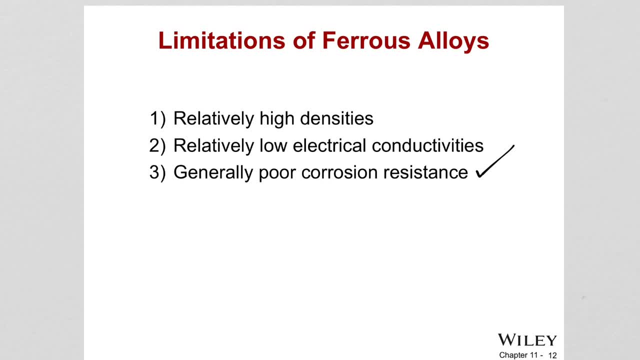 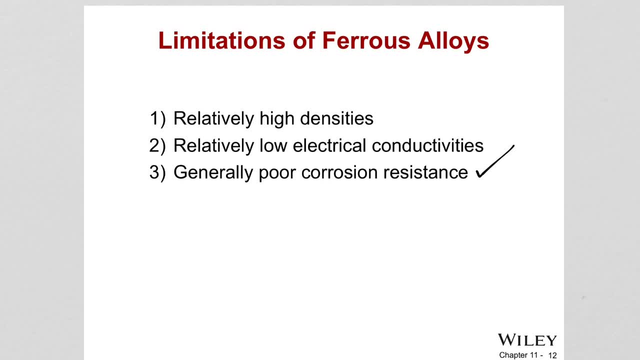 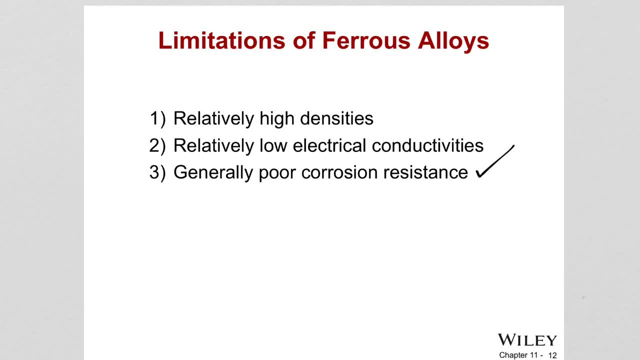 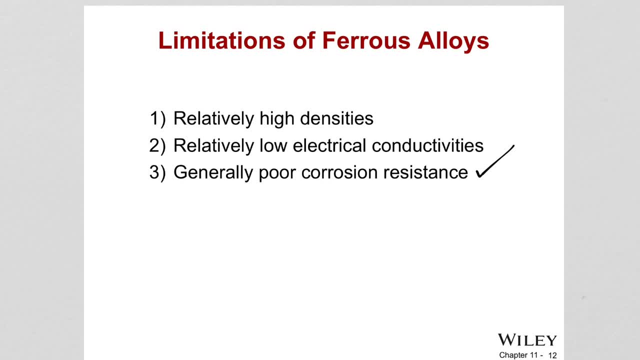 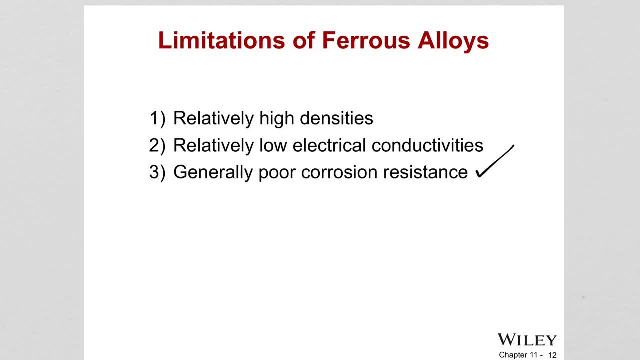 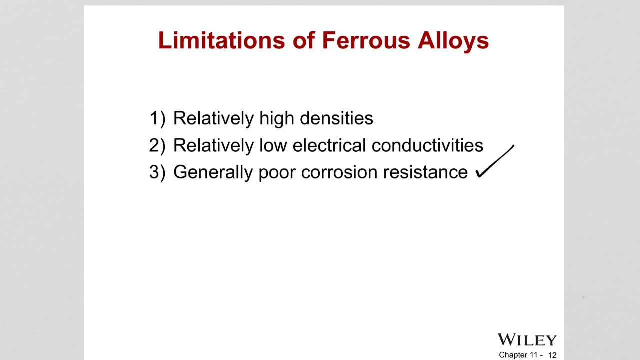 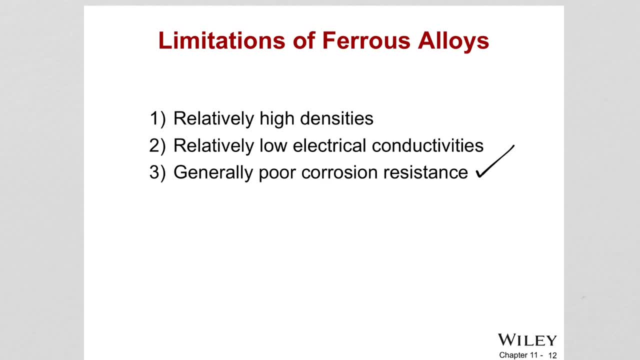 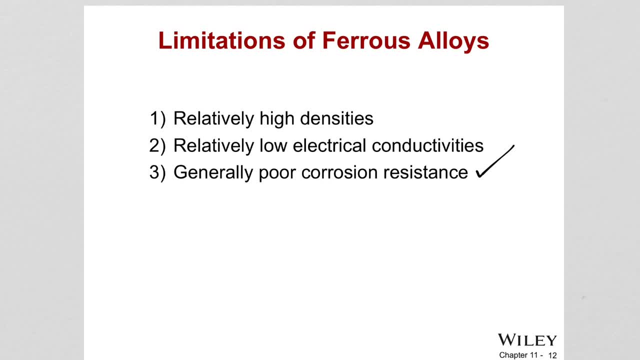 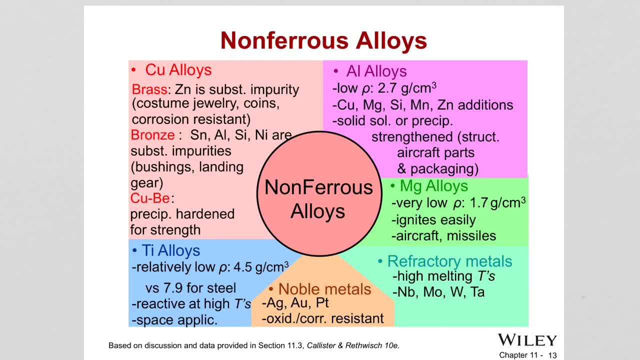 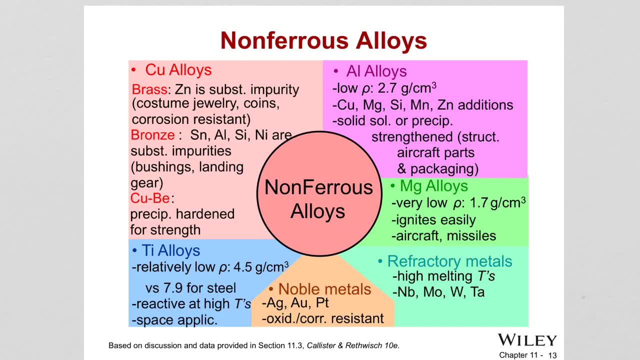 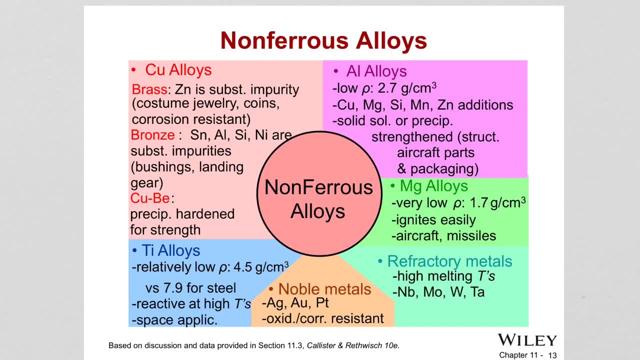 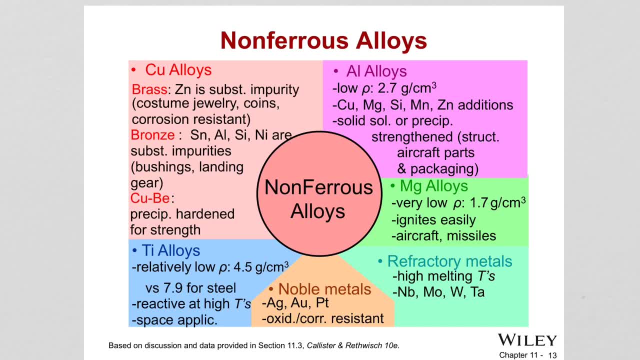 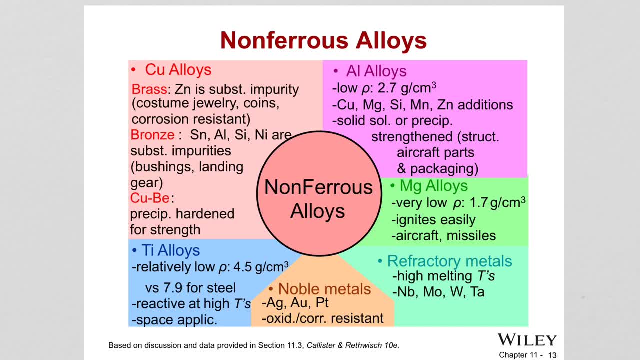 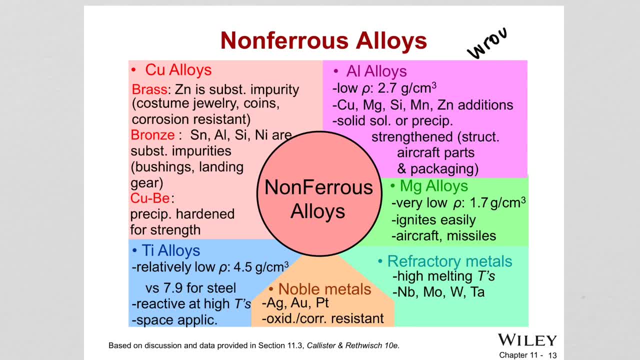 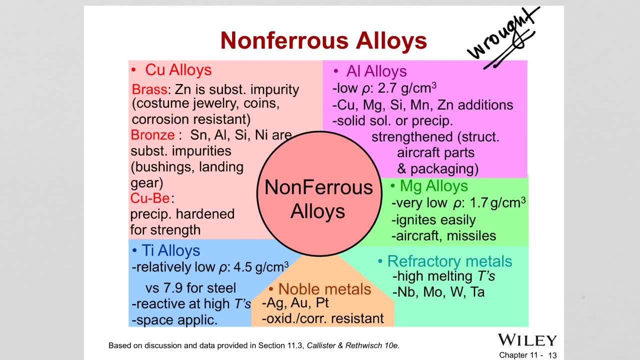 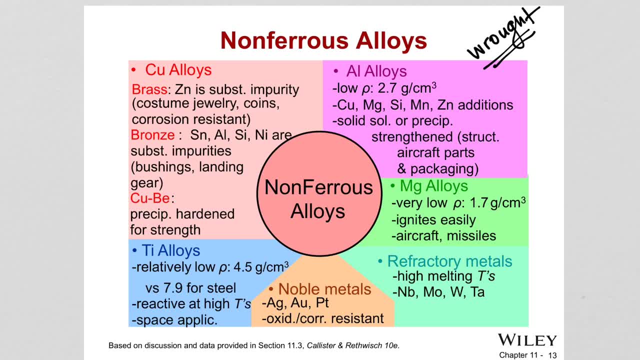 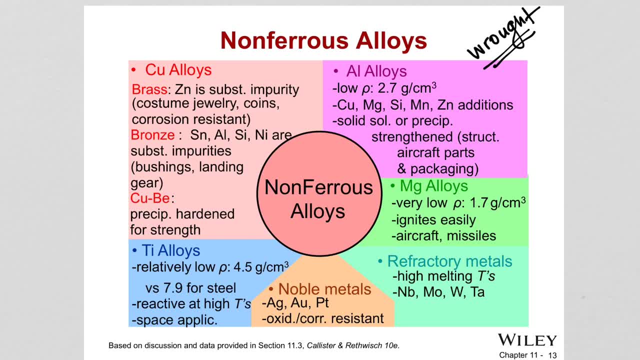 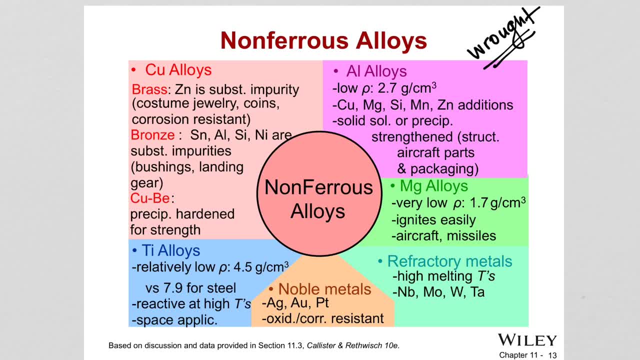 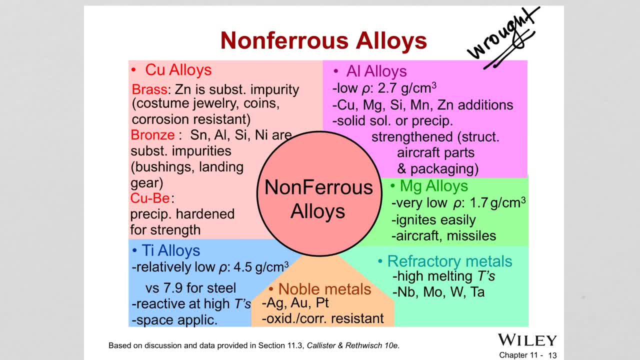 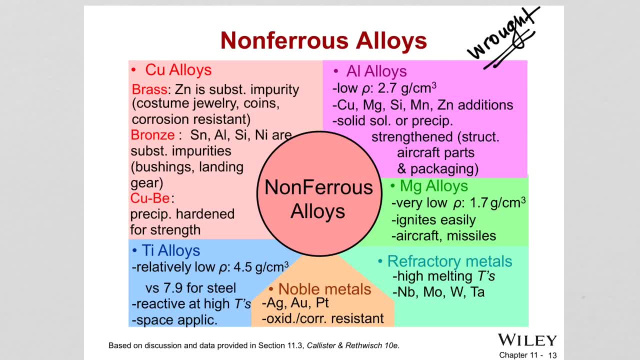 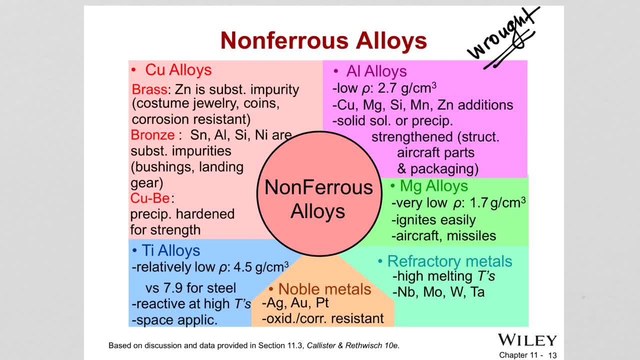 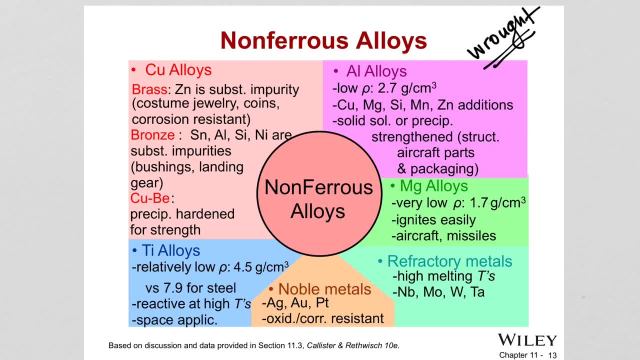 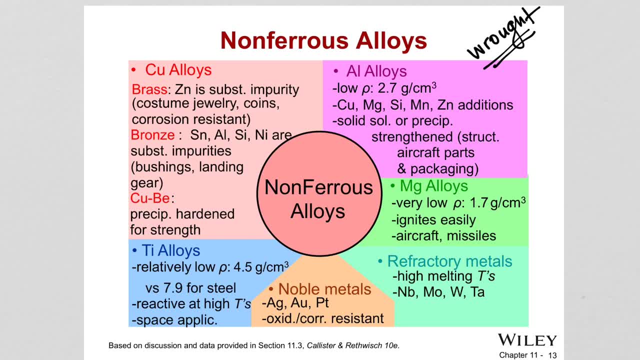 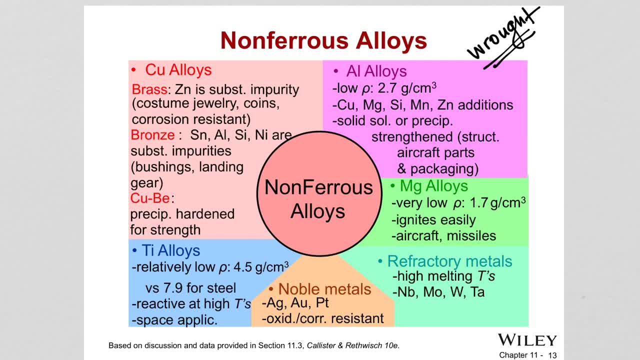 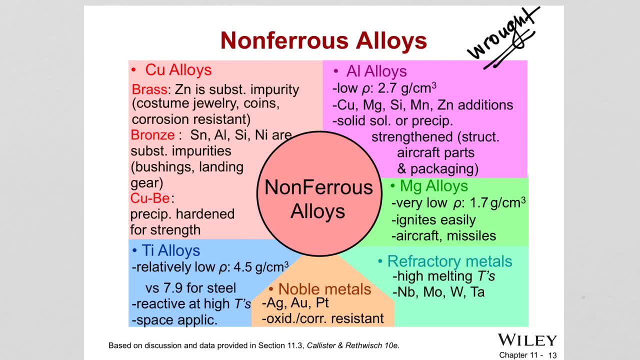 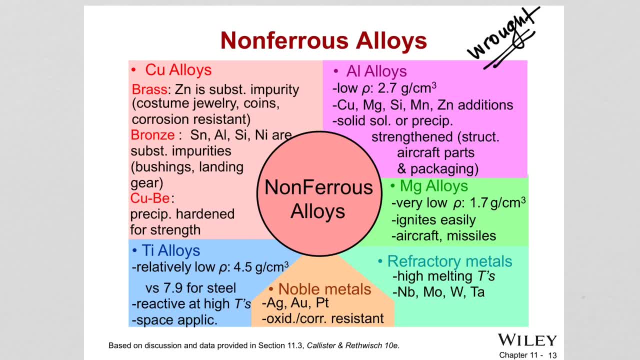 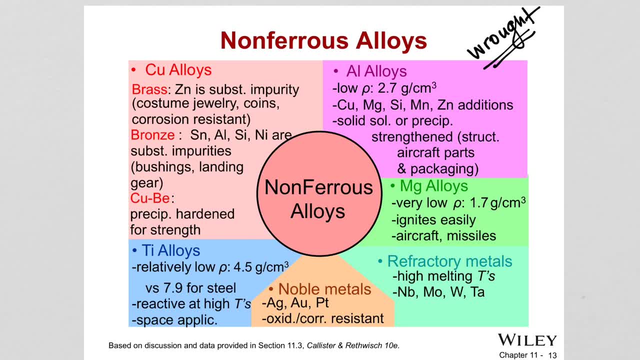 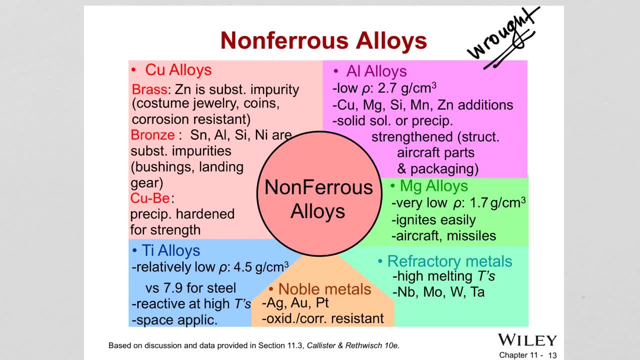 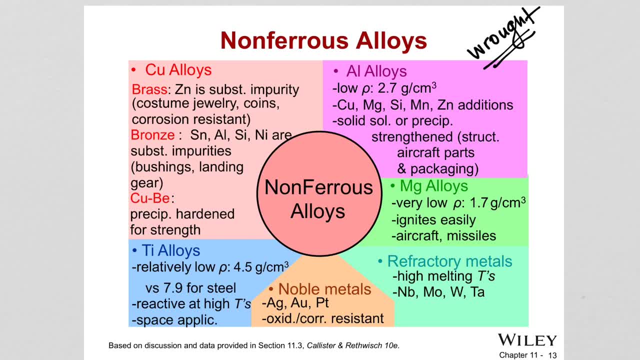 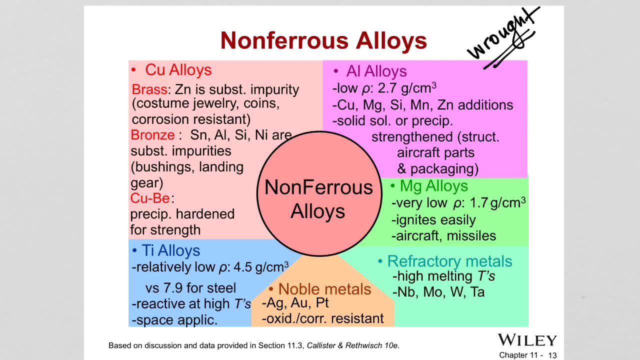 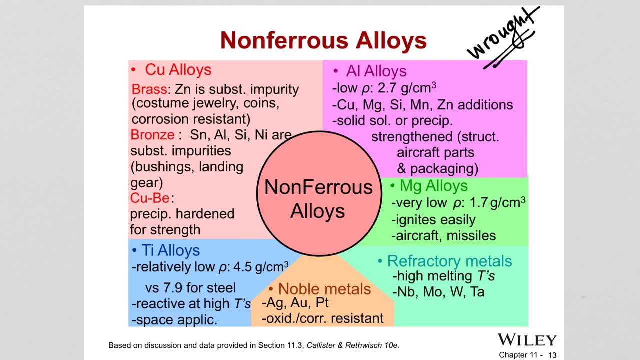 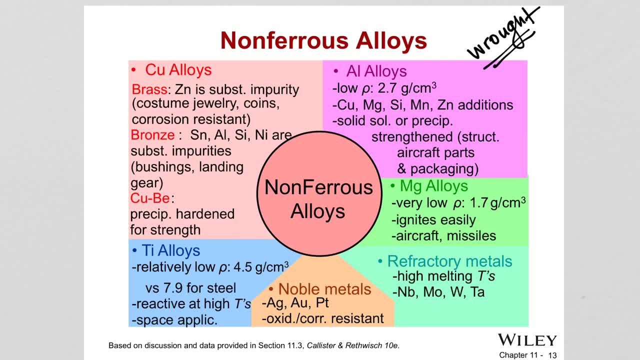 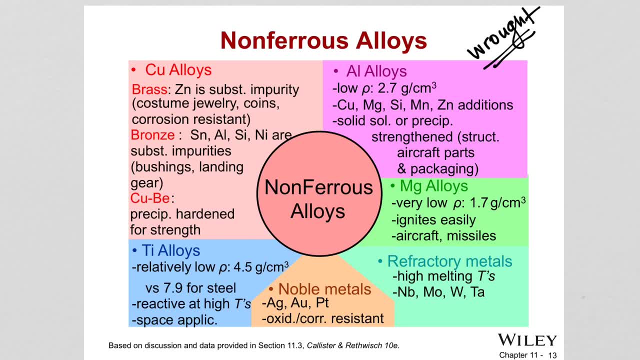 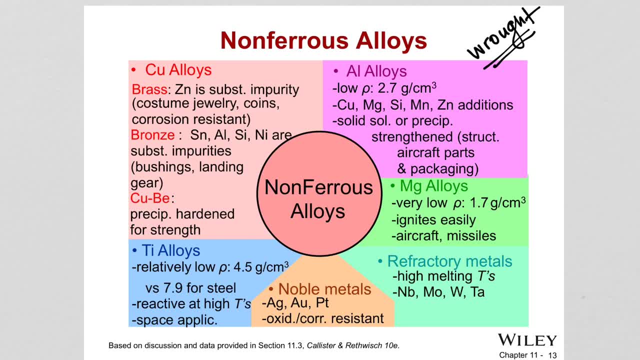 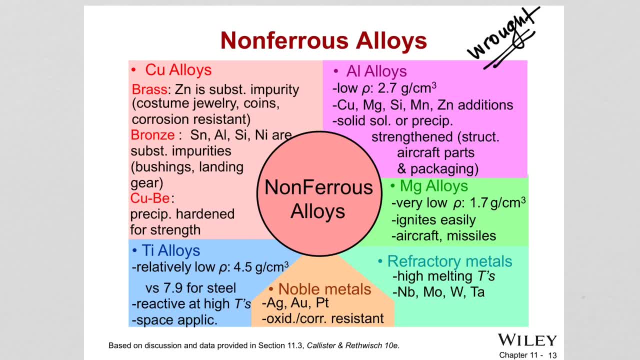 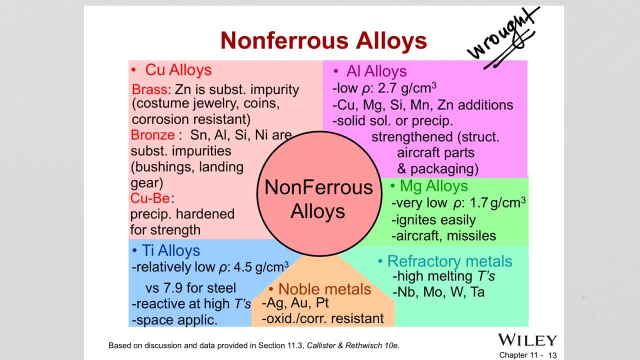 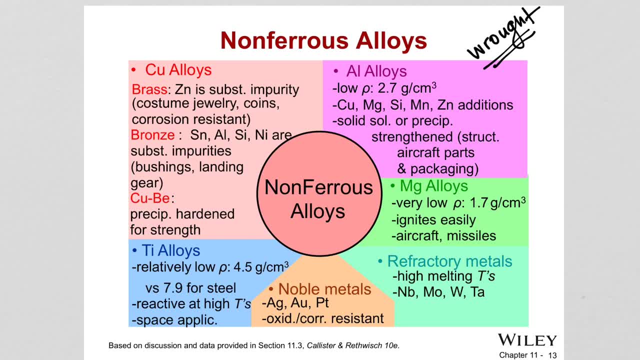 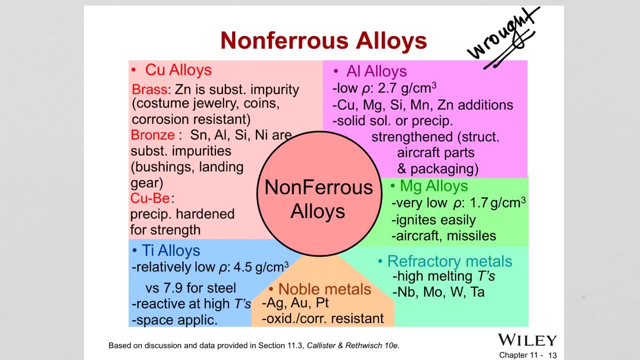 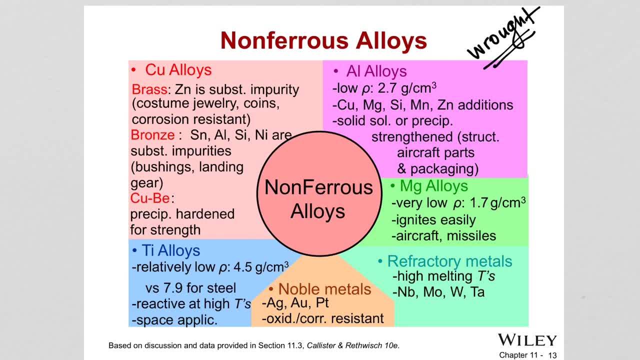 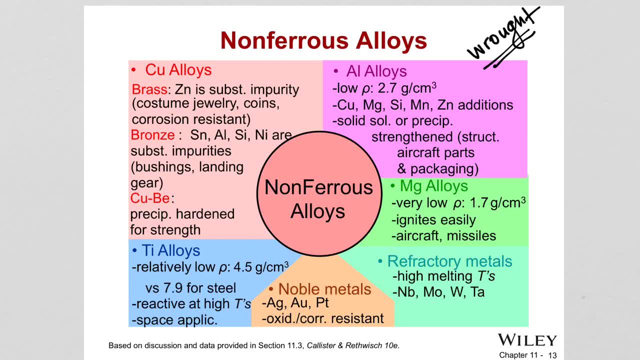 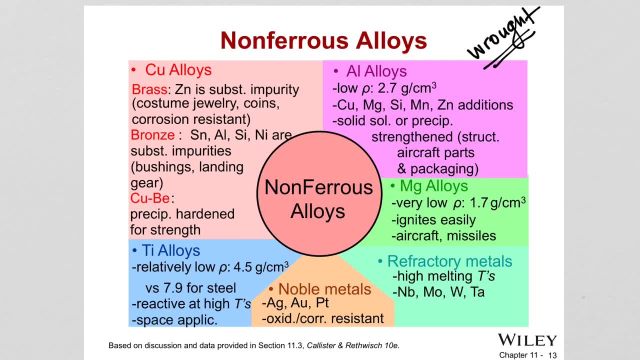 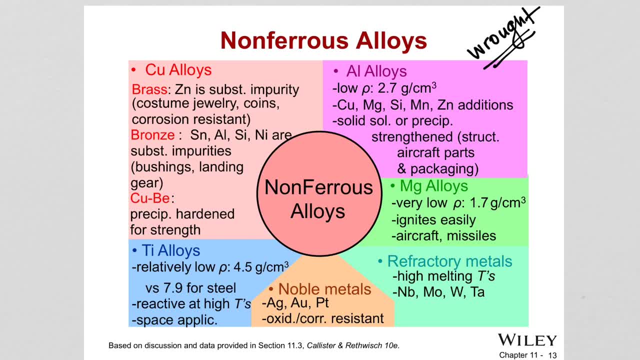 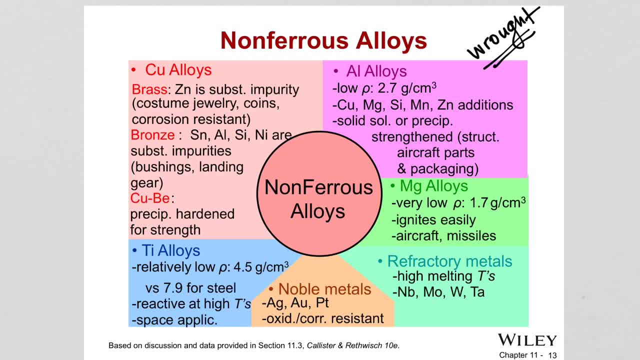 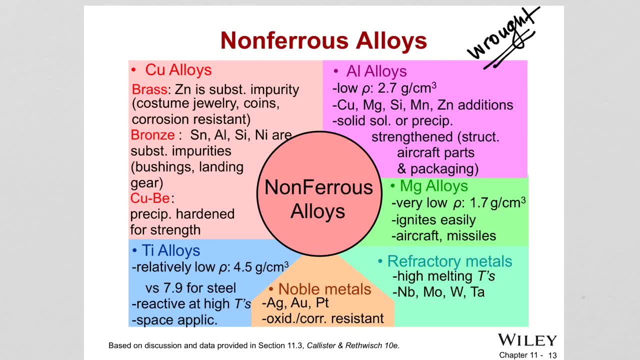 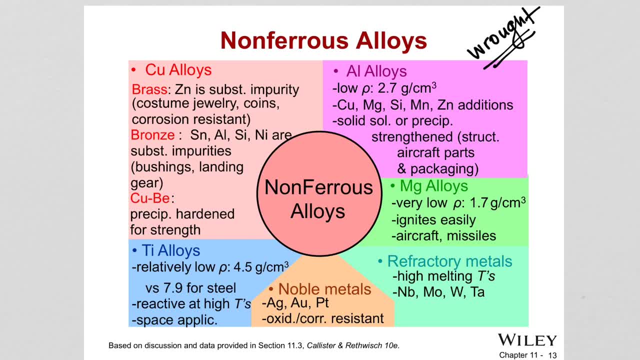 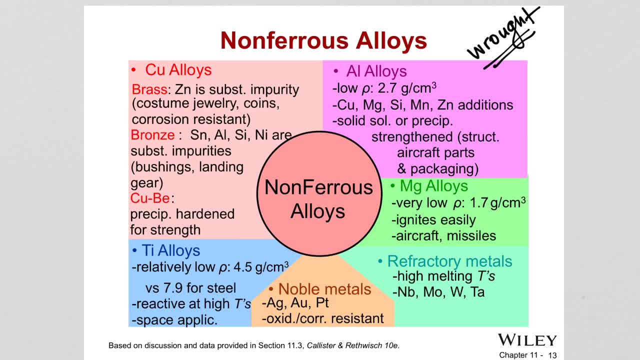 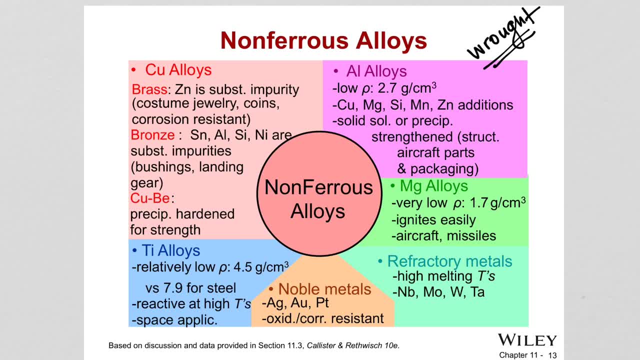 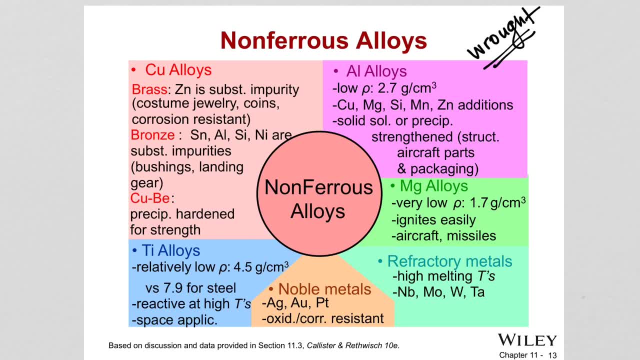 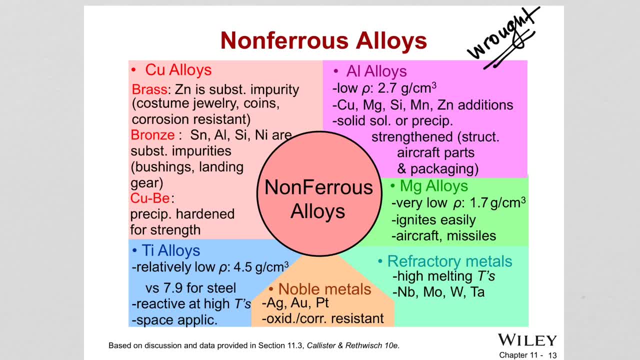 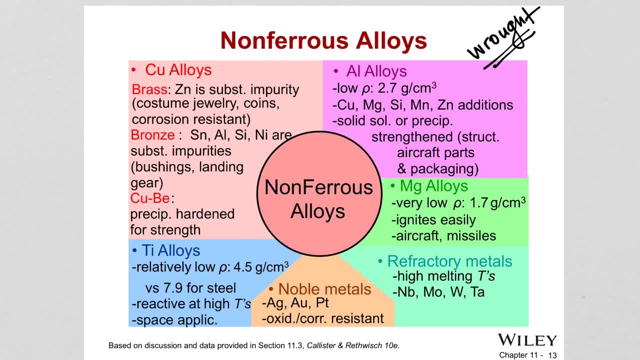 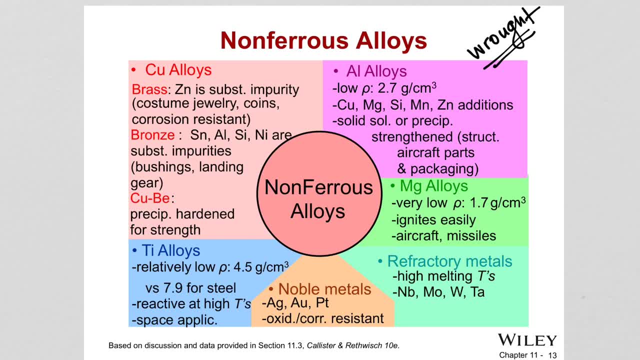 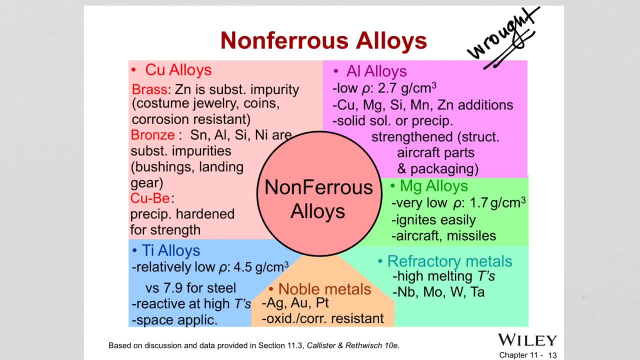 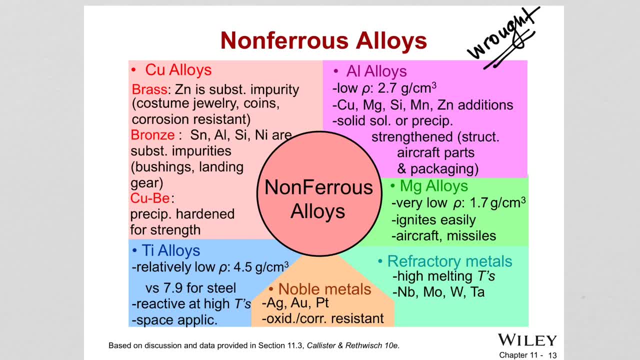 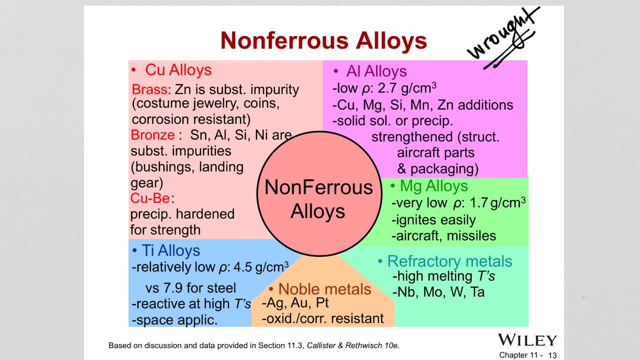 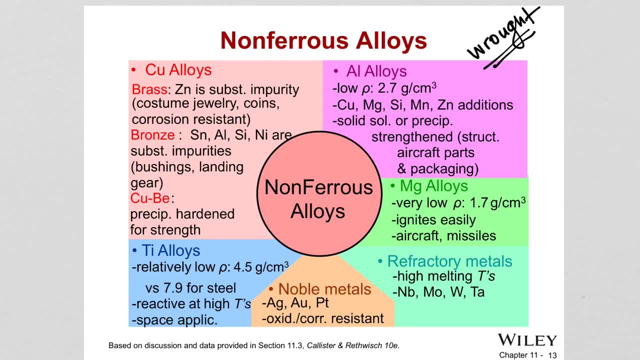 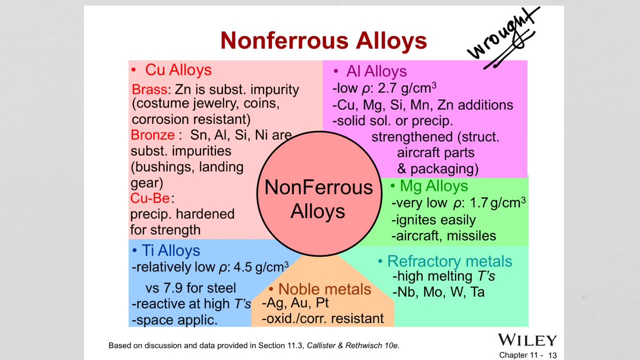 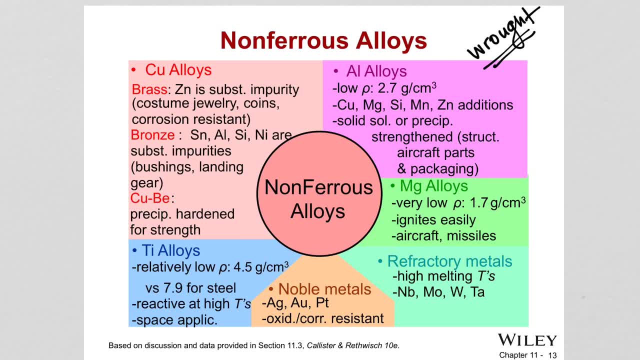 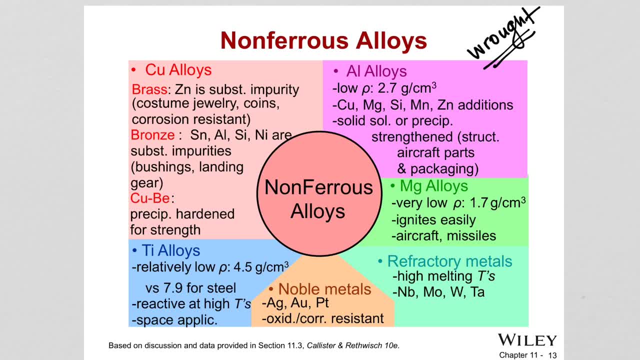 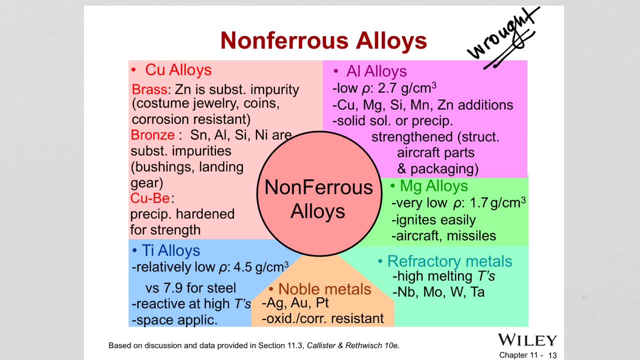 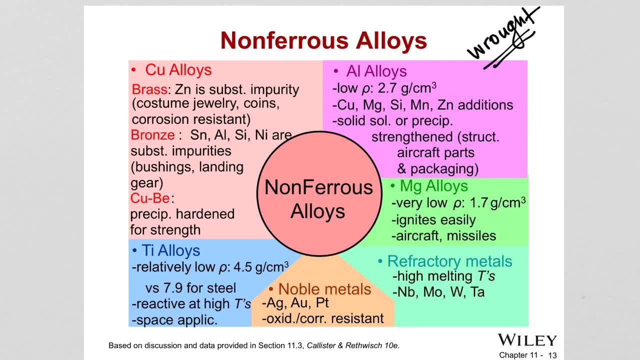 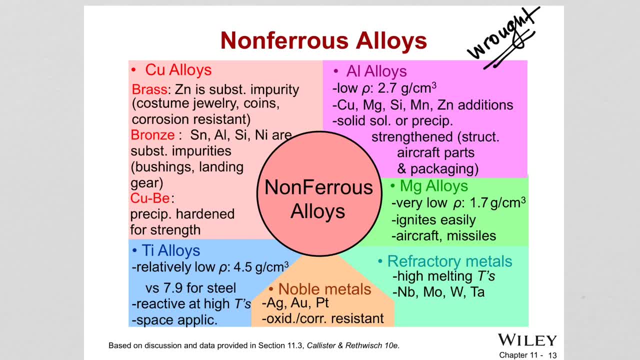 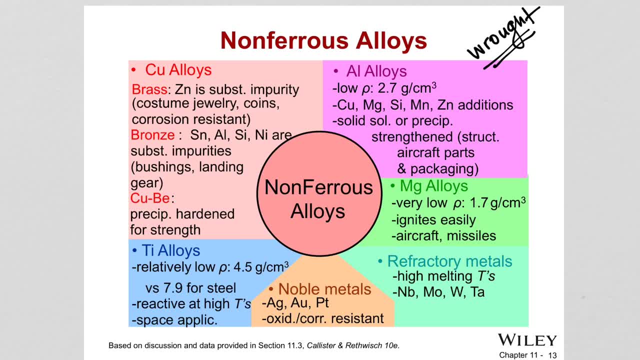 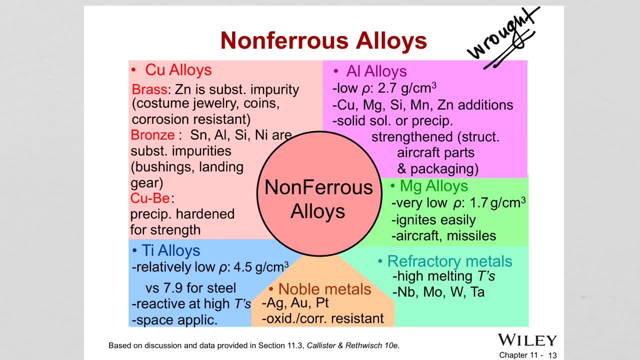 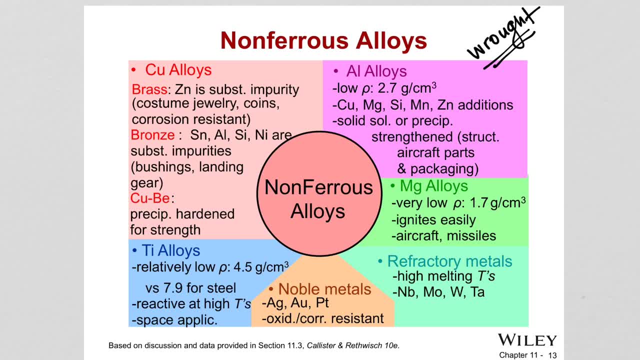 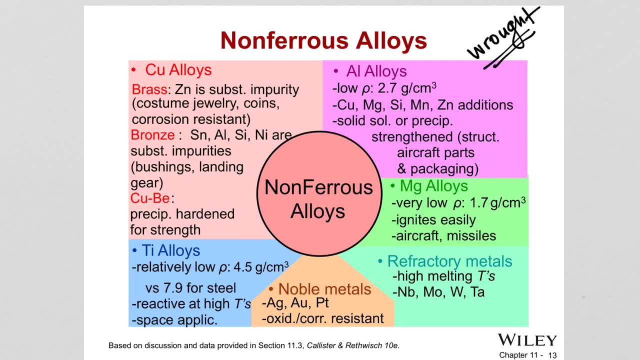 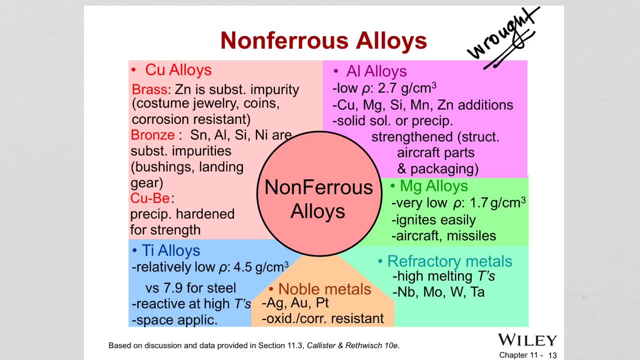 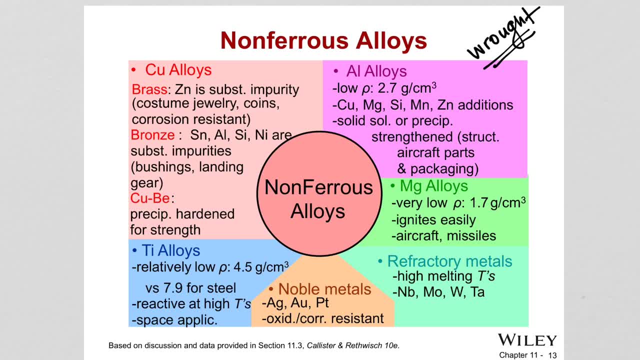 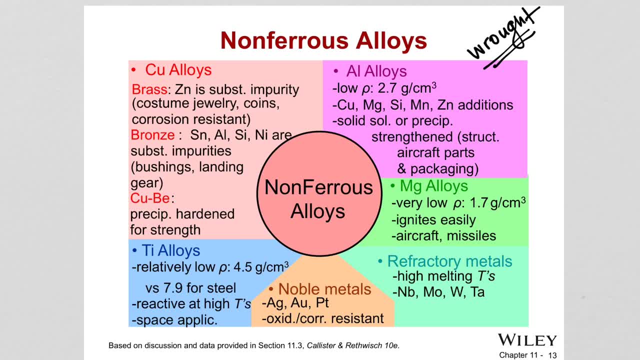 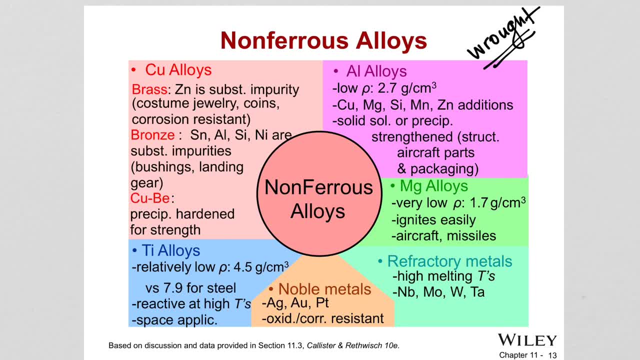 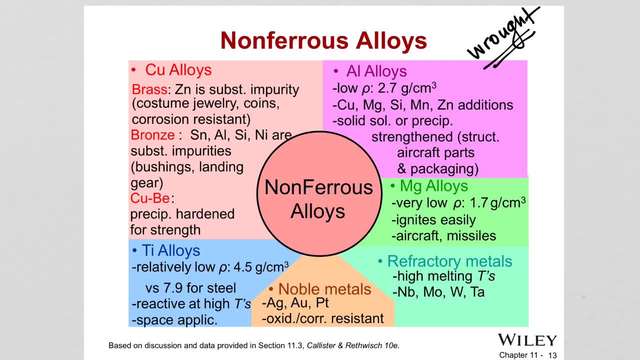 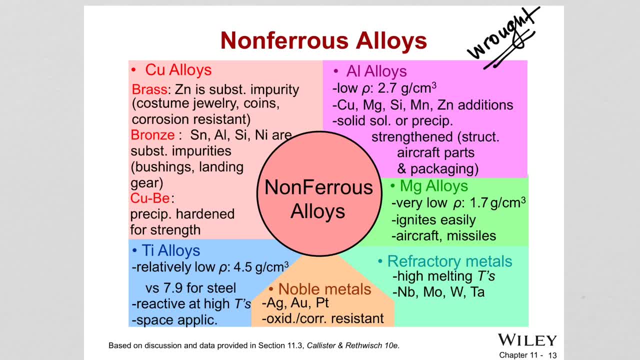 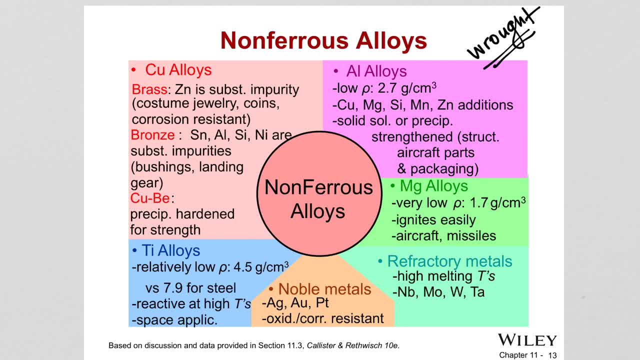 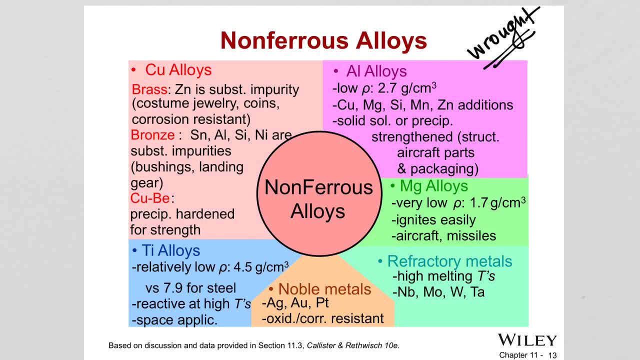 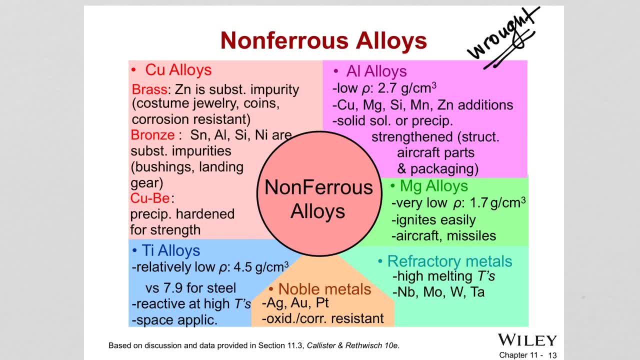 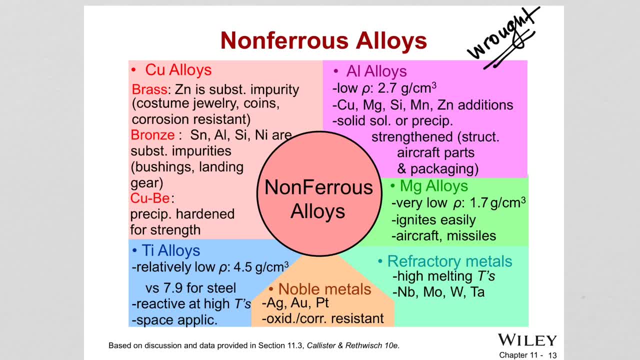 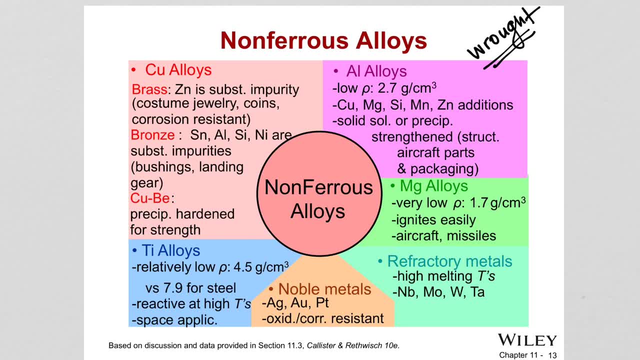 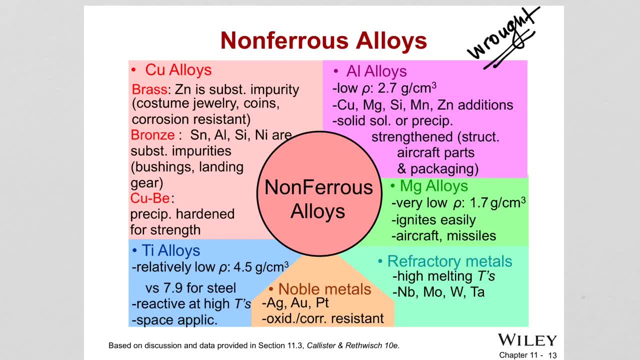 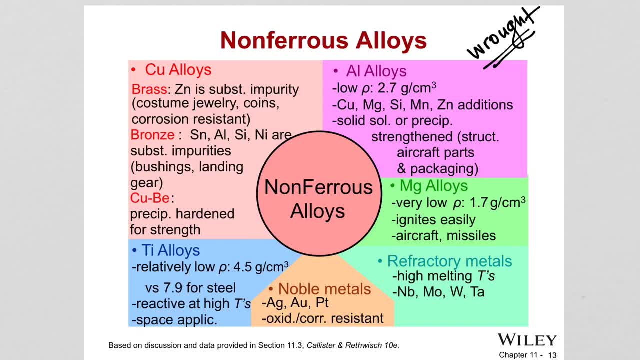 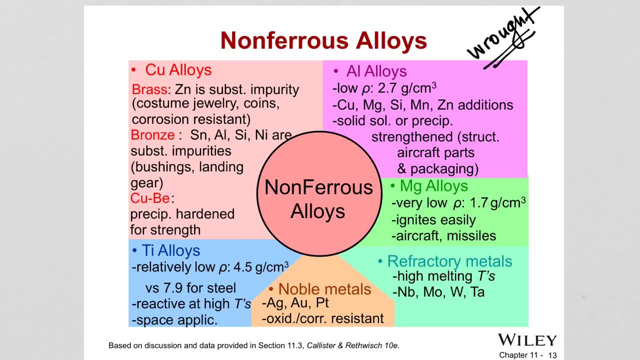 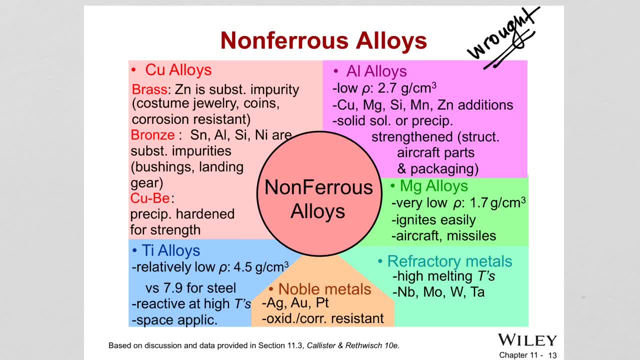 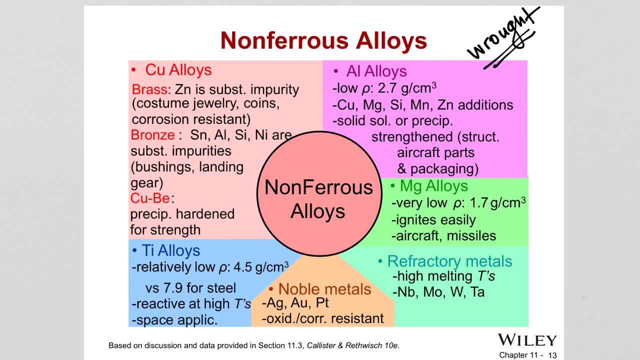 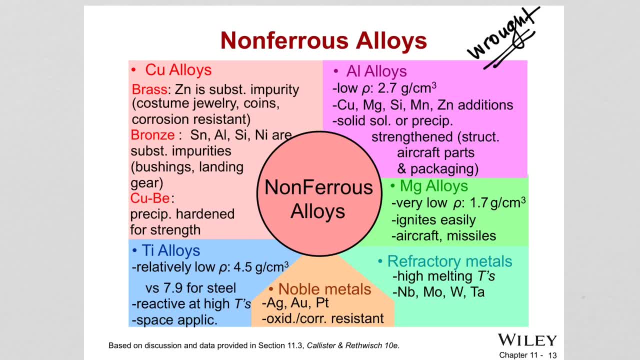 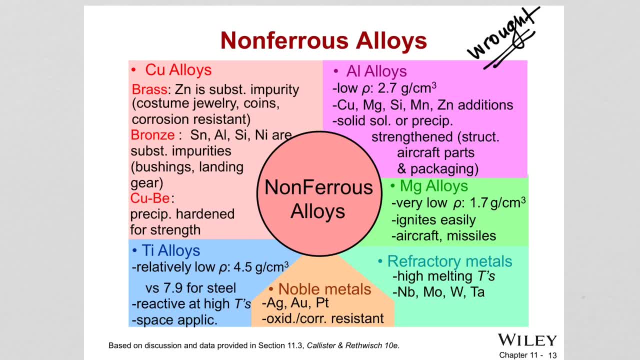 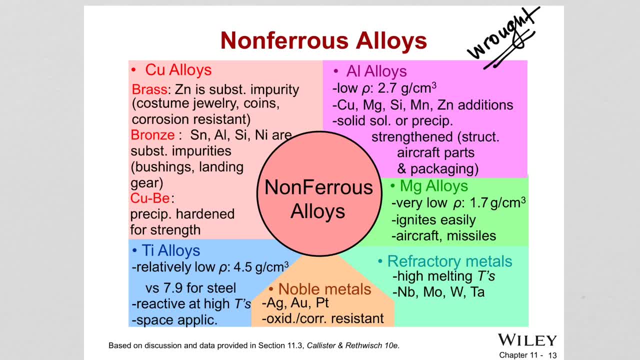 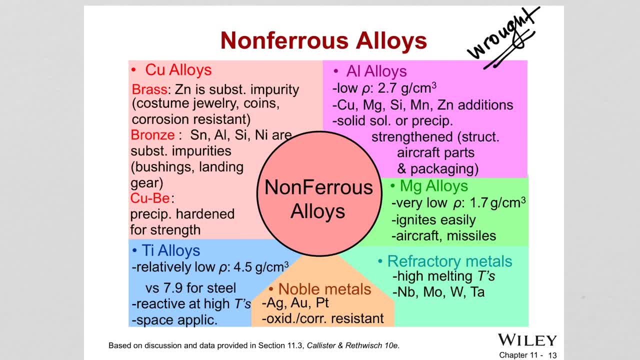 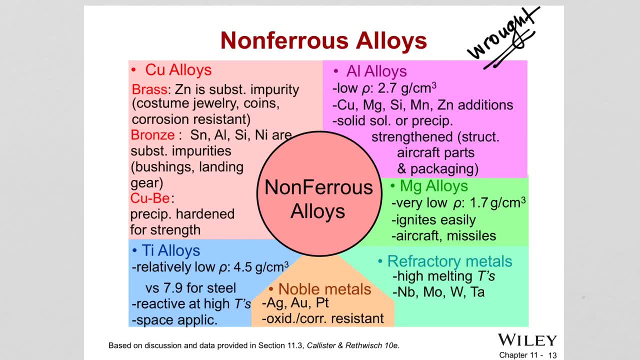 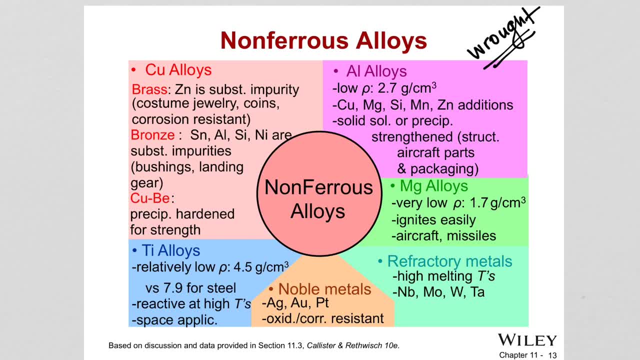 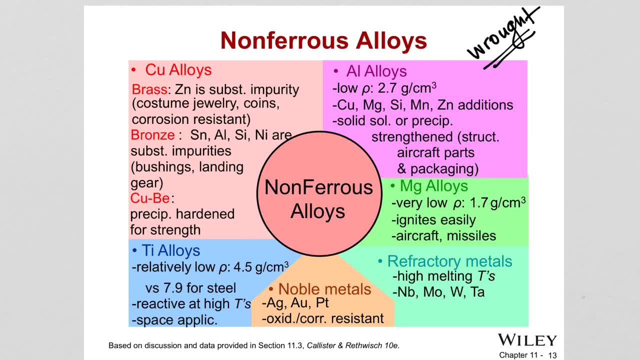 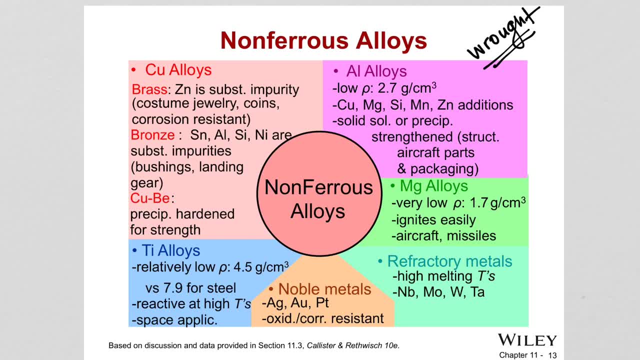 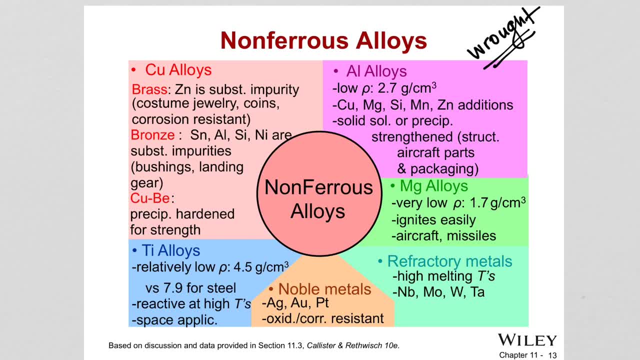 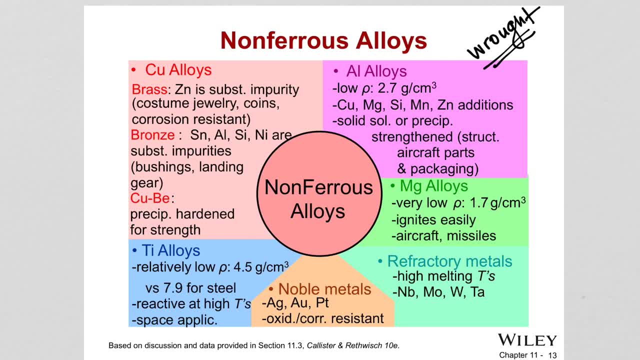 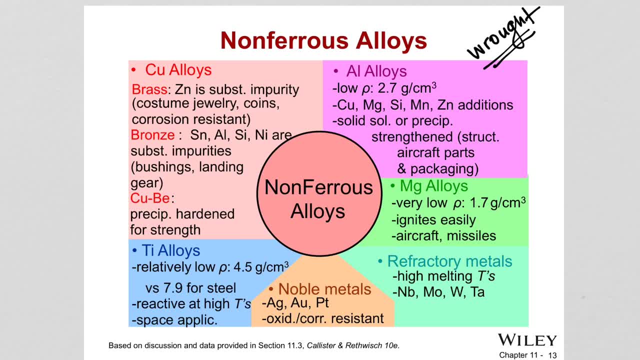 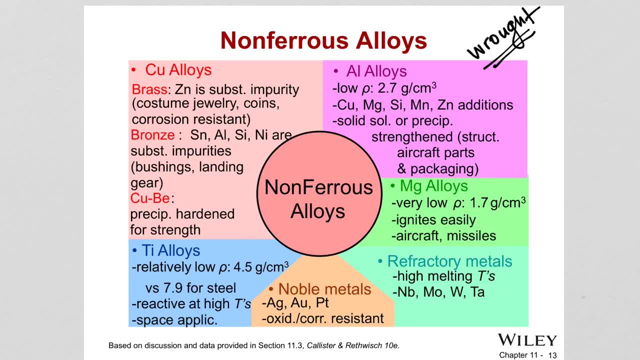 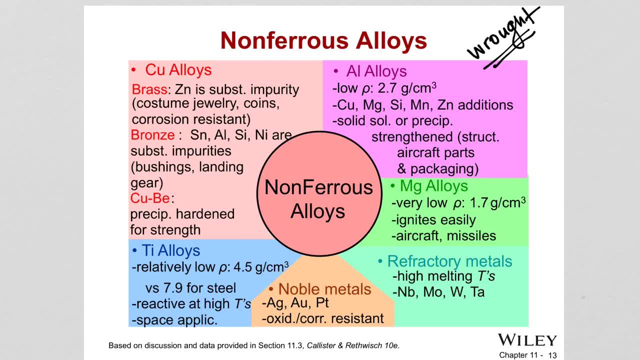 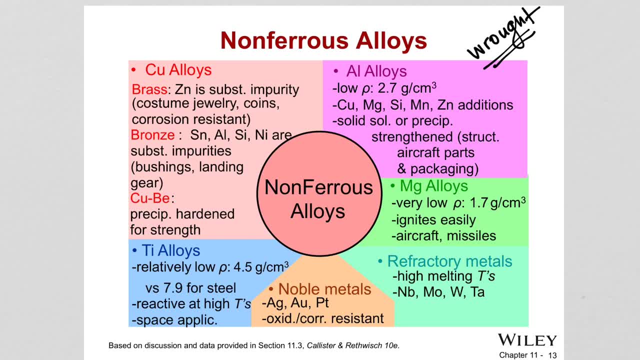 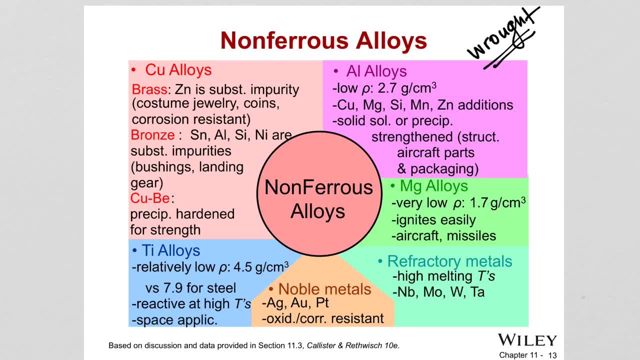 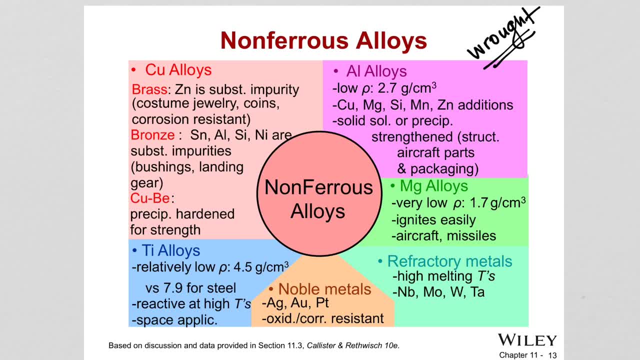 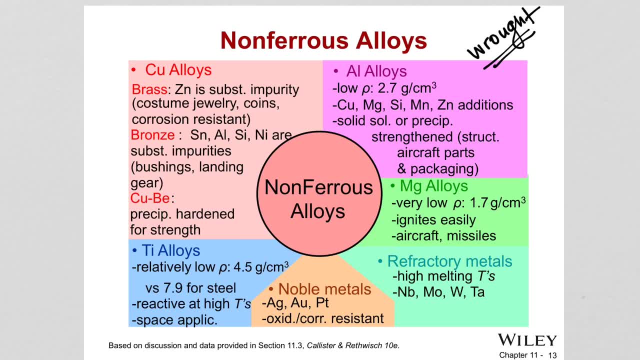 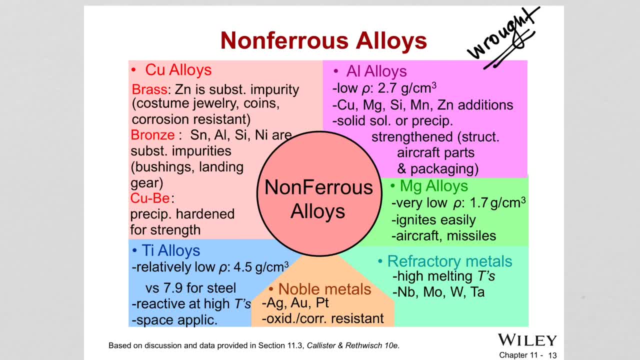 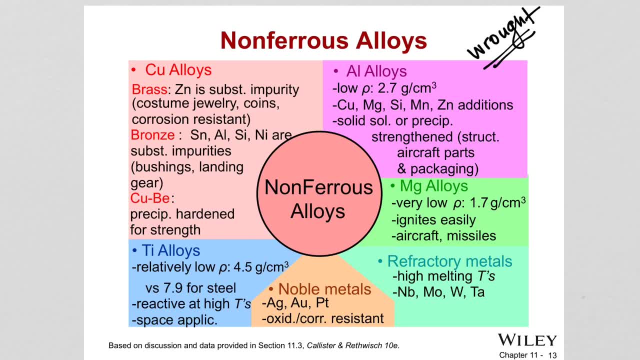 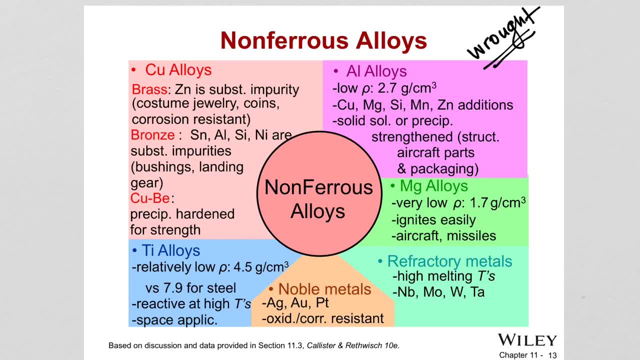 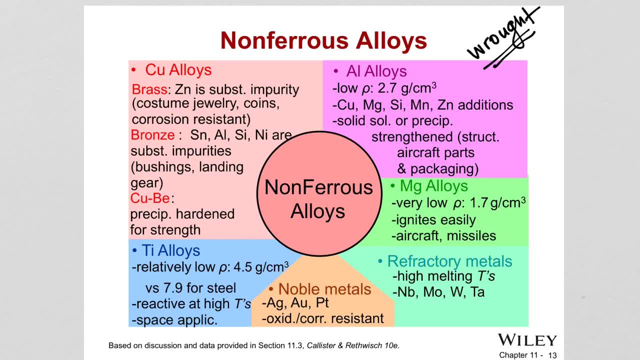 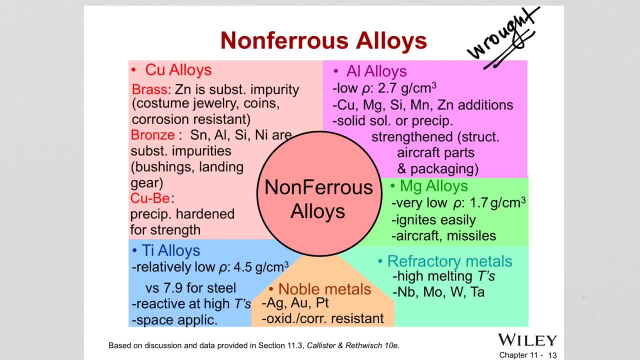 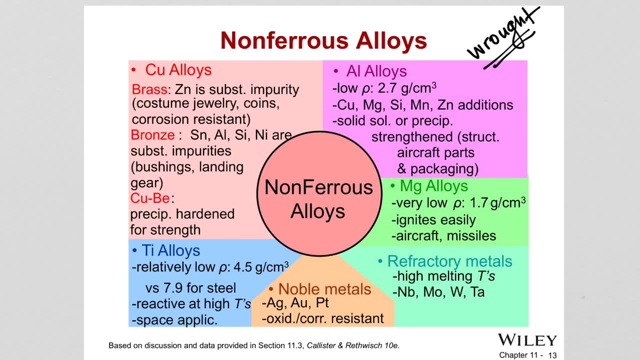 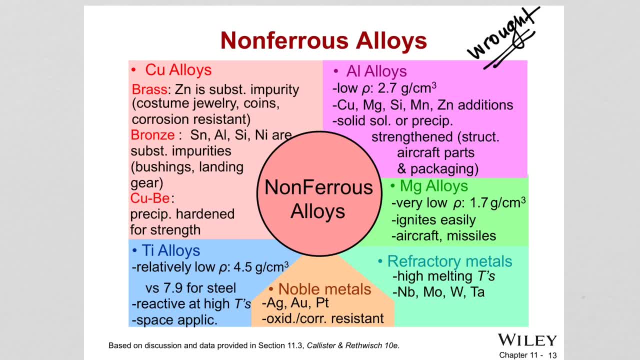 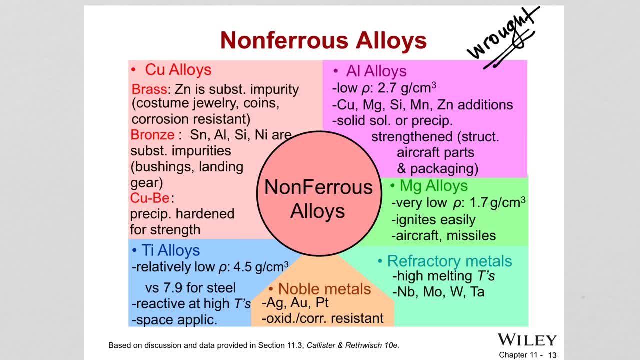 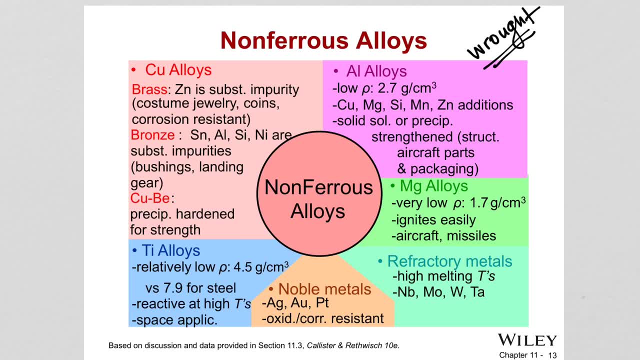 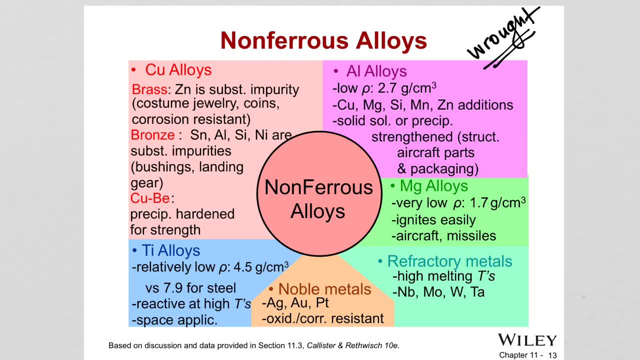 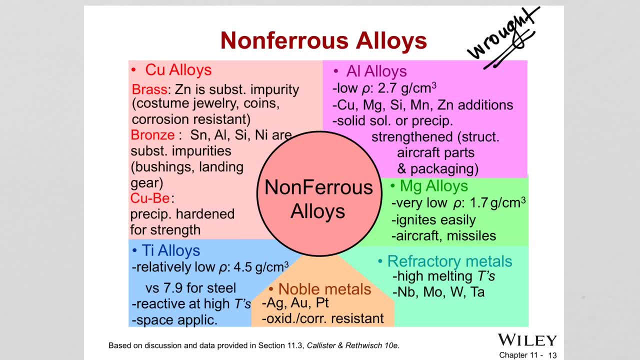 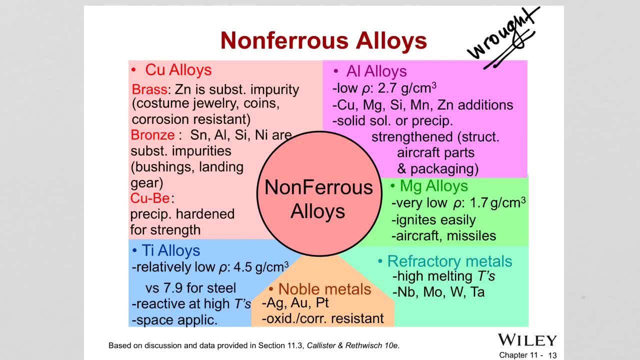 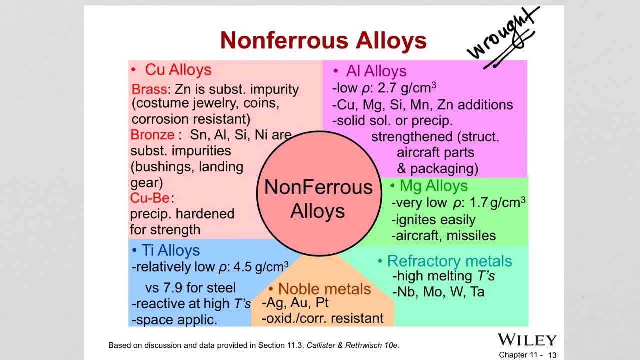 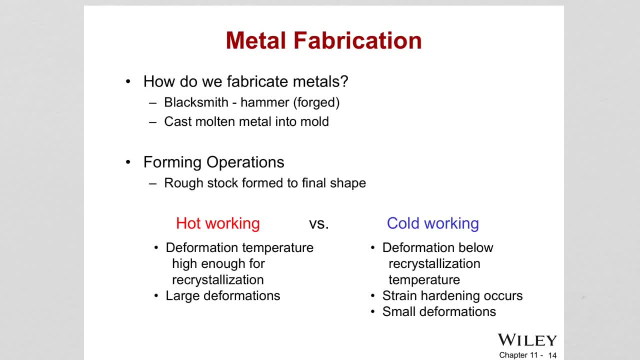 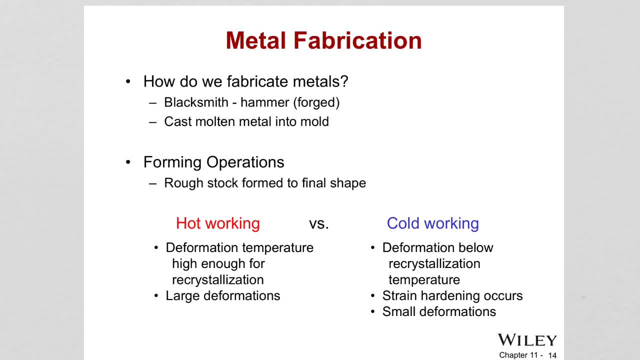 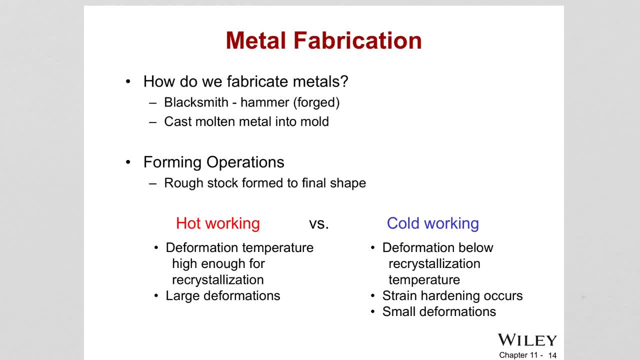 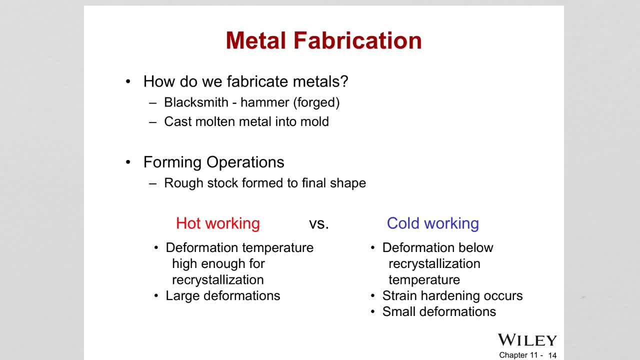 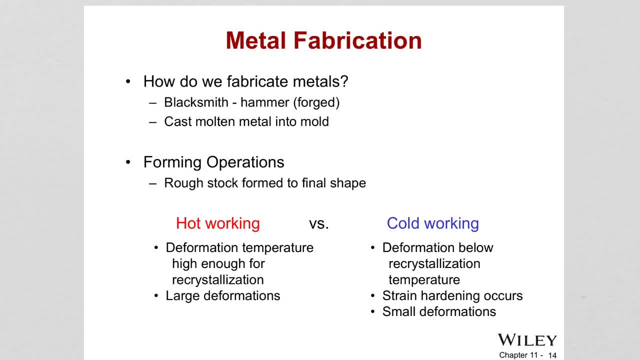 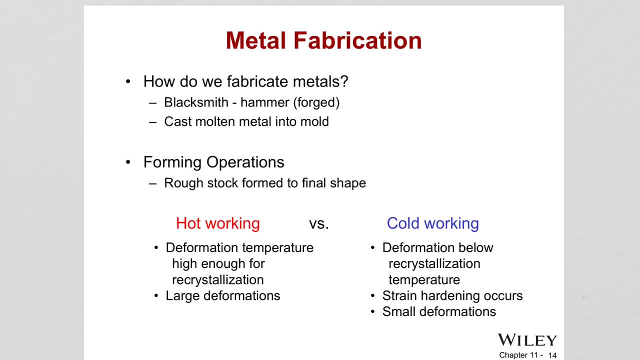 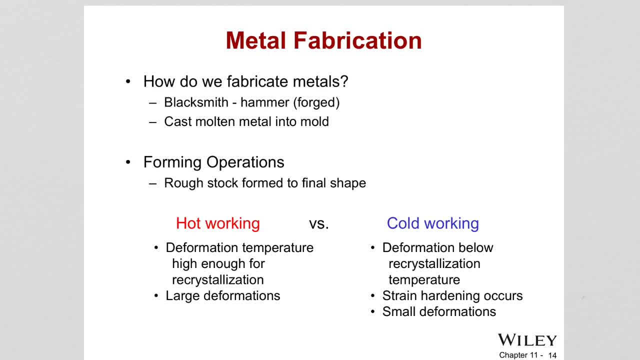 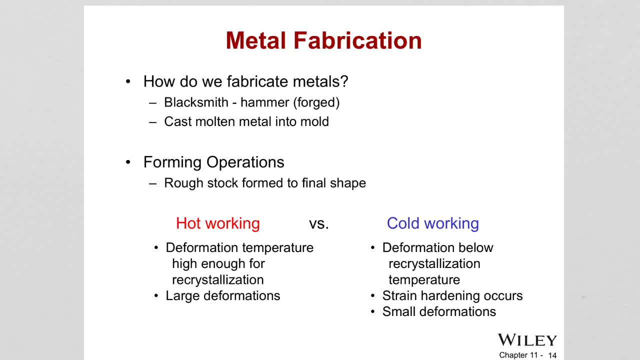 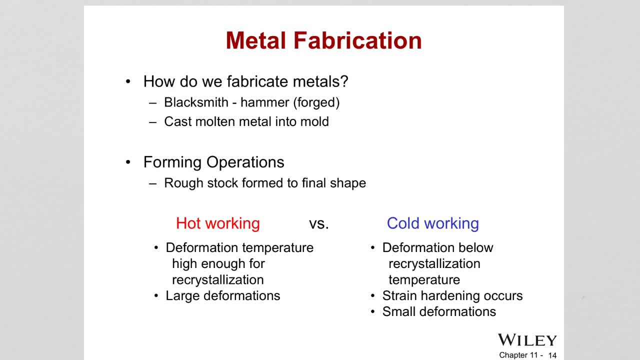 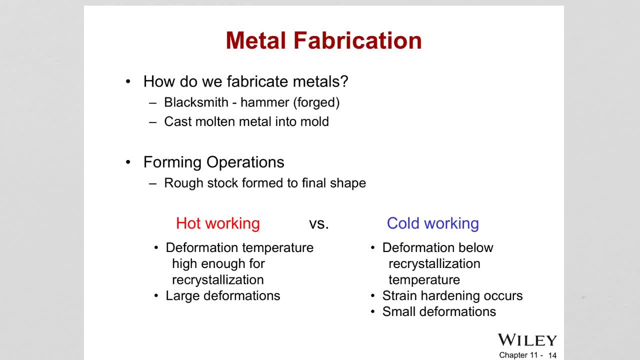 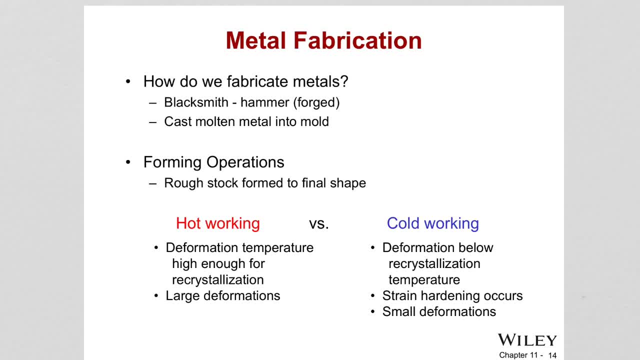 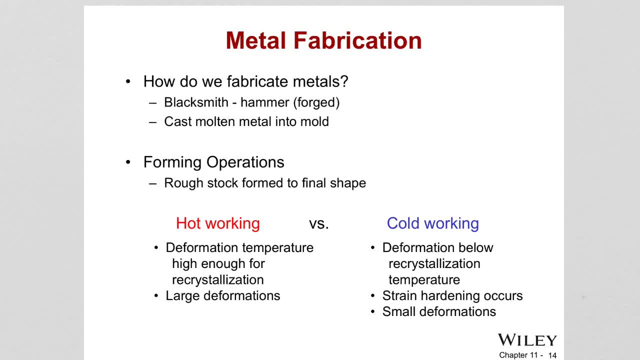 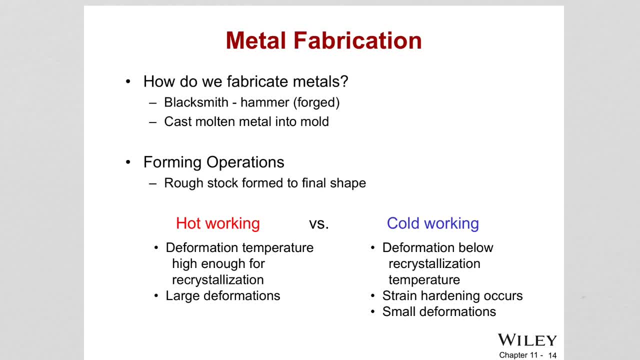 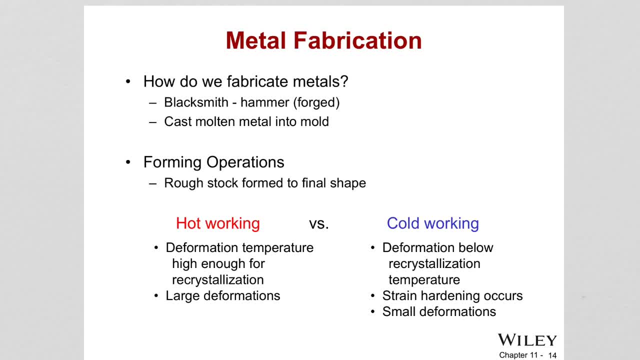 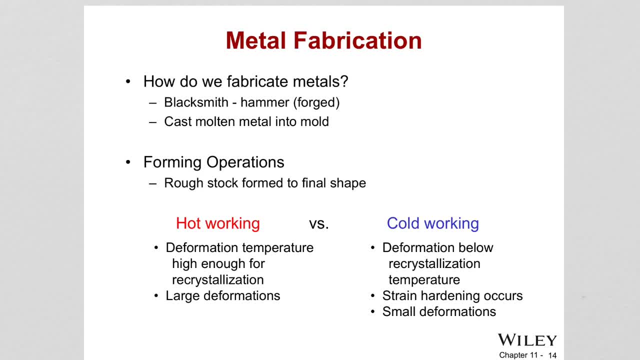 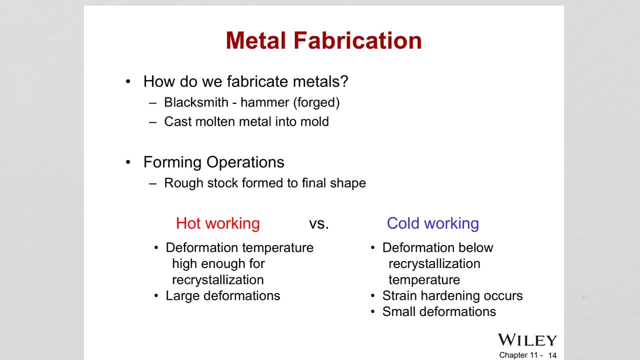 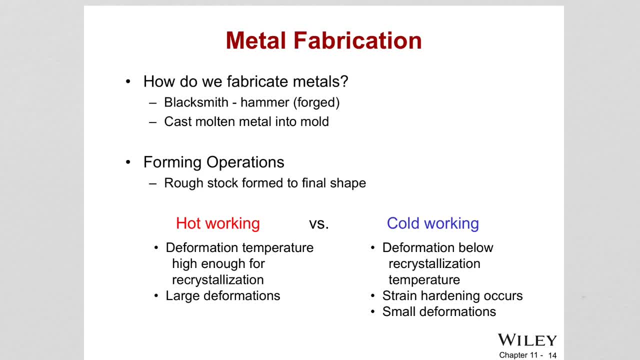 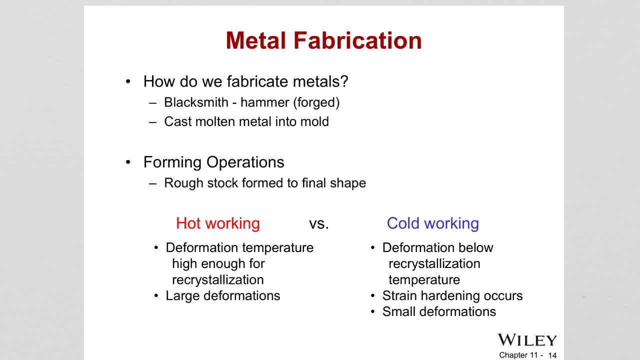 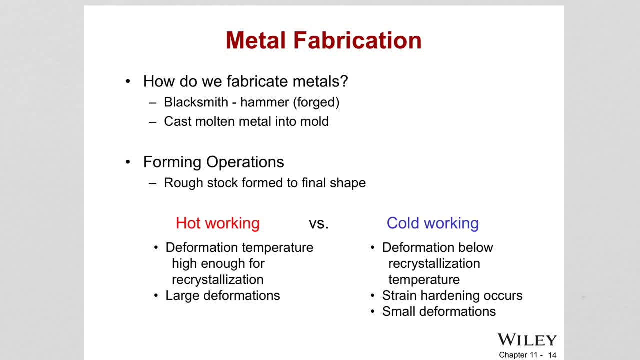 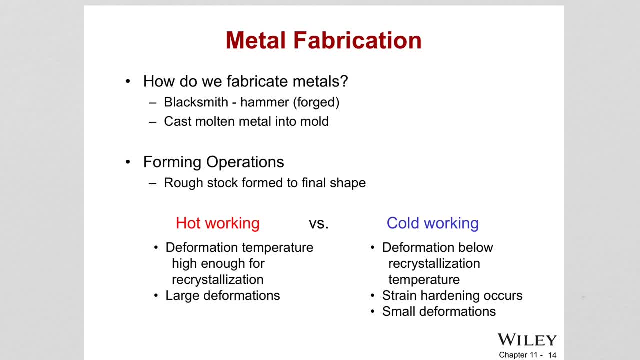 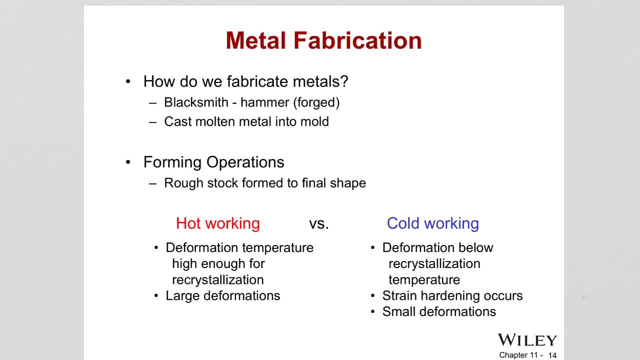 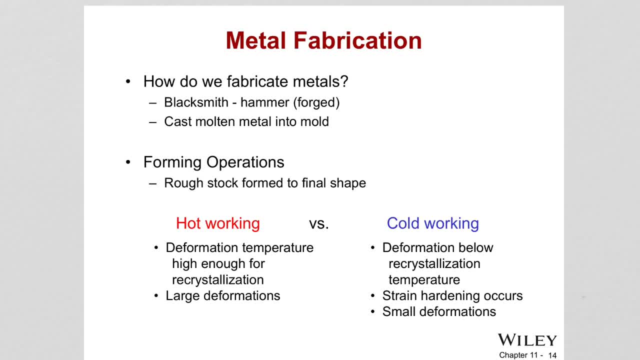 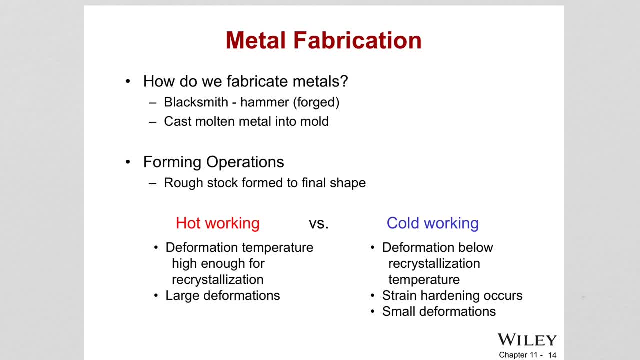 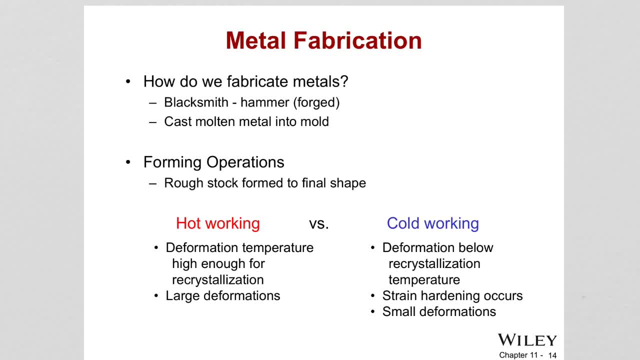 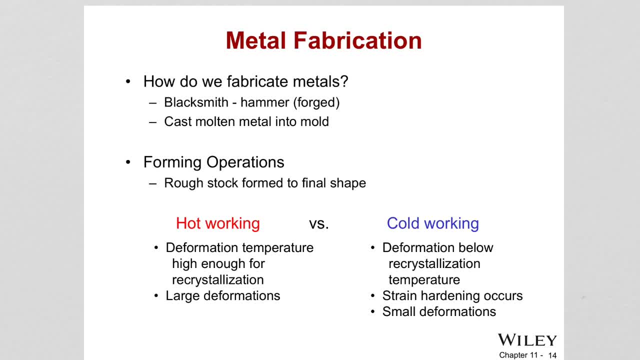 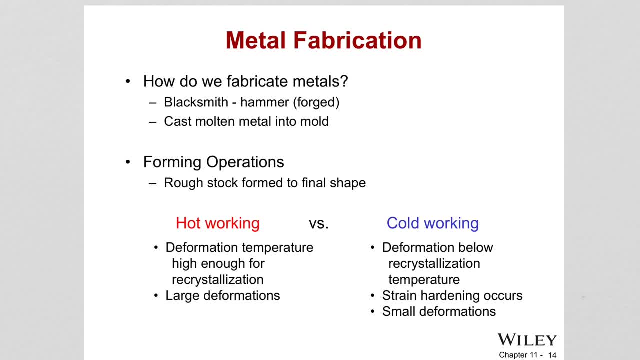 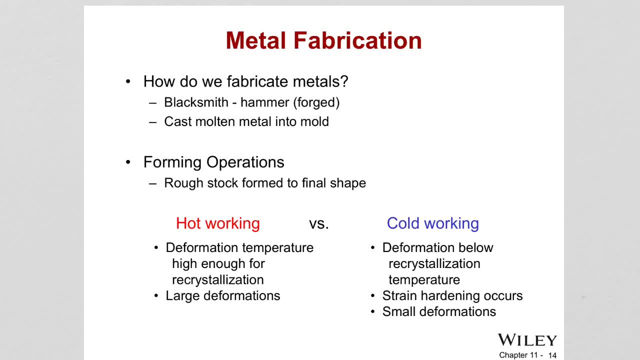 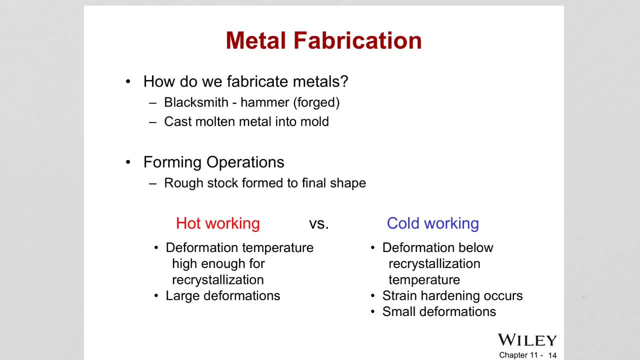 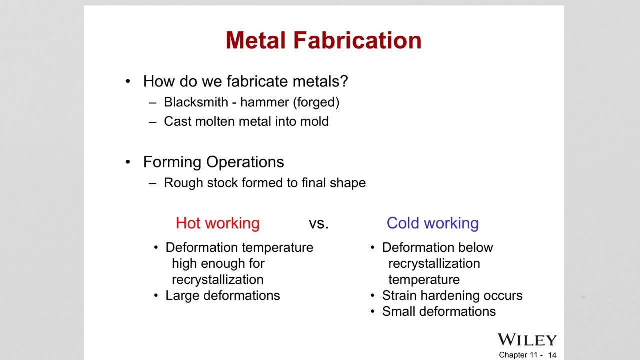 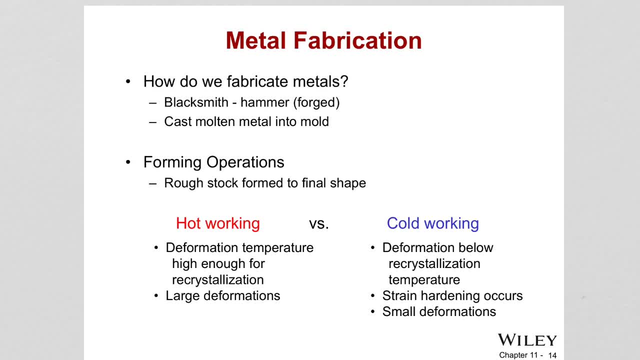 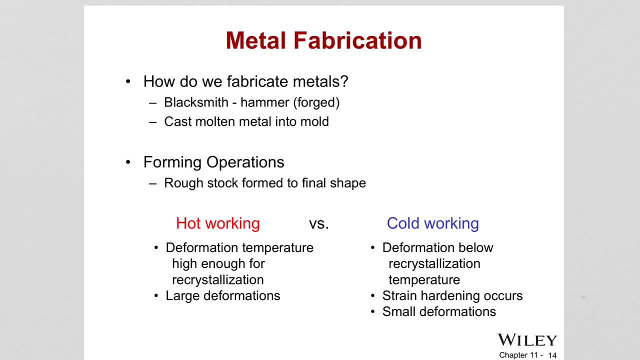 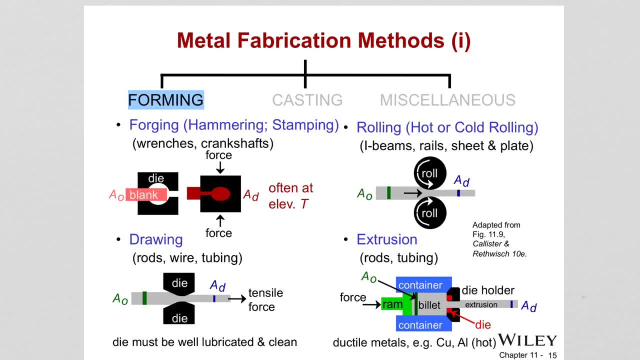 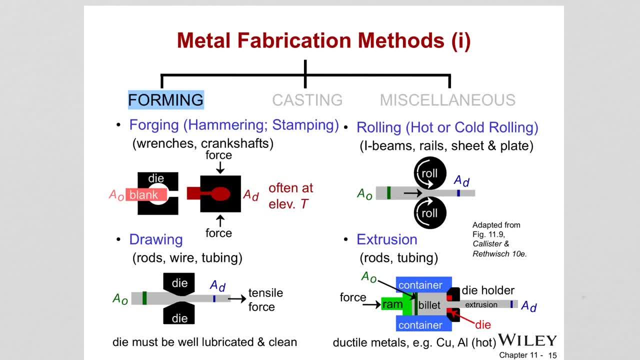 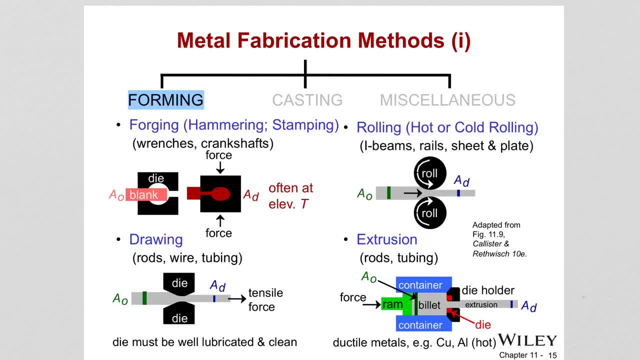 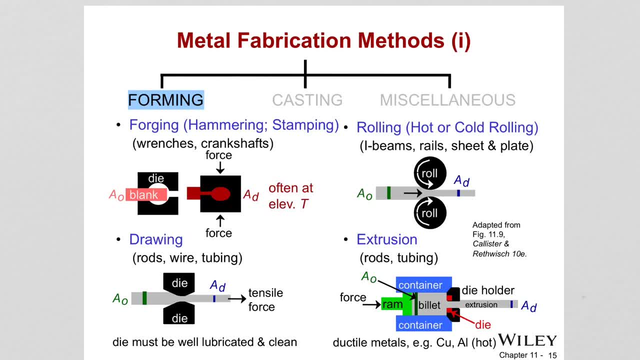 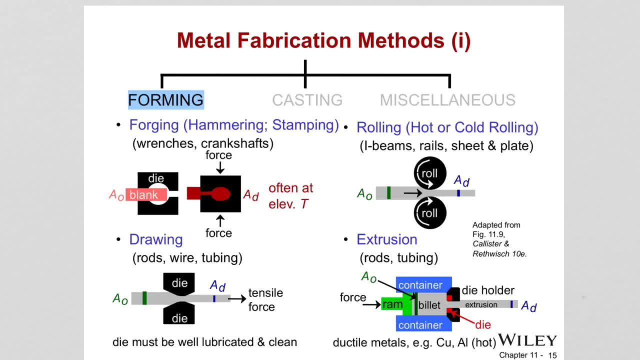 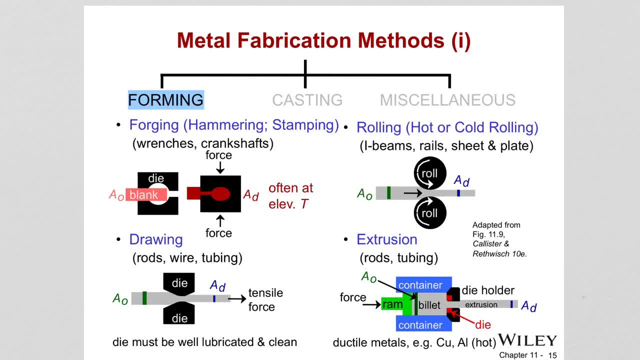 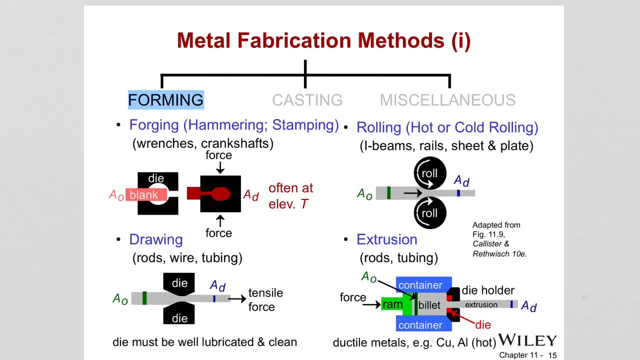 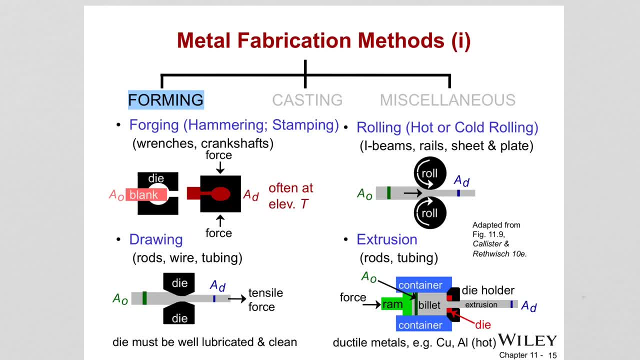 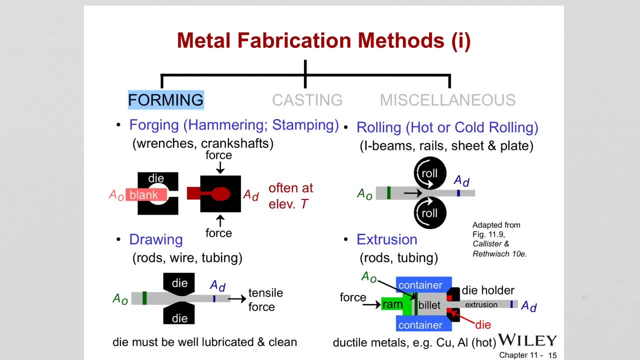 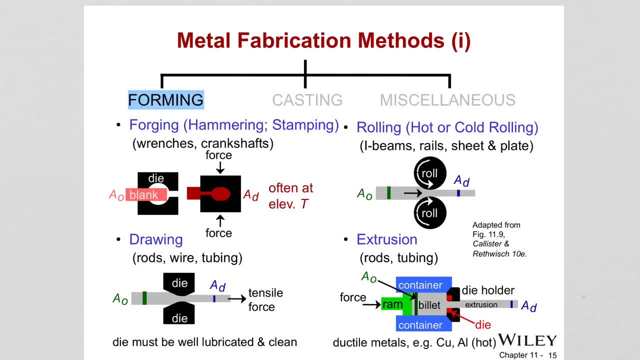 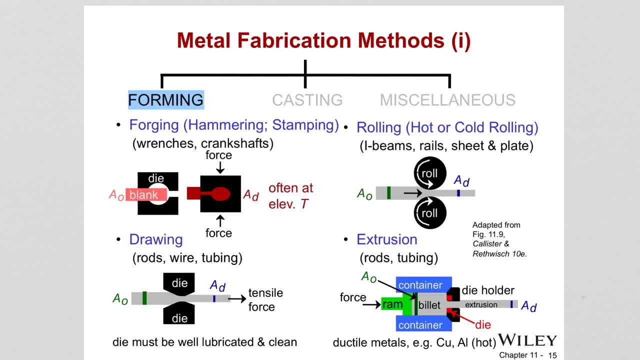 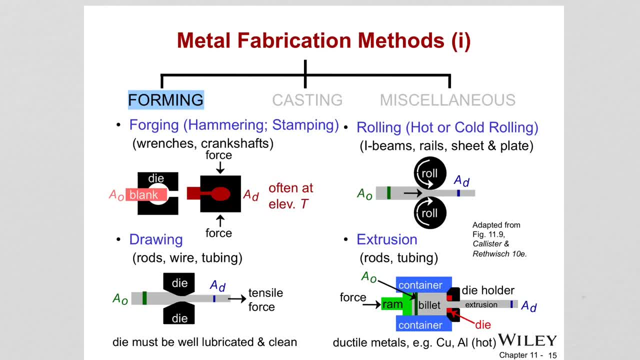 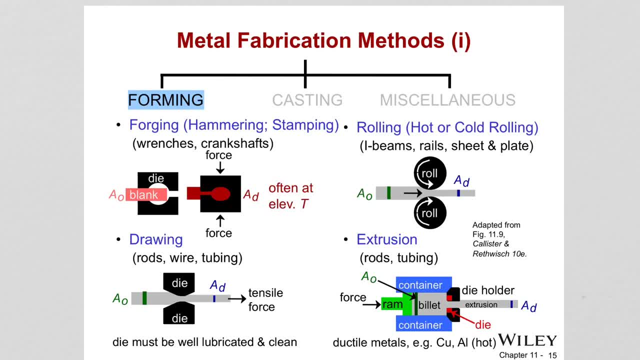 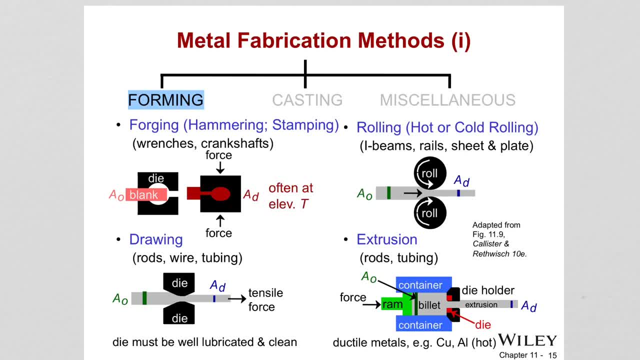 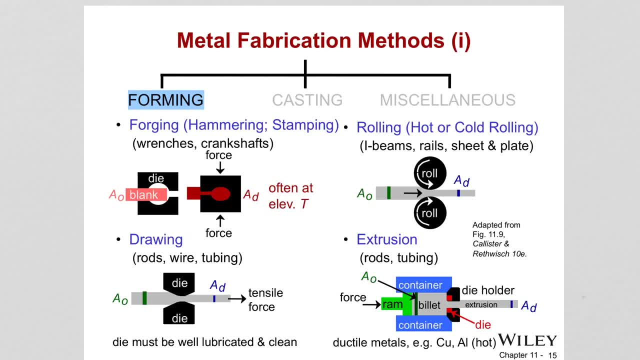 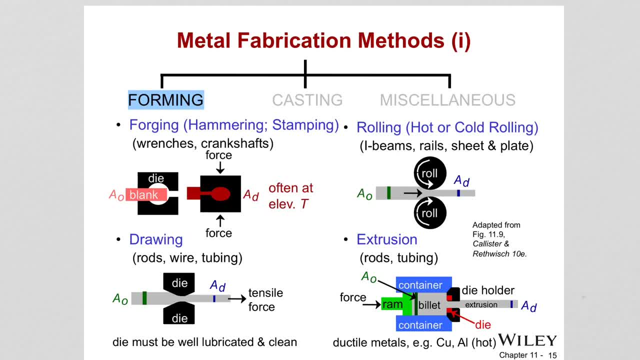 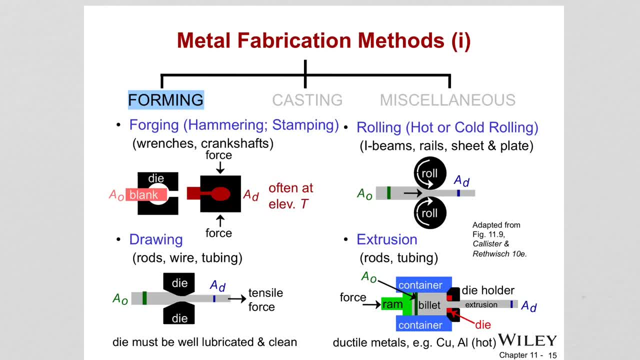 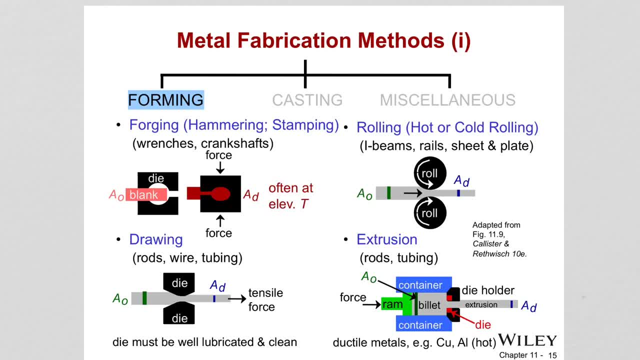 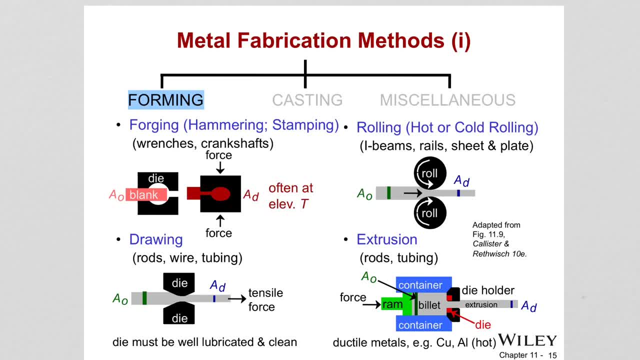 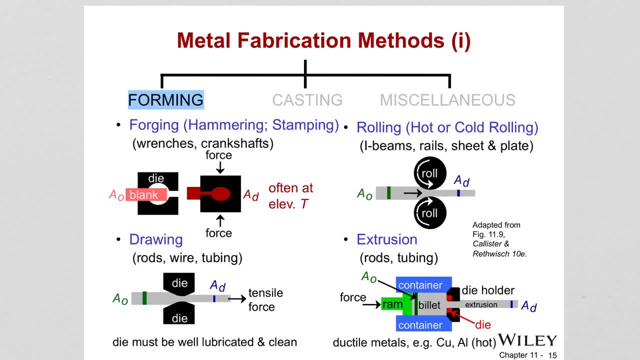 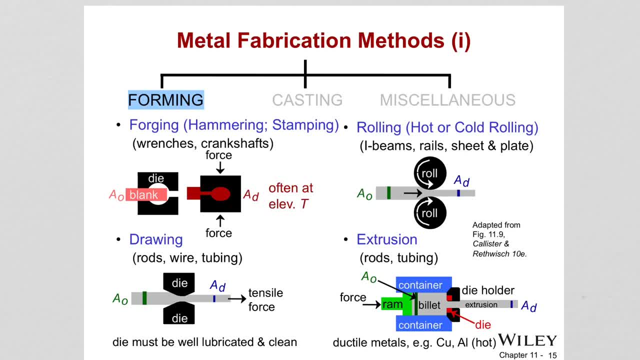 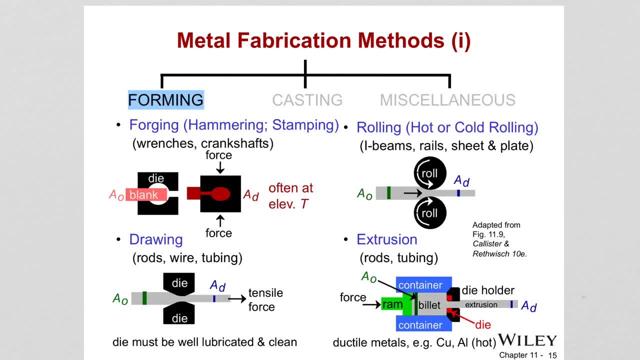 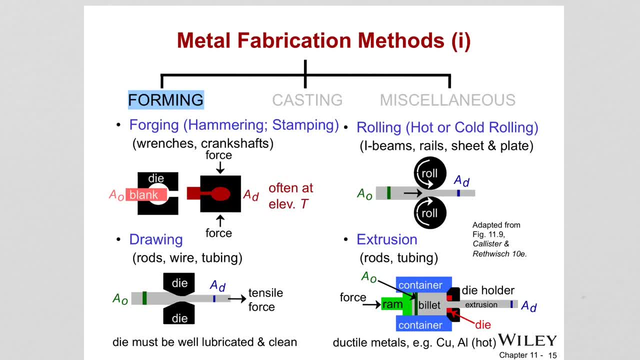 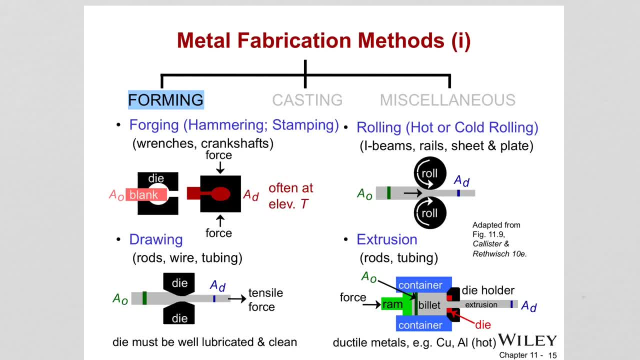 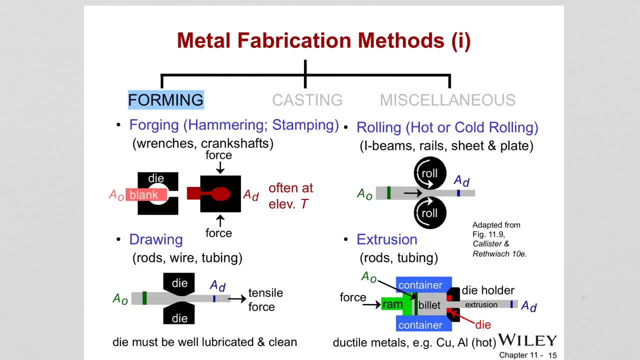 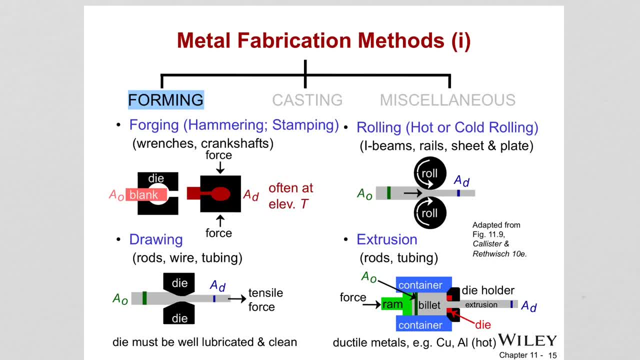 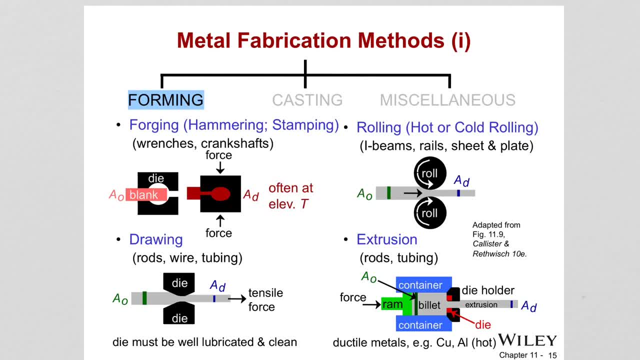 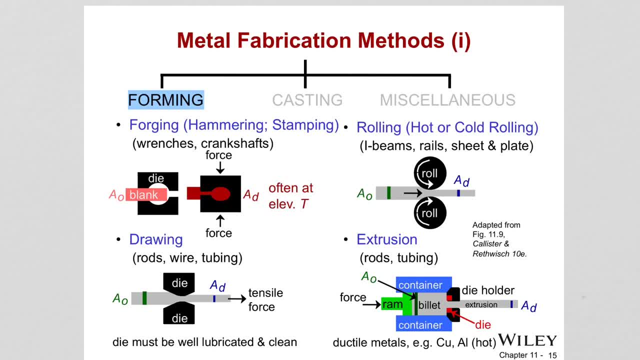 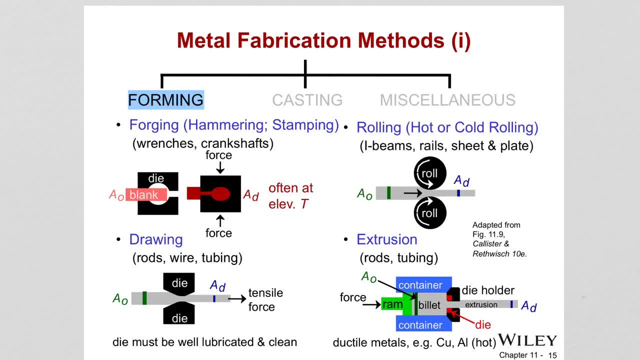 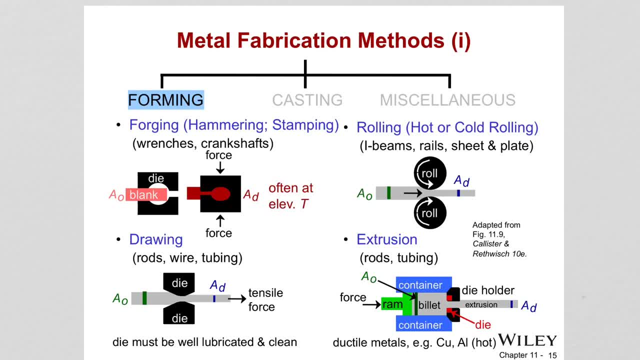 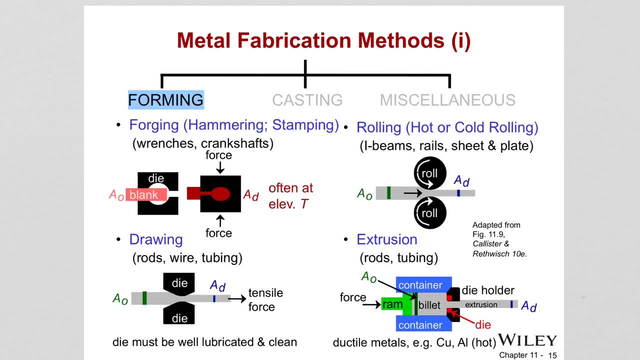 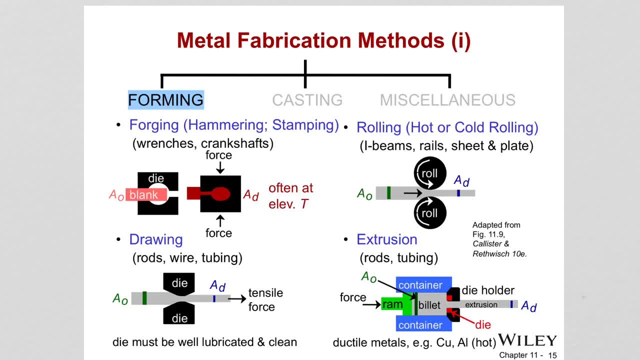 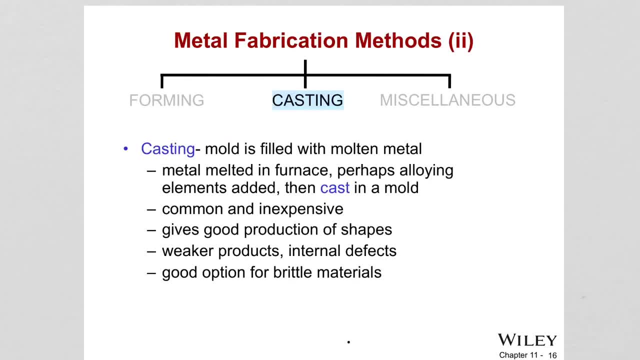 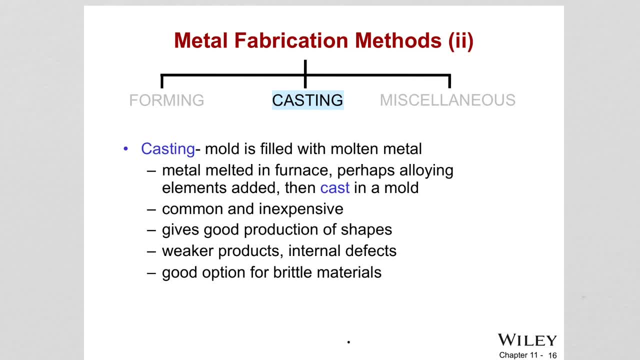 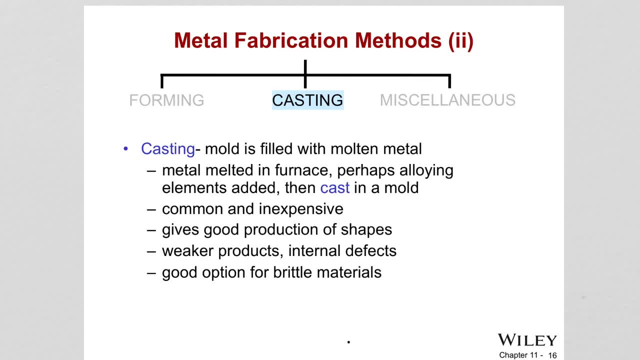 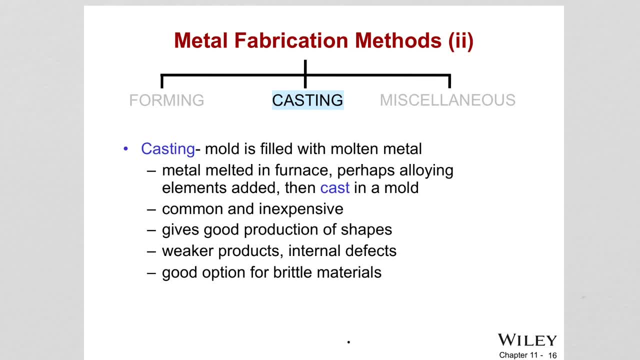 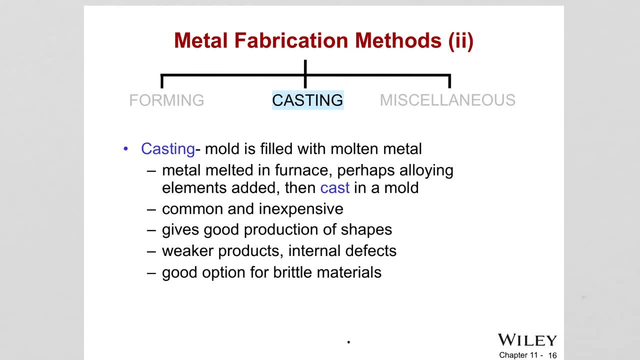 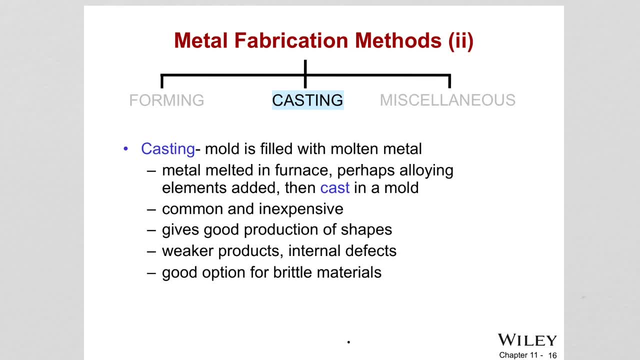 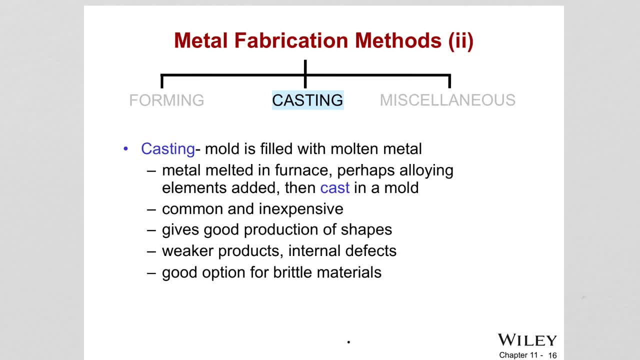 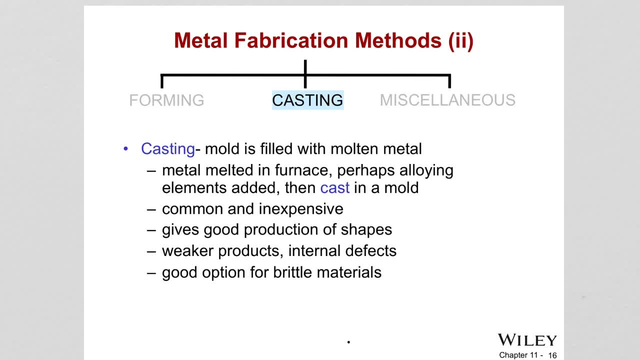 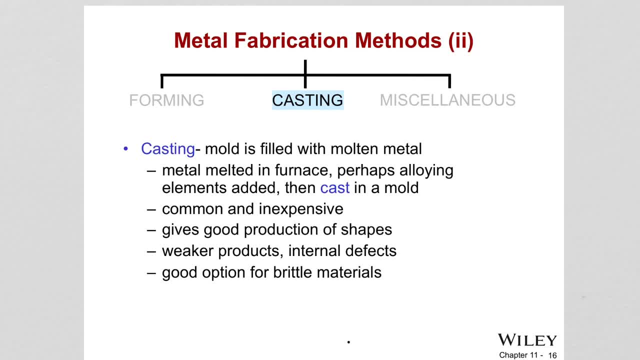 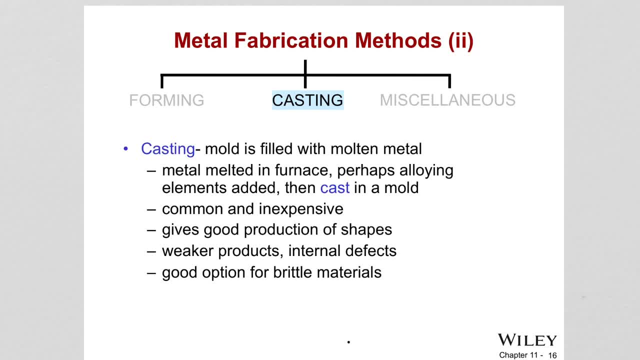 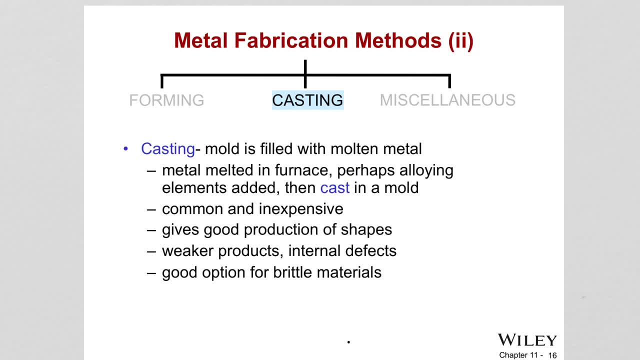 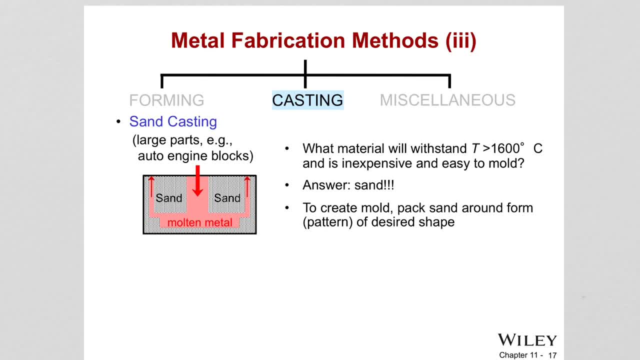 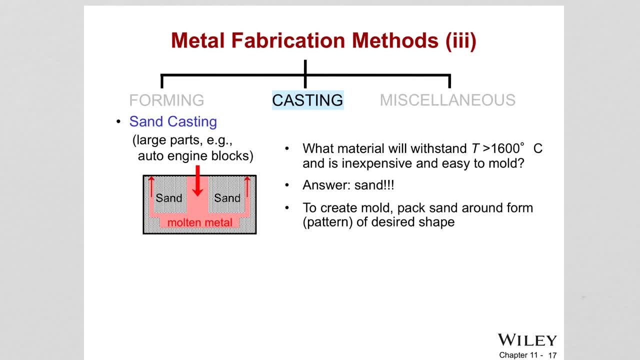 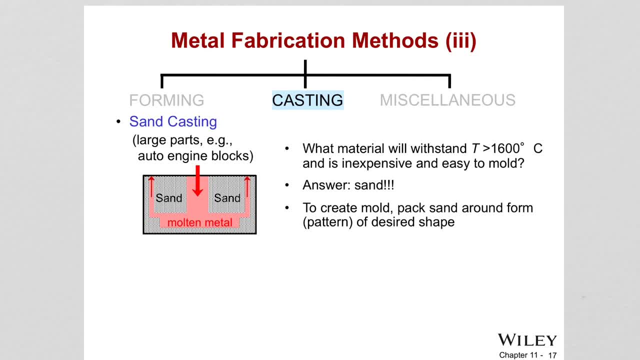 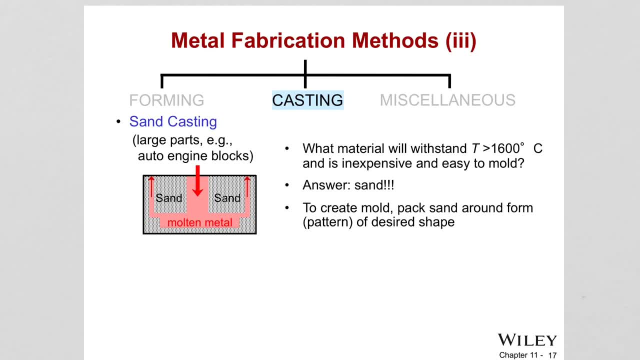 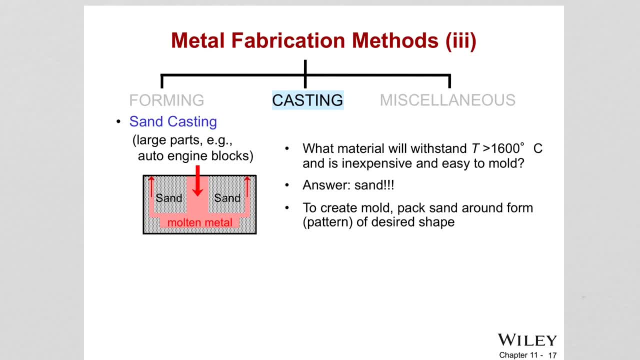 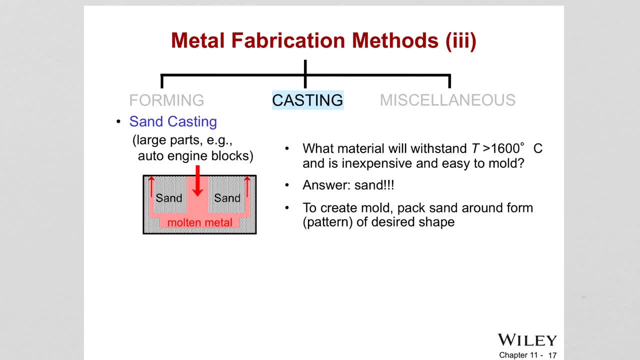 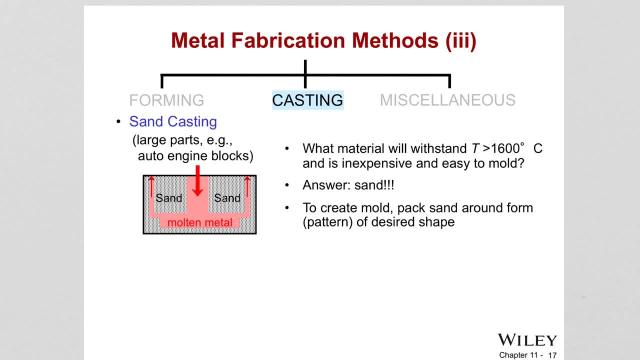 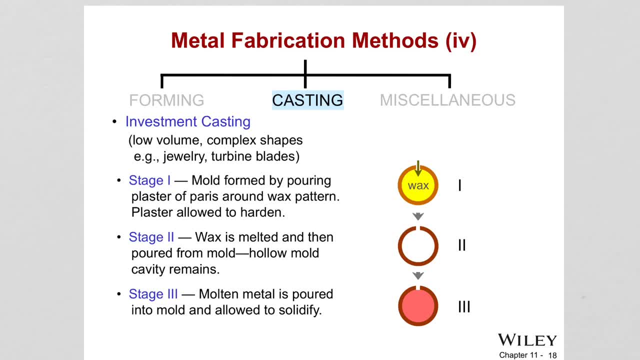 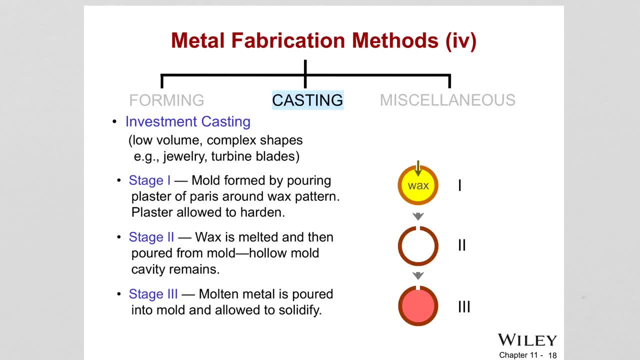 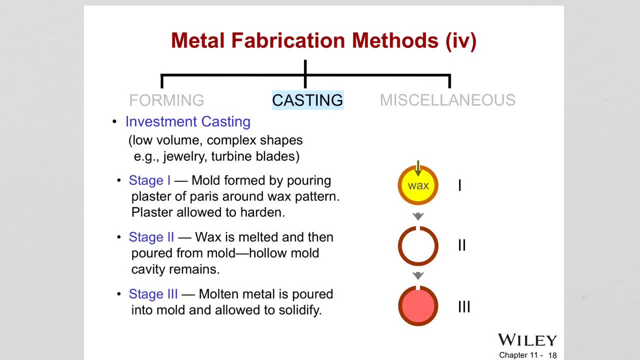 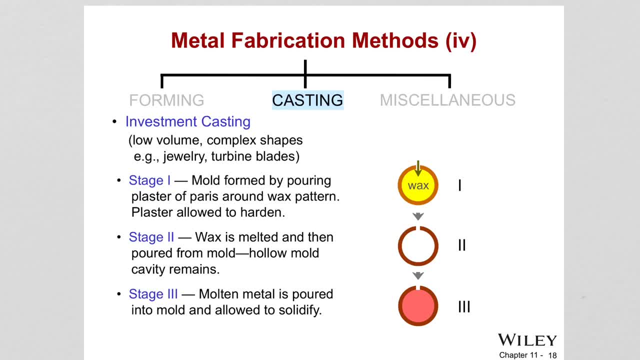 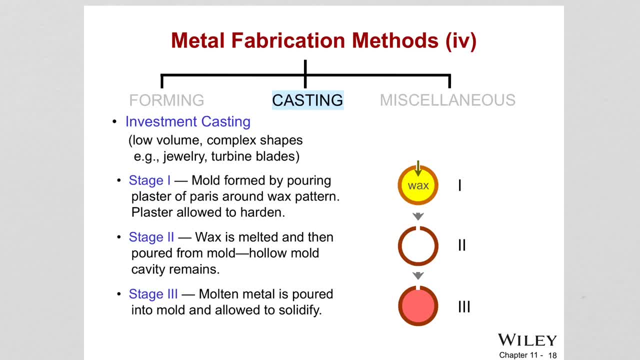 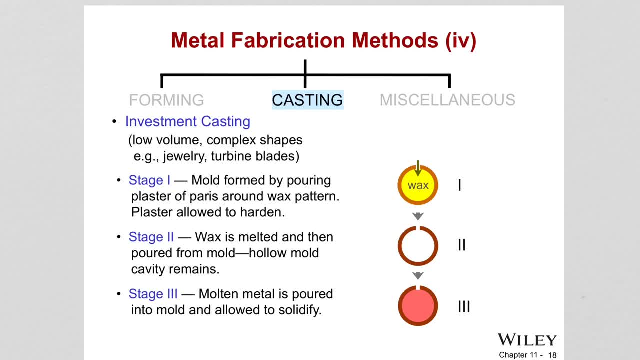 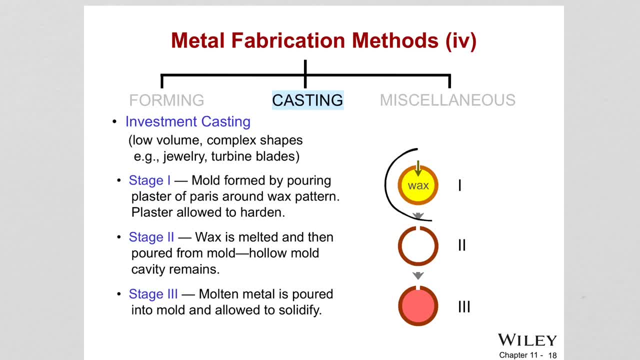 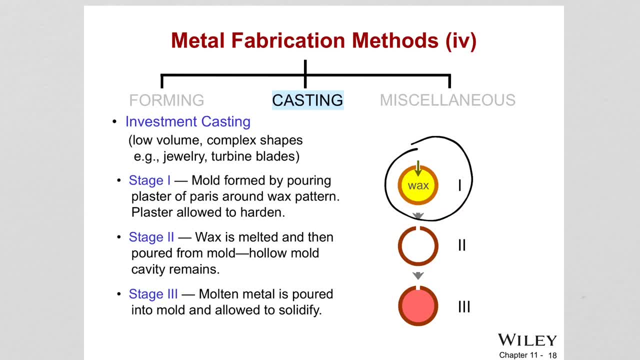 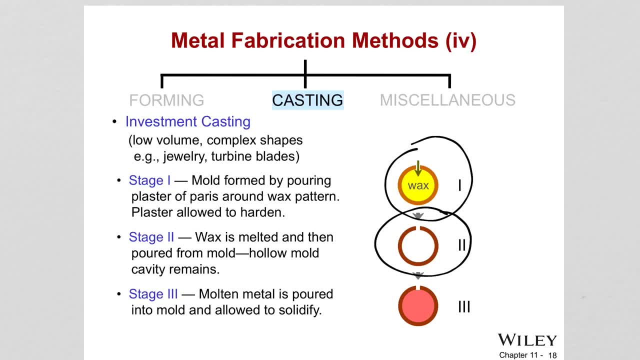 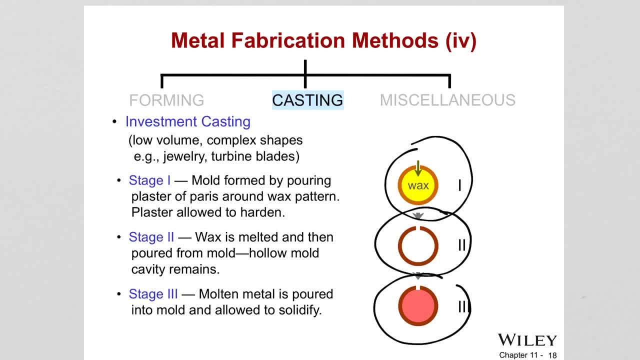 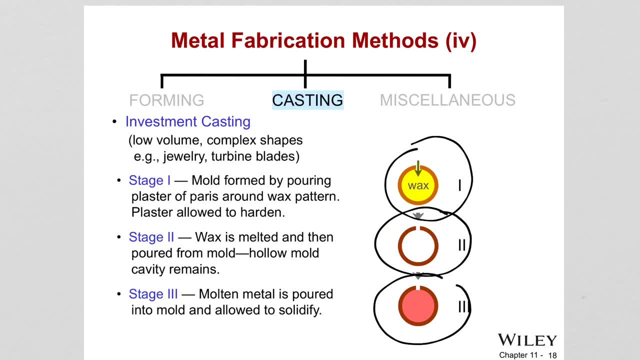 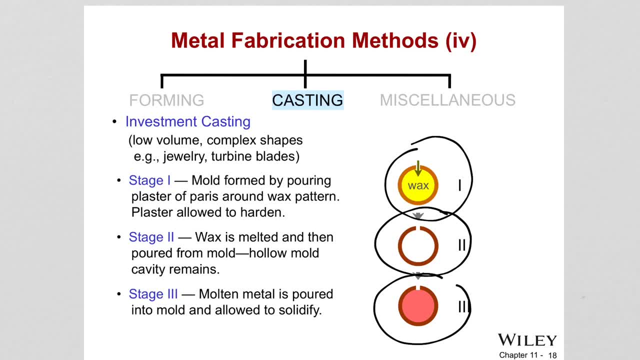 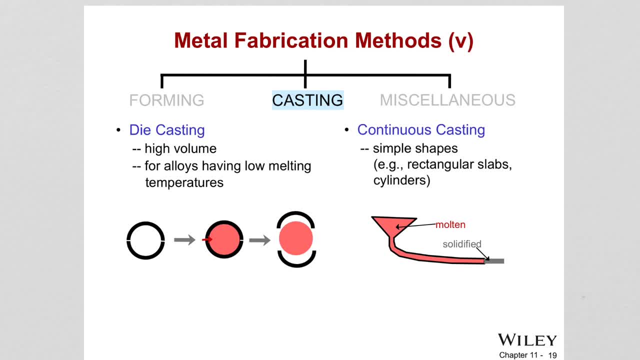 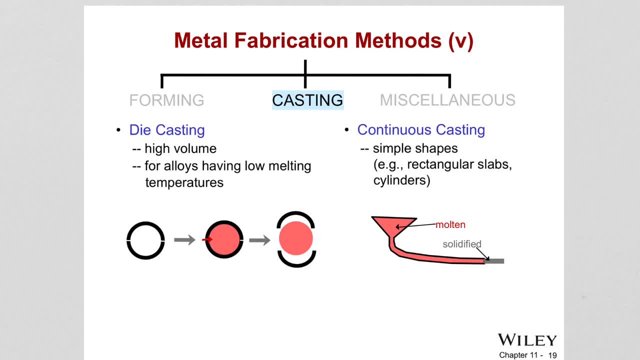 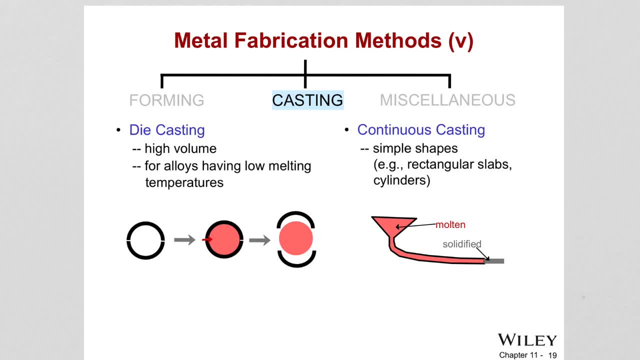 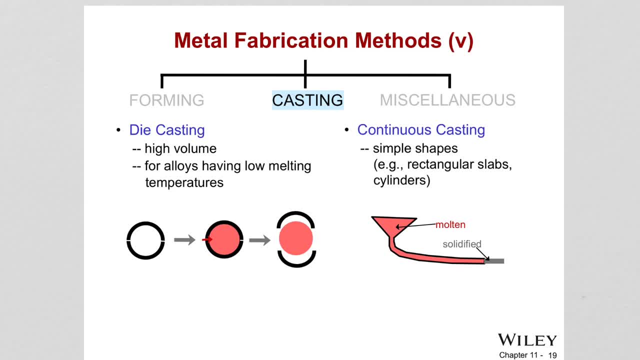 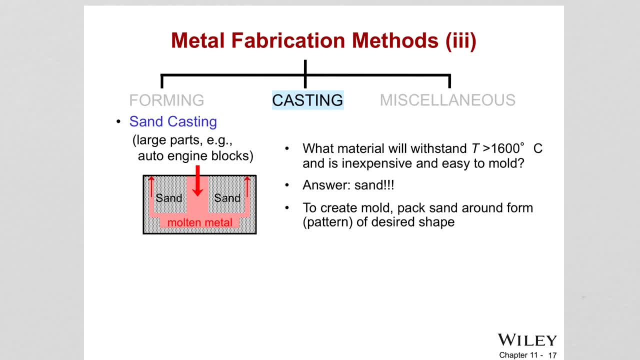 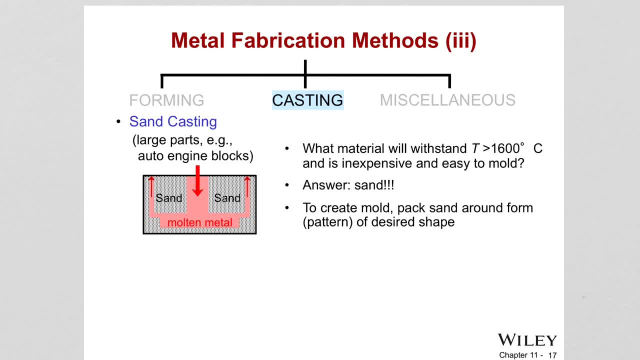 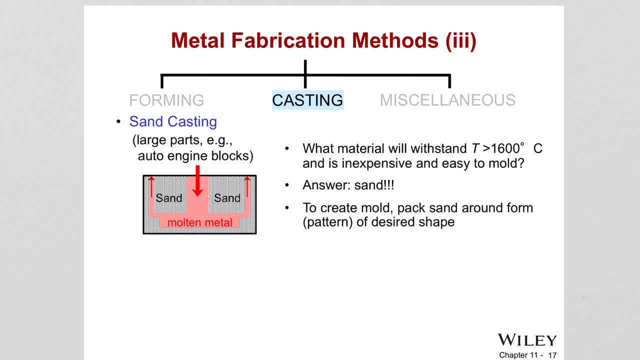 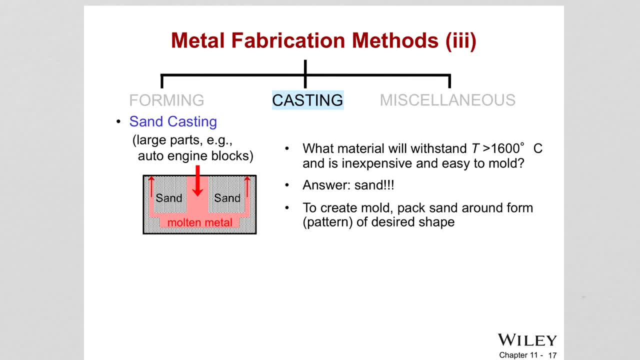 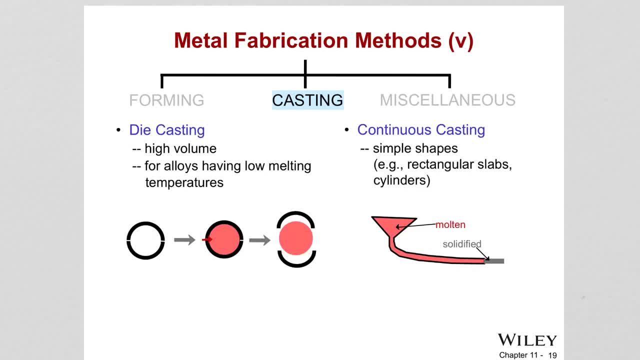 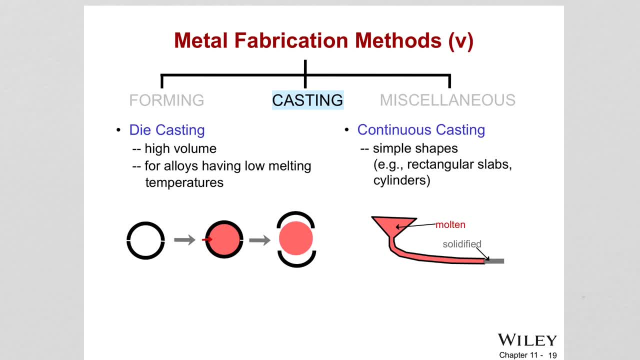 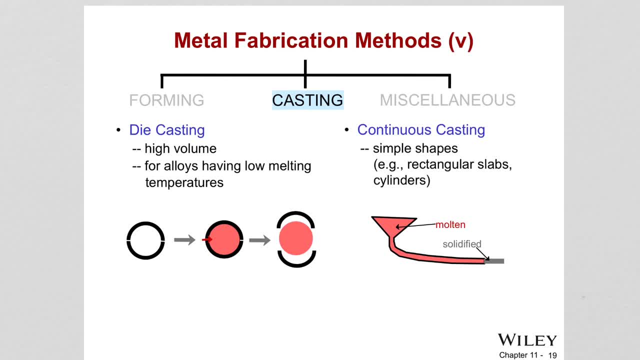 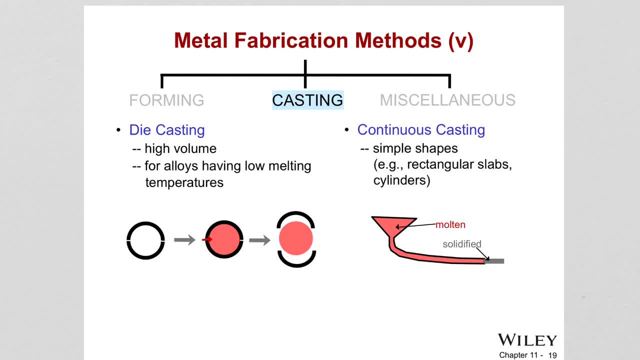 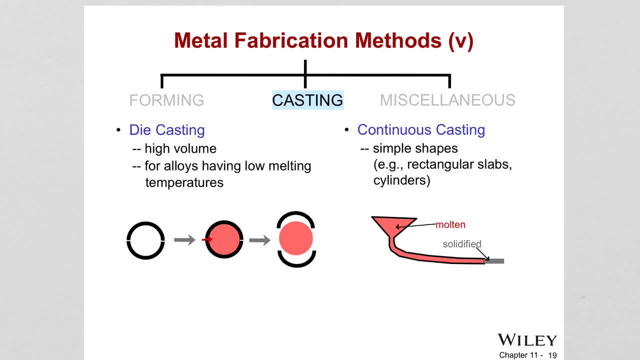 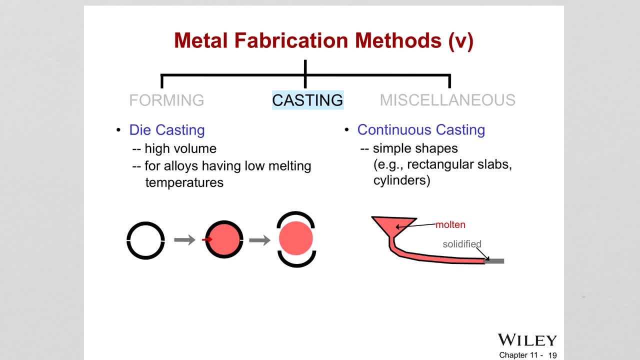 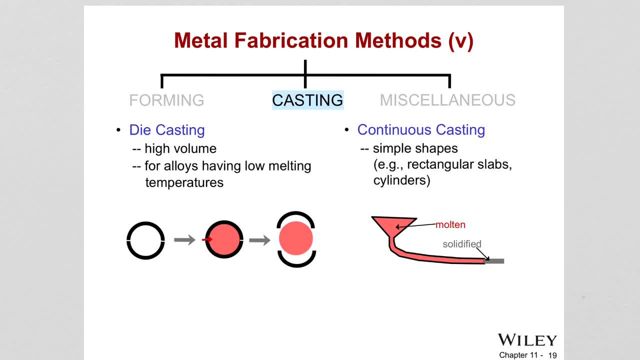 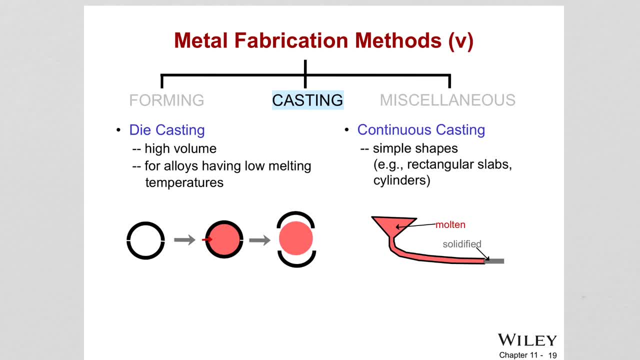 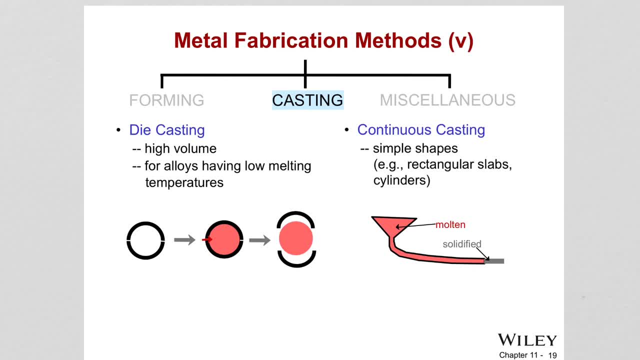 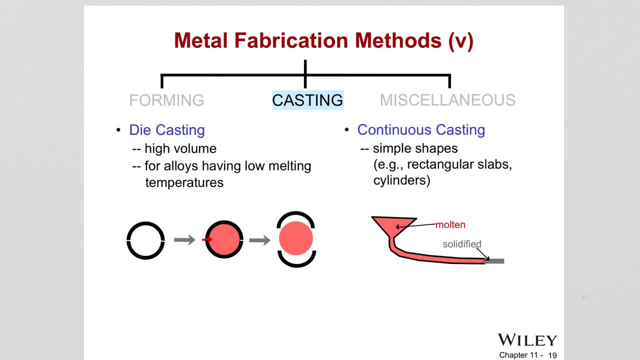 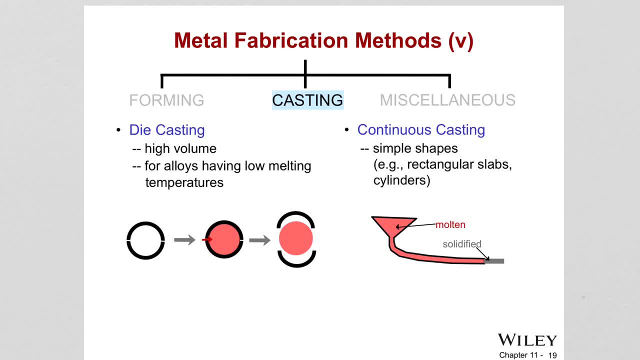 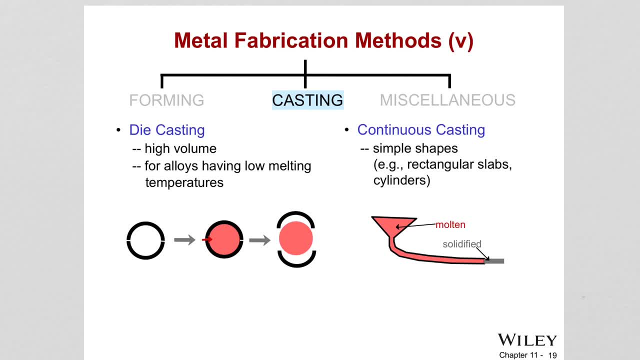 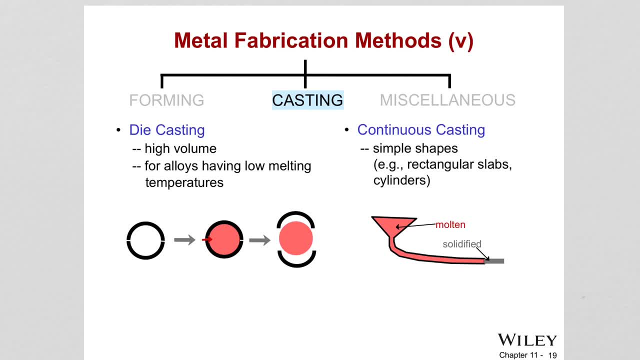 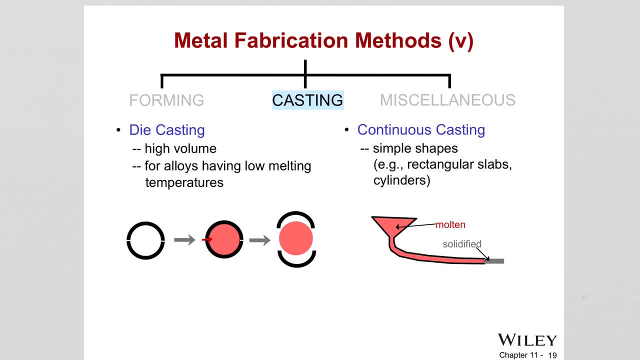 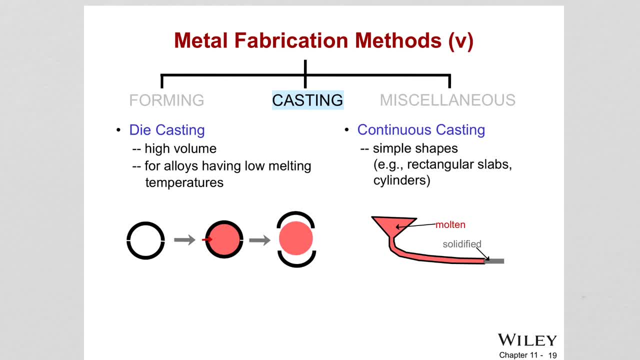 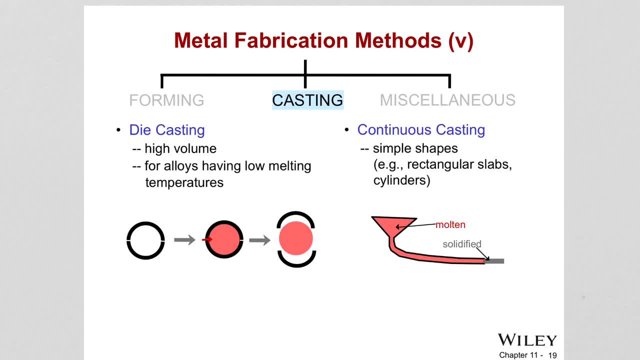 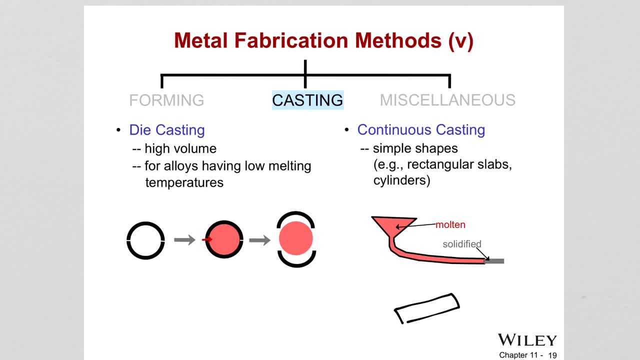 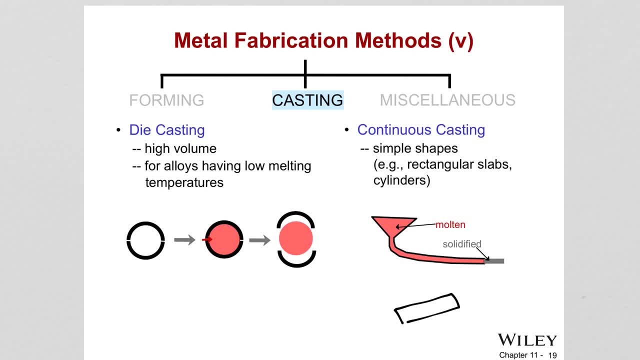 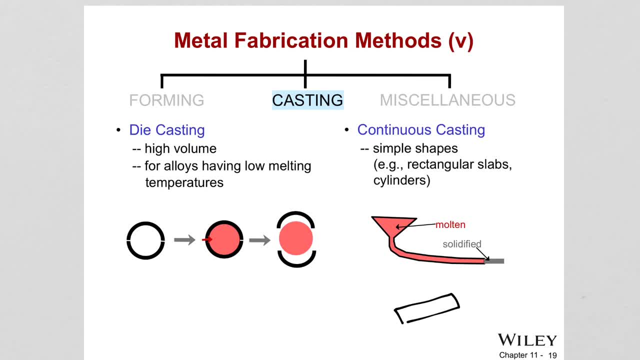 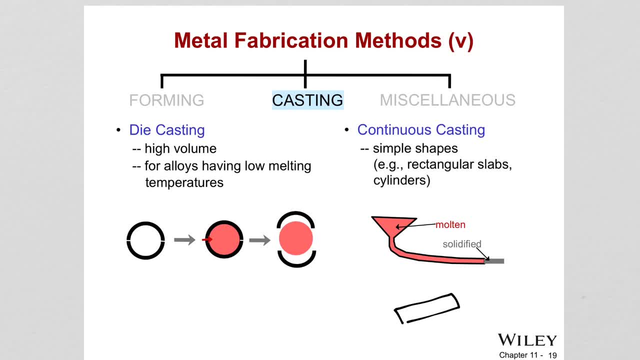 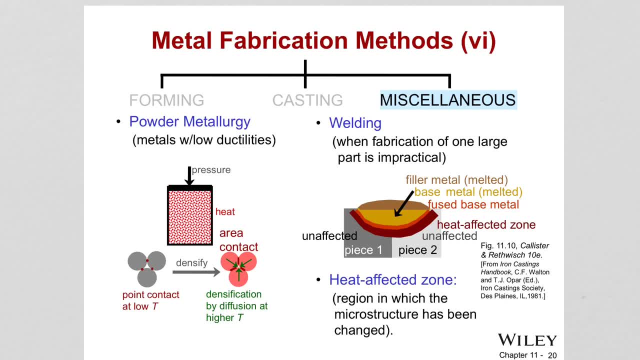 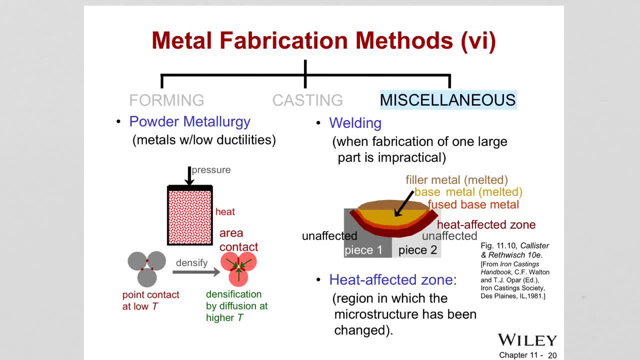 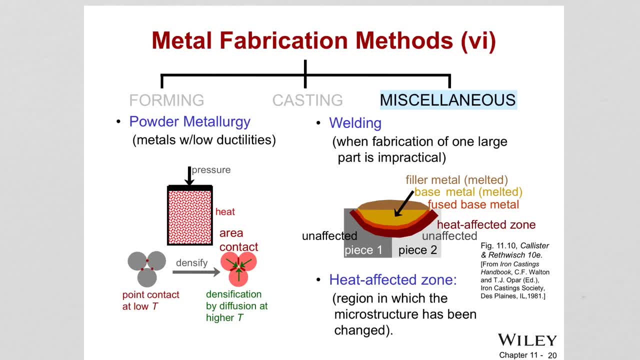 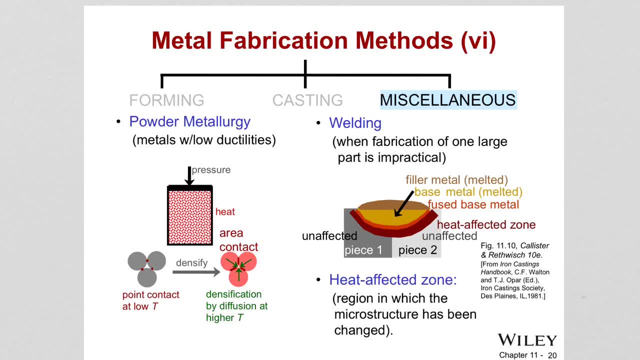 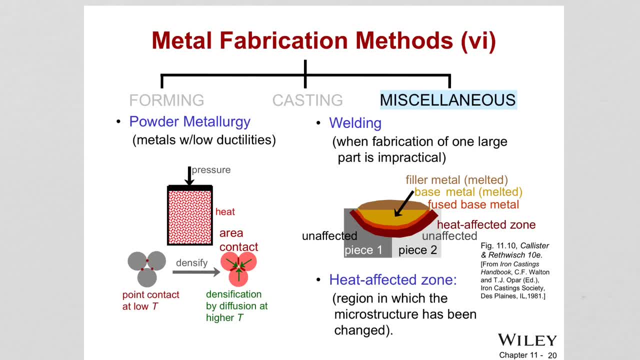 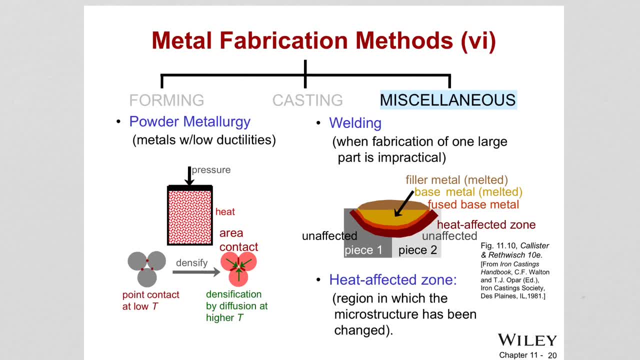 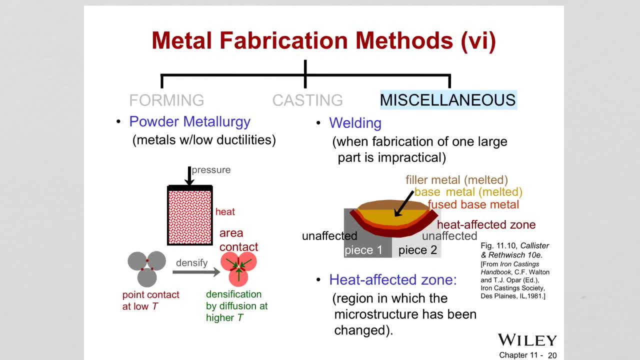 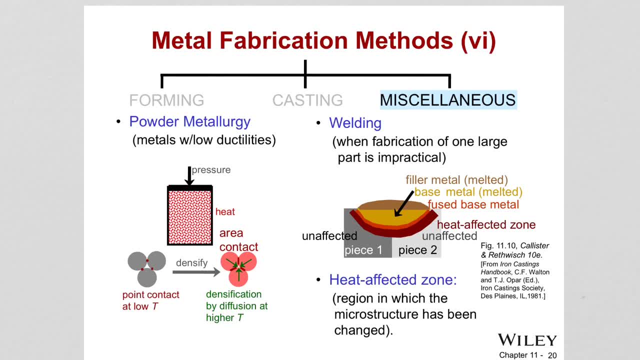 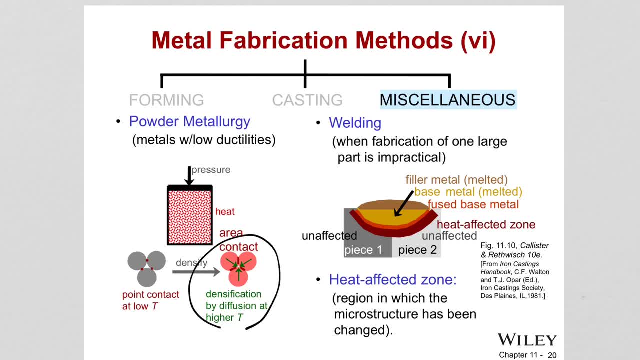 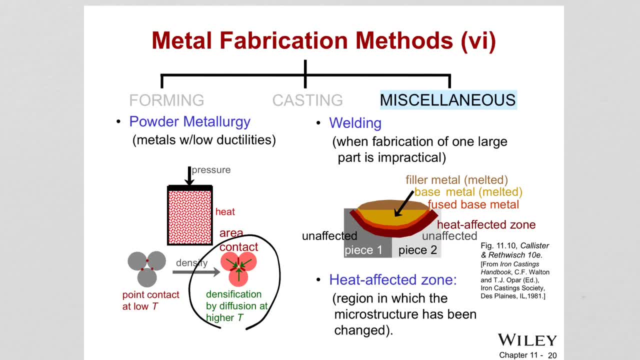 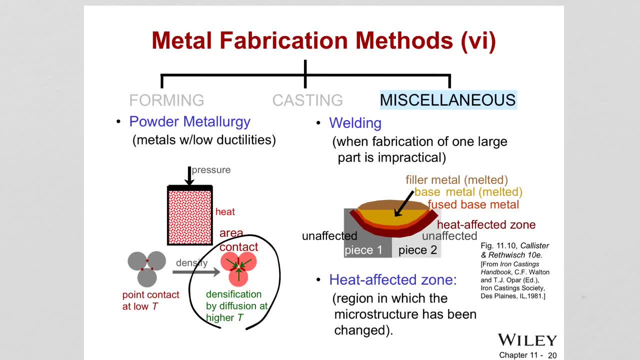 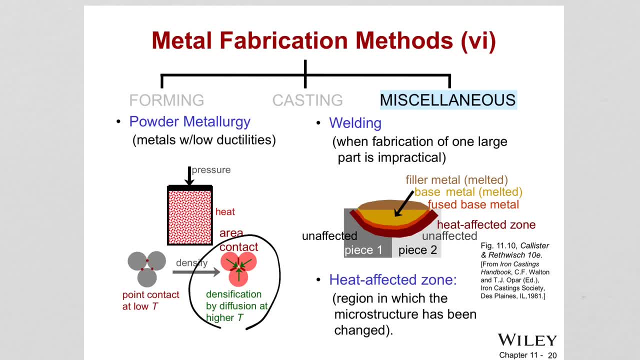 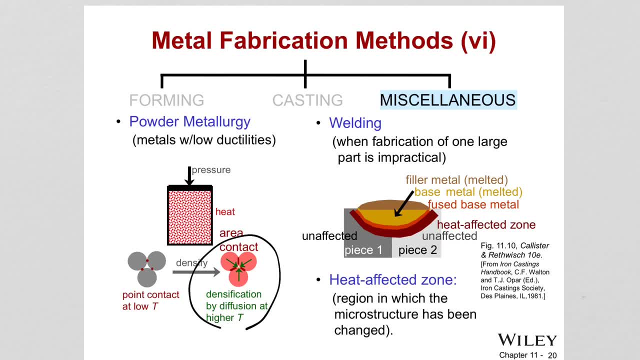 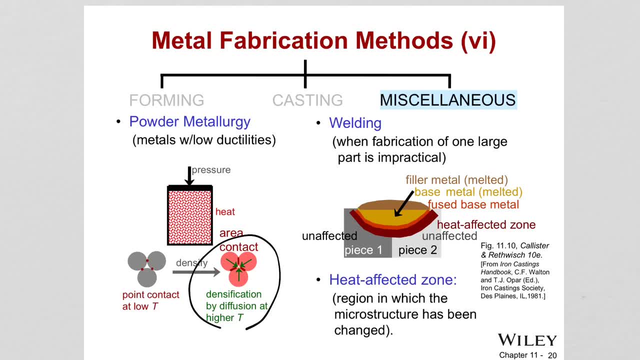 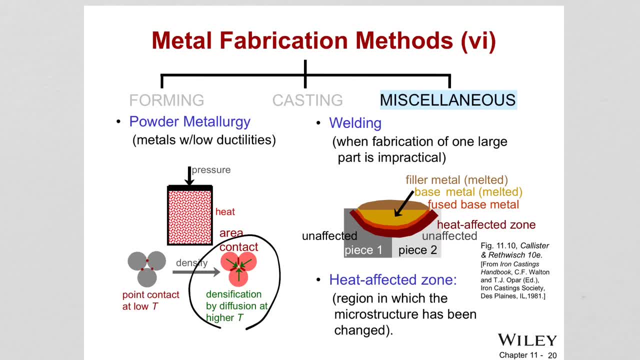 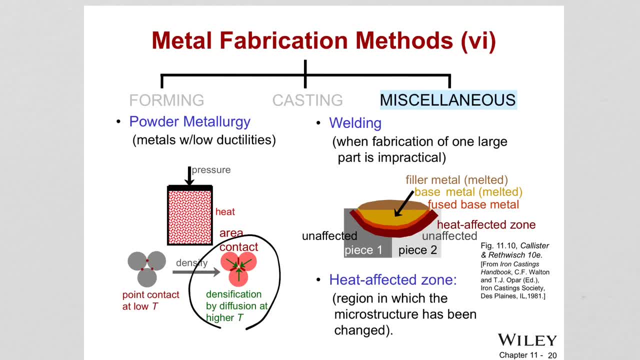 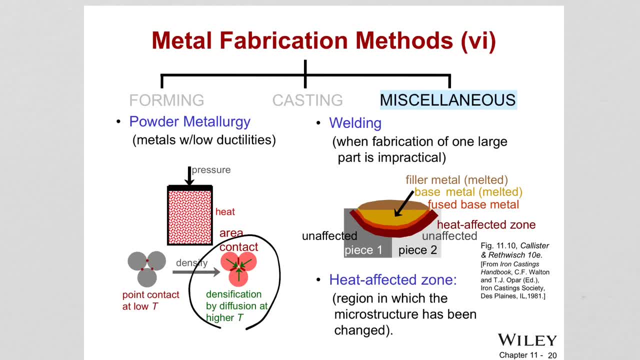 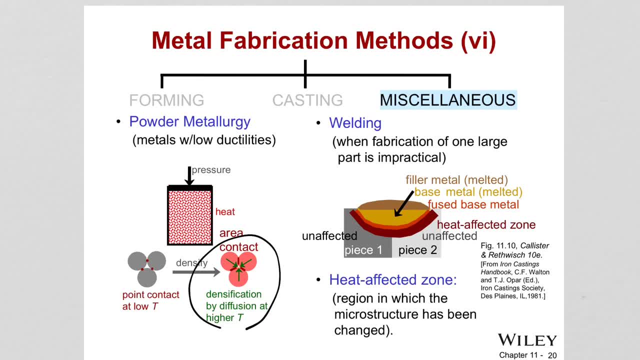 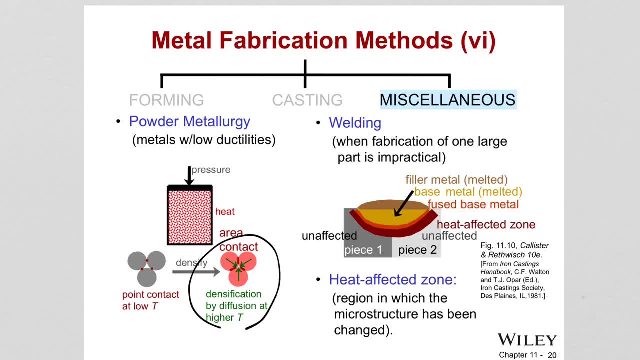 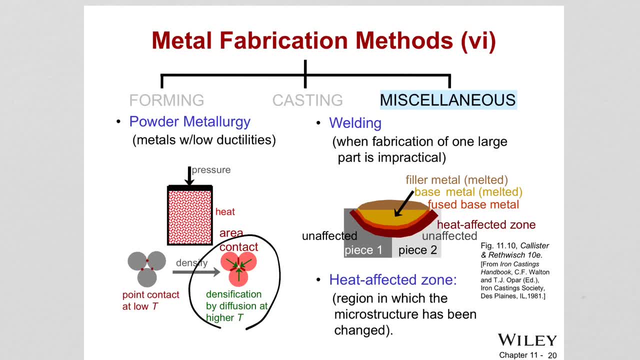 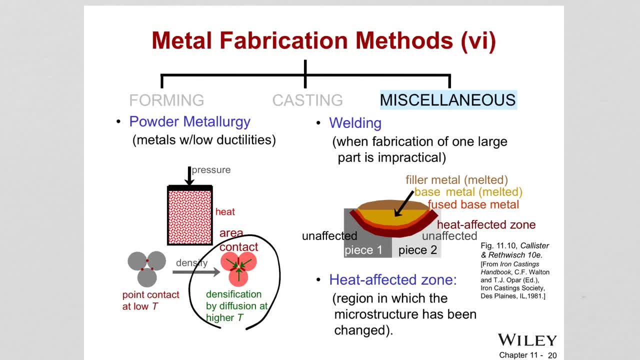 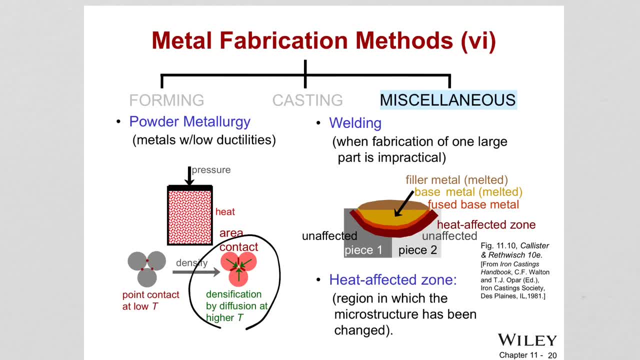 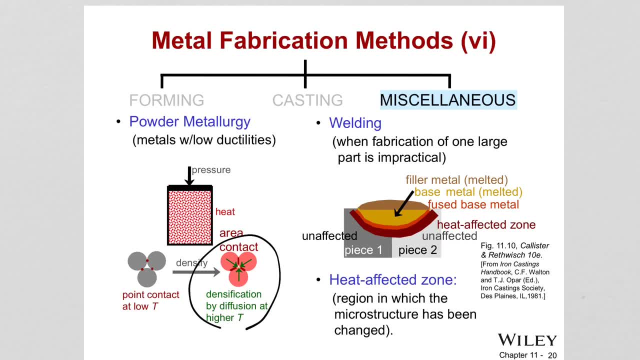 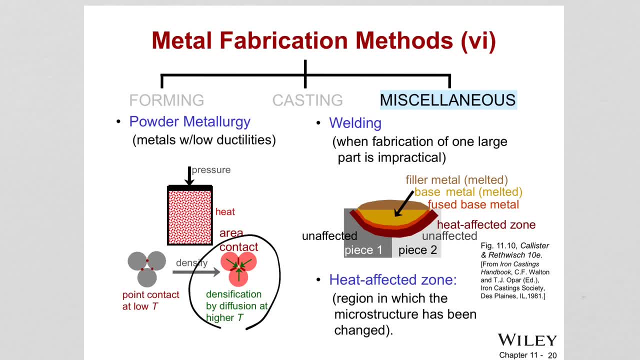 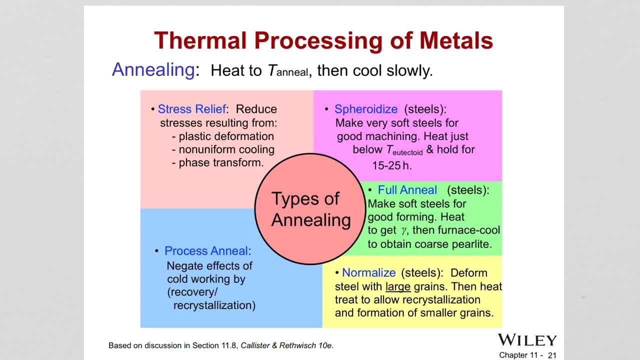 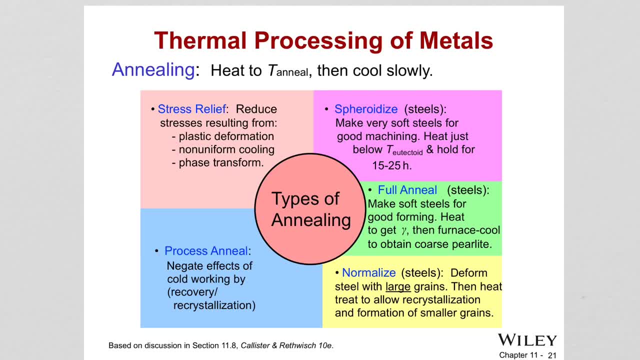 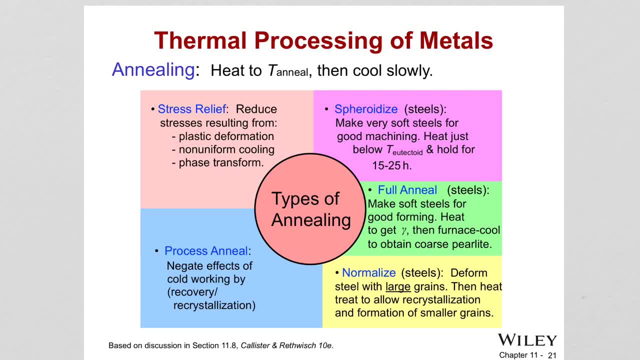 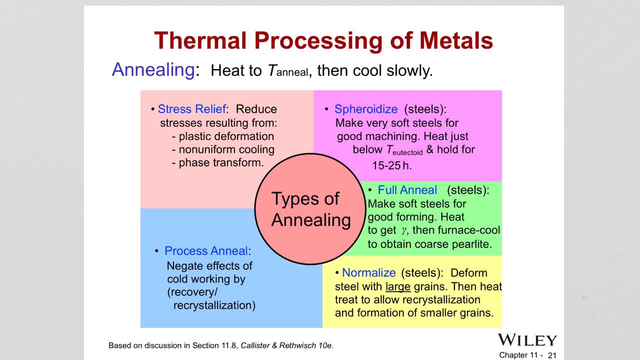 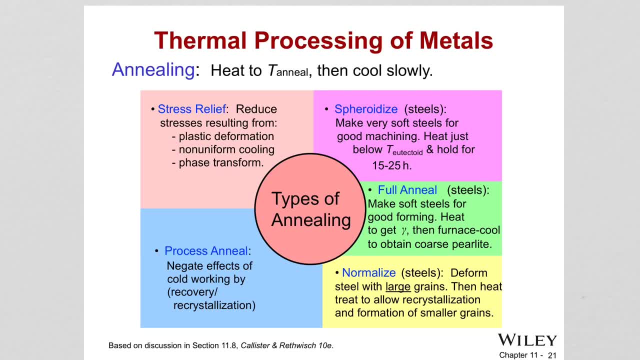 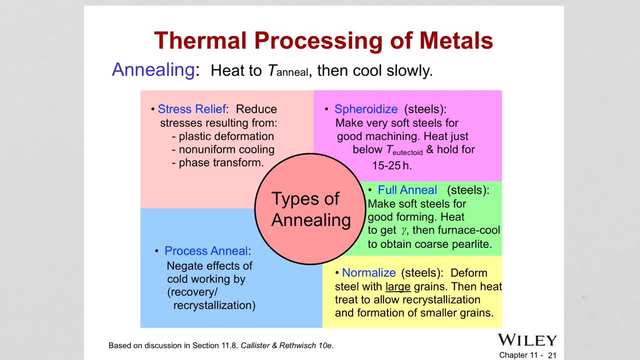 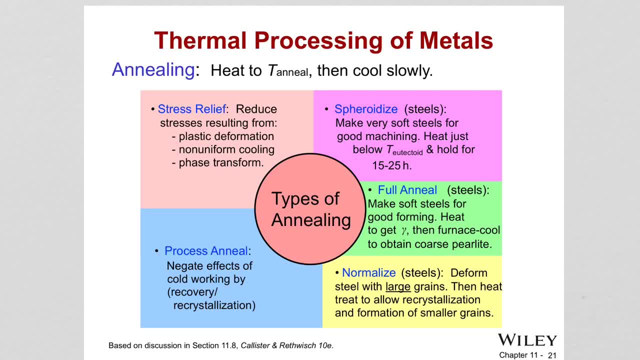 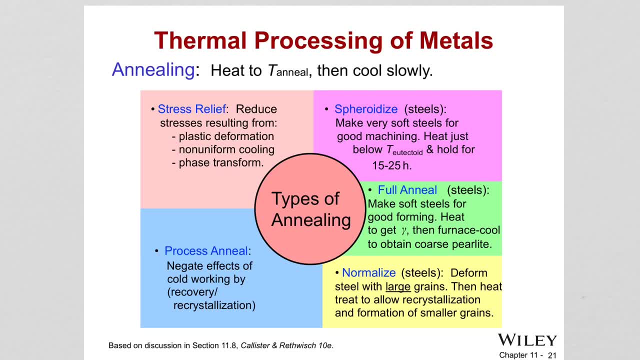 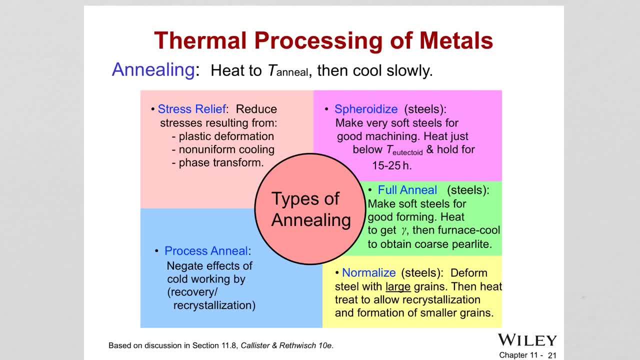 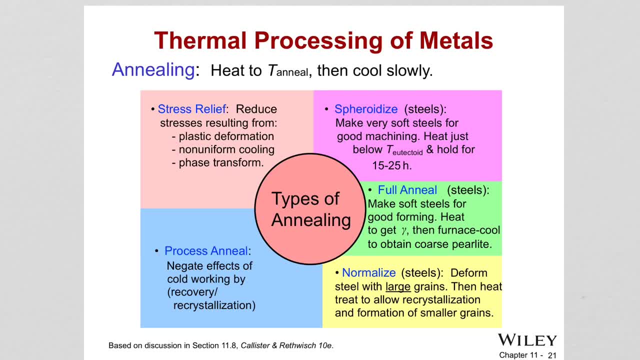 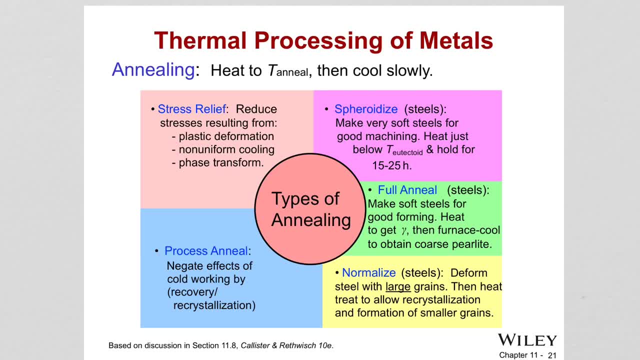 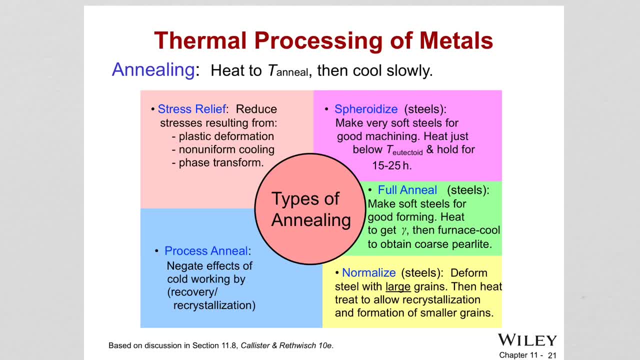 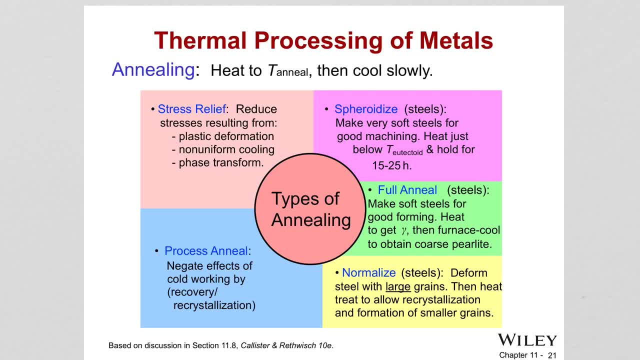 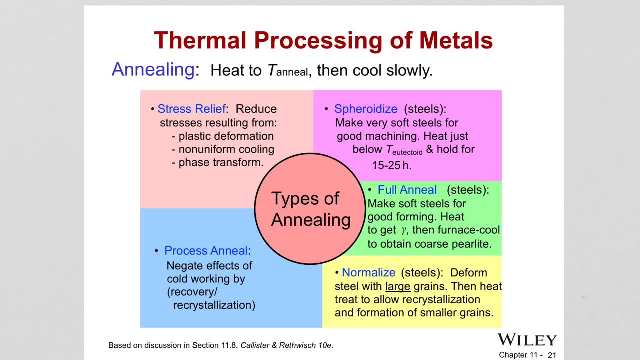 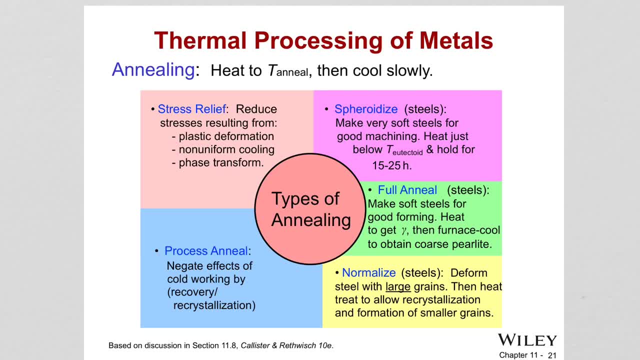 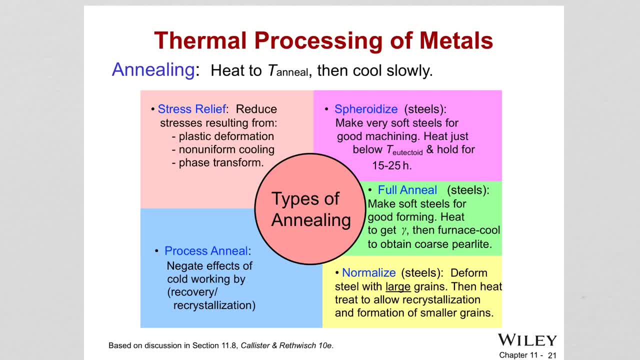 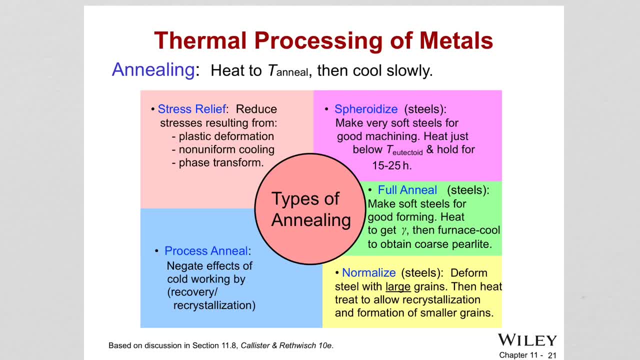 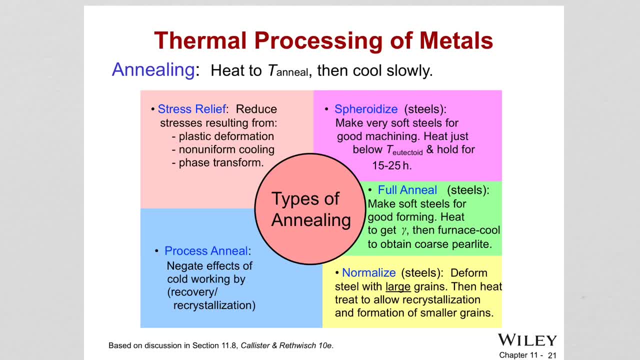 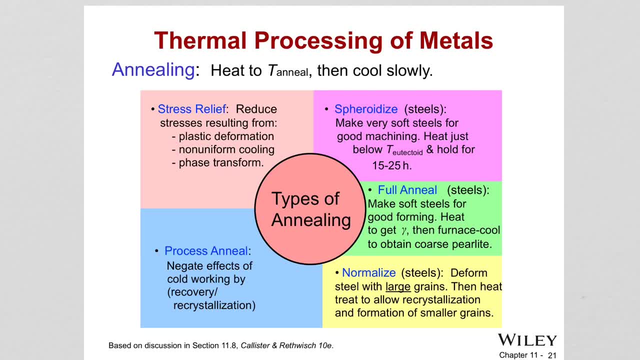 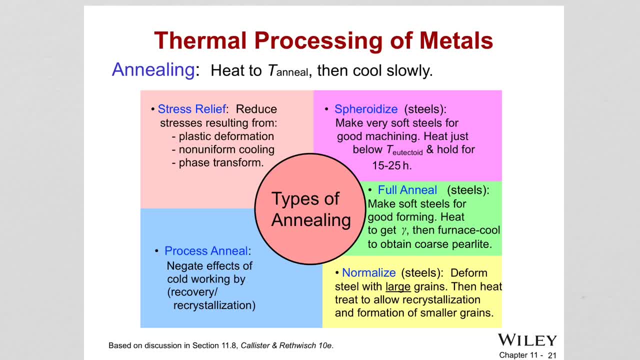 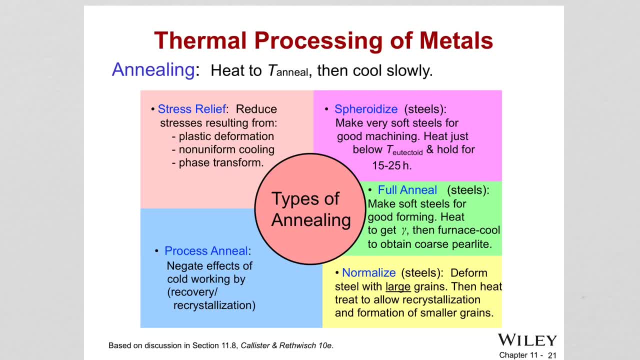 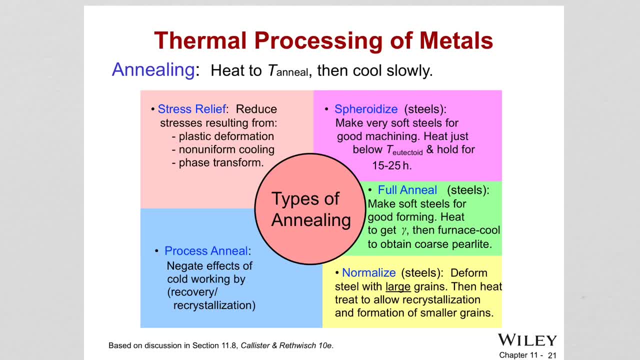 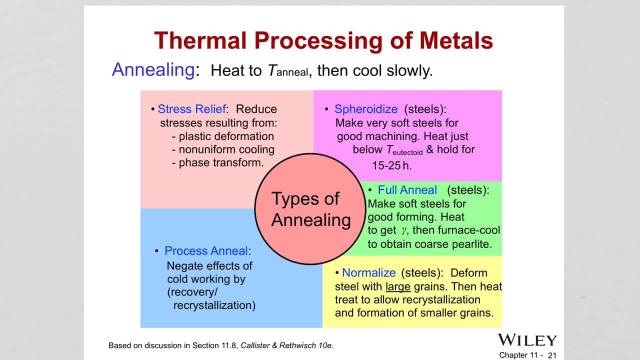 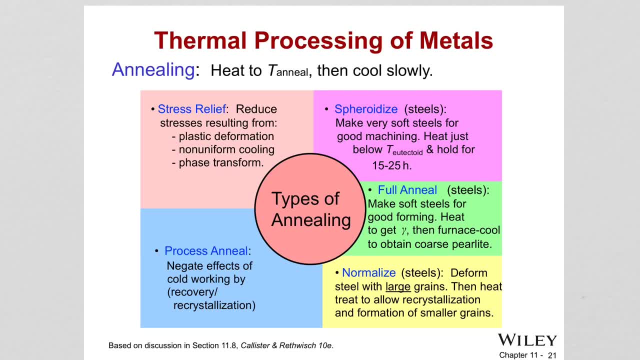 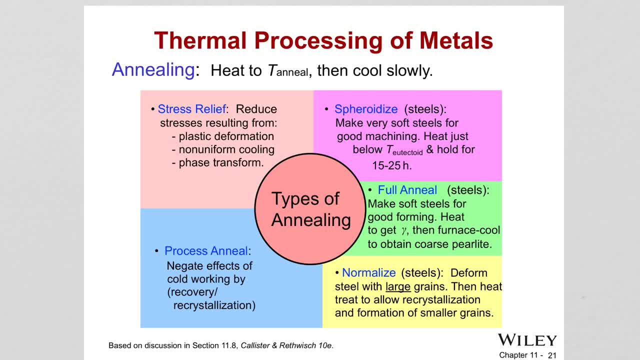 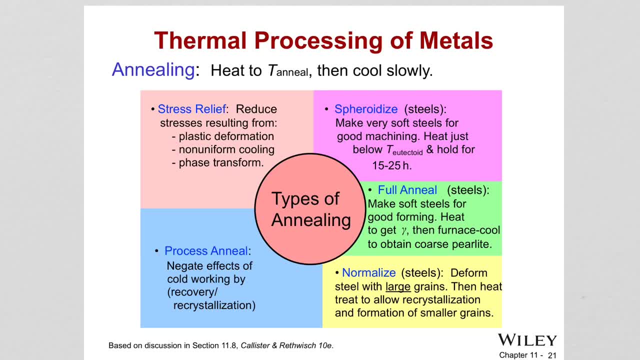 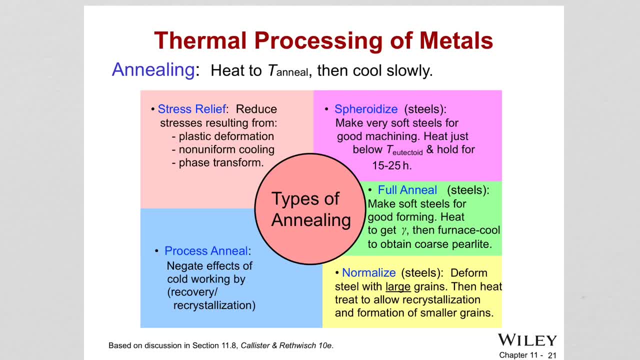 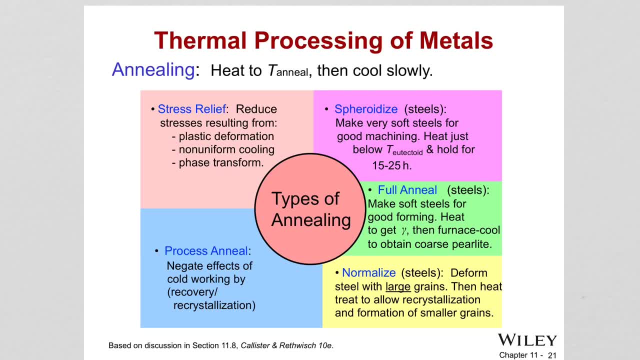 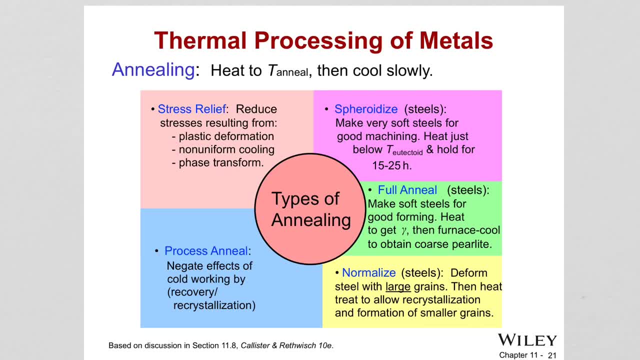 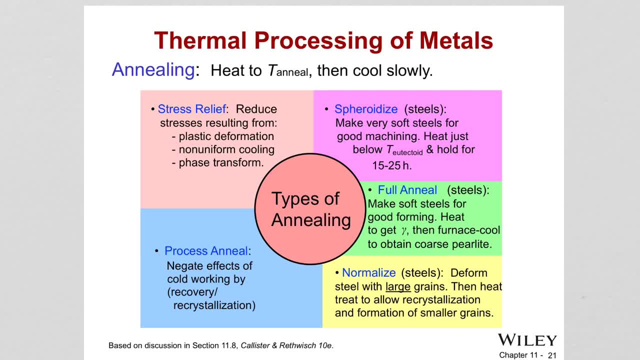 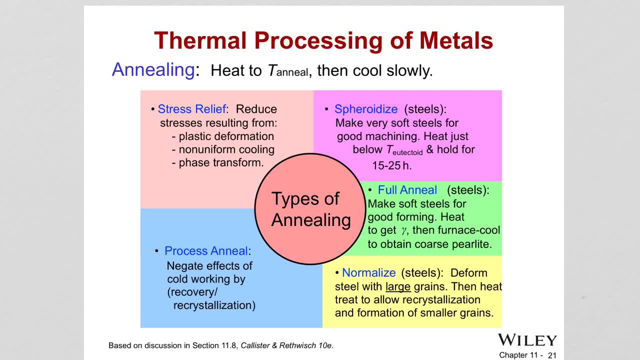 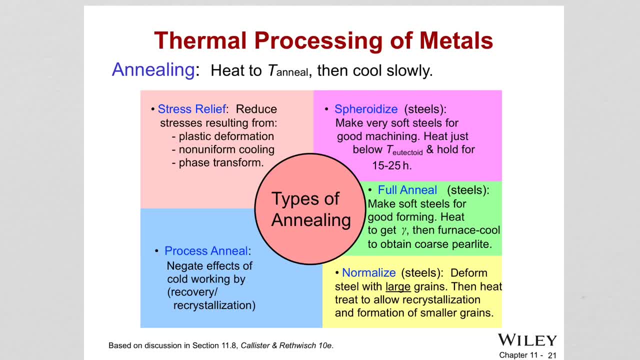 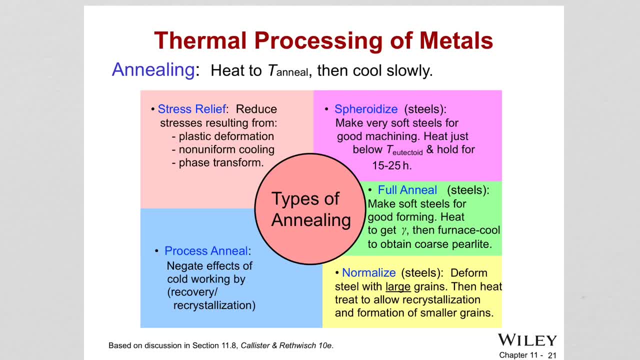 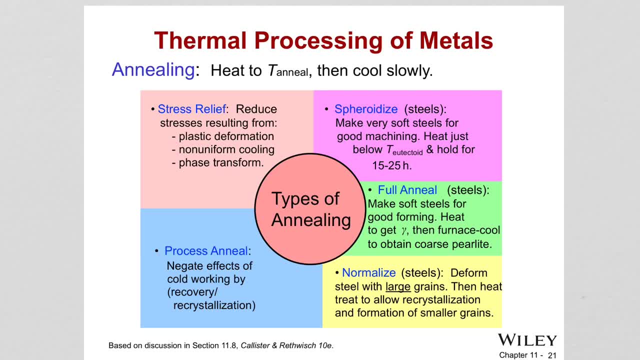 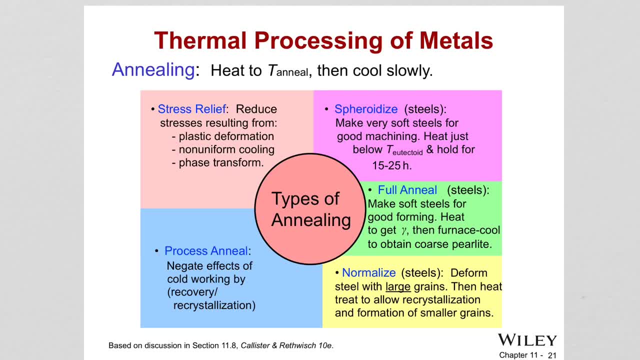 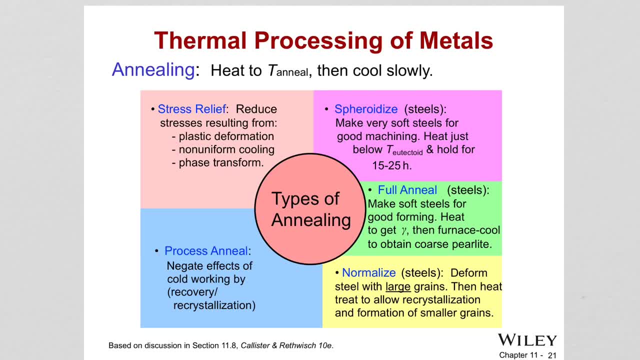 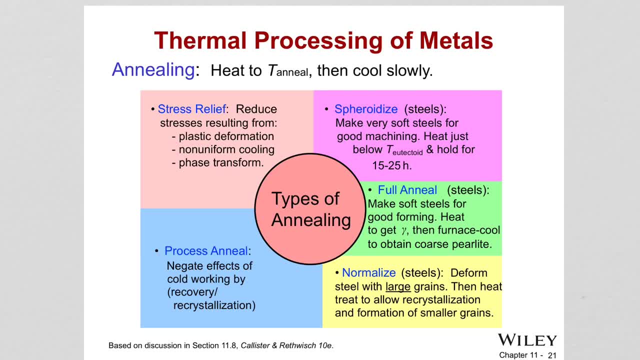 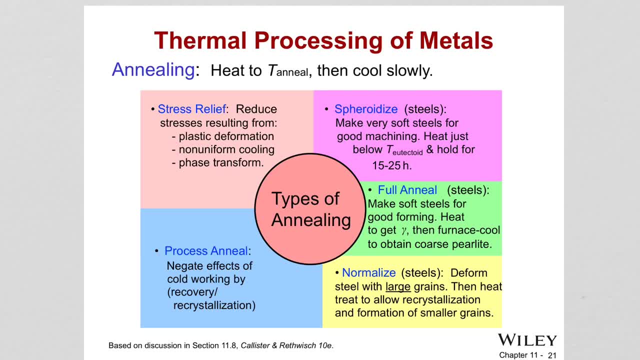 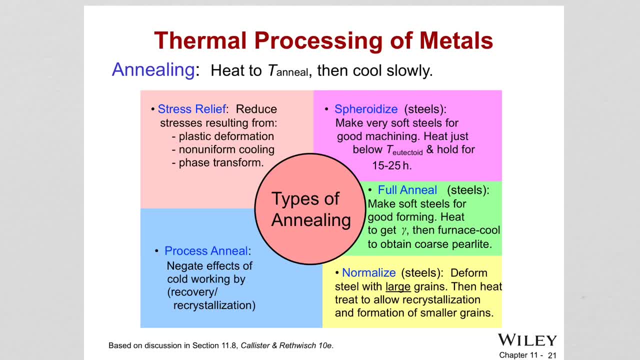 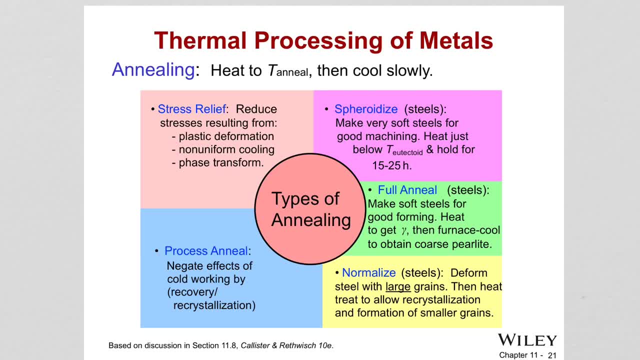 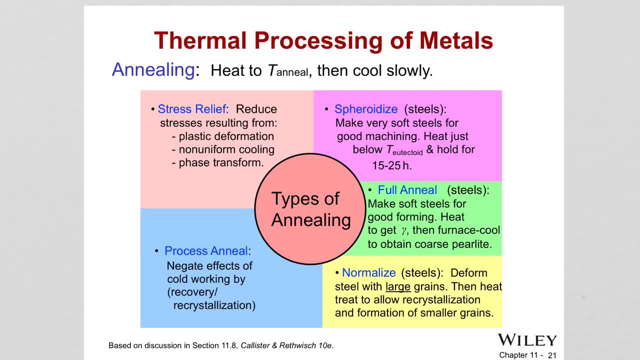 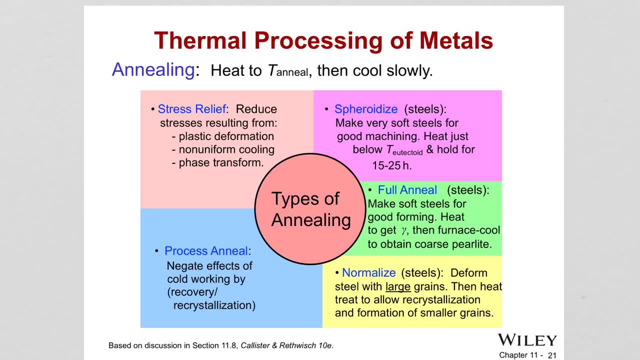 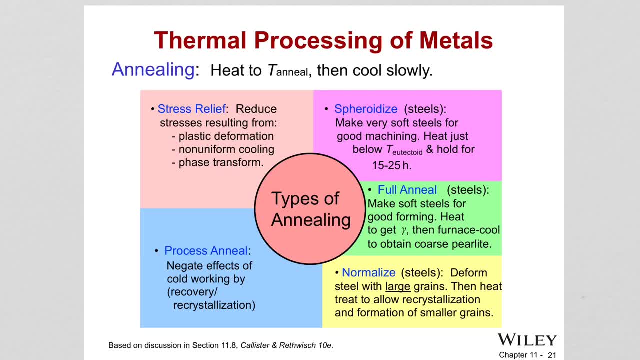 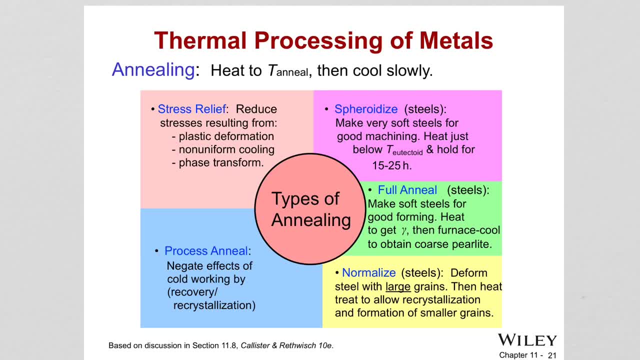 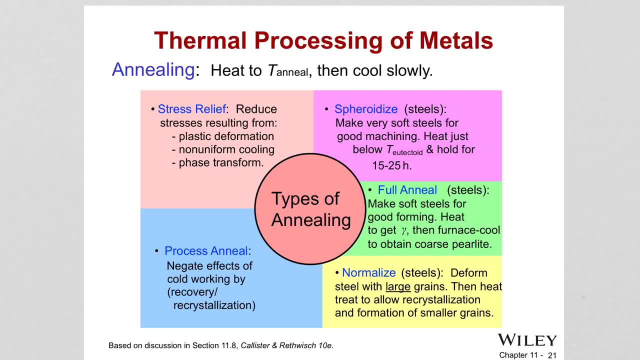 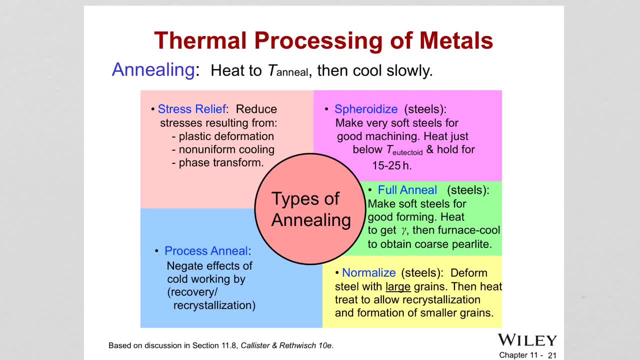 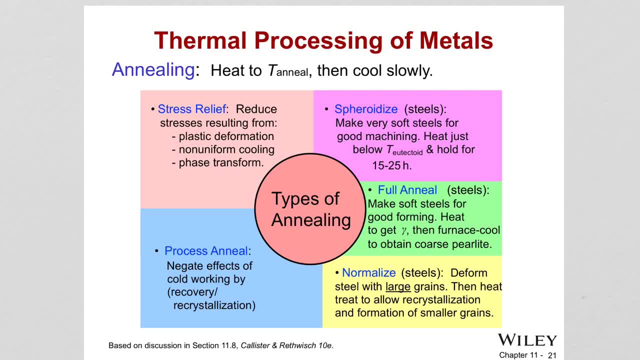 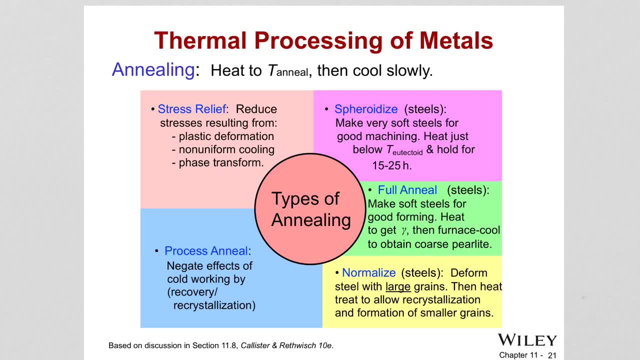 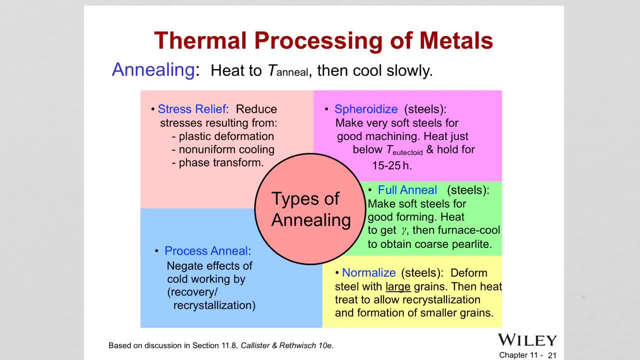 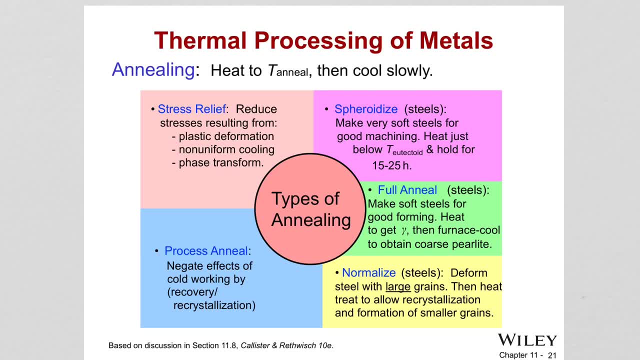 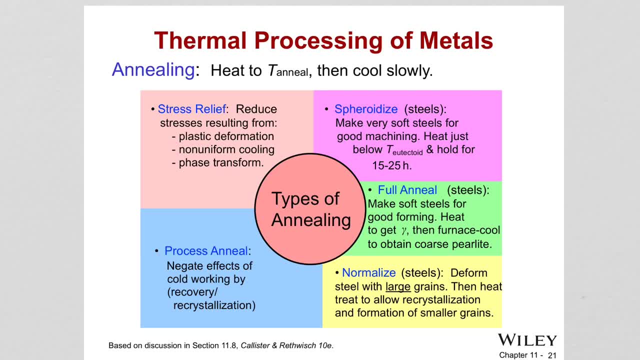 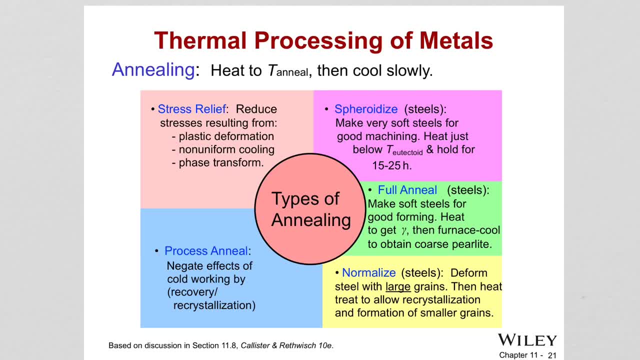 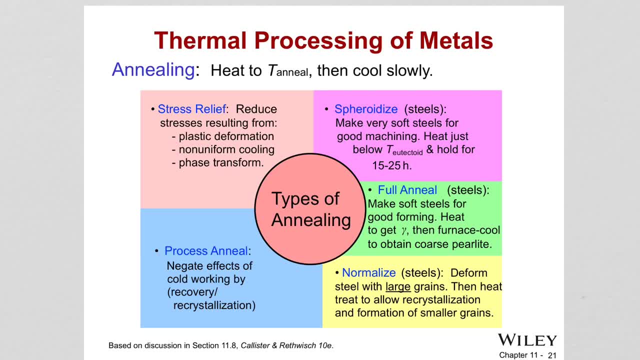 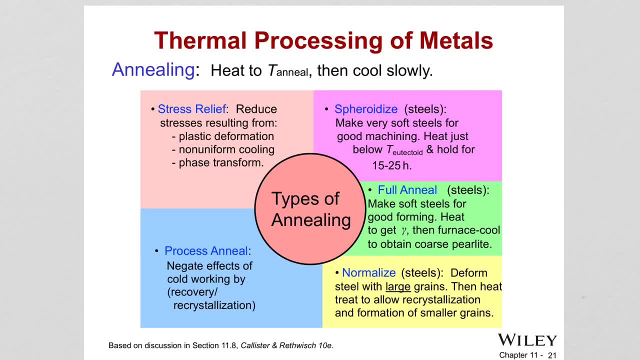 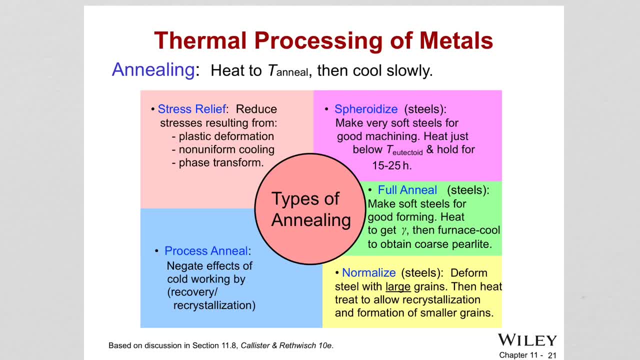 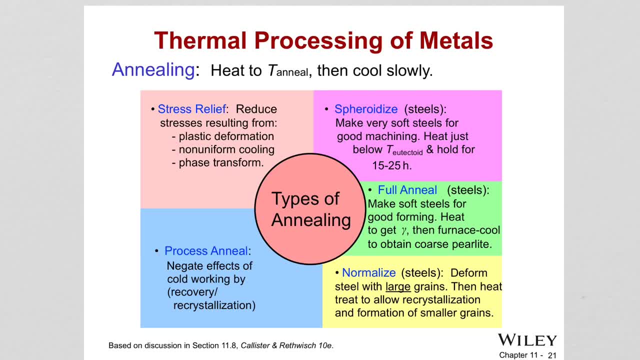 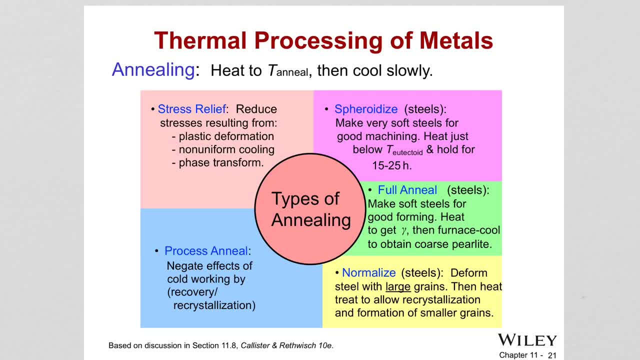 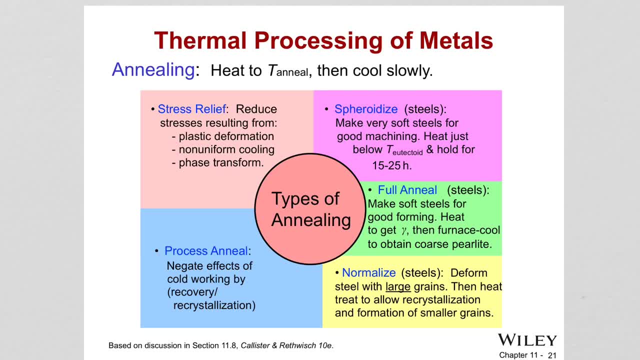 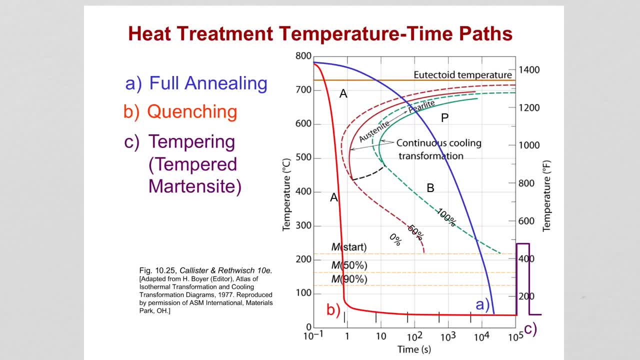 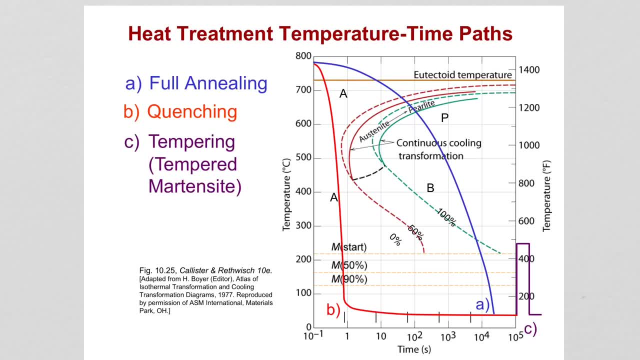 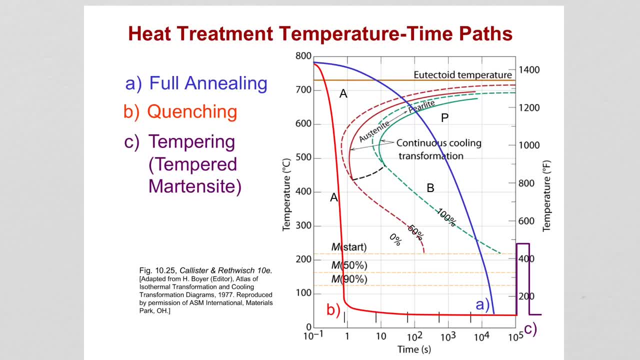 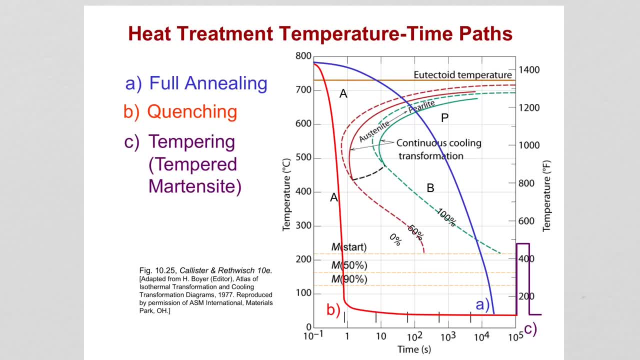 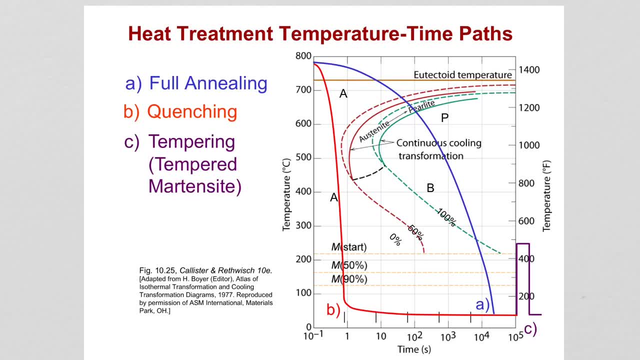 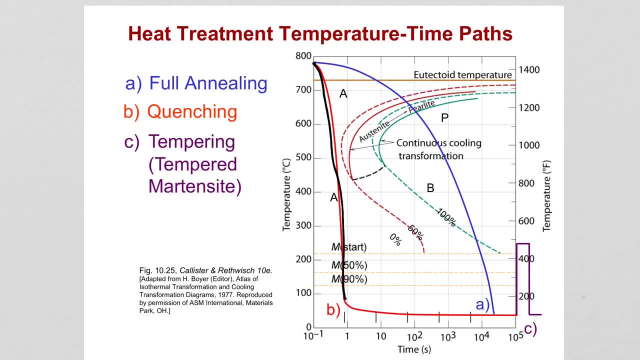 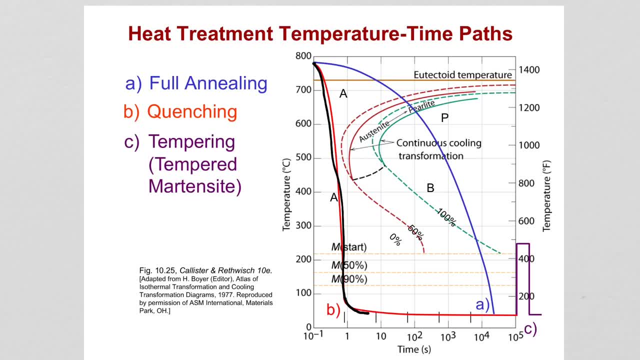 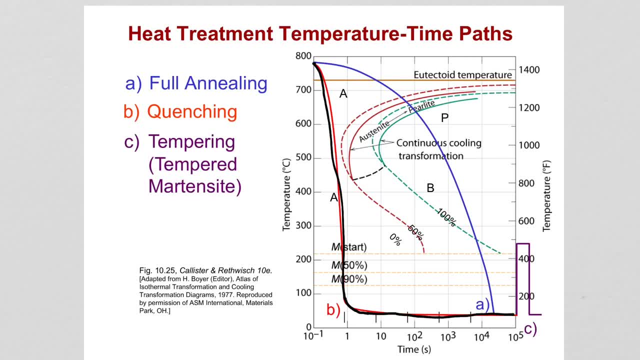 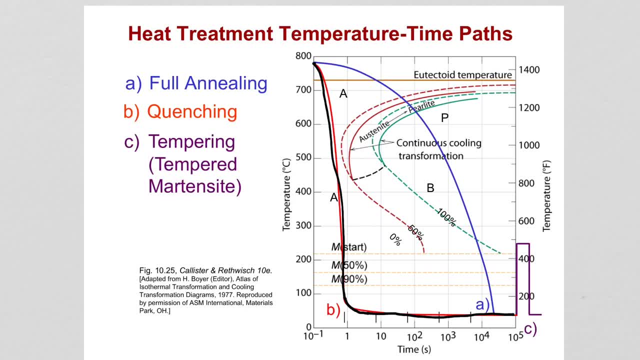 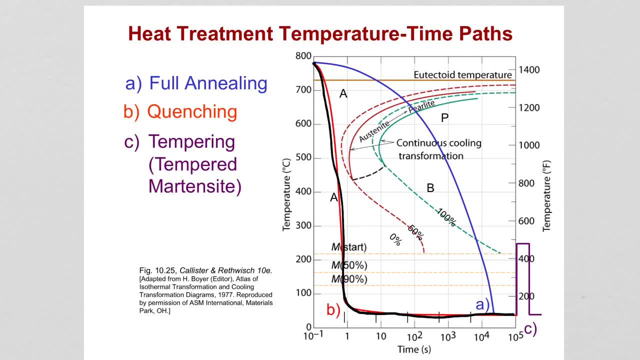 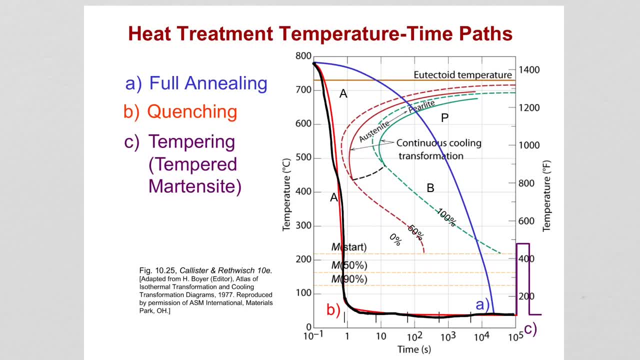 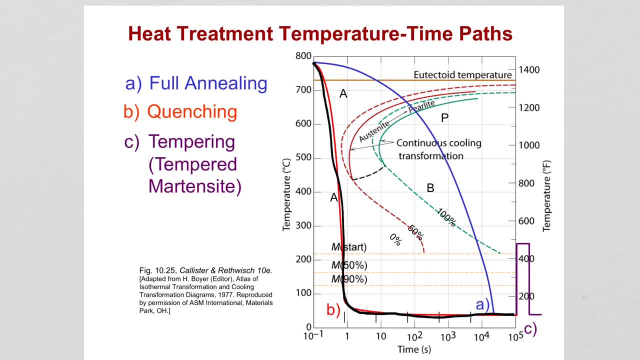 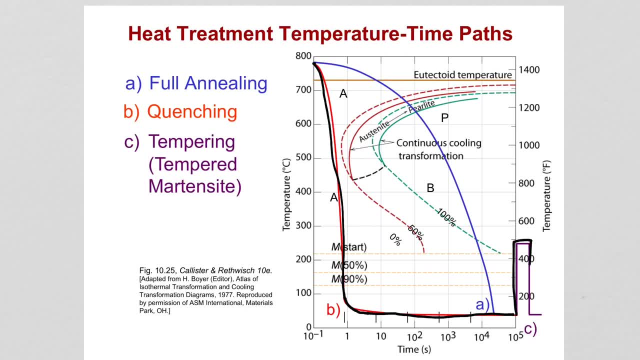 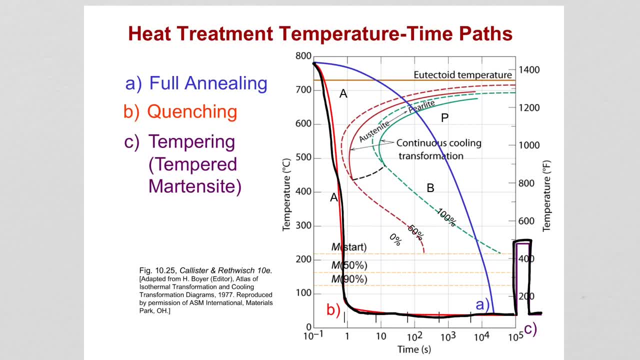 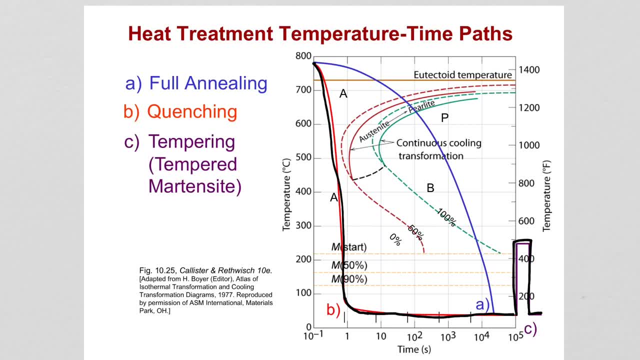 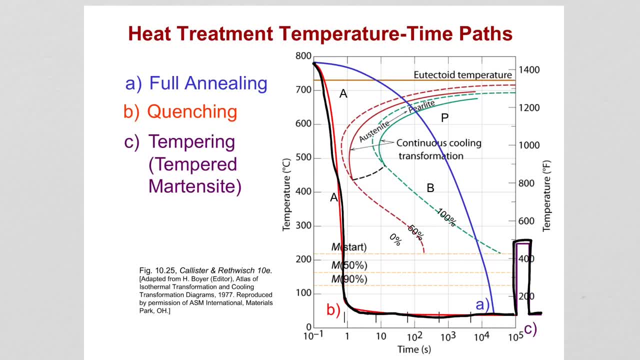 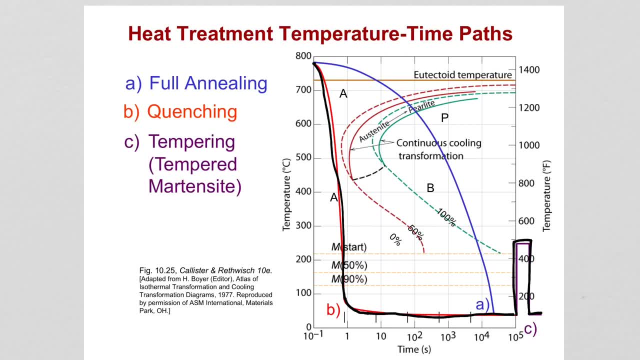 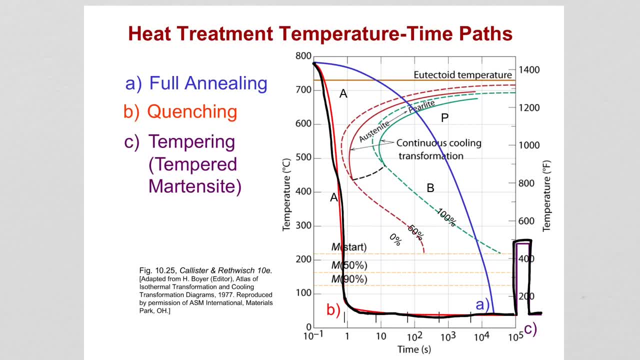 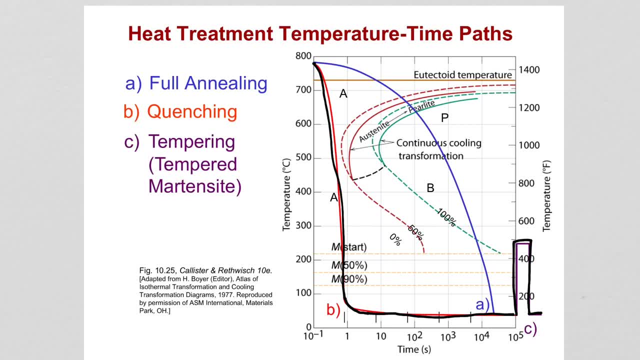 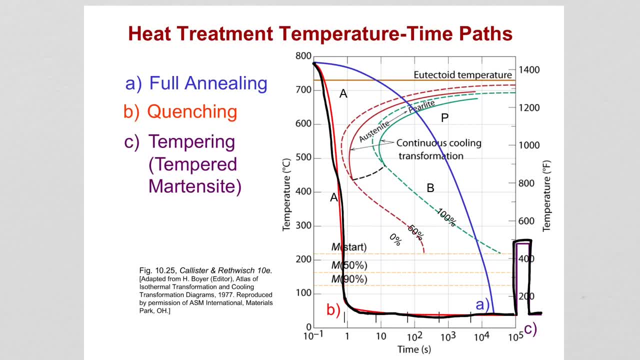 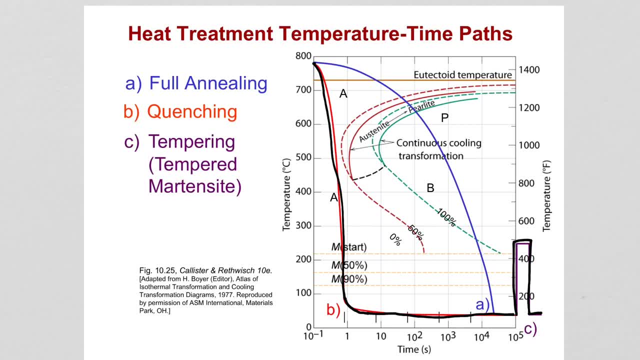 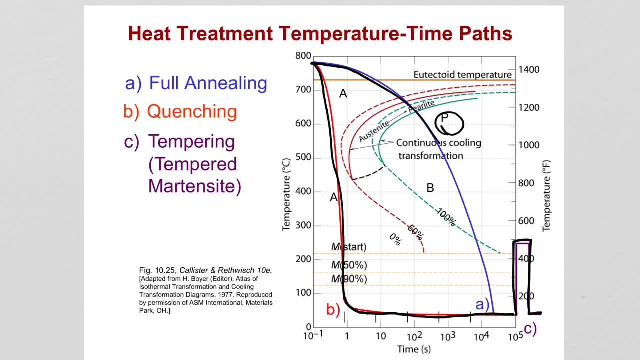 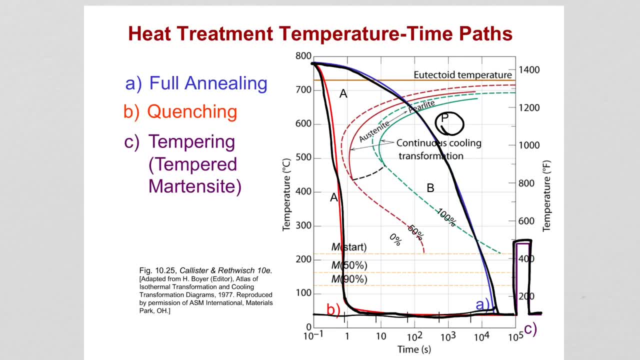 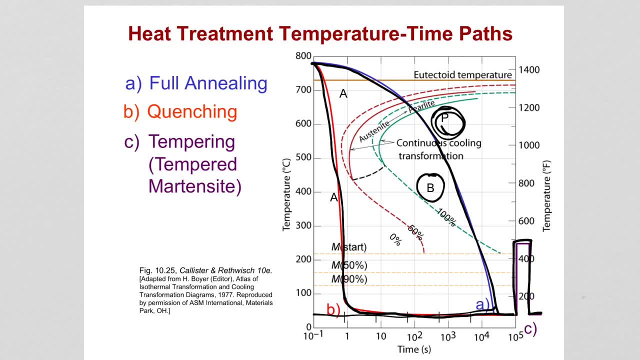 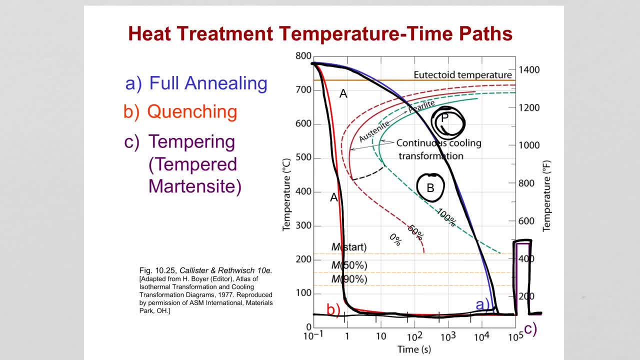 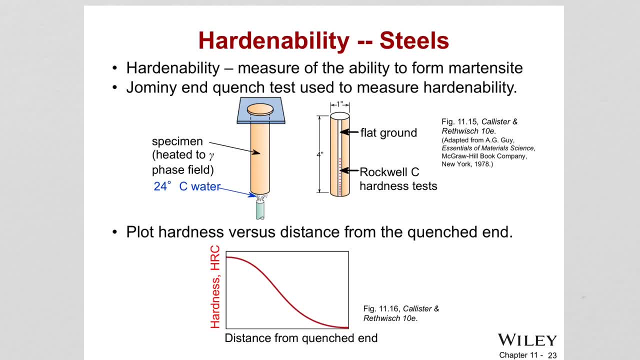 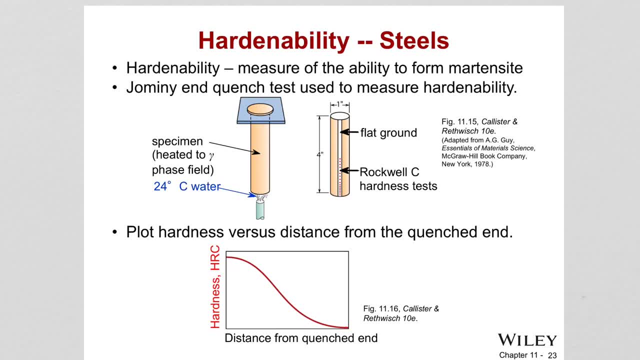 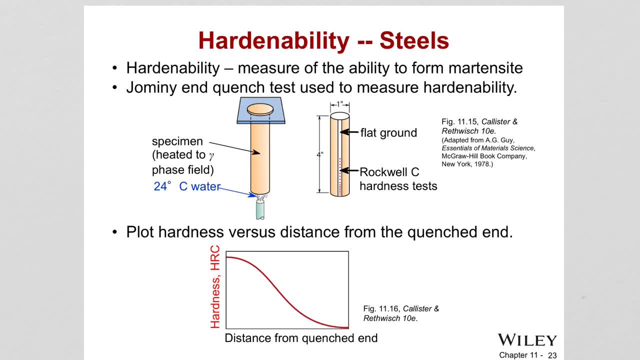 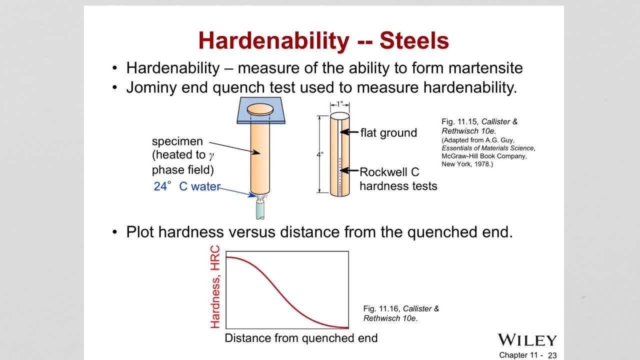 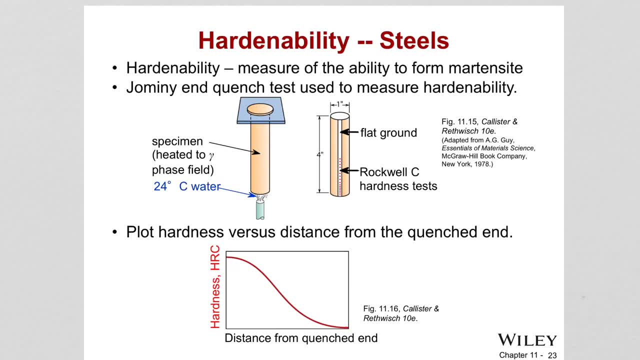 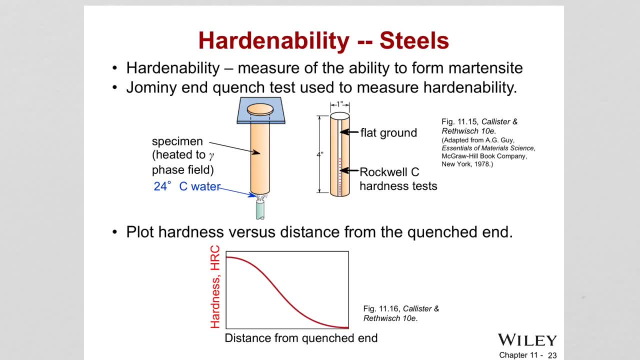 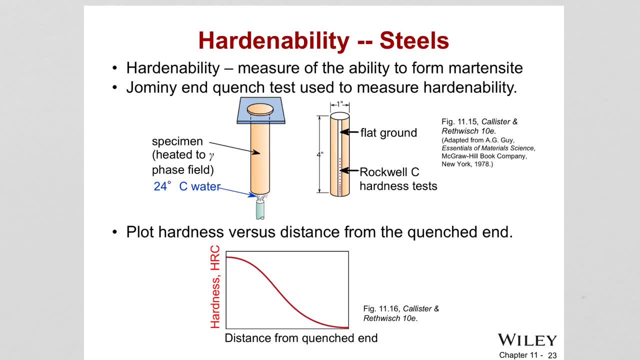 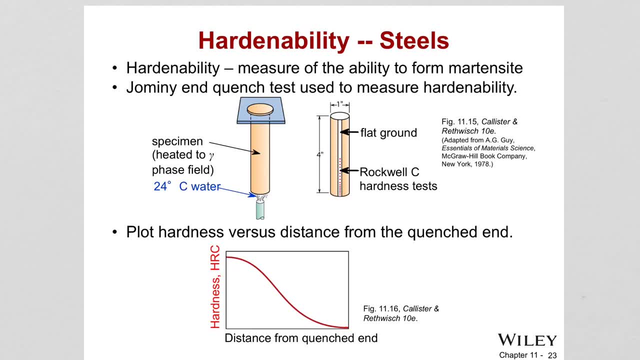 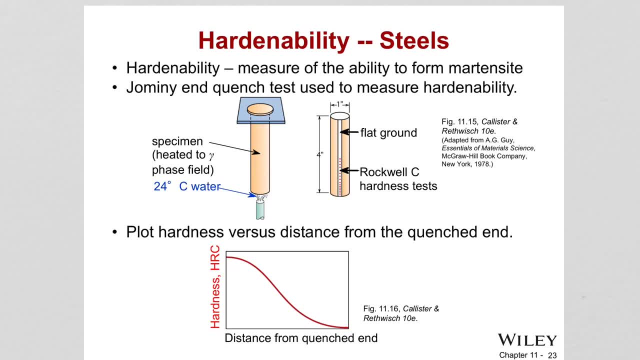 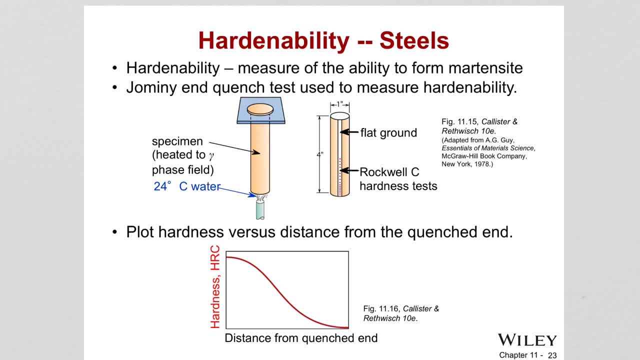 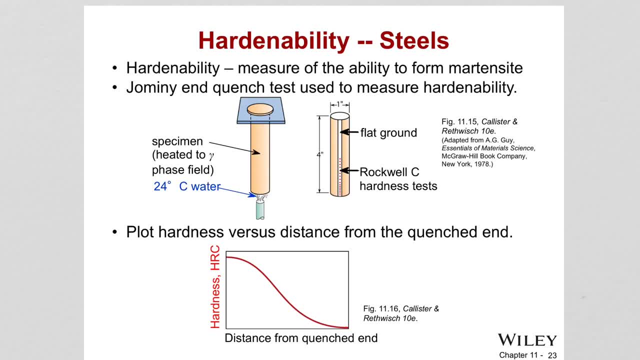 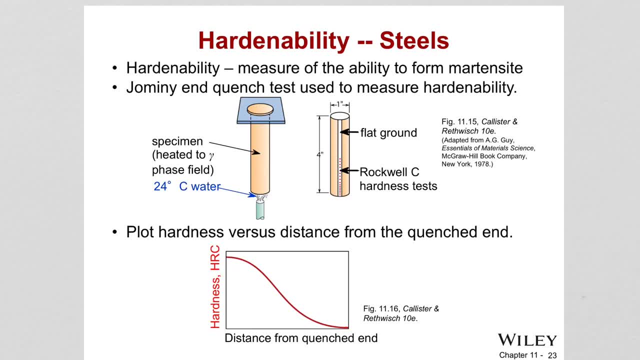 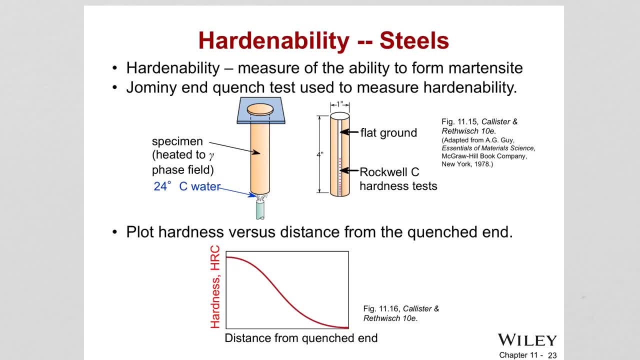 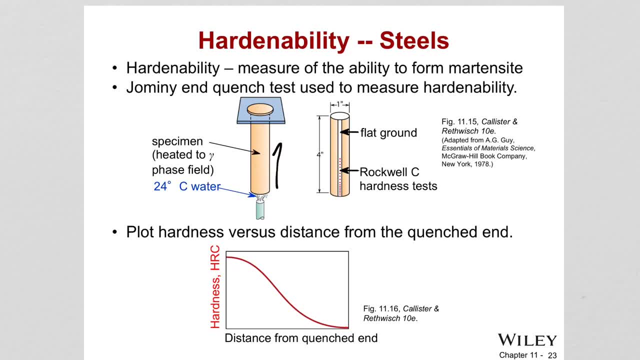 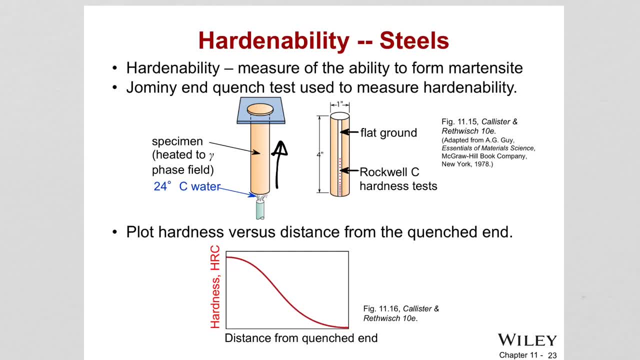 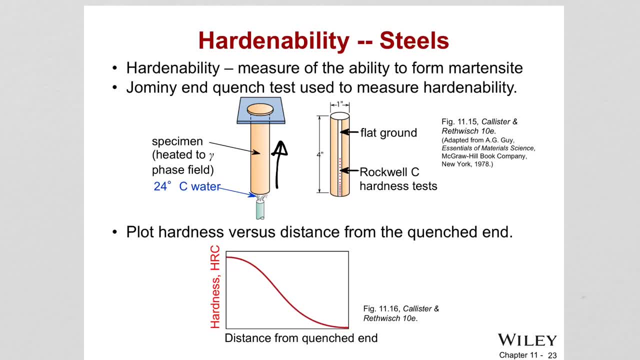 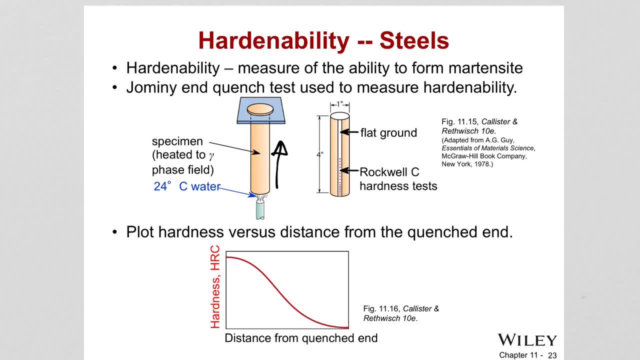 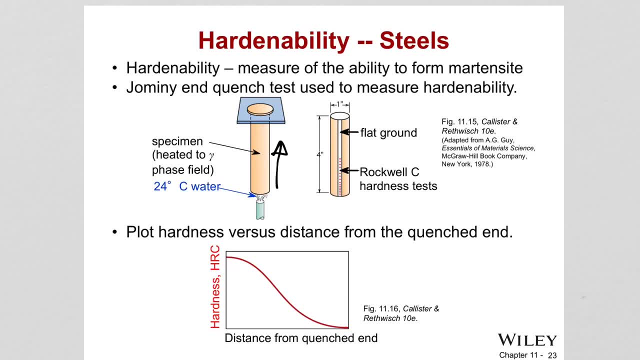 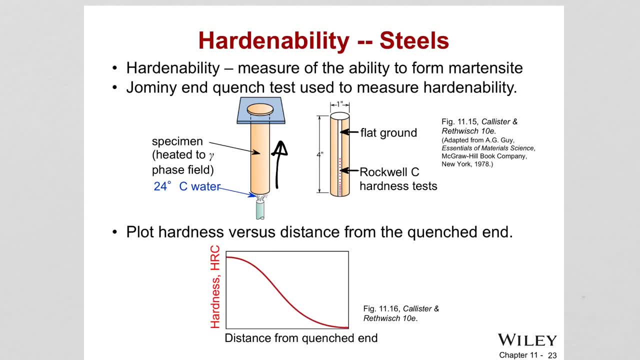 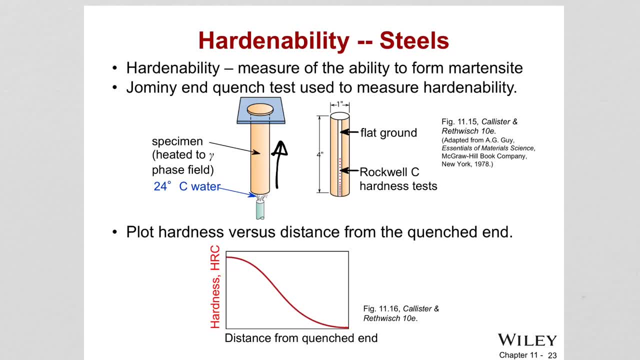 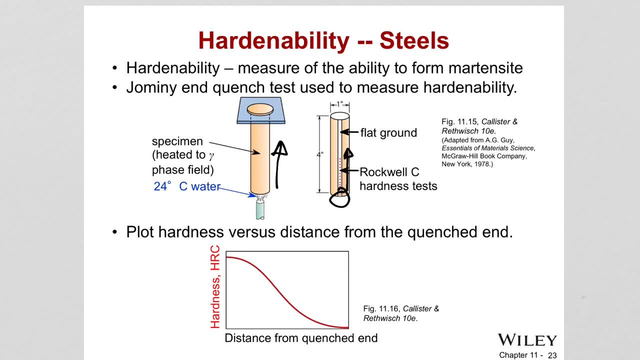 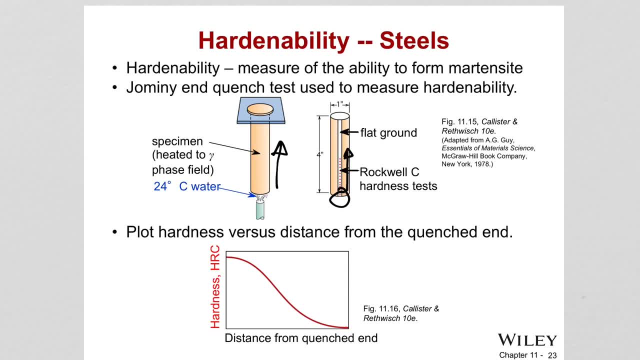 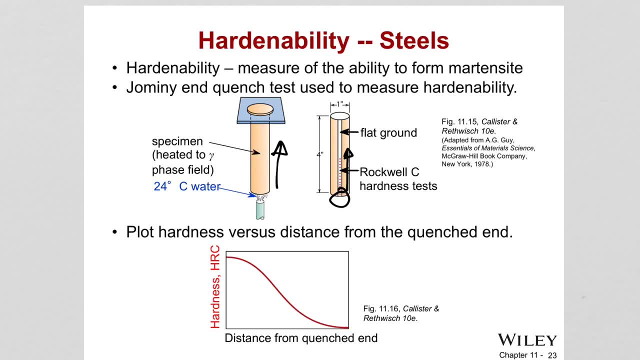 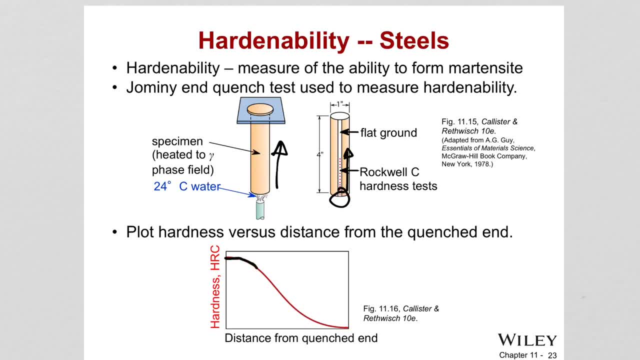 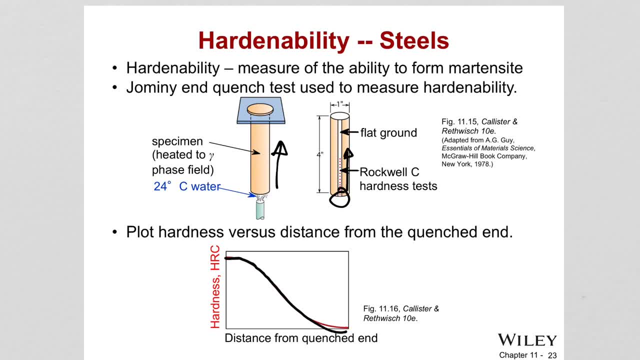 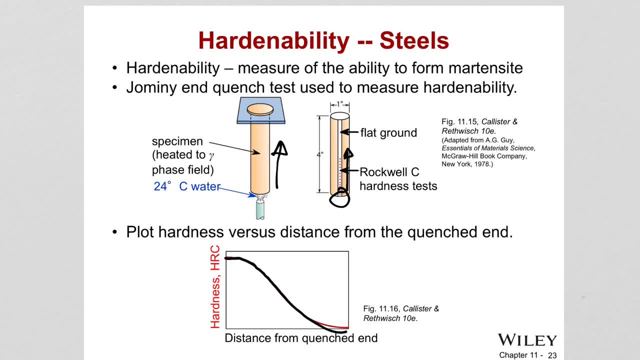 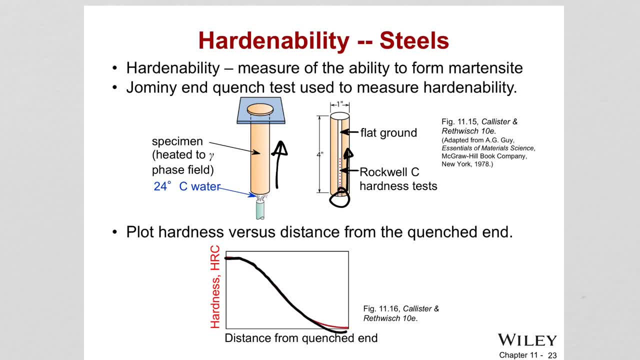 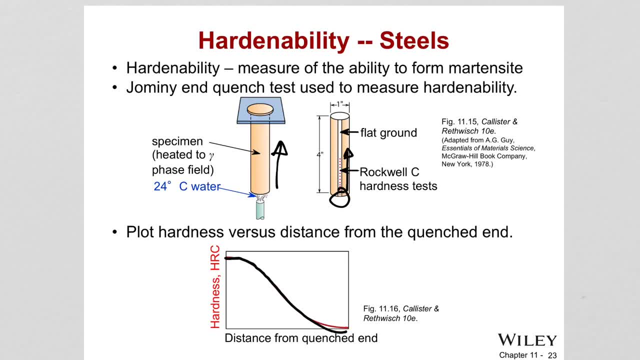 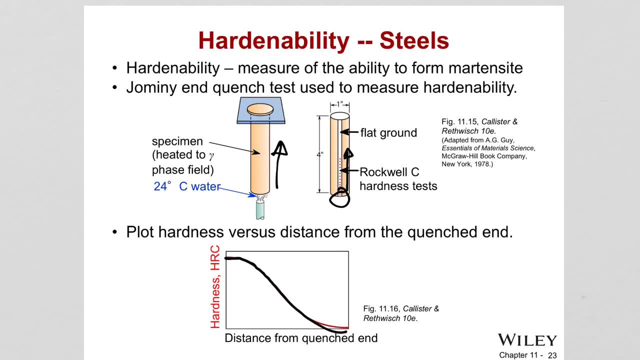 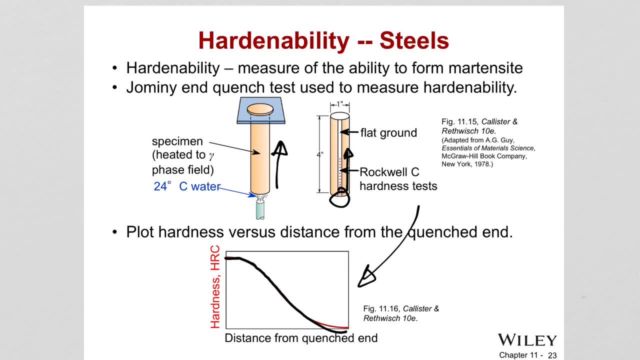 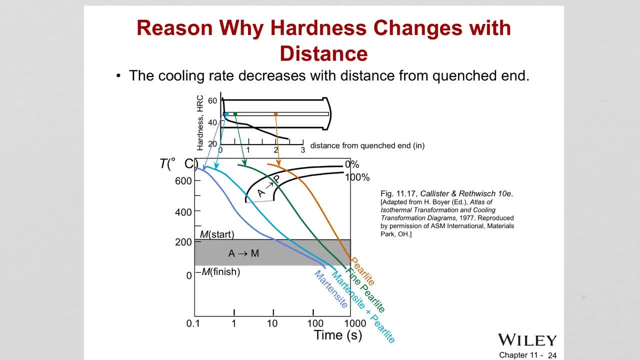 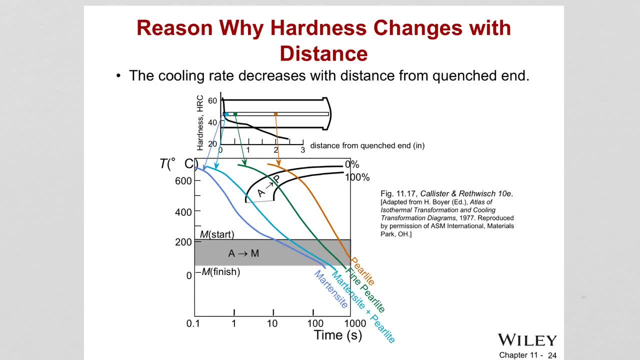 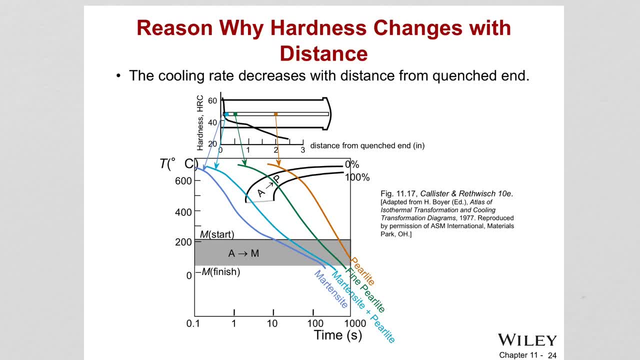 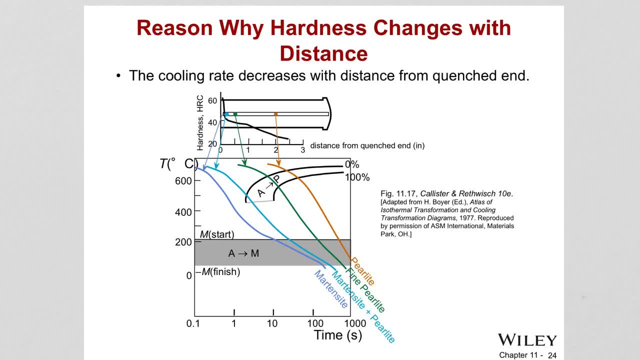 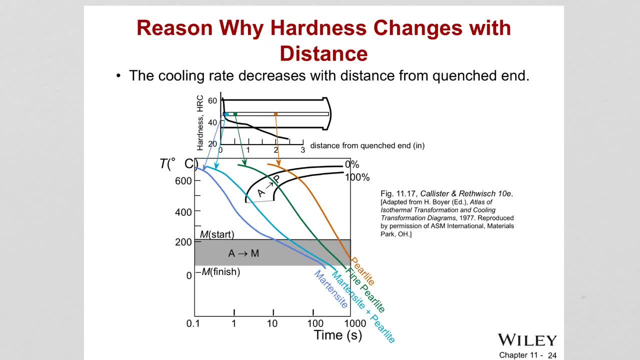 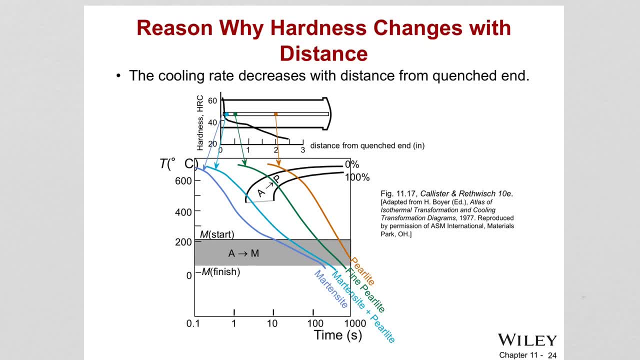 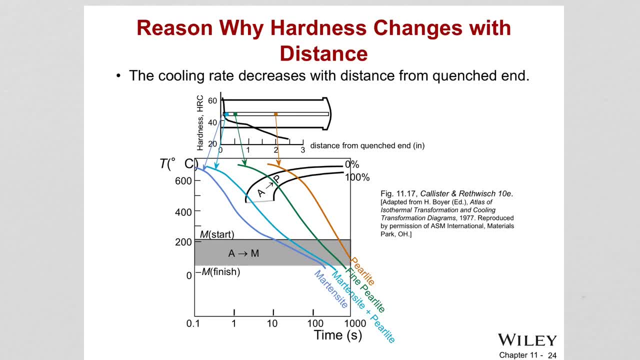 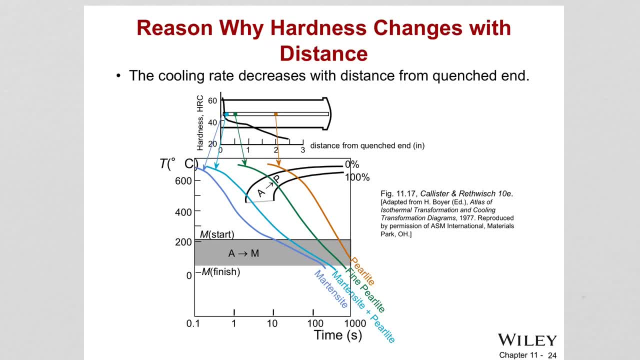 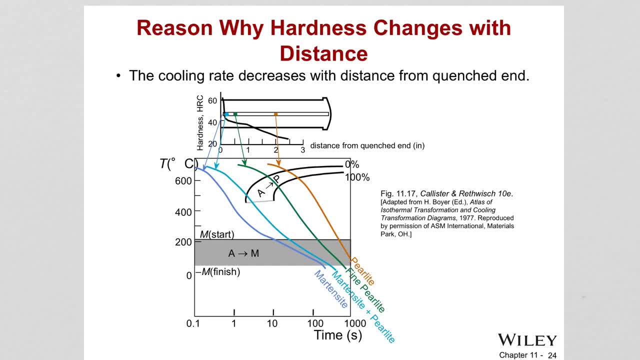 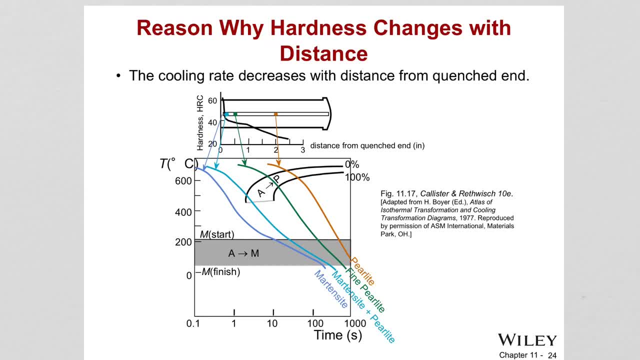 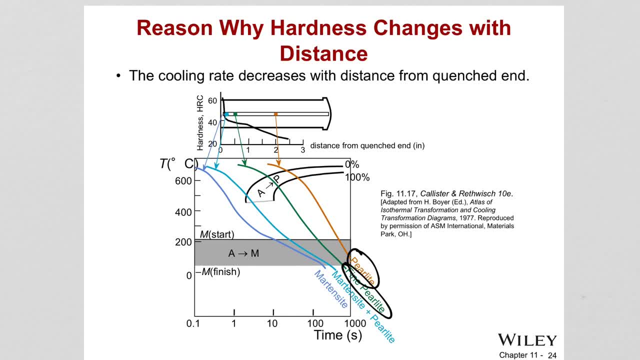 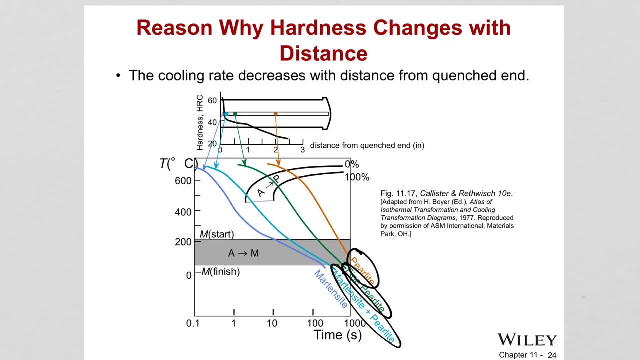 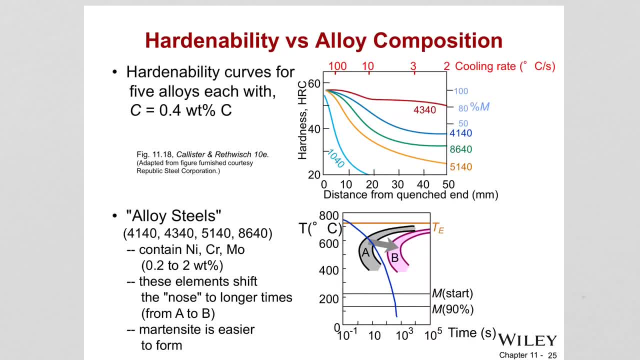 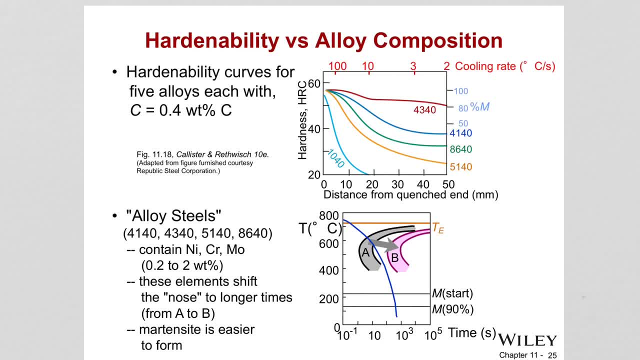 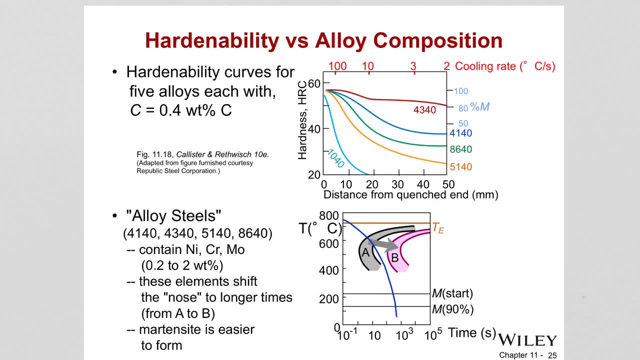 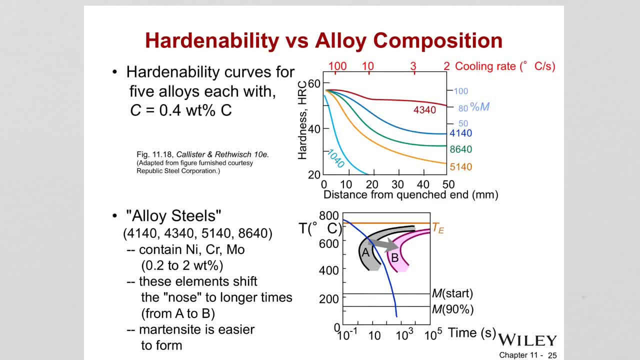 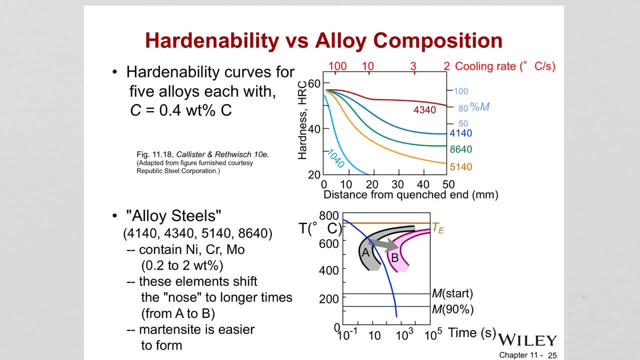 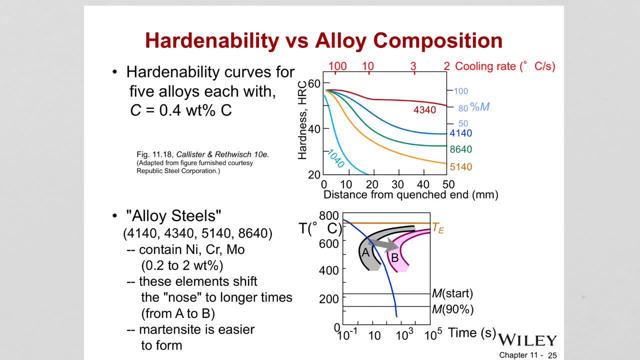 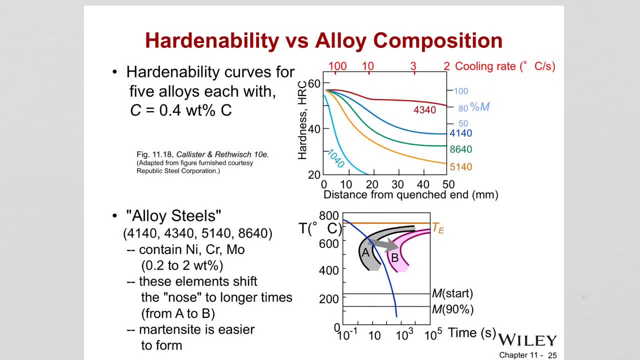 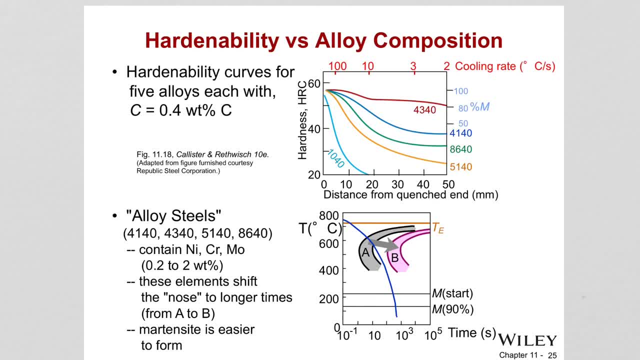 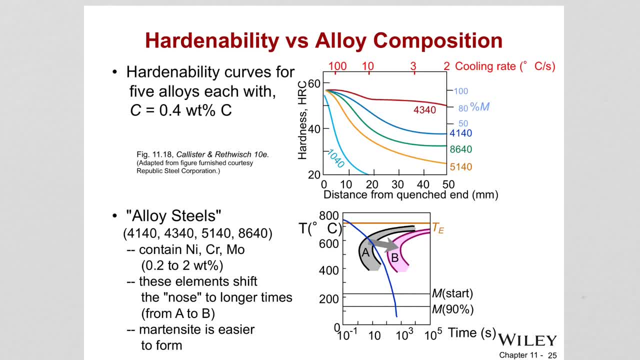 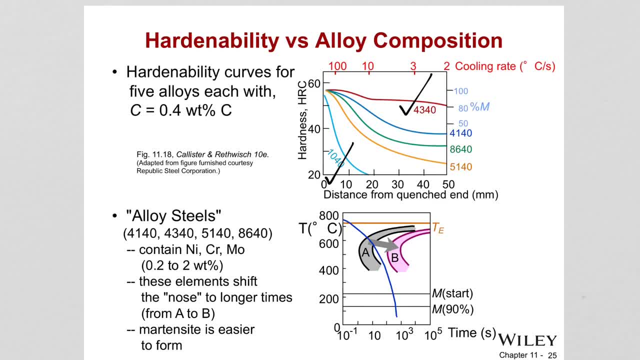 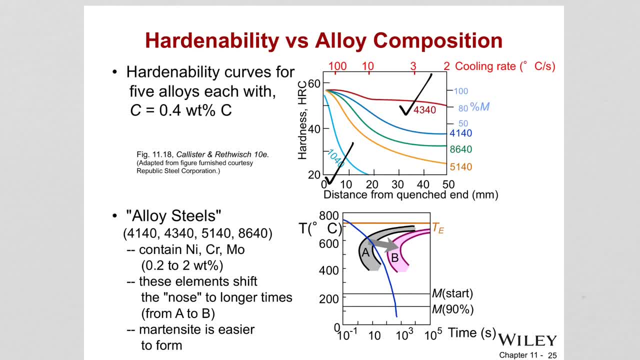 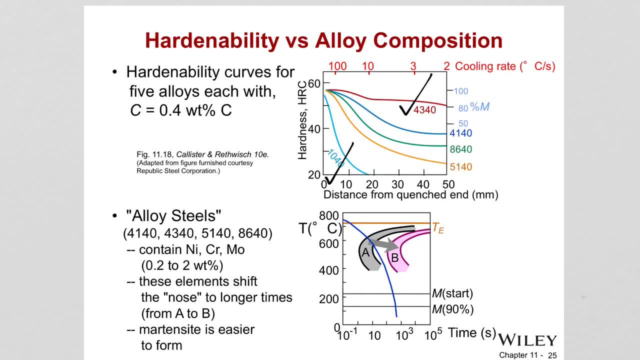 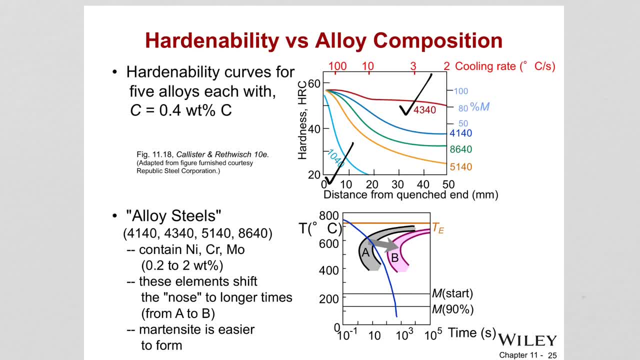 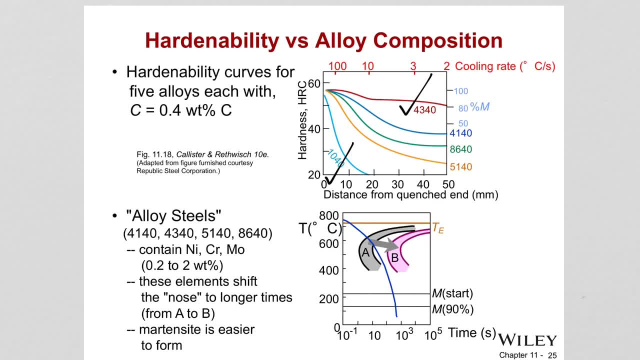 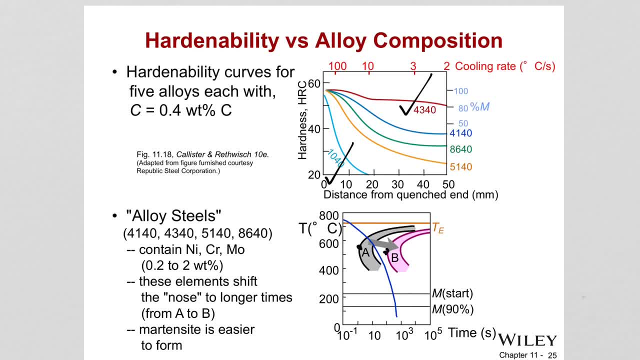 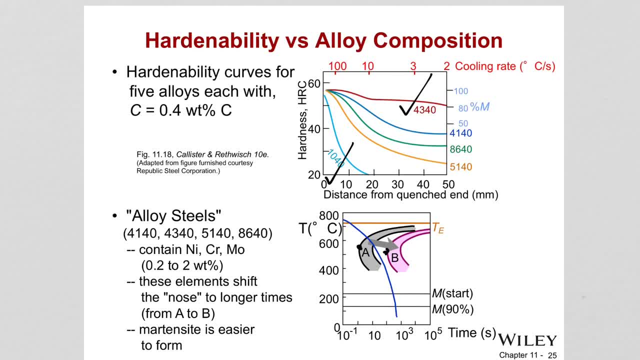 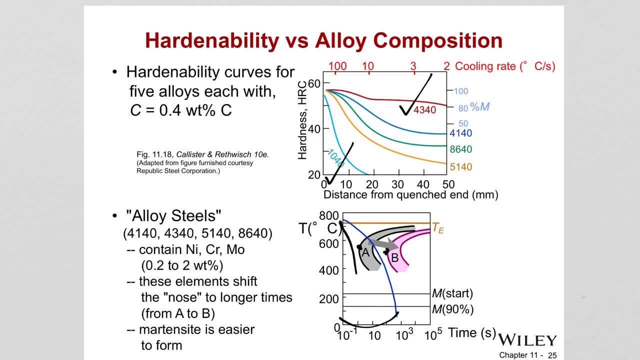 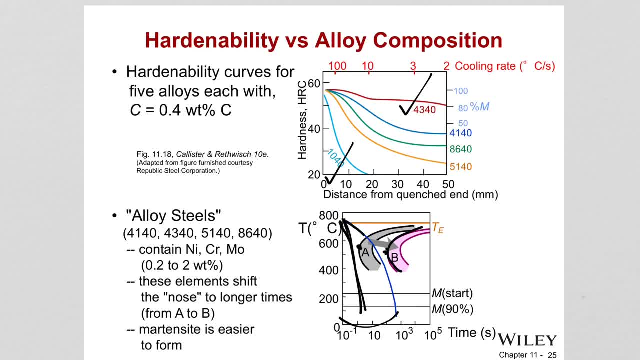 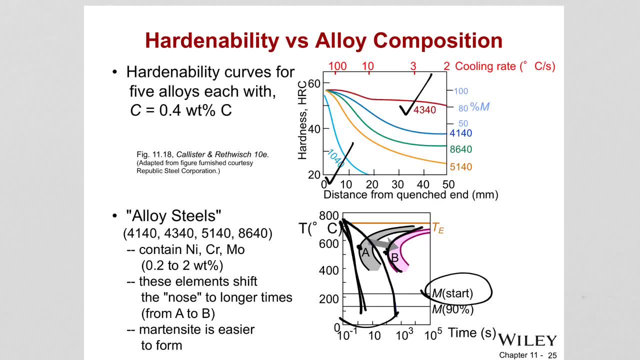 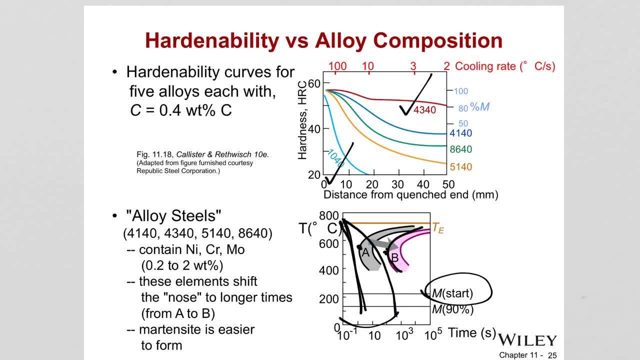 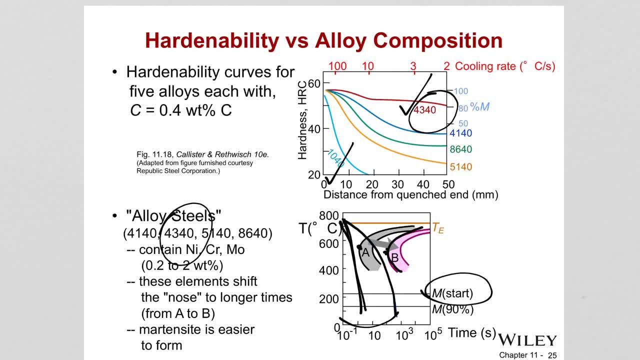 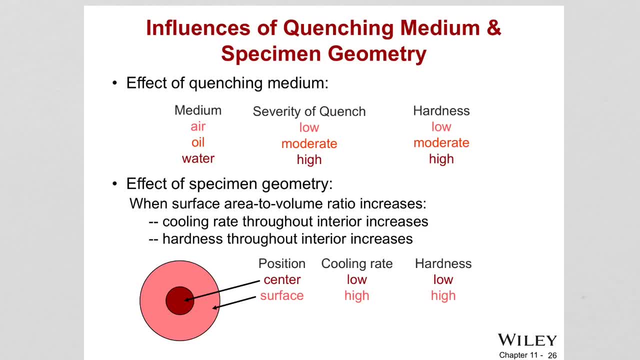 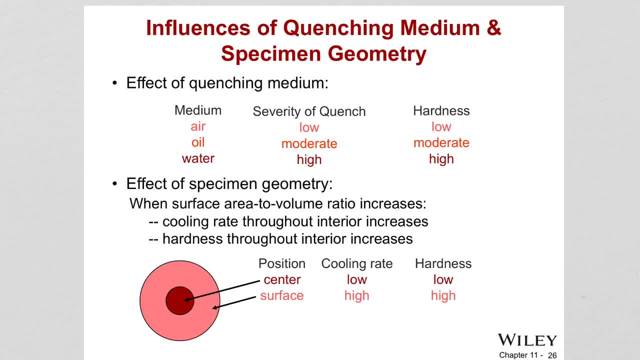 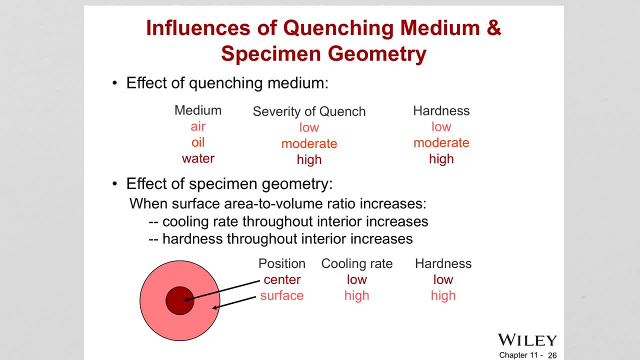 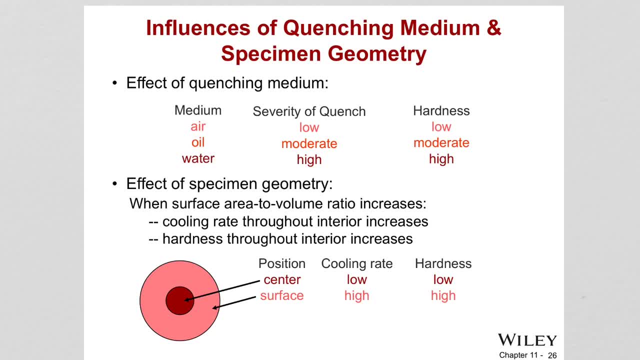 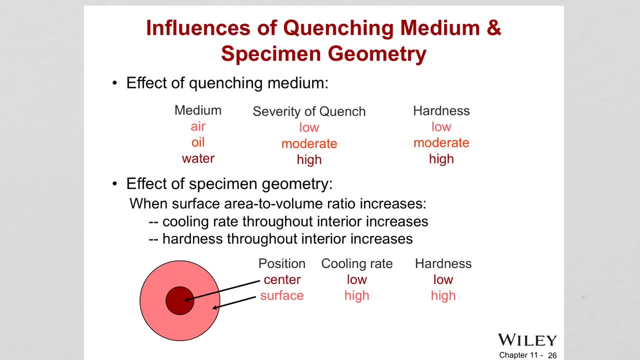 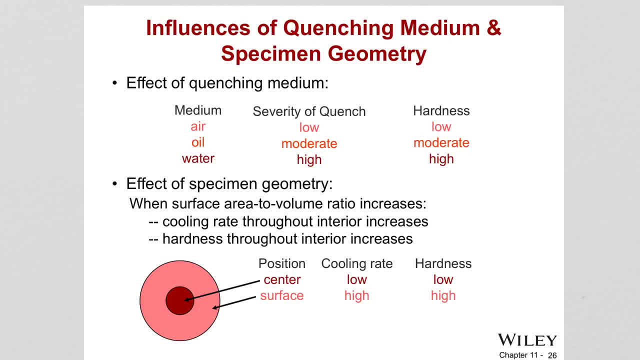 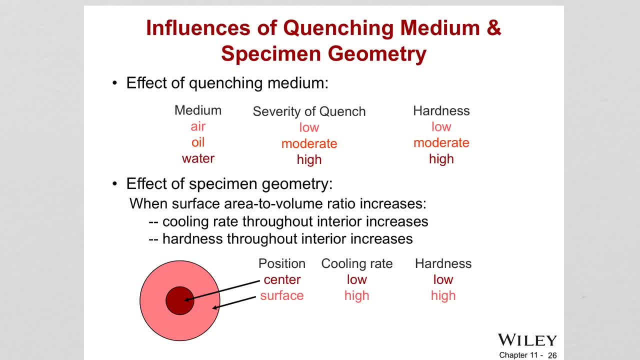 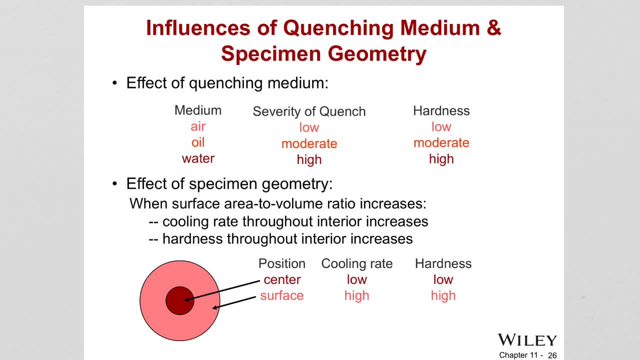 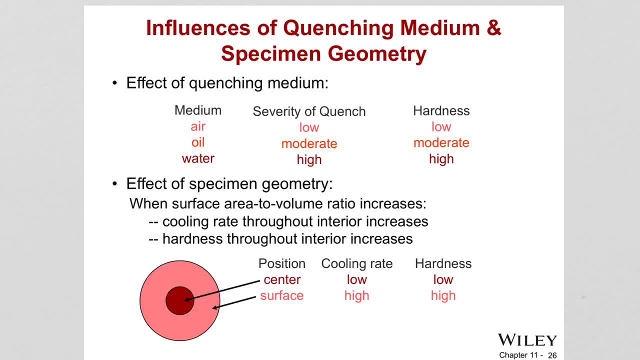 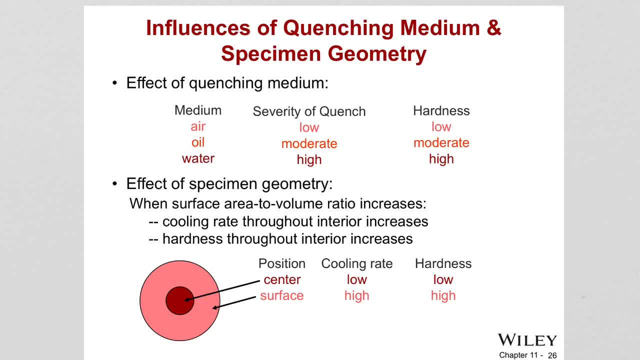 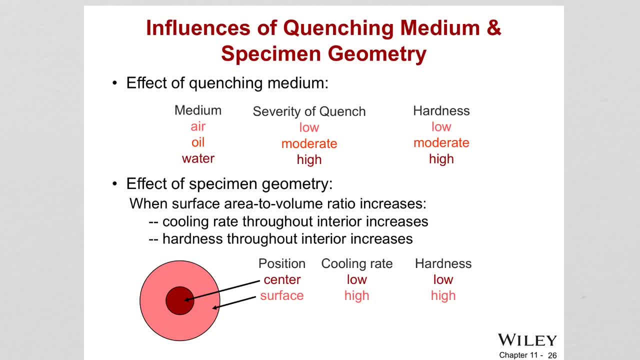 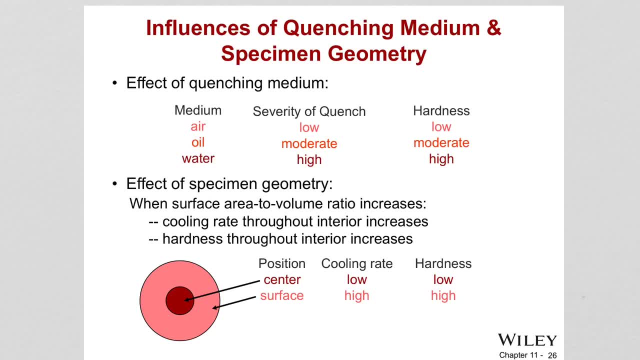 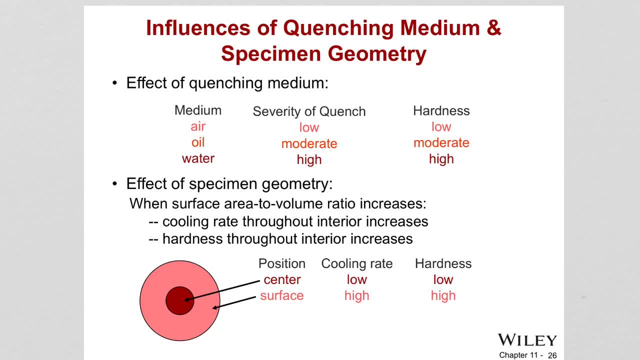 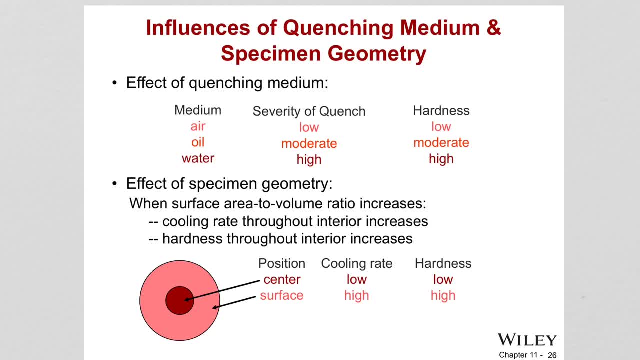 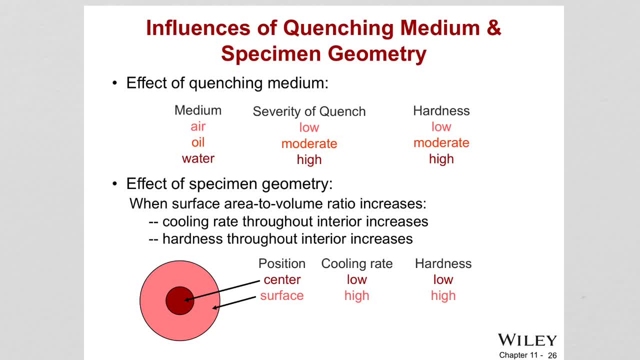 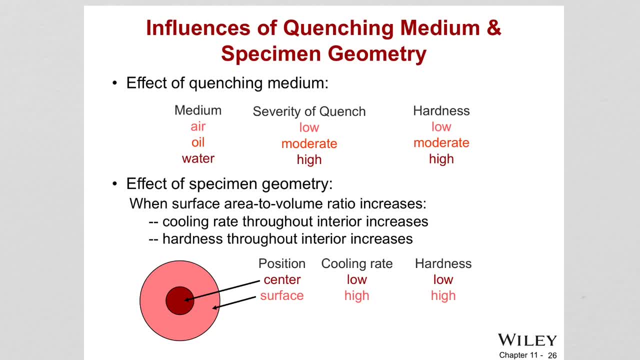 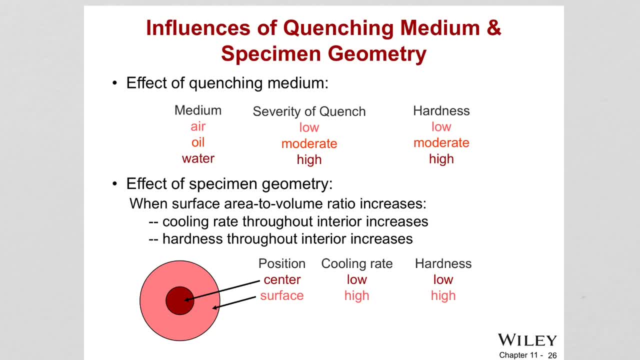 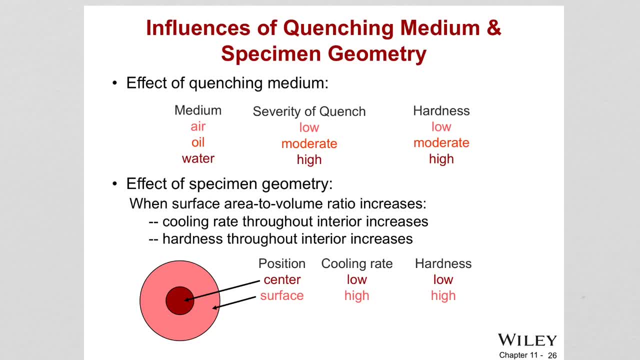 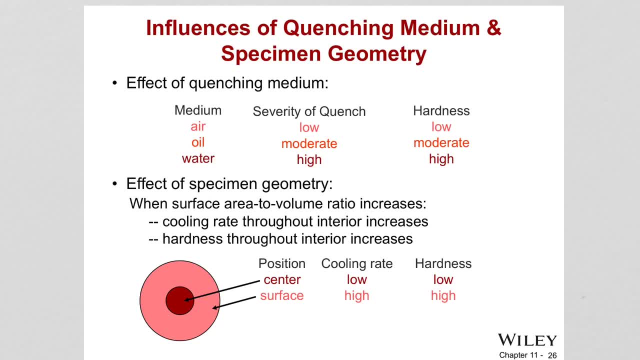 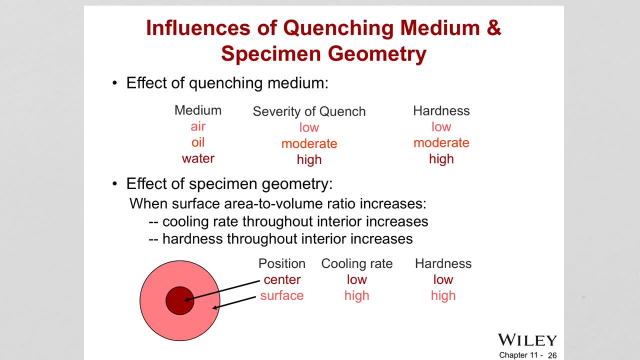 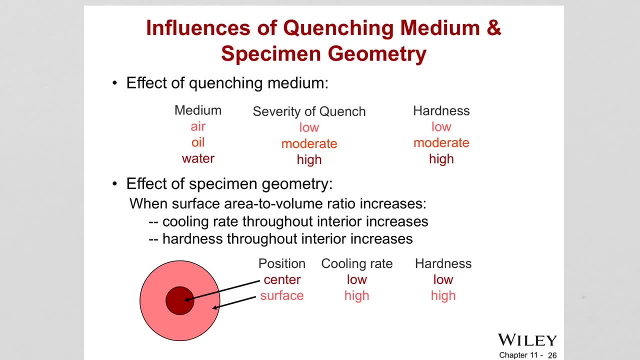 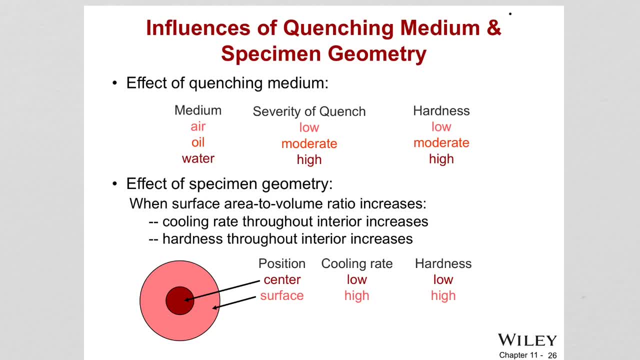 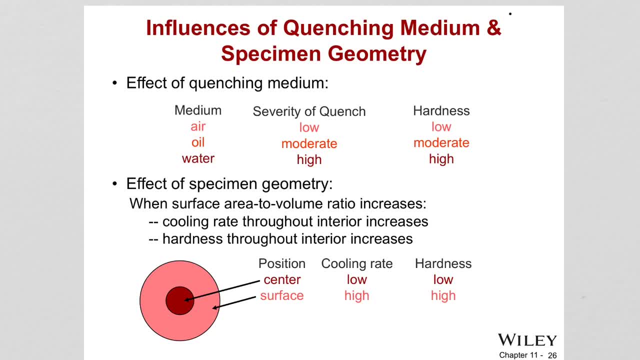 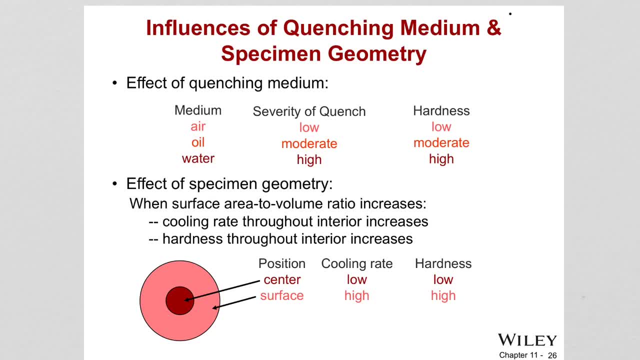 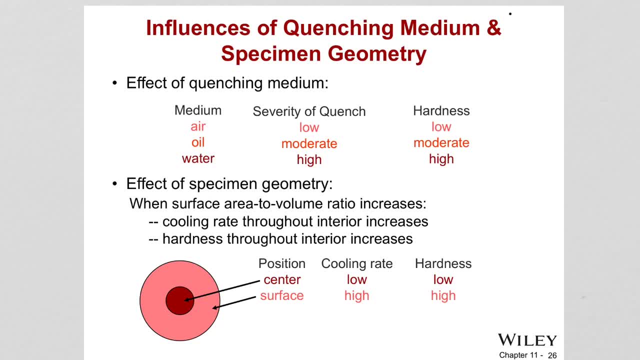 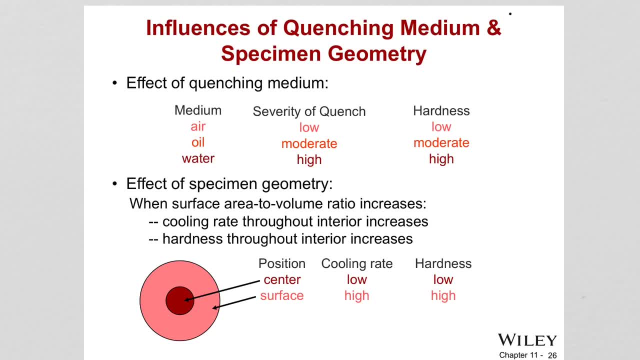 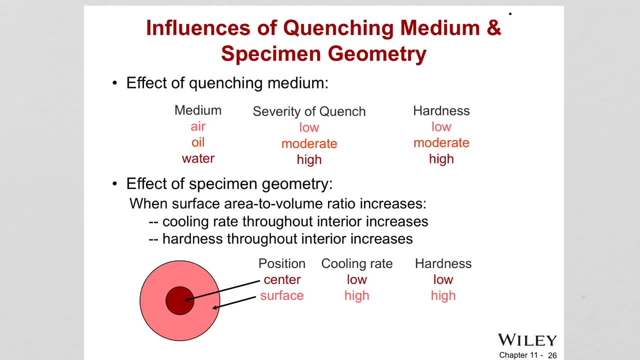 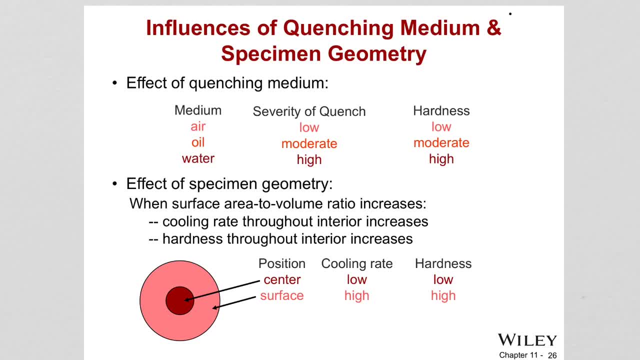 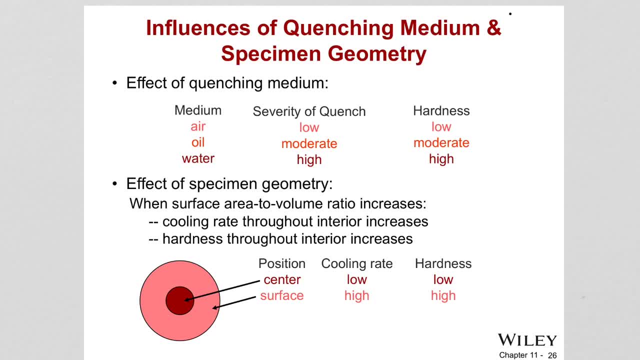 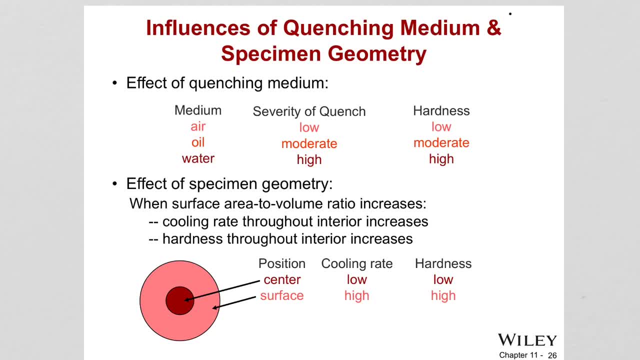 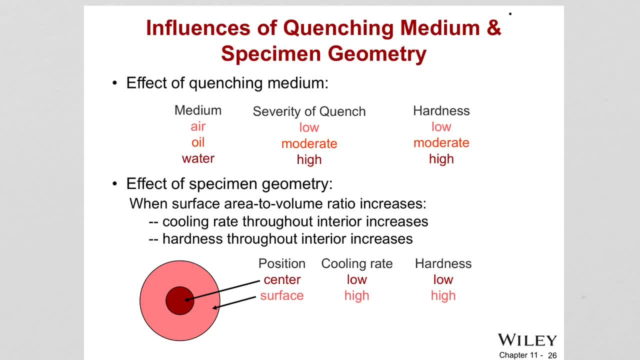 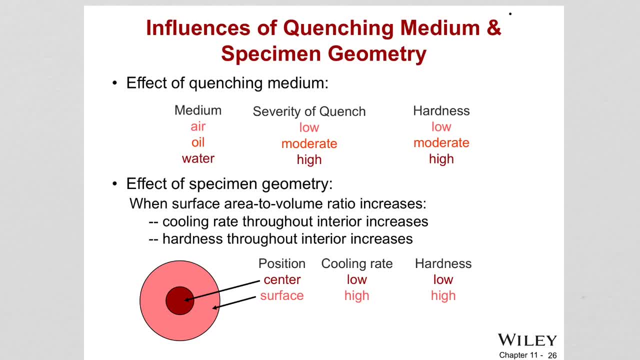 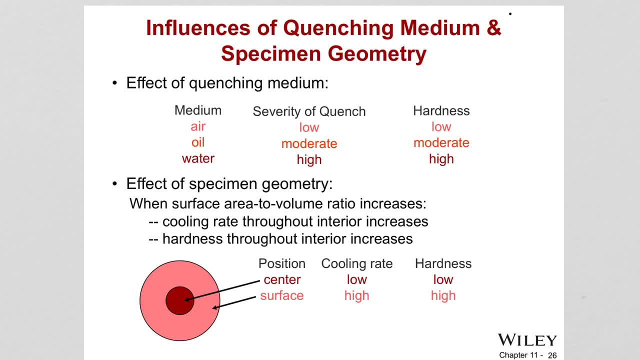 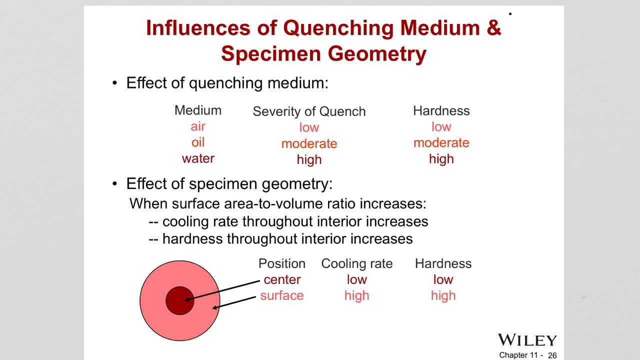 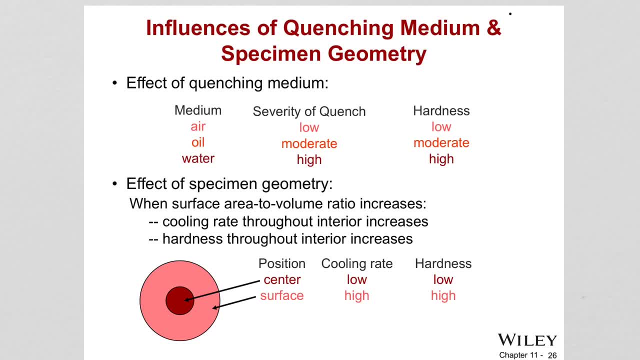 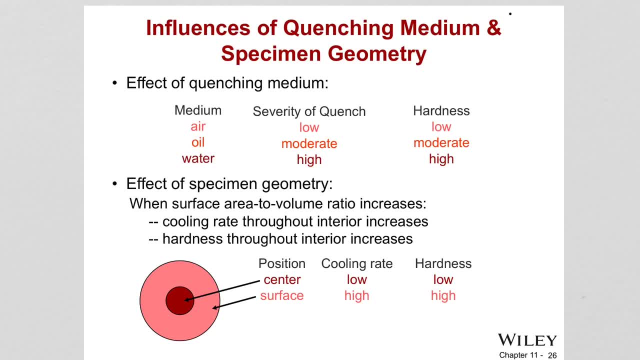 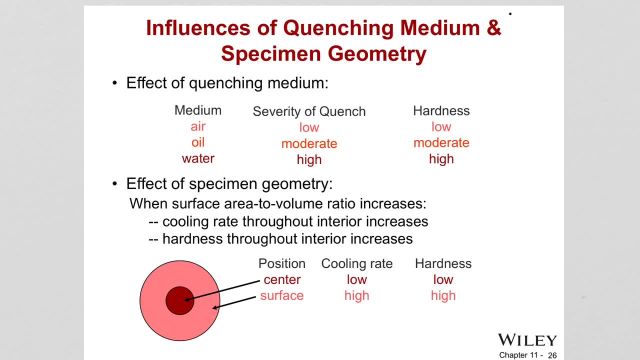 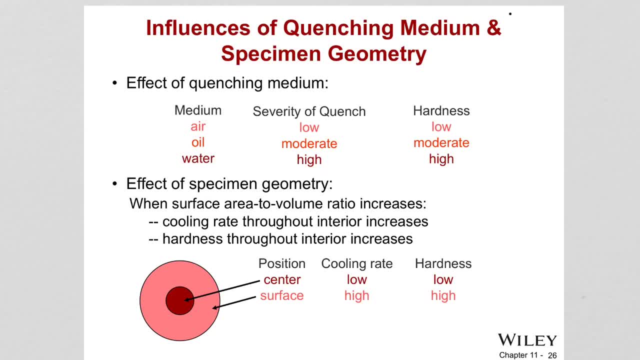 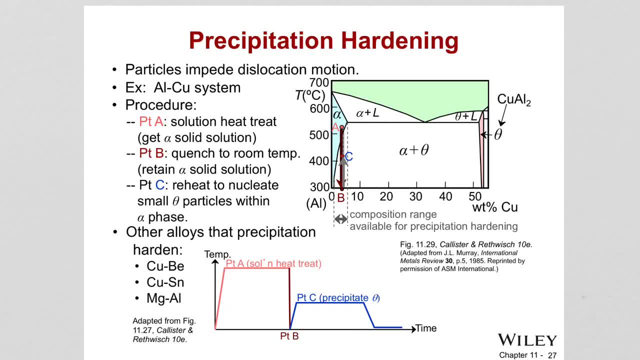 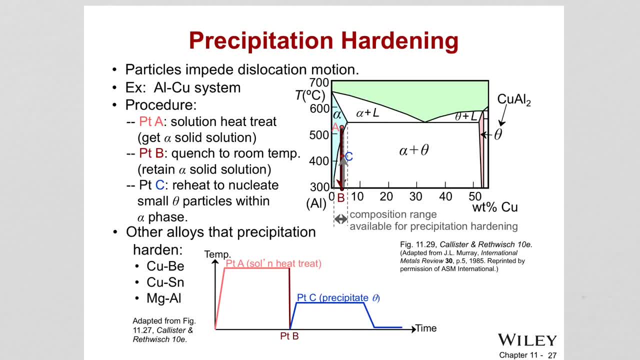 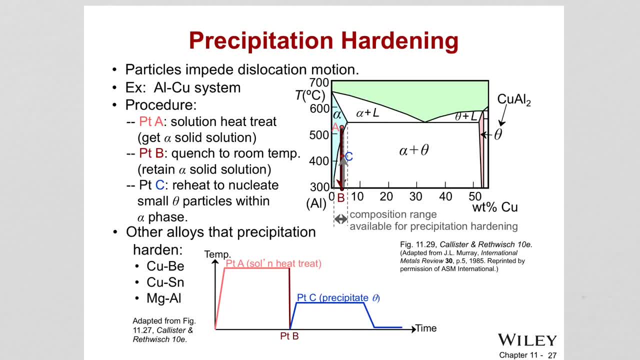 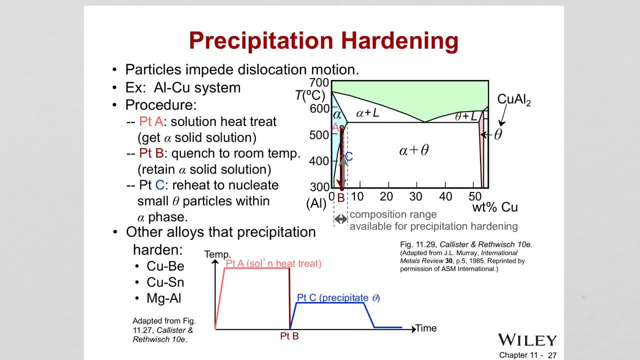 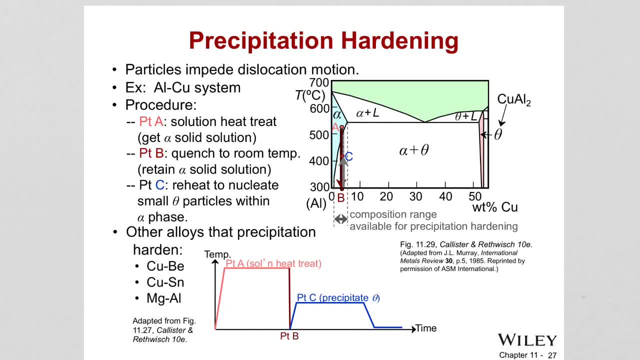 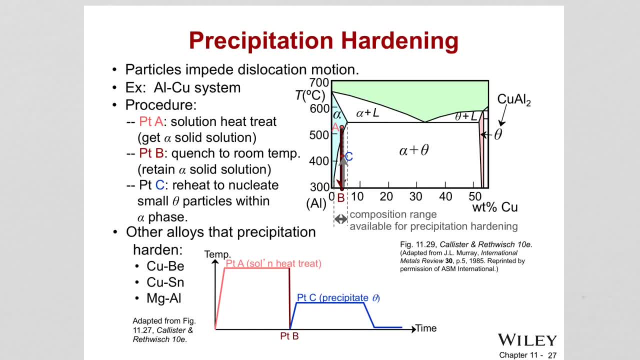 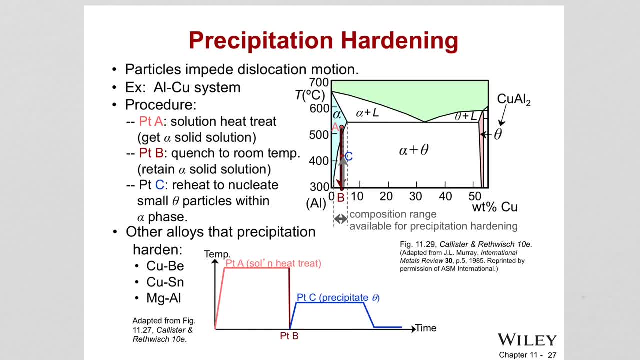 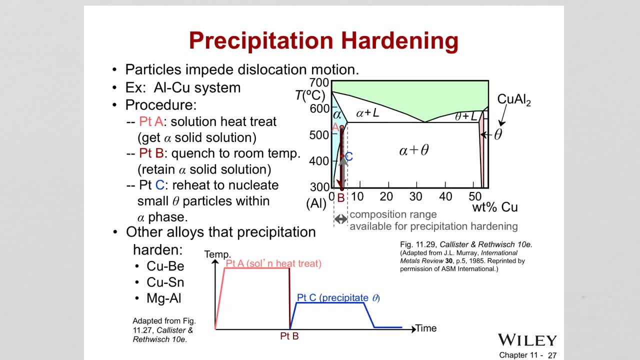 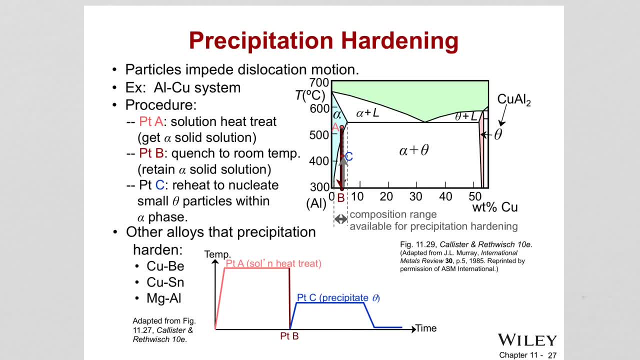 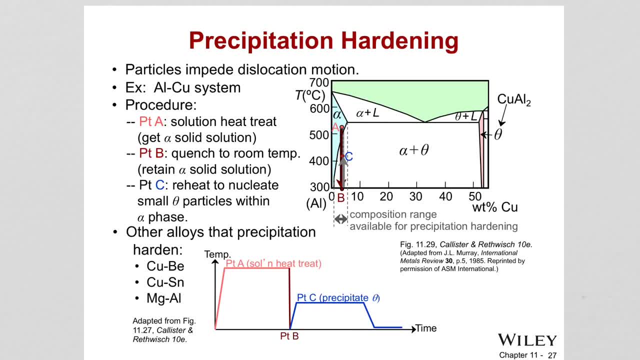 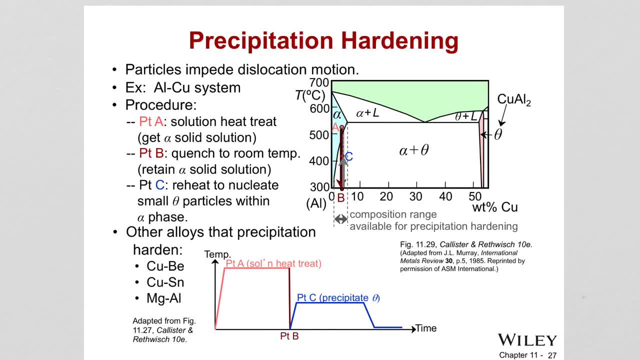 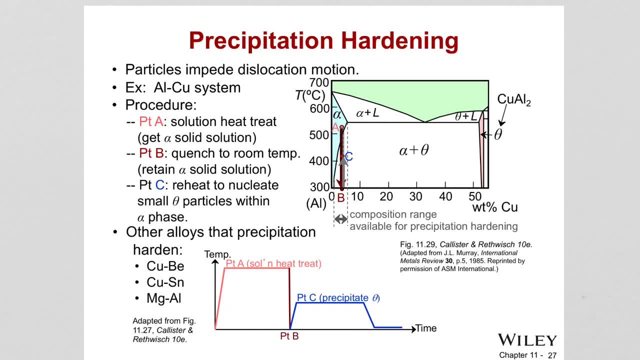 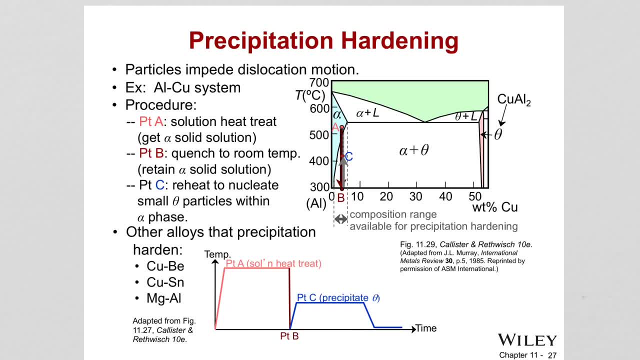 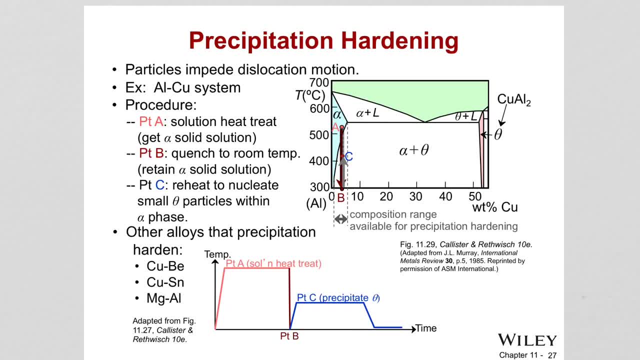 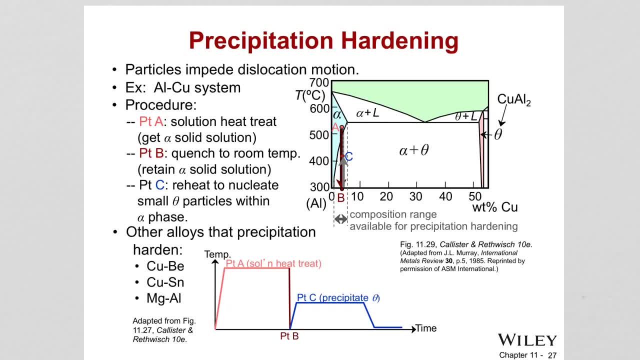 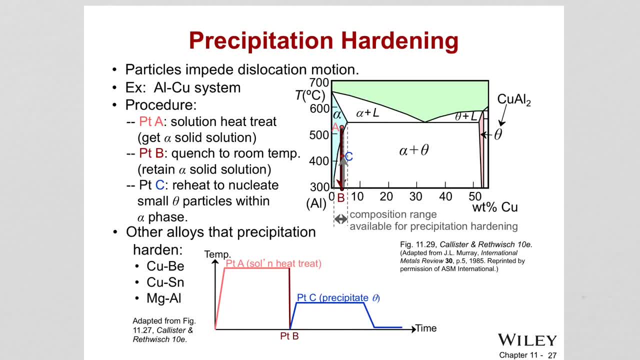 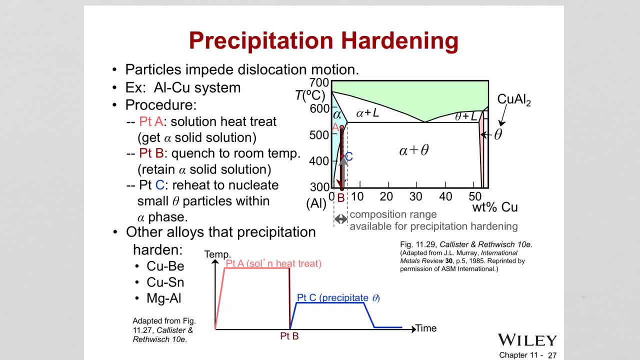 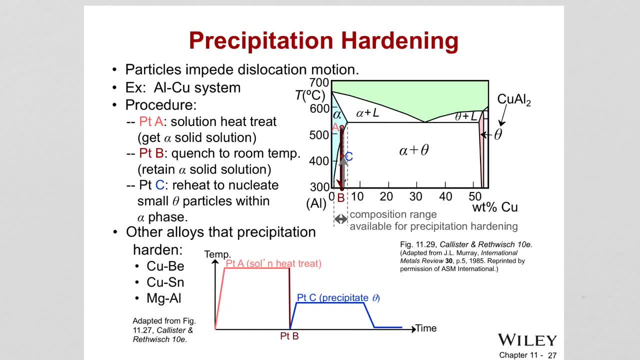 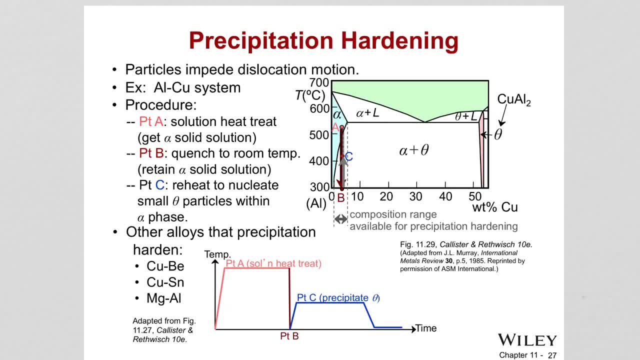 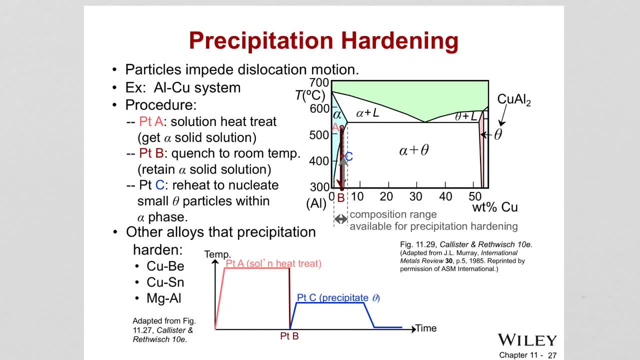 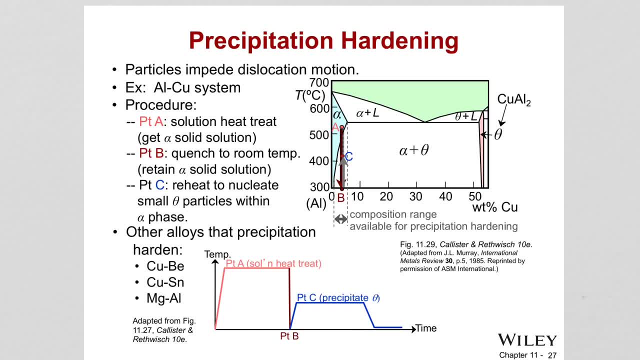 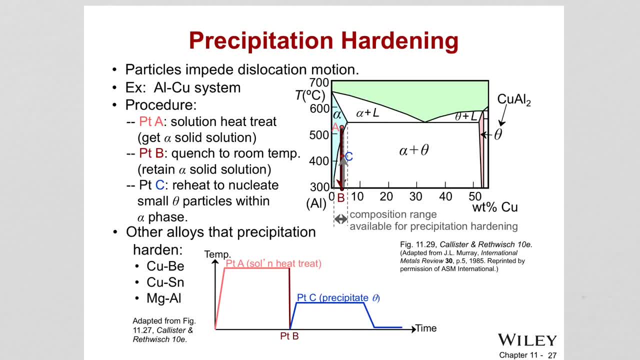 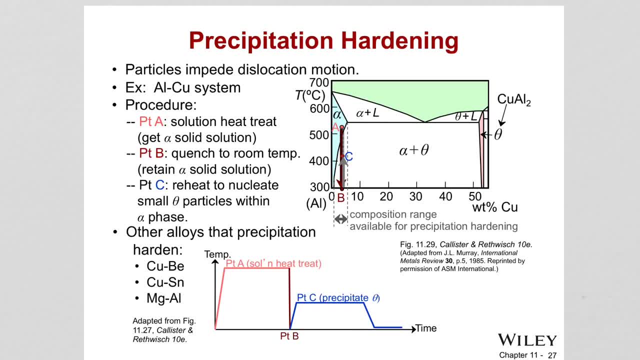 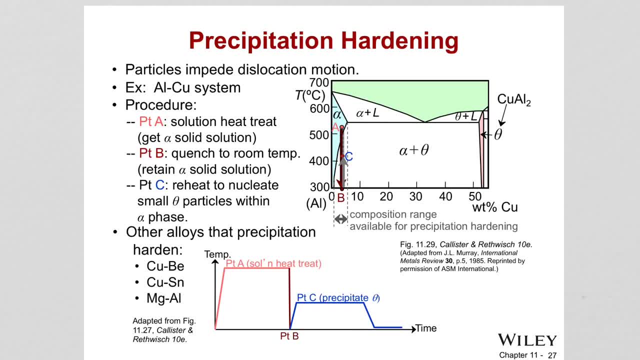 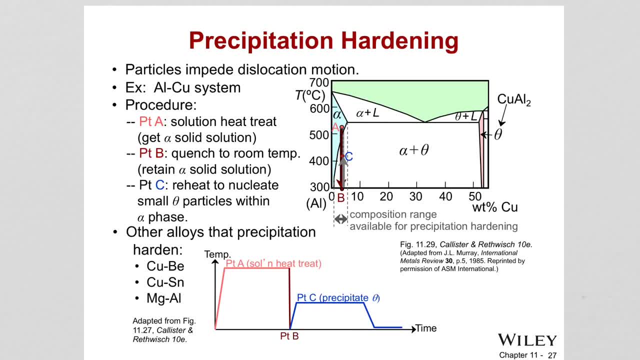 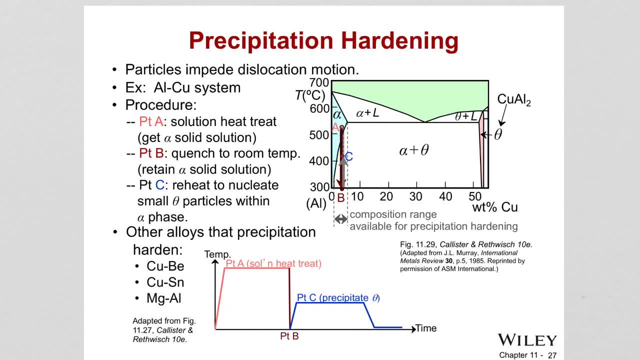 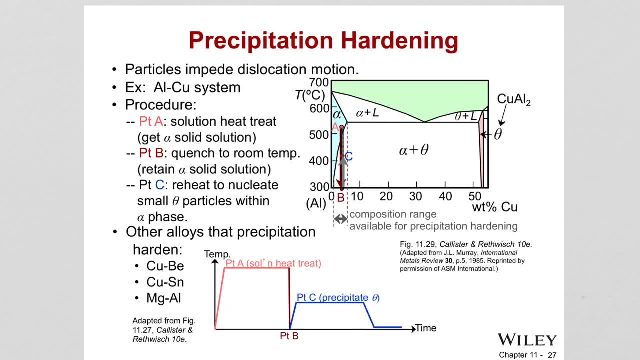 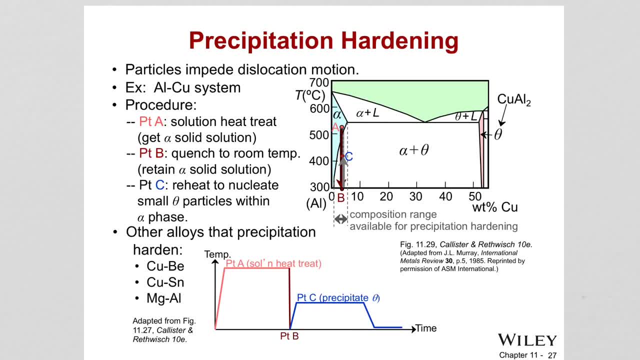 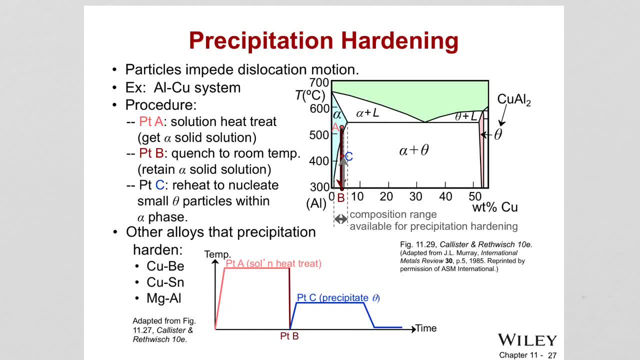 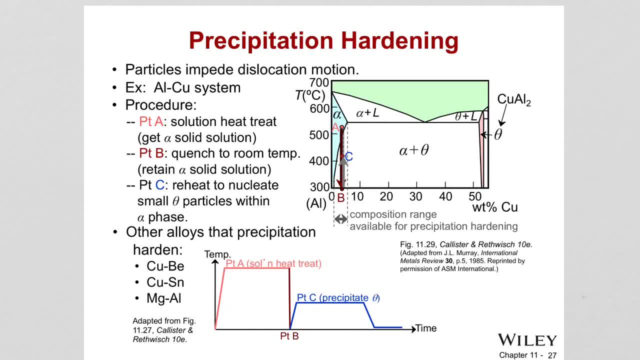 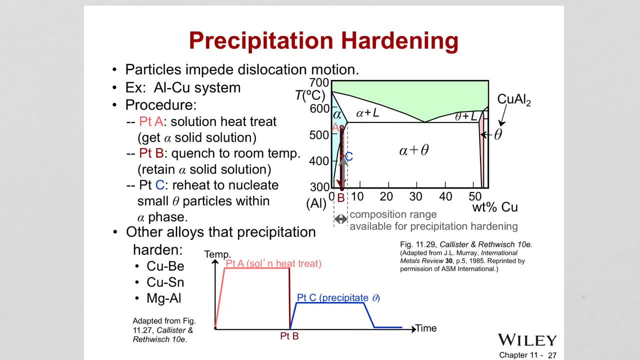 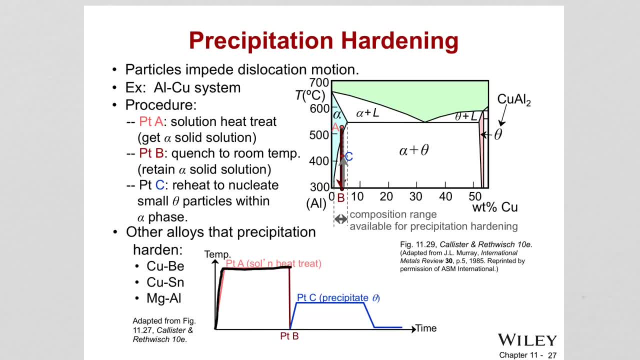 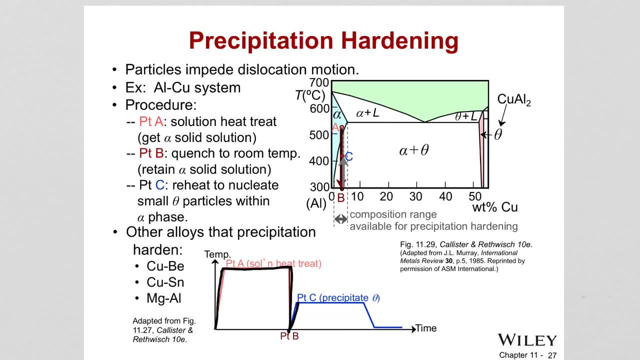 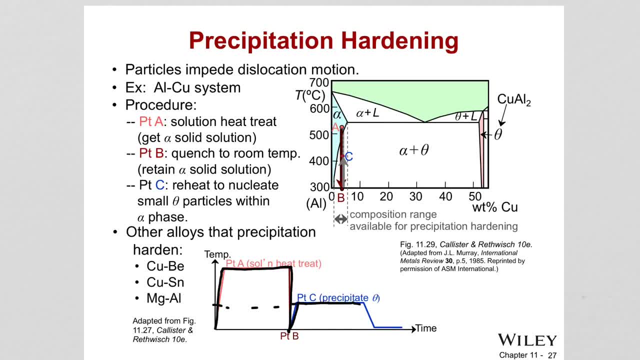 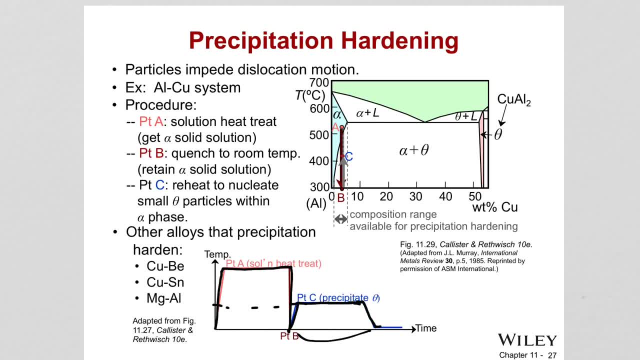 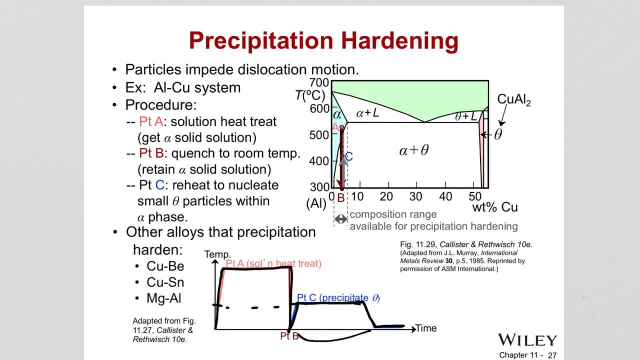 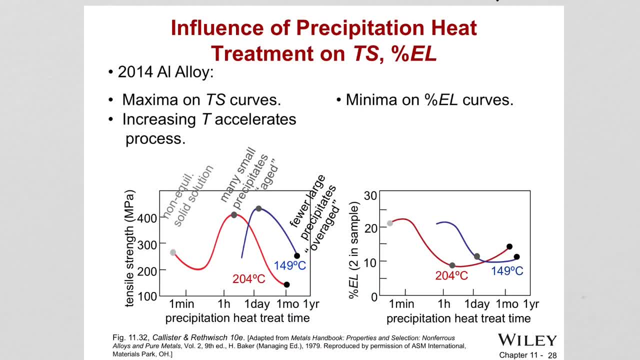 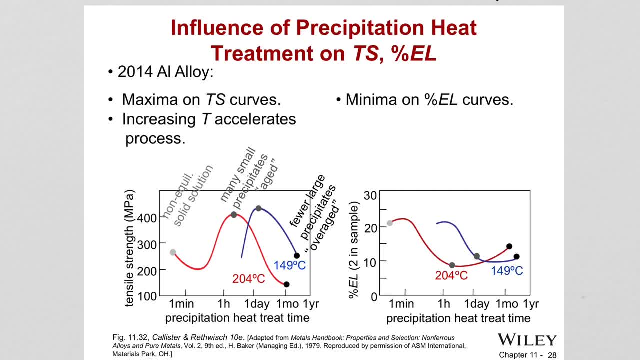 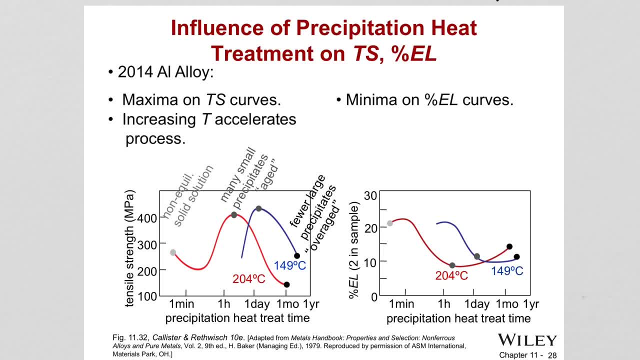 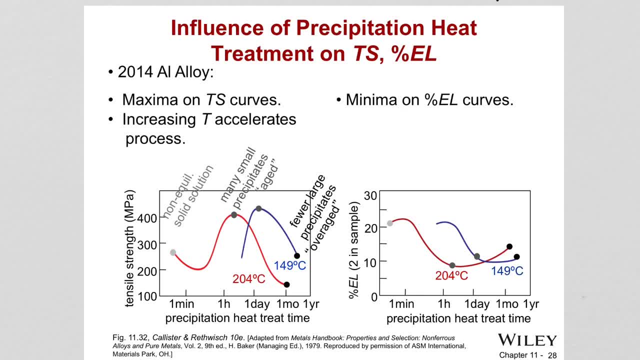 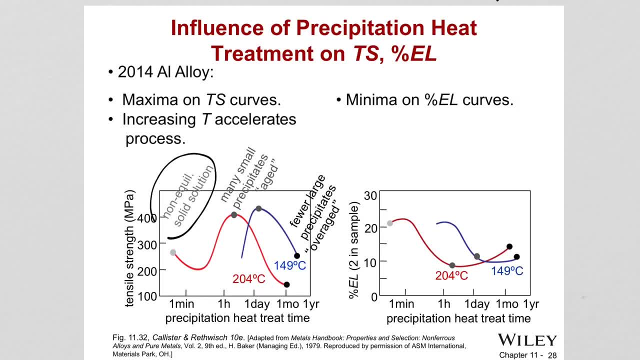 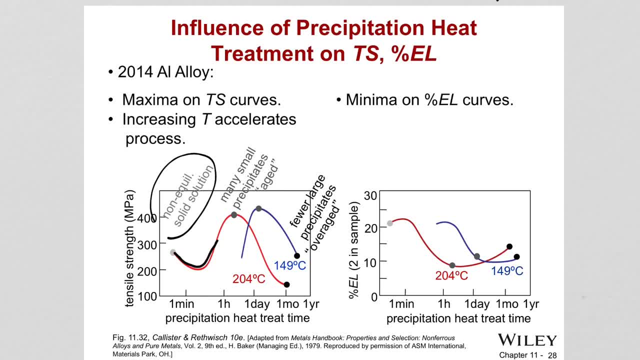 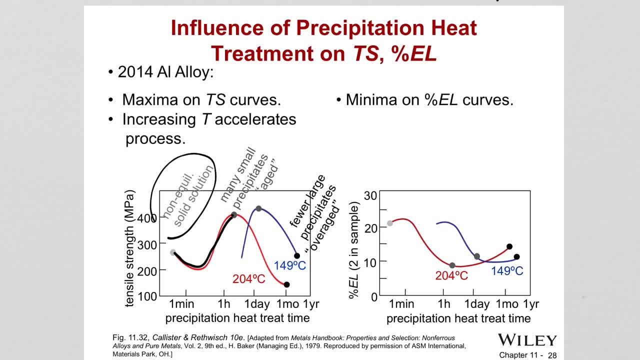 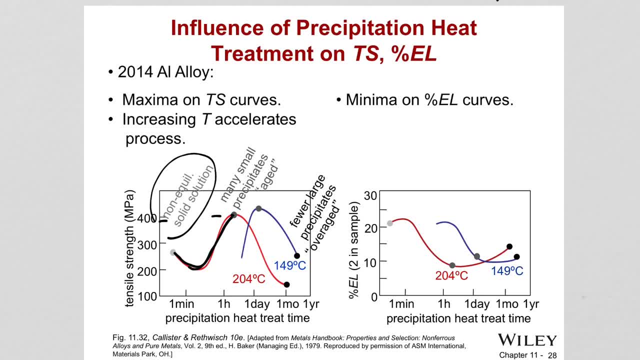 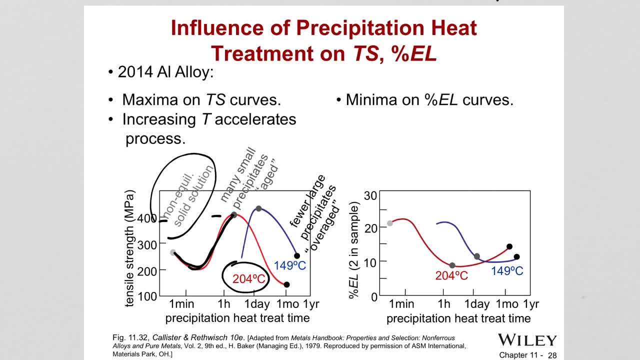 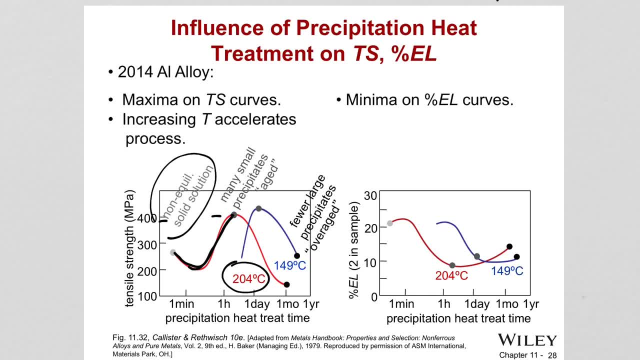 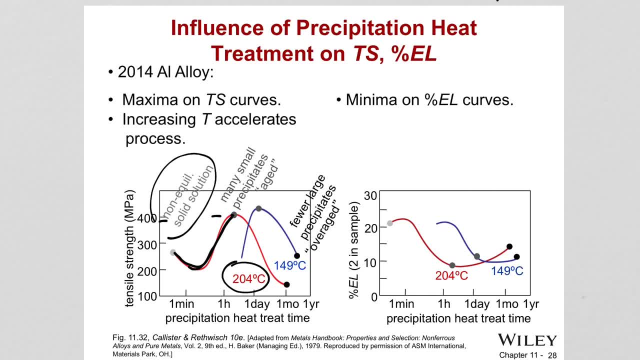 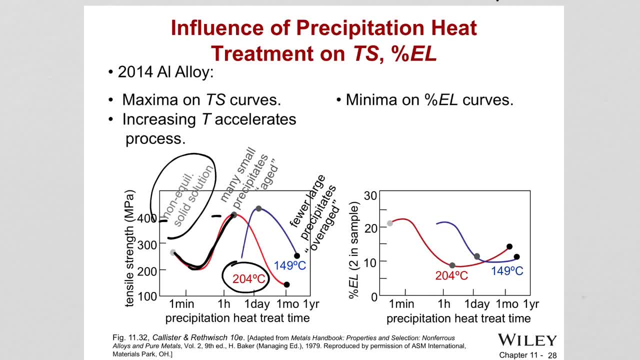 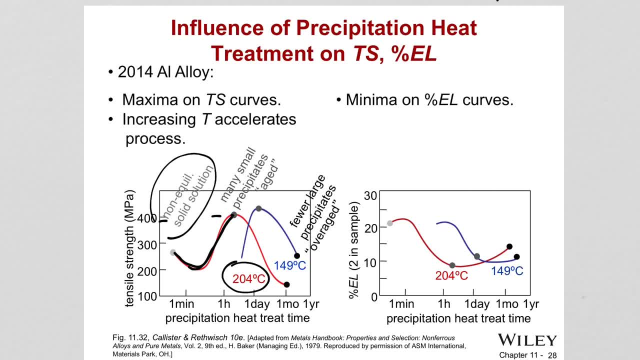 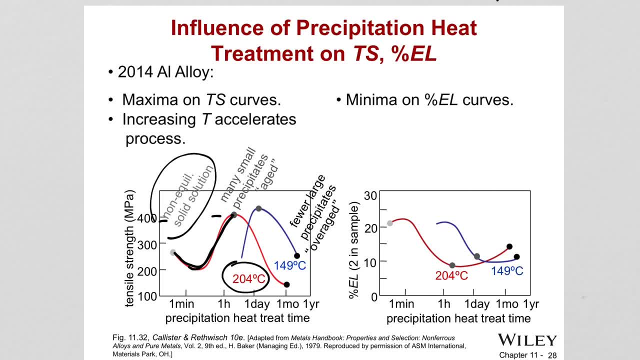 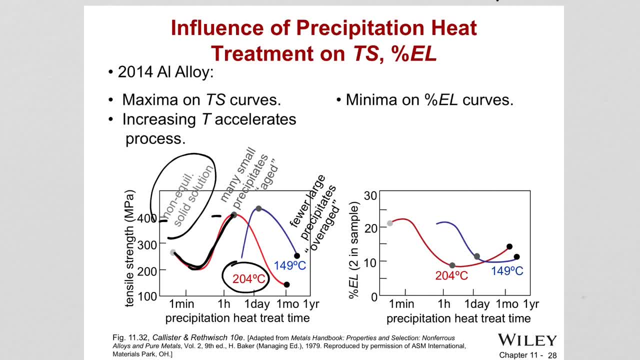 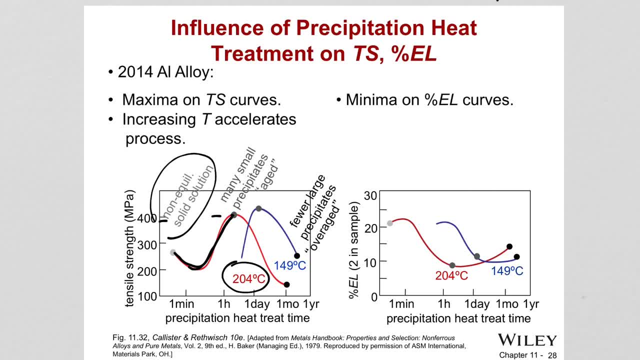 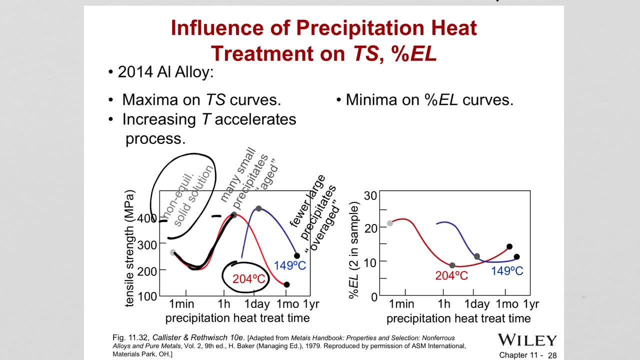 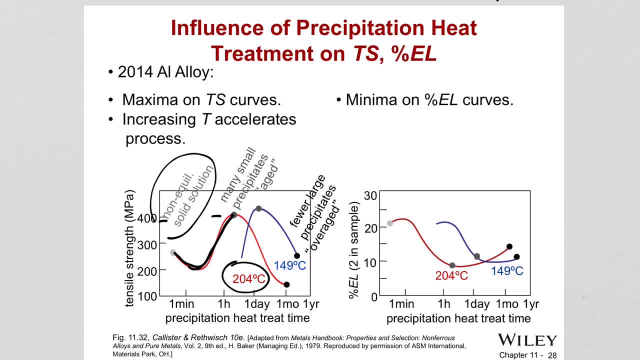 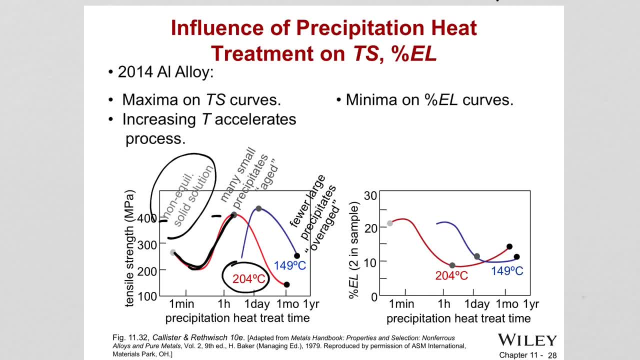 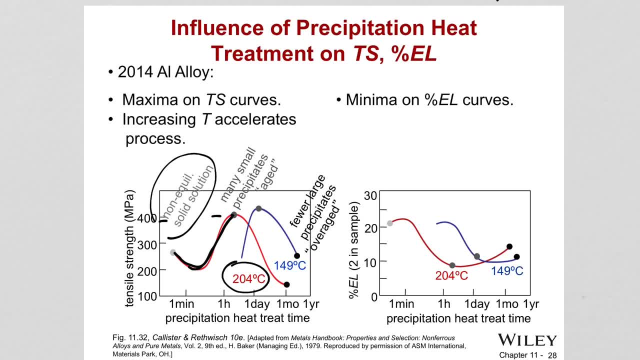 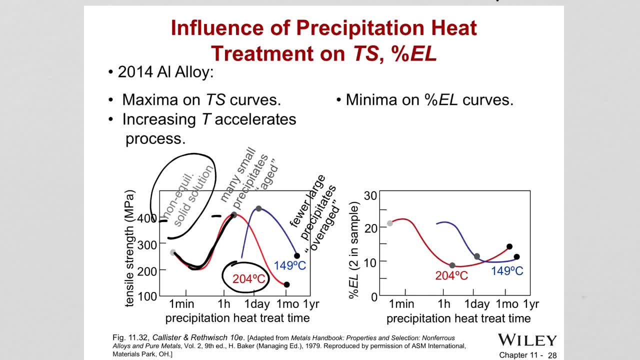 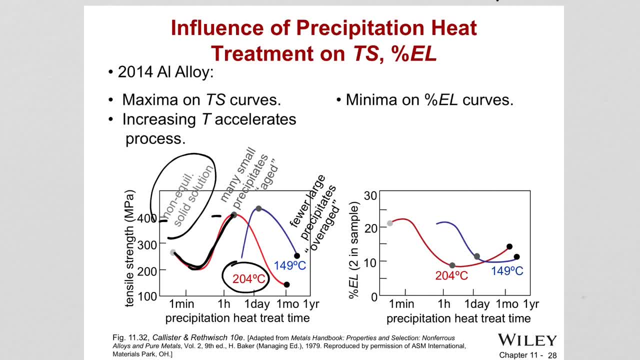 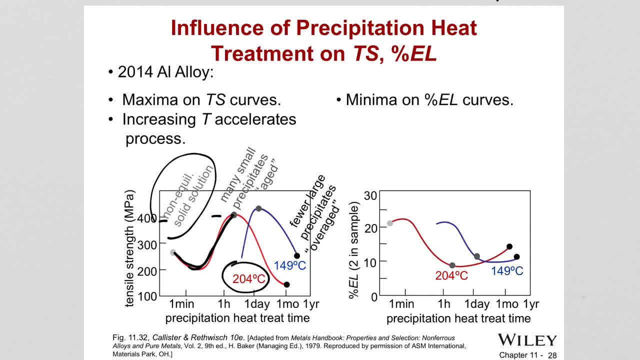 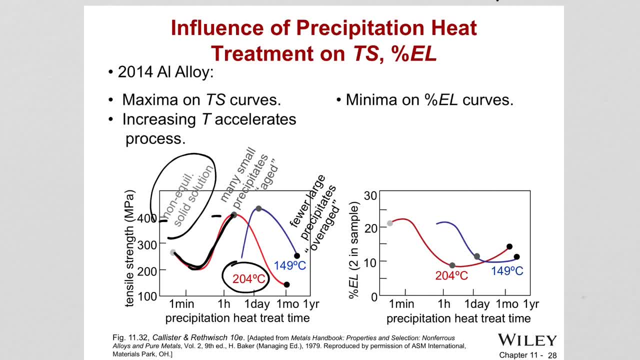 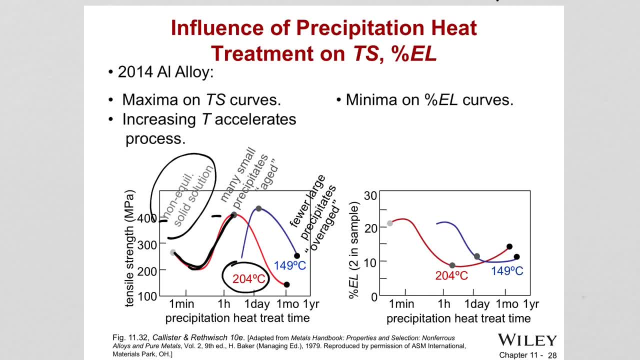 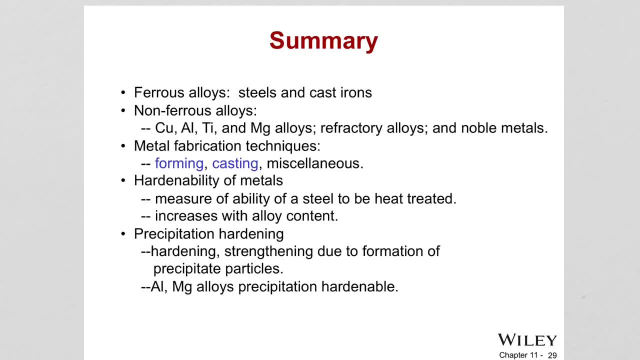 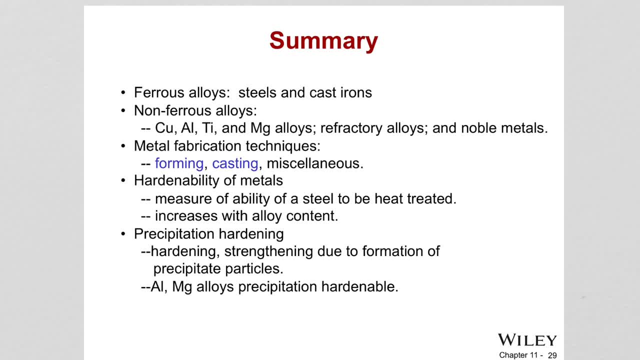 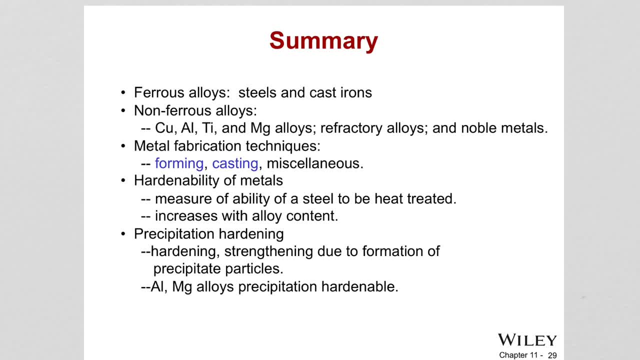 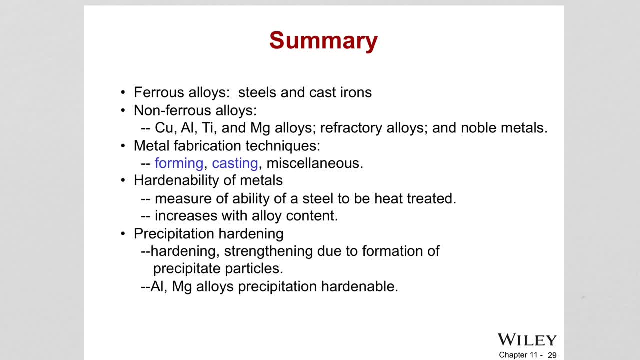 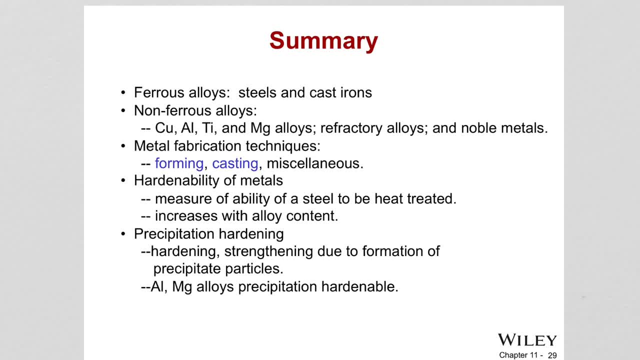 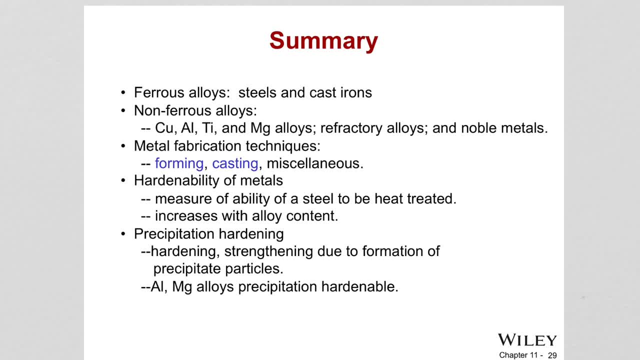 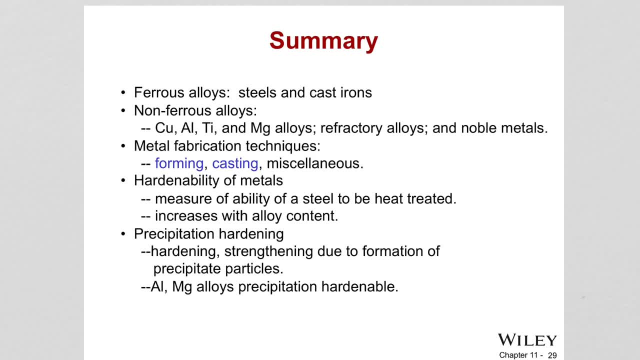 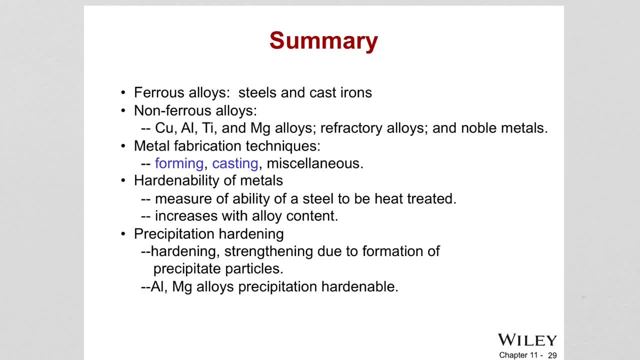 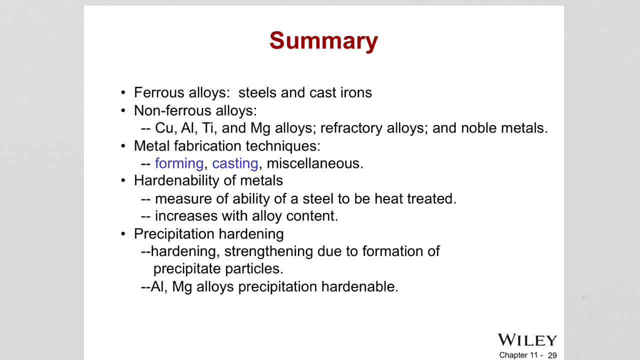 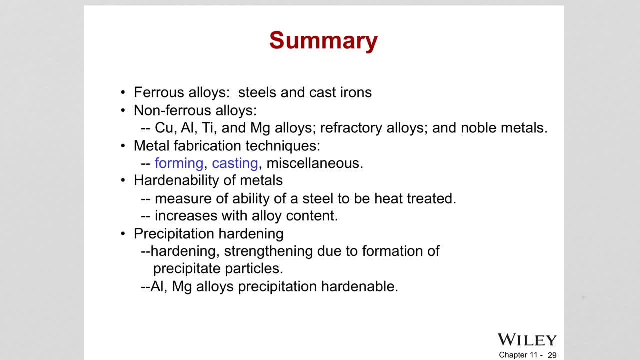 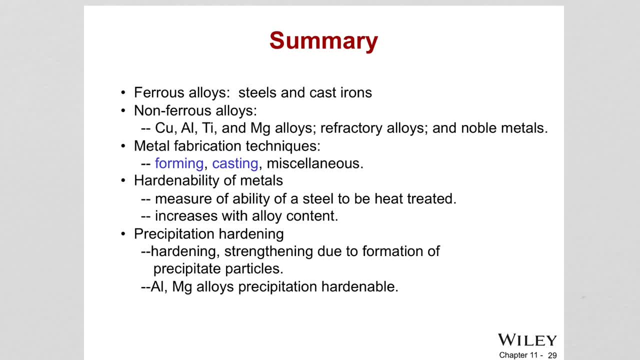 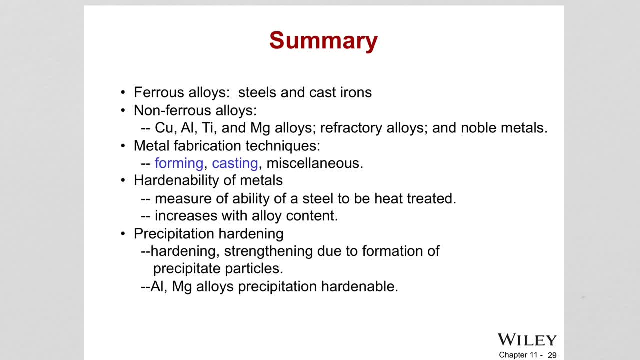 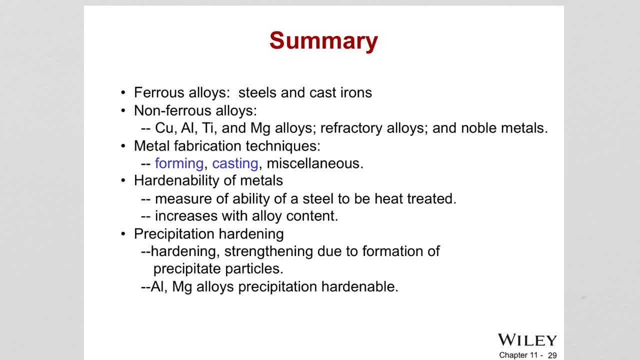 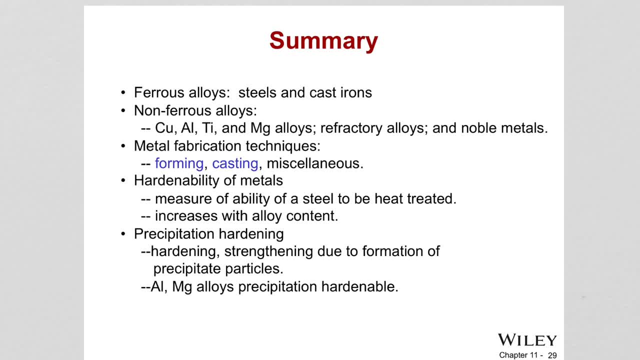 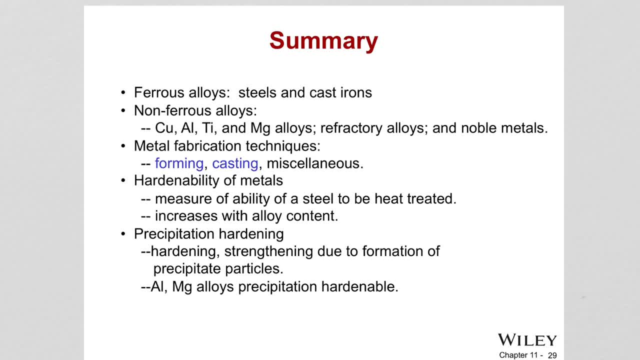